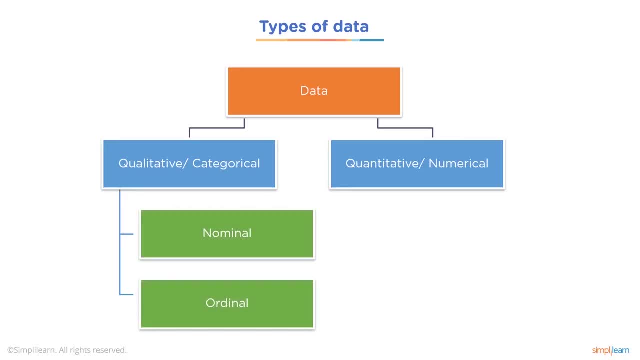 We have qualitative, categorical, When you think nominal or ordinal. then you have your quantitative or numerical, which is discreet or continuous, And let's look a little closer at those data types. Vocabulary: always people's favorite is the vocabulary words. Okay, not mine. 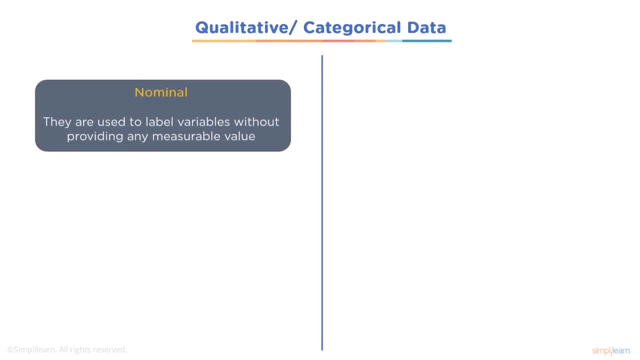 But let's dive into this what we mean by nominal Nominal. they are used to label our variables without providing any measurable value: Country, gender, race, hair color, etc. It's something that you either mark true or false. 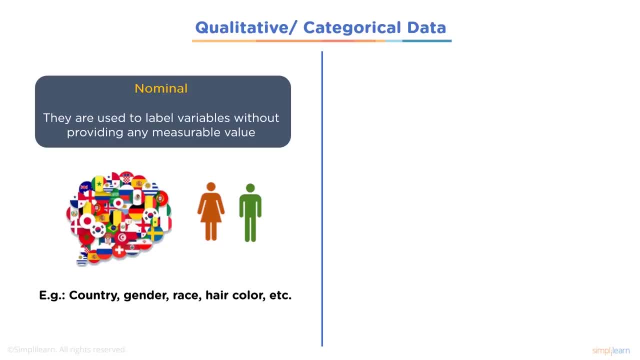 This is a label. It's on or off. Either they have a red hat on or they do not. A lot of times, when you're thinking nominal data labels, think of it as a true-false kind of setup. When we look at ordinal, this is categorical data with a set order or a scale to it. 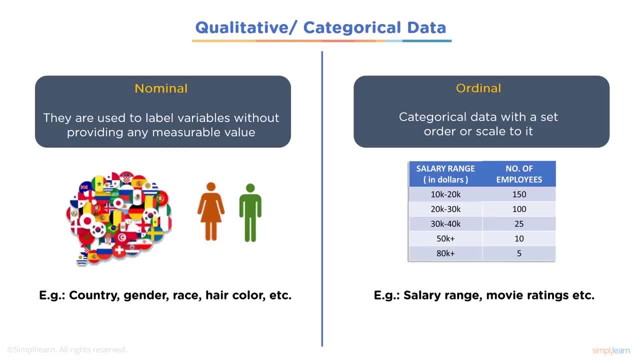 You can think of salary range as a great one, movie ratings, etc. You can see here the salary range. If you have $10,000 to $20,000, the number of employees earning that rate is $150,000.. $20,000 to $30,000,, $100,000, and so forth. 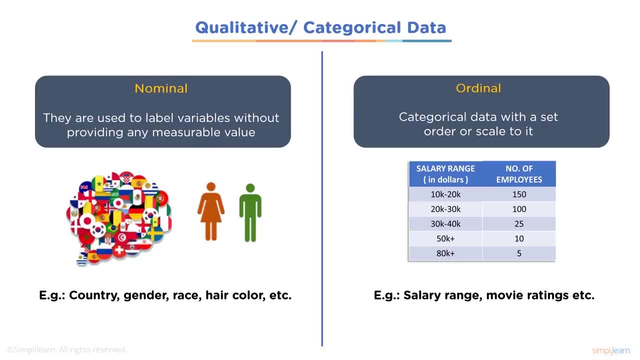 Some of the terms you'll hear is bucket. This is where you have 10 different buckets and you want to separate it into something that makes sense, into those 10 buckets. And so when we start talking about ordinal, a lot of times when you get down to the brass bones again, we're talking true-false. 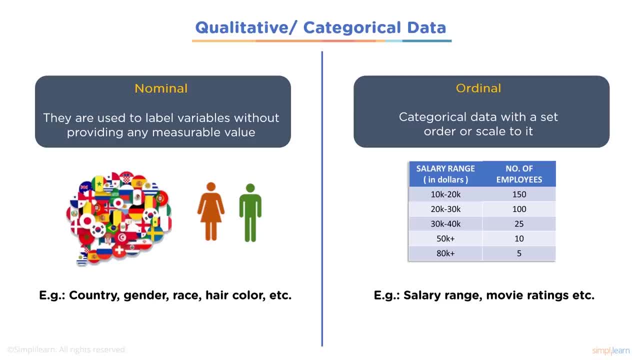 So if you're a member of the $10,000 to $20,000 range, so forth, Those would each be either part of that group or you're not. But now we're talking about buckets and we want to count how many people are in that bucket. 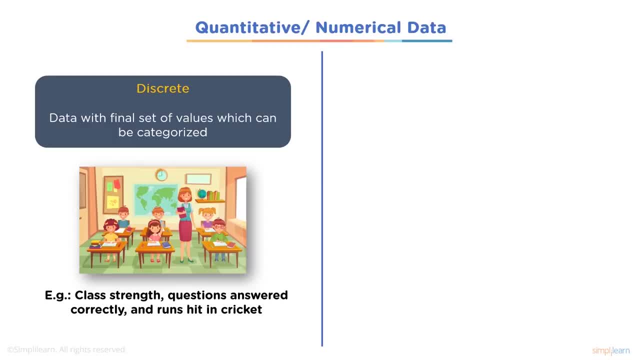 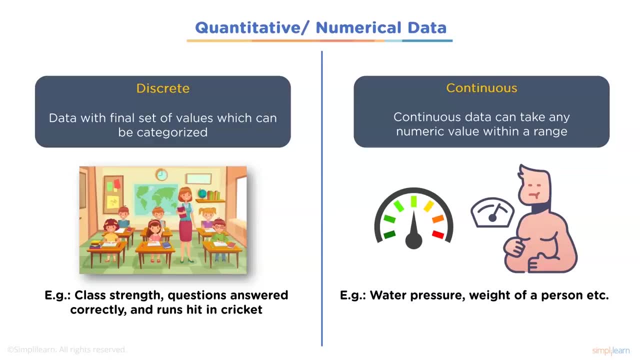 Quantitative numerical data. Quantitative numerical data falls into two classes: discrete or continuous, And so data with a final set of values which can be categorized- Class strength, questions answered correctly and runs hit and cricket A lot of times. when you see this, you can think integer and a very restricted integer. 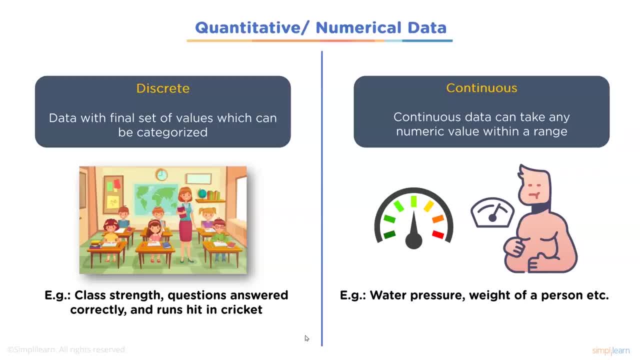 Ie. you can only have 100 questions on a test, so it's very discrete. I only have 100 different values that it can attain. So usually you're talking about integers, But within a very small range. they don't have an open-end or anything like that. 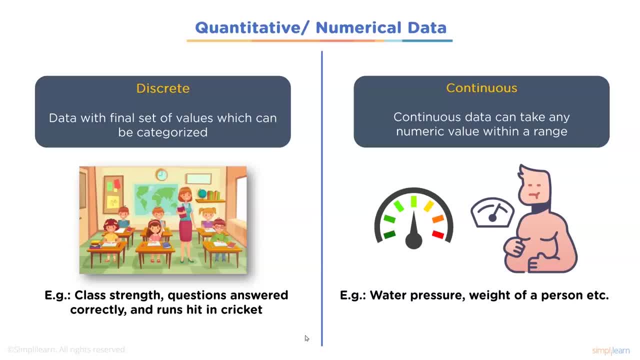 So discrete is very solid, Simple to count, set number, Continuous. on the other hand, continuous data can take any numerical value within a range, So water pressure, weight of a person, etc. Usually we start thinking about float values, where they can get phenomenally small in what they're worth. 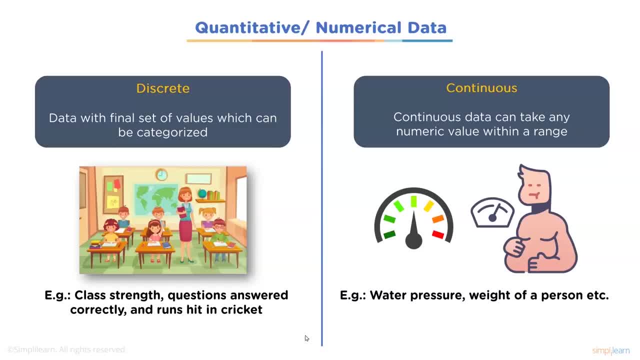 And there's a whole series of values that falls right between discrete and continuous. You can think of the stock market. You have dollar amounts, It's still discrete, but it starts to get complicated enough when you jump in the stock market from $525.33 to $580.67.. 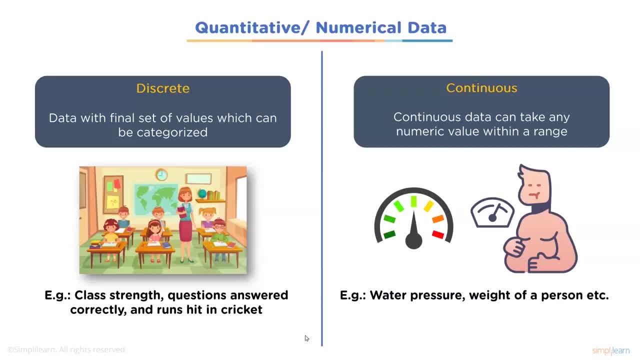 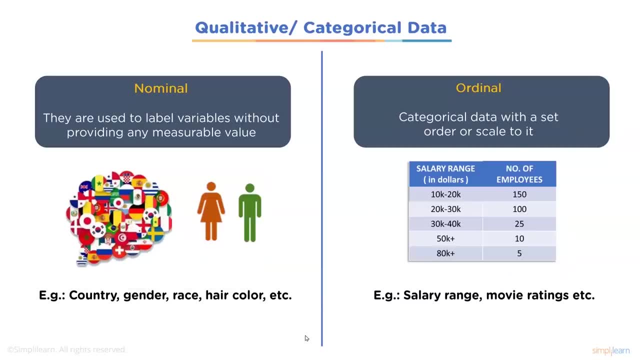 There's a lot of point values in there. It'd still be called discrete, but you start looking at it as almost continuous because it does have such a variance in it. Now we talked about, we went over nominal and ordinal, Almost true-false charts. 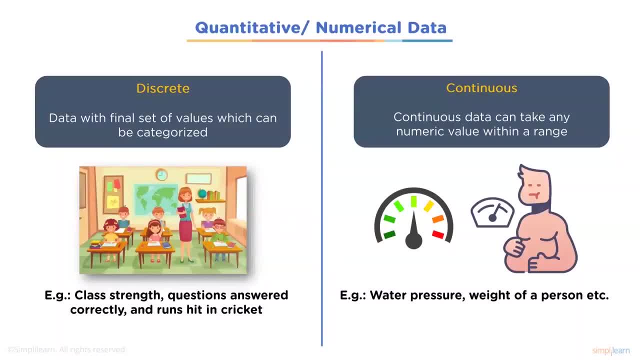 And we looked at quantitative and numerical data which we're starting to get into numbers Discrete- you can usually a lot of times discrete will be put into, could be put into true-false, but usually it's not. So we want to address this stuff and the first thing we want to look at is the very basic, which is your algebra. 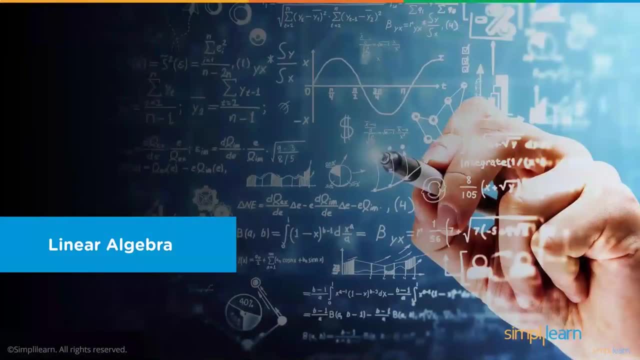 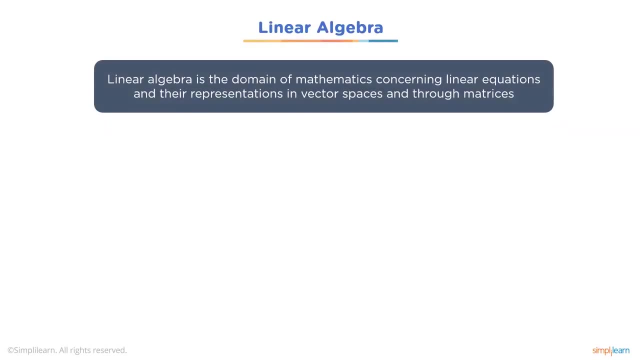 So we're going to take a look at linear algebra. You can remember back when your Euclidean geometry. We have a line. Well, let's go through this. We have a linear algebra. It's the domain of methods, It's the domain of numbers. 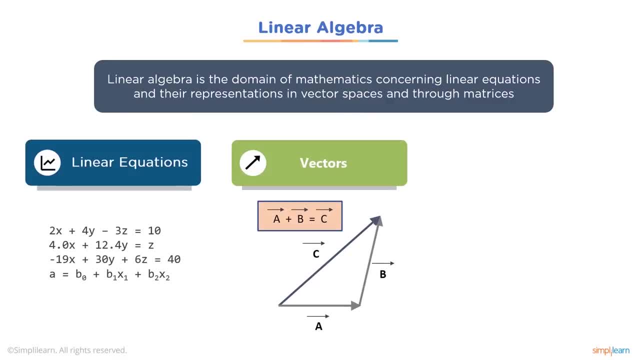 It's the domain of mathematics concerning linear equations and their representations in vector spaces and through matrices. I told you we were going to talk about matrices, So a linear equation is simply: 2x plus 4y minus 3z equals 10.. 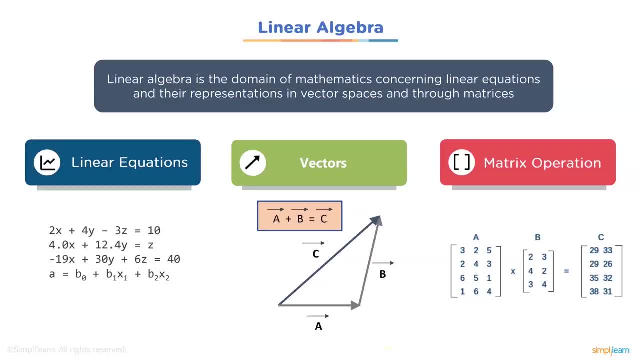 Very linear: 10x plus 12.4y equals z. And now you can actually solve these two equations by combining them, And that's why we're talking about a linear equation, And the vectors we have: a plus b equals c. 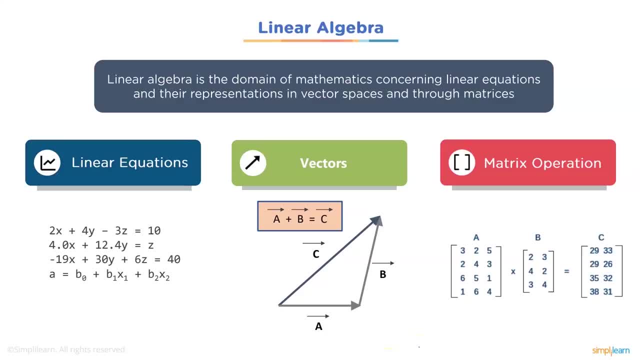 Now we're starting to look at a direction, And these values usually think of an x, y, z plot. So each one is a direction, And the actual distance of like a triangle, a, b is c, And then your matrix can describe all kinds of things. 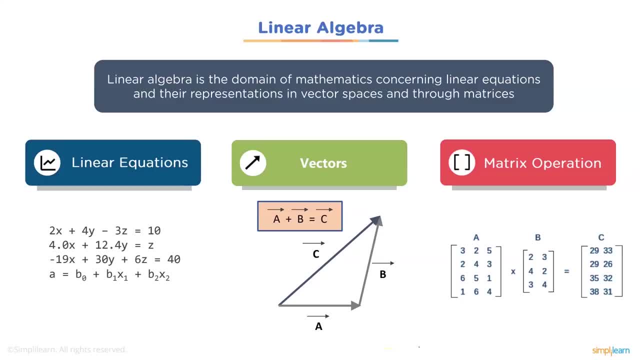 I find matrices confuse a lot of people, not because they're particularly difficult, but because of the magnitude and the different things they're used for. And a matrix is a chart or a- you know, think of a spreadsheet- but you have your rows and your columns. 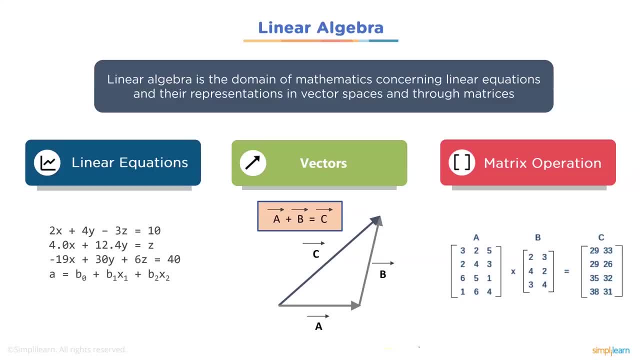 And you'll see here we have a times b equals c, Very important to know your counts. So, depending on how the math is being done and what you're using it for, making sure you have the same rows and number of columns or a single number. 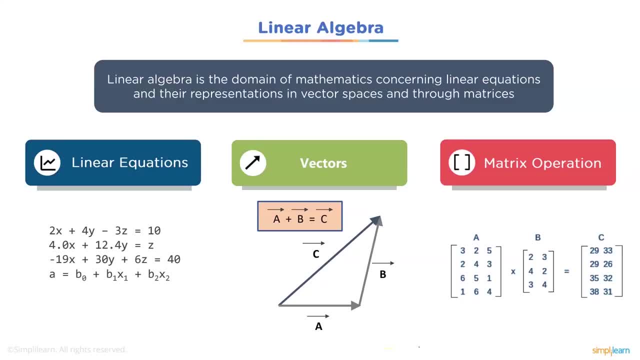 There's all kinds of things that play in that that can make matrices confusing, But really it has a lot more to do with what domain you're working in. Are you adding in multiple polynomials where you have like a, x squared plus b, y plus you know? 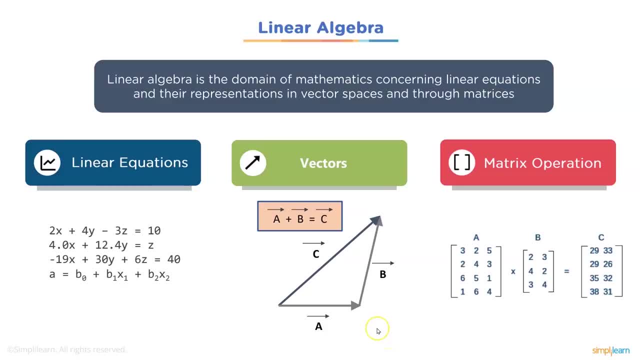 you start to see that it can be very confusing versus a very straightforward matrix, And let's just go a little deeper into these because these are such primary. this is what we're here to talk about is these different mathematical computations that come up. So we're looking at linear equations. 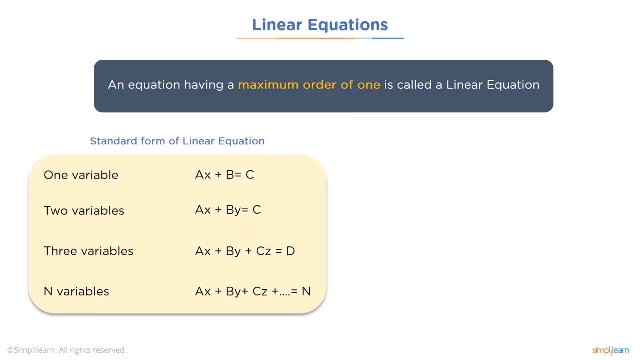 Let's dig deeper. Let's dig deeper into that one. An equation having a maximum order of one is called a linear equation. So it's linear because when you look at this, we have ax plus b equals c, which is a: one variable. 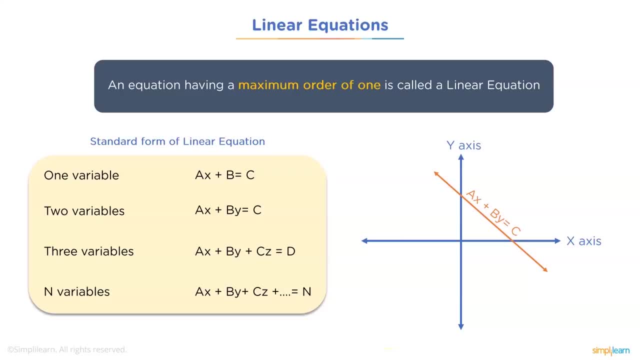 We have two variables: ax plus b, y equals c, ax plus b, y plus c, cz equals d and so forth. But all of these are to the power of one. You don't see x squared, You don't see x cubed. 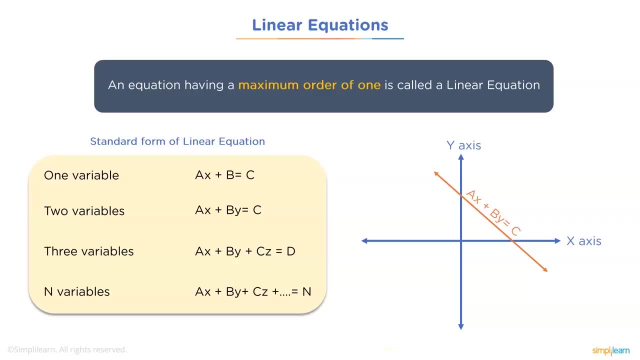 So when we're talking about linear equations, that's what we're talking about. In their addition, if you have already dived into, say, neural networks, you should recognize this: ax plus b, y plus c, z setup plus the intercept, which is basically your neural network, each node adding up all the different inputs. 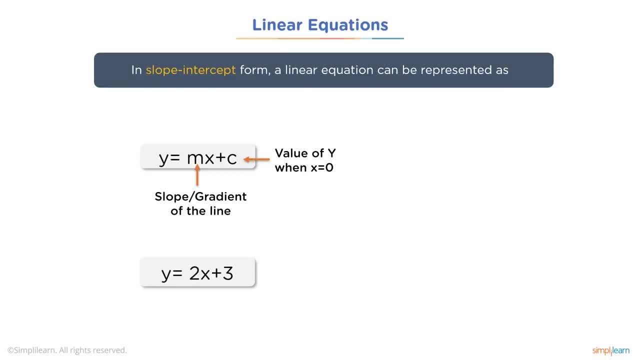 And we can drill down into that. Most common formula is: your y equals mx plus c. So you have your y equals the m, which is your slope, Your x value plus c, which is your y intercept. I kind of labeled it wrong here. 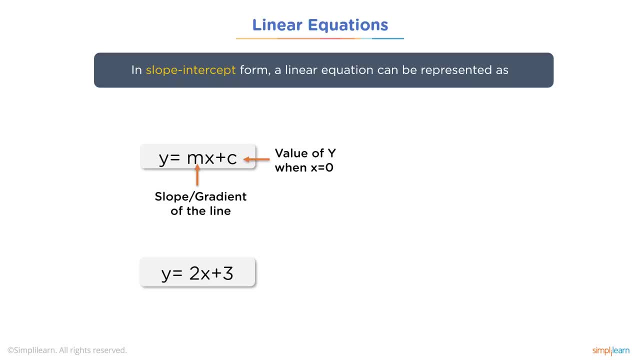 Threw me for a loop, But the c would be your y intercept. So when you set x equal to 0, y equals c And that's your y intercept, right there, And they just had a reverse value of y. when x equals 0 equals the y intercept, which is c. 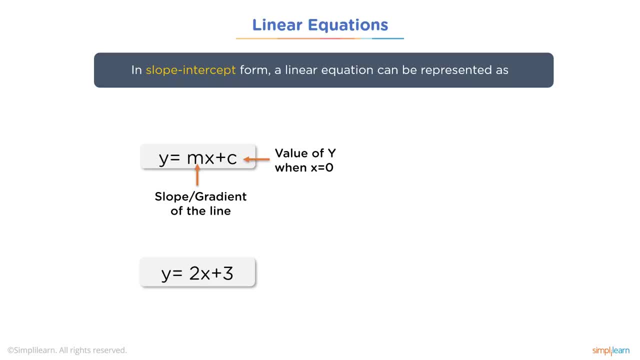 And your slope gradient line, which is your m. So you get your y equals 2x plus 3.. And there's lots of easy ways to compute this. This is why we always start with the most basic one when we're solving one of these problems. 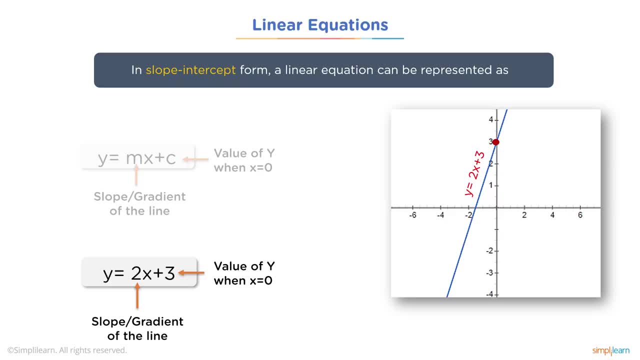 And then, of course, one of the most important takeaways is the slope gradient of the line. So the slope is very important. that m value In this case. we went ahead and solved this. If you have, y equals 2x plus 3, you can see how it has a nice line graph here on the right. 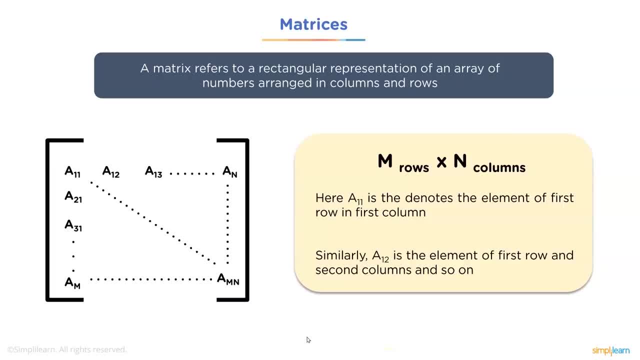 So matrixes? A matrix refers to a rectangular representation of an array of numbers arranged in columns and rows, So we're talking m rows by n columns. Here, a11 denotes the element of the first row and the first column, Similarly a12, and it's really pronounced a11 in this particular setup. 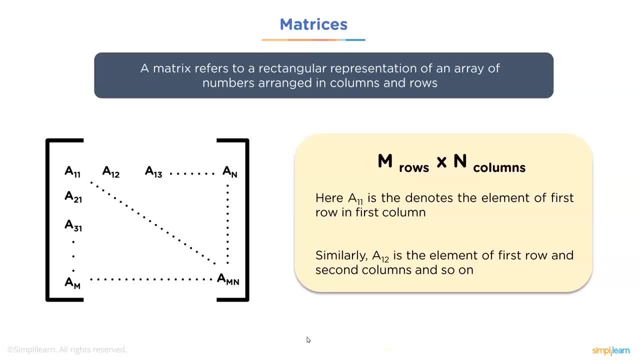 So it's row 1, column 1.. a12 is a row 1, column 2.. First row and second column and so on, And there's a lot of ways to denote this. I've seen these as like a capital letter, A smallercase a for the top row. 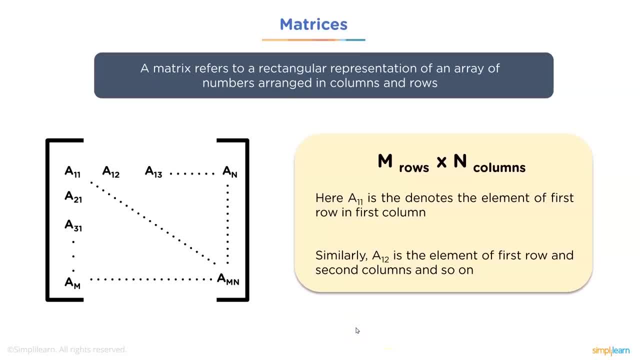 Or I mean you can see where they can go, all kinds of different directions. as far as the value, You just take a moment to realize. there needs to be some designation as far as what row it's in and what column it's in. 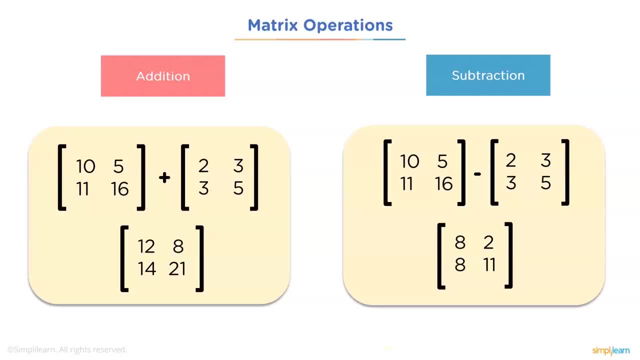 And we have our basic operations, We have addition. So when you think about addition, you have two matrices of 2x2.. And you just add each individual number in that matrix And then, when you get to the bottom, you have- in this case, the solution is 12.. 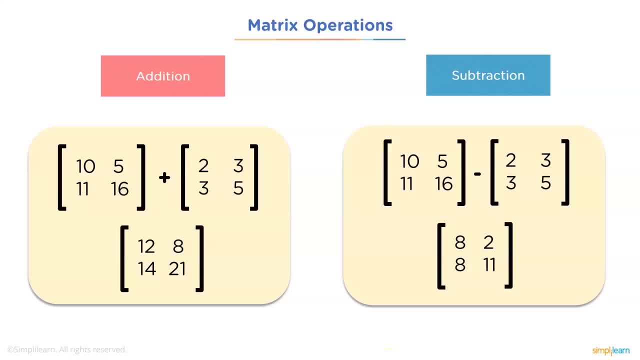 10 plus 2 is 12.. 5 plus 3 is 8. And so on And the same thing with subtraction. Now again, you're counting matrices. You want to check your dimensions of the matrix, The shape. 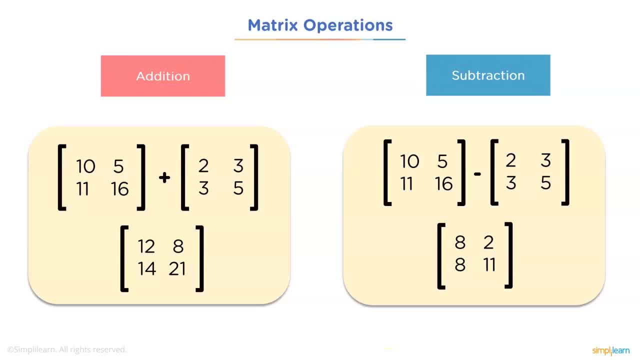 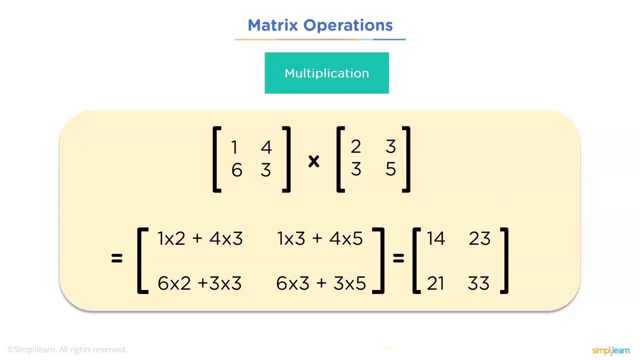 You'll see shape come up a lot in programming. So we're talking about dimensions, We're talking about the shape. If the two shapes are equal, this is what happens when you add them together or subtract them And we have multiplication. When you look at the multiplication, you end up with a very slightly different setup going. 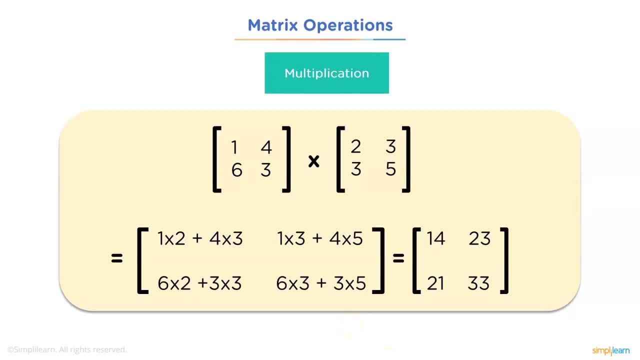 Now, if we look at our last one, we're like why? This always gets to me when we get to matrices, because they don't really say why you multiply matrices. You know, my first thought is: 1 times 2,, 4 times 3.. 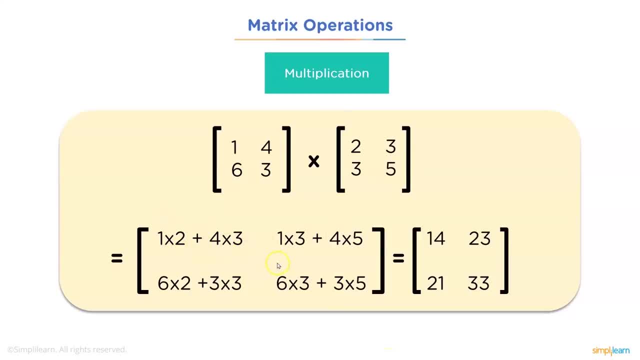 But if you look at this, we get 1 times 2 plus 4 times 3.. 1 times 3 plus 4 times 5.. 6 times 2 plus 3 times 3.. 6 times 3 plus 3 times 5.. 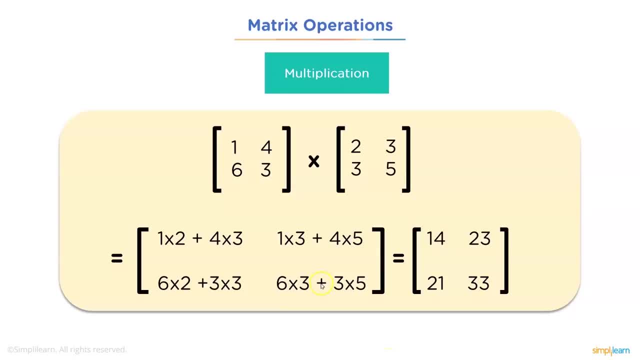 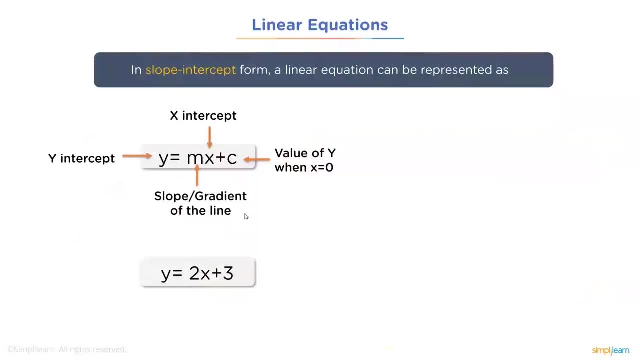 If you're looking at these matrices, think of this more as an equation, And so we have. if you remember when we went back up here for our multiple line equations, Let's just go back up a couple slides where we were looking at a 2 variable. 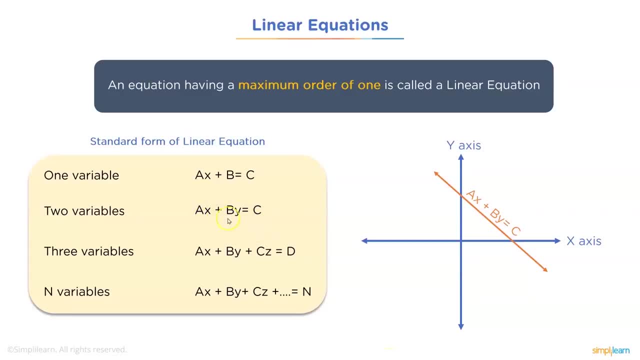 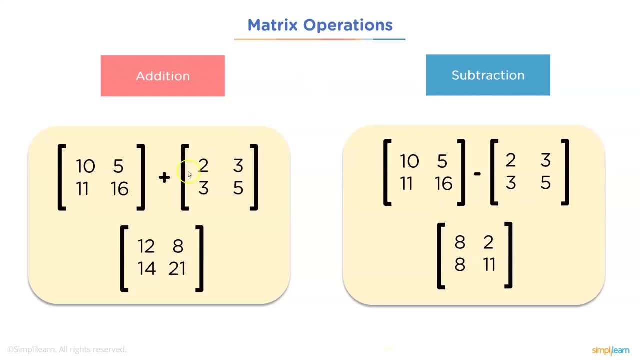 So this is a 2 variable equation, Ax plus By equals C, And this is a way to make it very quick to solve these variables, And that's why you have the matrix And that's why you do the multiplication the way they do. 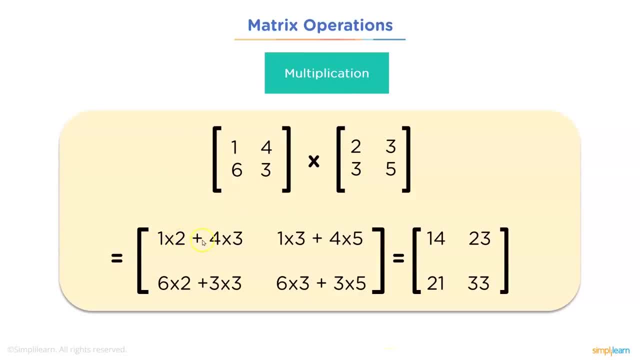 And this is the dot product of 1 times 2 plus 4 times 3.. 1 times 3 plus 4 times 5.. 6 times 2 plus 3 times 3.. 6 times 3 plus 3 times 5.. 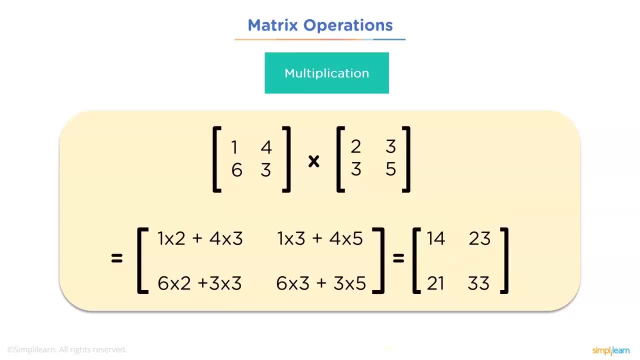 And it gives us a nice little 14,, 23,, 21, and 33 over here, Which then can be used and reduced down to a sample. So that's the formula as far as solving the variables, as you have enough inputs. 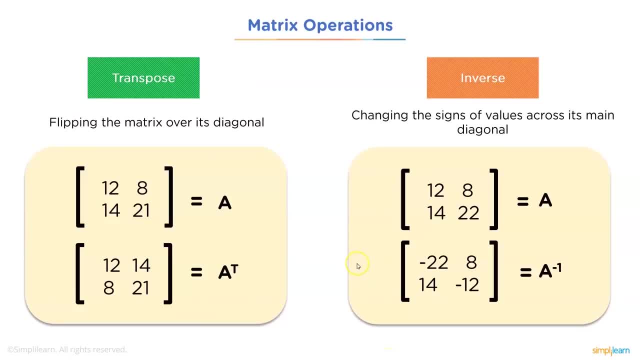 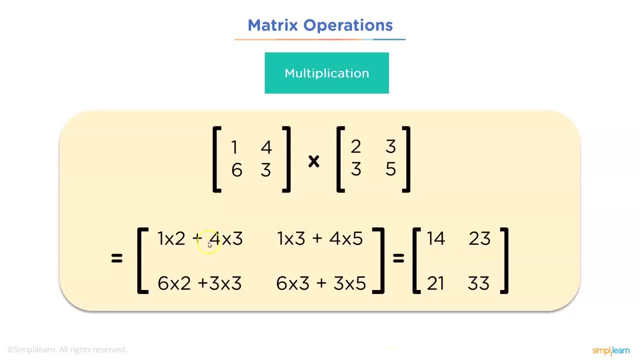 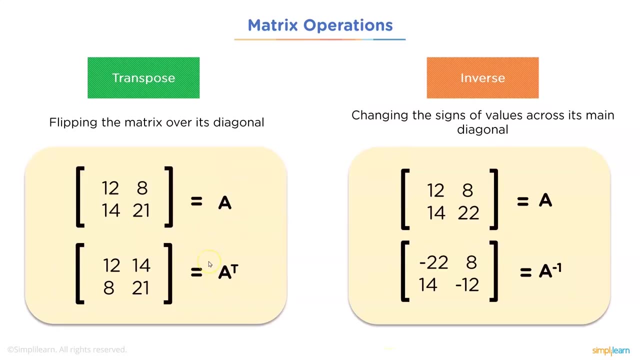 And then in matrix operations, when you're dealing with a lot of matrices. Now, keep in mind, multiplying matrices is different than finding the product of 2 matrices. So when we're talking about multiplication, we're talking about solving for equations. When you're finding the product, you are just finding 1 times 2.. 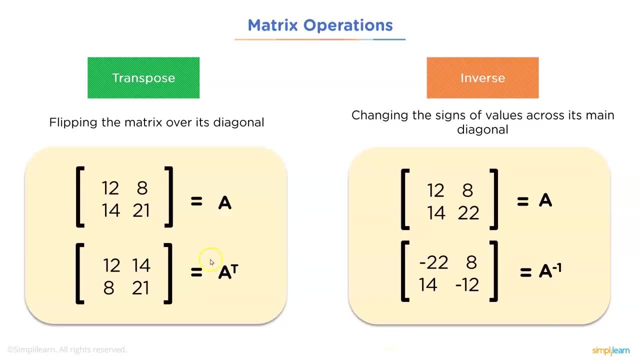 Keep that in mind because that does come up. I've had that come up a number of times where I'm altering data And I get confused as to what I'm doing with it. Transpose, Flipping the matrix over its diagonal Comes up all the time. 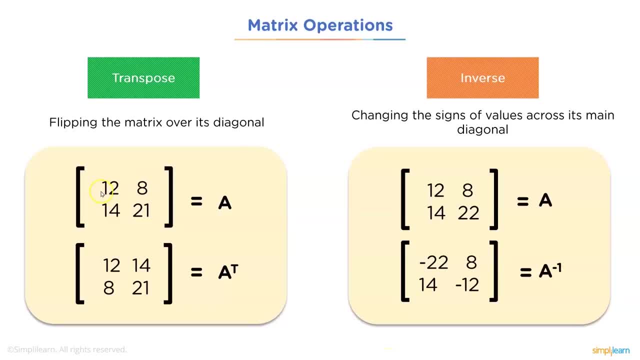 Where you still have 12,, but instead of it being 12, 8,, it's now 12, 14, 8, 21.. You're just flipping the columns and the rows, And then, of course, you can do an inverse. 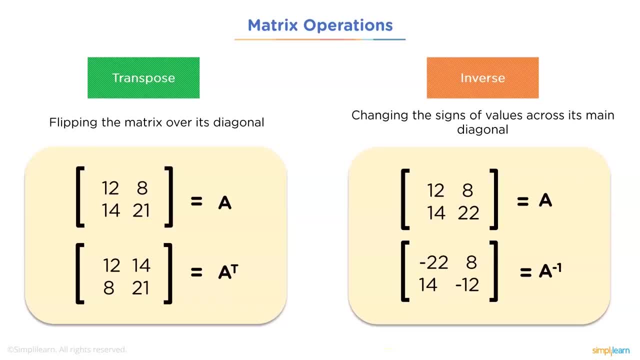 Changing the signs of the values across its main diagonal, And you can see here we have the inverse 8 to the minus 1.. And it ends up with, instead of 12, 8,, 14, 12.. It's now minus 22,, minus 12.. 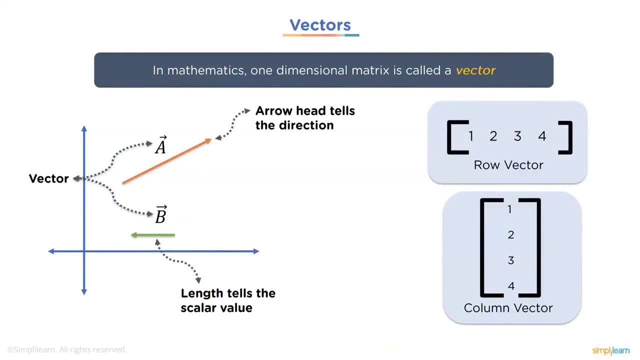 Vectors. Vector just means we have a value and a direction And we have down 4 numbers here on our vector. In mathematics a 1-dimensional matrix is called a vector. So if you have your x-plot and you have a single value, that value is along the x-axis. 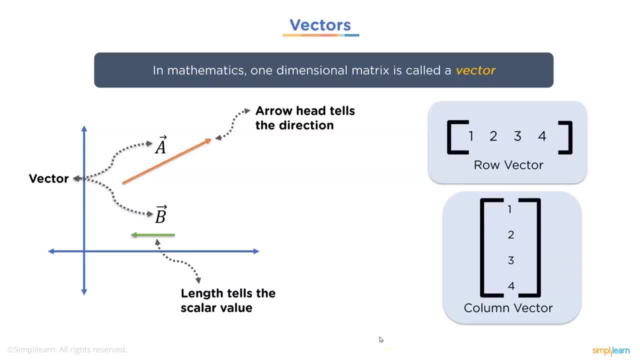 And it's a single dimension. If you have 2 dimensions, you can think about putting them on a graph. You might have x and you might have y, And each value denotes a direction, And then, of course, the actual distance is going to be the hypothesis of that triangle. 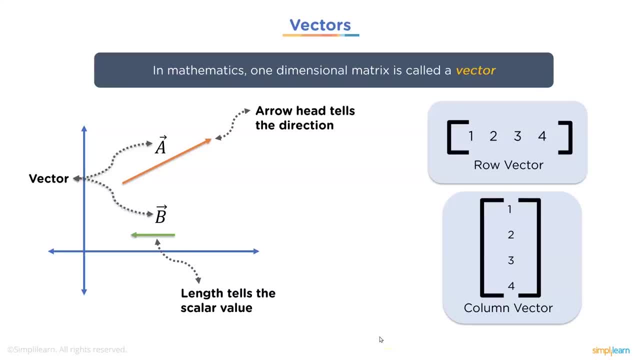 And you can do that with 3-dimensionals- x, y and z, And you can do it all the way to nth dimensions. So when they talk about the k-means for categorizing and how close data is together, they will compute that based on the Pythagorean theorem. 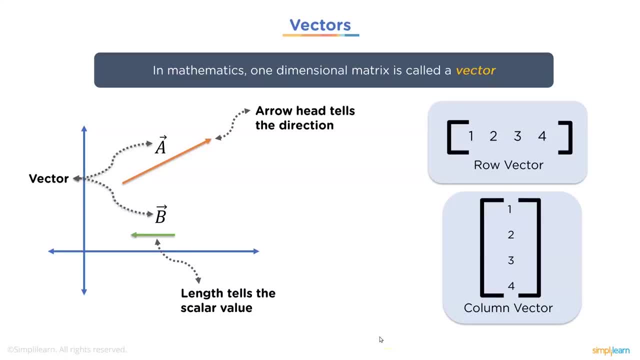 So you would take the square of each value, add them all together and find the square root, And that gives you a distance as far as where that point is, where that vector exists, or an actual point value, And then you can compare that point value to another one. 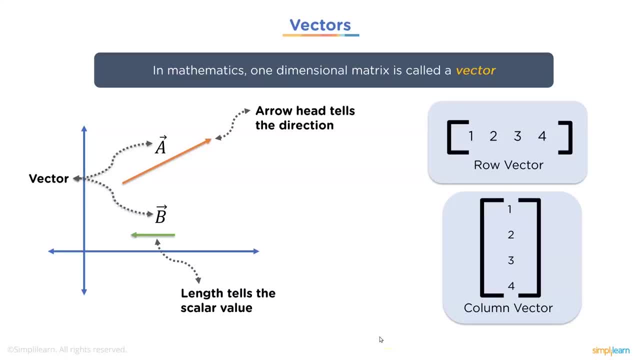 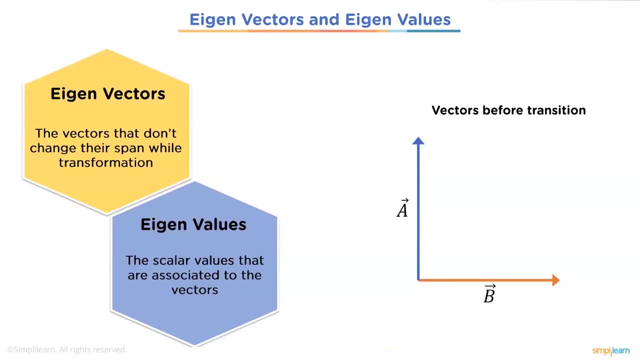 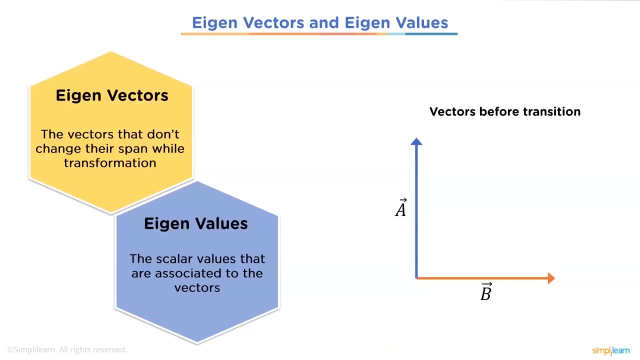 It makes a very easy comparison versus comparing 50 or 60 different numbers. And that brings us up to i-gene vectors and i-gene values. i-gene vectors: the vectors that don't change their span while transformation, And i-gene values, the scalar values. 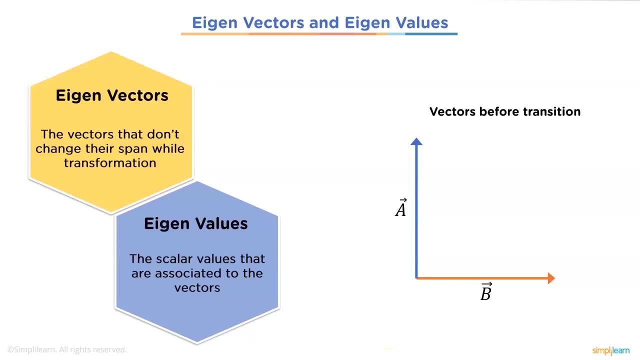 that are associated to the vectors. Conceptually, you can think of the vector as your picture. You have a picture. it's 2 dimensions, x and y, And so when you do those 2 dimensions and those 2 values or whatever that value is, that is that point. 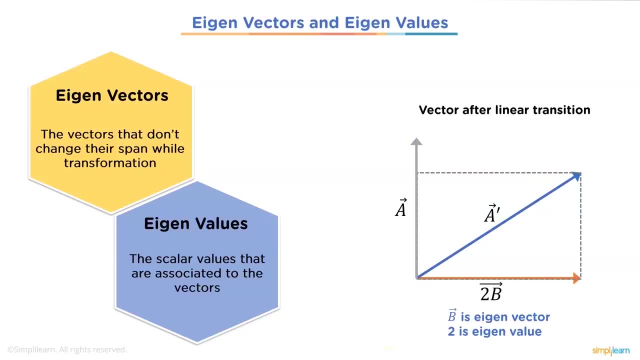 But the values change when you skew it. And so if we take and we have a vector a and that's a set value, you have a and b, which is your i-gene vector 2 is the i-gene value. 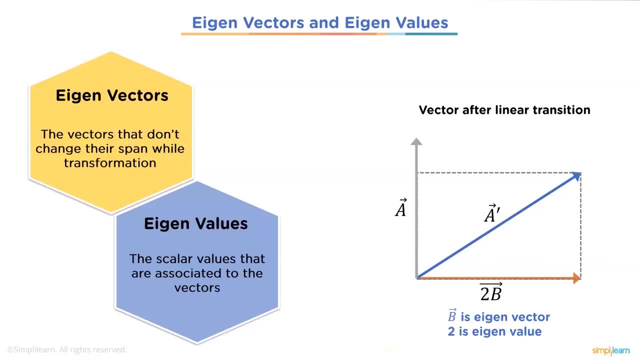 So we're altering all the values by 2. That means maybe we're stretching it out one direction, making it tall. if you're doing picture editing, That's one of the places this comes in, But you can see when you're transforming your different information. 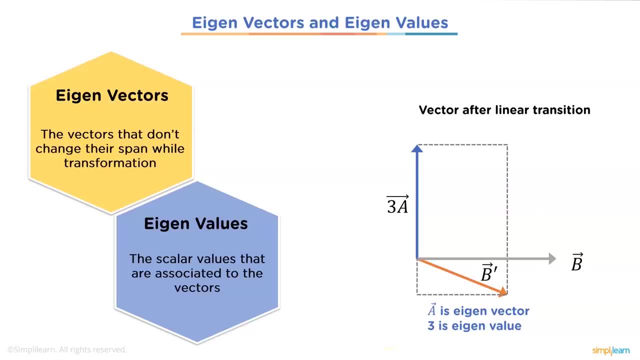 how you transform. it is then your i-gene value, And you can see here a vector after line transition. we have 3a. a is the i-gene vector, 3 is the i-gene value, So a doesn't change. 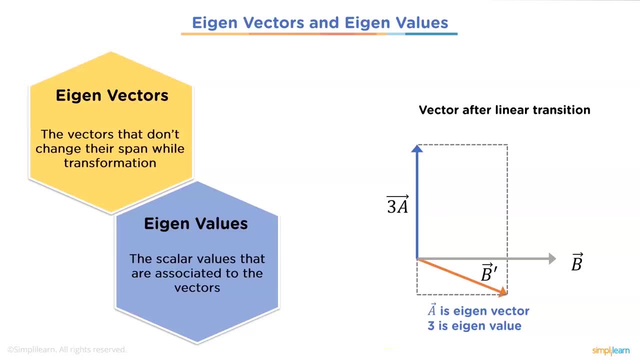 That's whatever we started with. That's your original picture, And 3 is skewing it one direction, And maybe b is being skewed another direction, And so you have a nice tilted picture because you've altered it by the i-gene values. 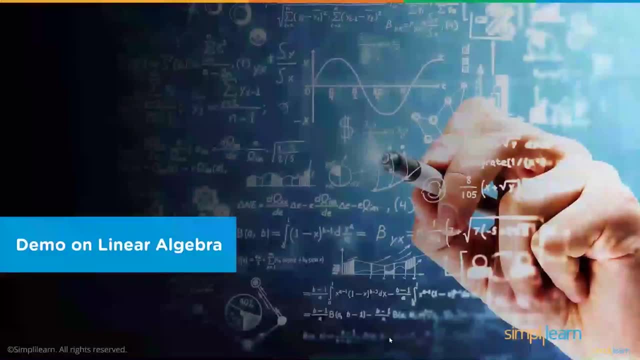 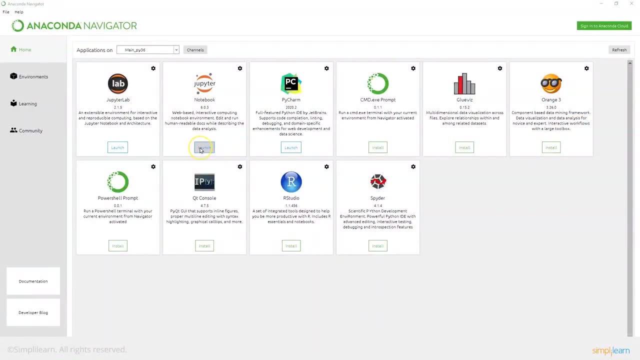 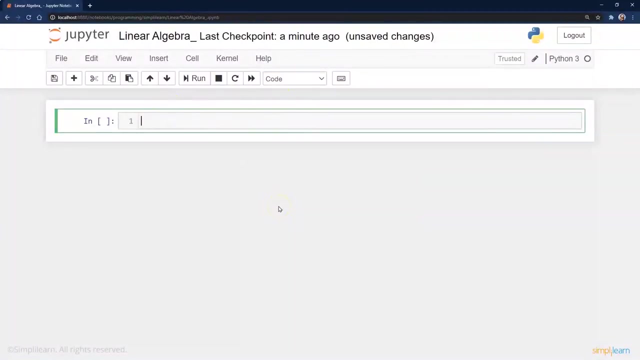 So let's go ahead and pull up a demo on linear algebra, And to do this, I'm going to go through my trusted Anaconda into my Jupyter notebook And we'll create a new notebook called Linear Algebra, Since we are working in Python. 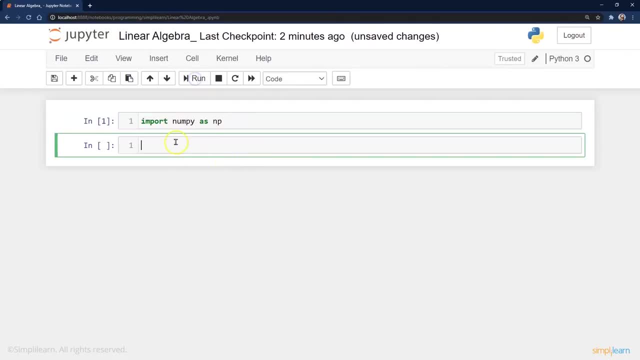 we're going to use our numpy. I always import that as np, our numpy array, Probably the most popular module for doing matrixes and things in. Given that this is part of a series, I'm not going to go too much into numpy. 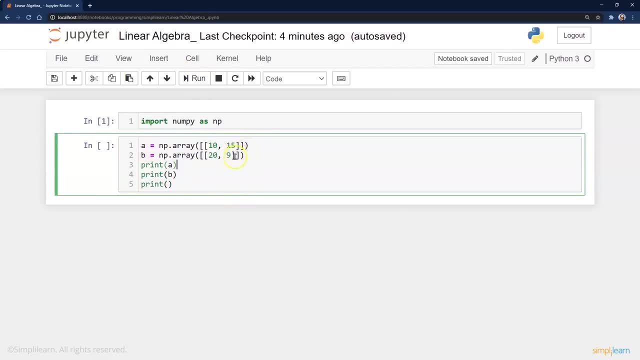 We are going to go ahead and create 2 different variables: a for a numpy array- 10, 15, and b 29. We'll go ahead and run this and you can see there's our 2 arrays: 10,, 15, 29.. 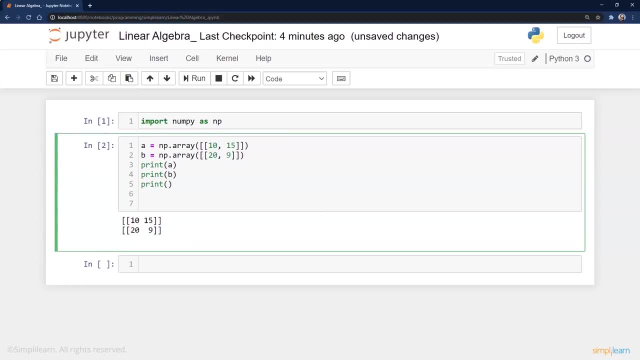 And I went ahead and added a space there in between so it's easier to read And since it's the last line, we don't have to put the print statement on it unless you want. but we can simply do a plus b. So when I run this, we have 10,, 15,, 29,. 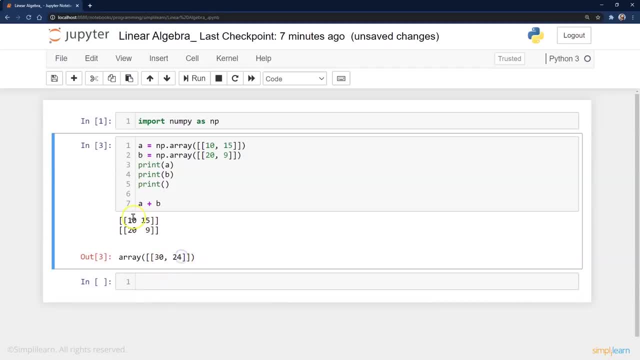 and we get 30,, 24, which is what you expect: 10 plus 20,, 15 plus 9.. You could almost look at this addition as being just adding up the columns on here coming down. And if we wanted to do it a different way? 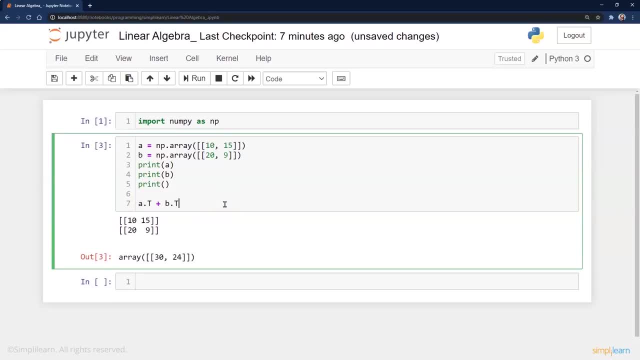 we could also do at plus bt. Remember that t flips them And so if we do that, we now get them. we now have 30, 24 going the other way. We could also do something kind of fun. There's a lot of different ways to do this. 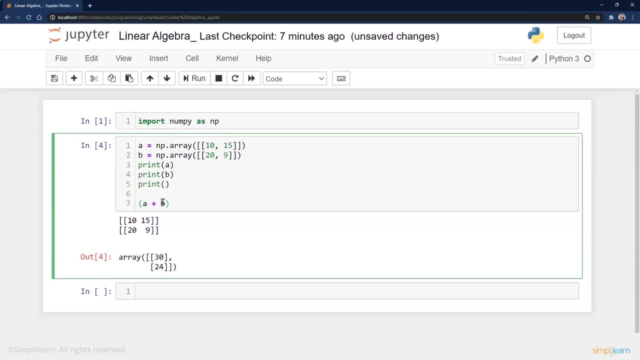 As far as a plus b, I can also do a plus b dot t, And you're going to see that that will come out the same- the 30, 24,, whether I transpose a and b or transpose them both at the end. 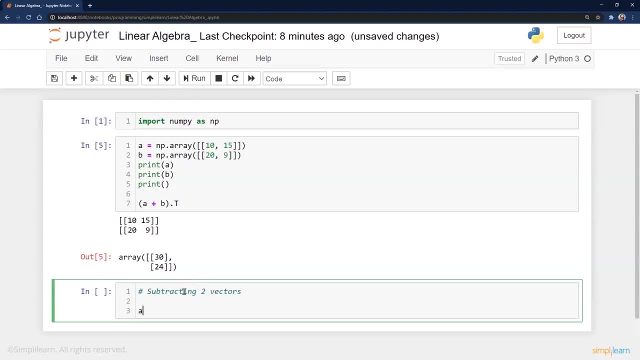 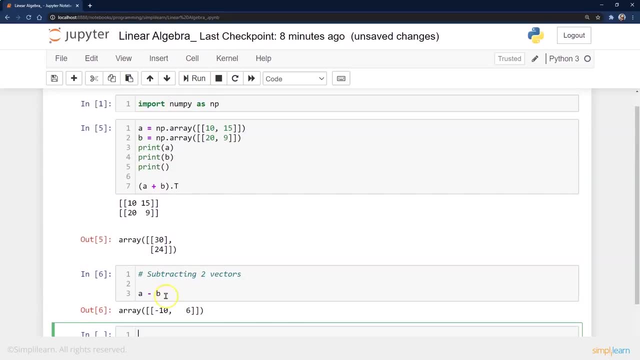 And likewise we can very easily subtract 2 vectors. I can go a minus b And we run that and we get minus 10, 6.. Now, remember, this is the last line in this particular section, And so I don't have to put the print around it. 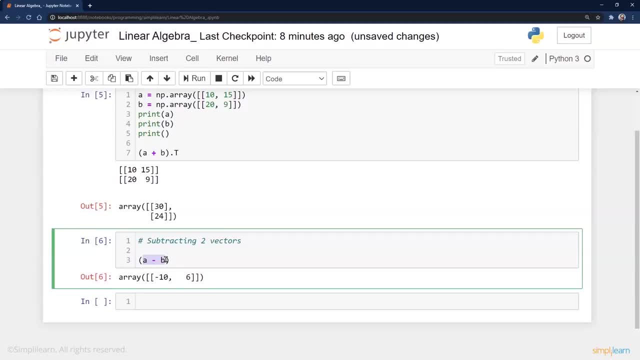 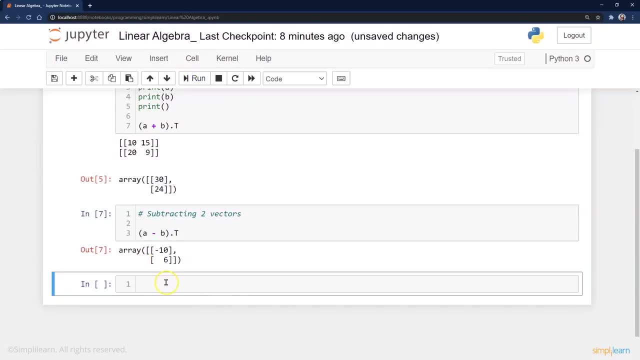 And, just like we did before, we can transpose either the individual or we can transpose the main setup, and then we get a minus 10, 6 going the other way. Now, we didn't mention this in our notes, but you can also do a scalar multiplication. 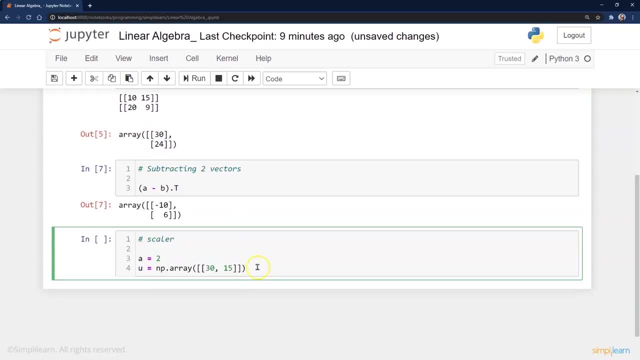 Let me just put down the scalar so you can remember that What we're talking about here is: I have this array here u, and if I go a times u, we'll take the value 2,. we'll multiply it by every value in here. 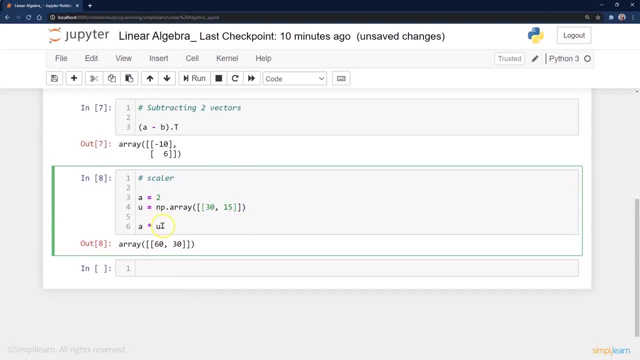 So 2 times 30 is 60.. 2 times 15.. And, just like we did before- this happens a lot because when you're doing matrixes you do need to flip them. You get 60, 30 coming this way. 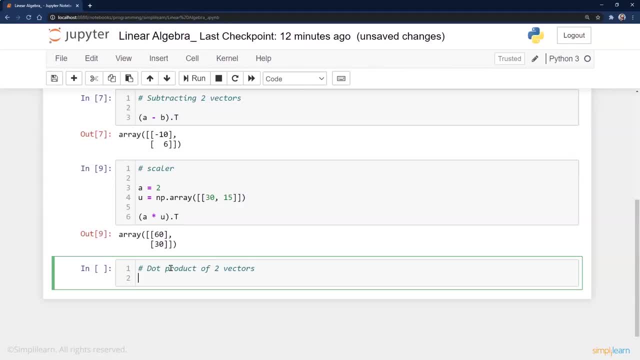 So in NumPy we have what they call dot product And with this this is in a two-dimensional vector. It is the equivalent of two matrix multiplication. Remember we were talking about matrix multiplication. where it is the well, let's walk through it. 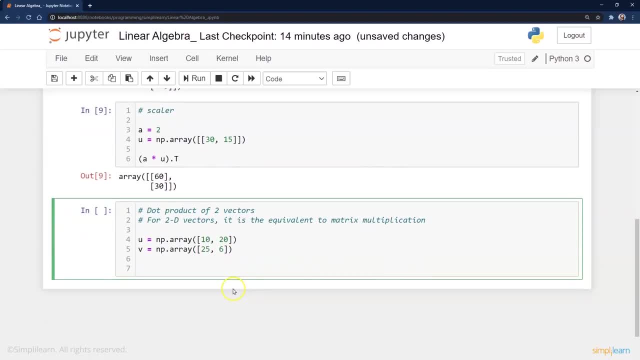 We'll go ahead and start by defining two NumPy arrays. We'll have 10,, 20,, 25, 6, for our u and our v, And then we're going to go ahead and do, if we take the values. 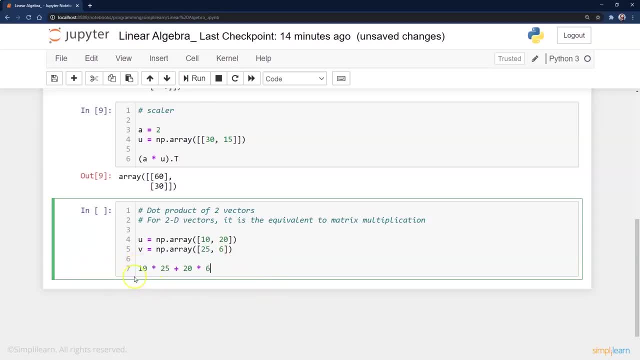 and if you remember correctly, an array like this would be 10 times 25 plus 20 times 6.. We'll go ahead and print that. There we go, And then we'll go ahead and do the npdot of u, comma v. 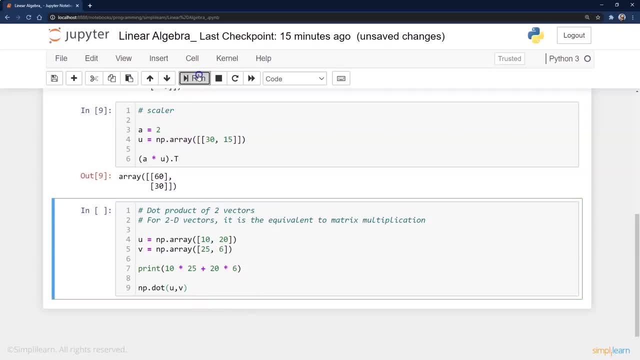 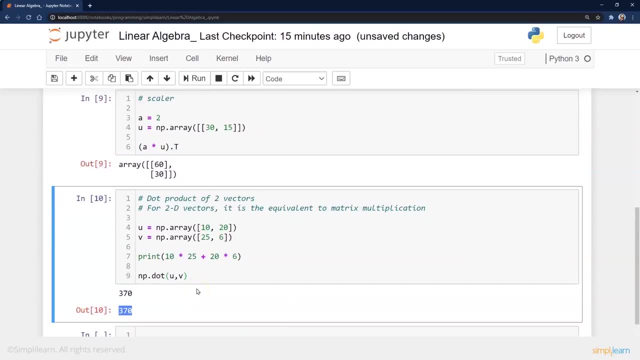 And we'll find when we do this, when we go ahead and run this, we're going to get 370, 370.. So this is a strain multiplication, where they use it to solve linear algebra when you have multiple numbers going across. 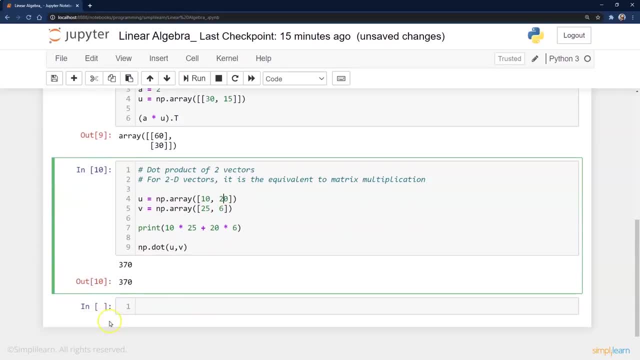 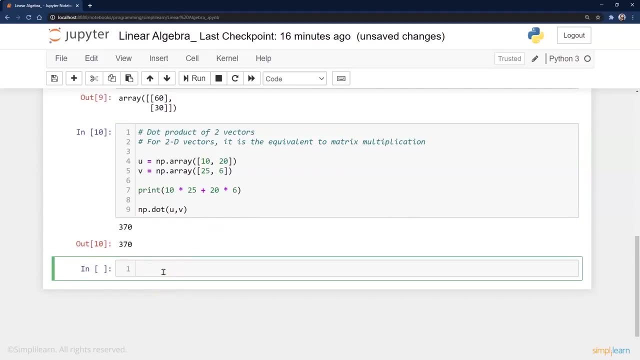 And so this could be very complicated. We could have a whole string of different variables going in here, But for this we get a nice value for our dot multiplication, And we did addition earlier, which is just your basic addition, And of course the matrix. 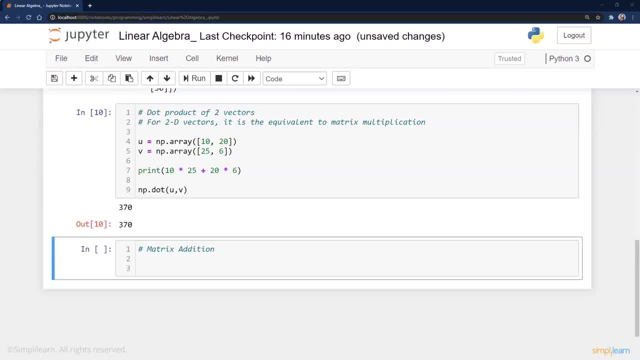 you can get very complicated on these, Or, in this case, we'll go ahead and do. let's create two complex matrices. This one is a matrix of 12, 10, 4, 6, 4, 31.. 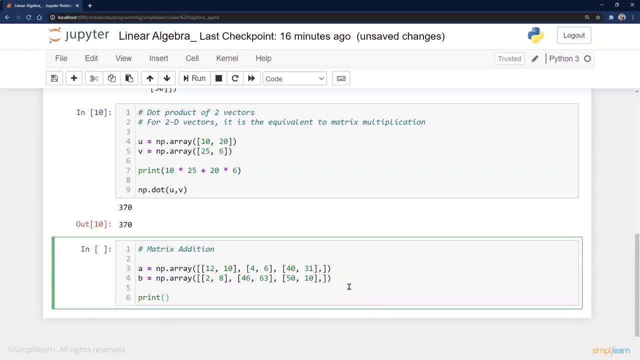 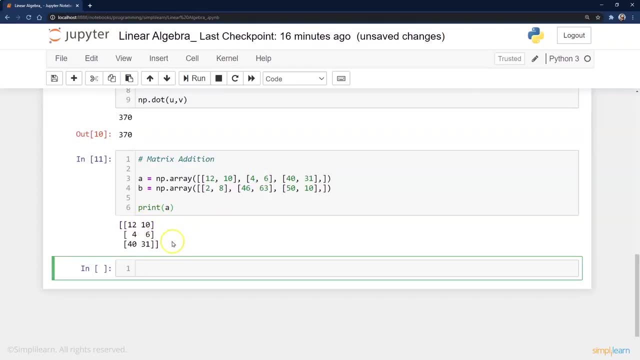 We'll just print out a so you can see what that looks like. Here's print a. When we print a out, you can see that we have. we can see that we have a two by three layer matrix for a And we can also put together. 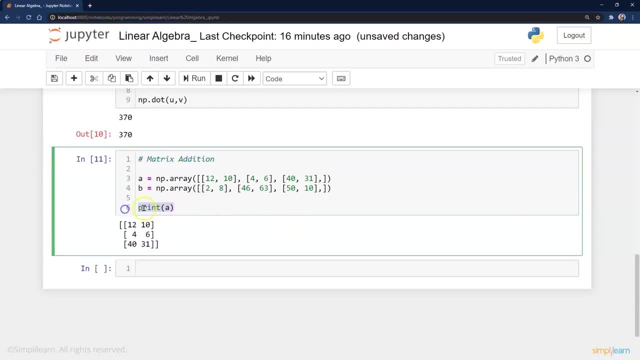 always kind of fun when you're playing with print values. we can do something like this: We could go in here, There we go, We could print a, We have it, end with equals a run, And this kind of gives it a nice look. 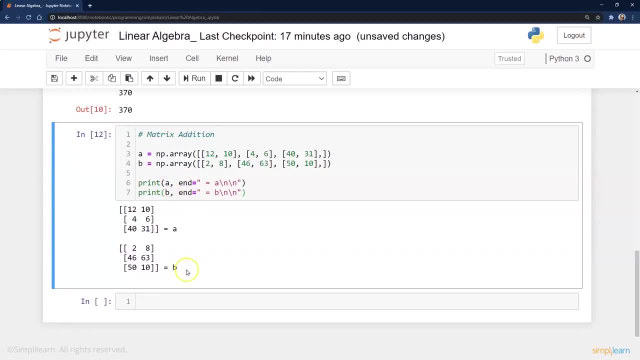 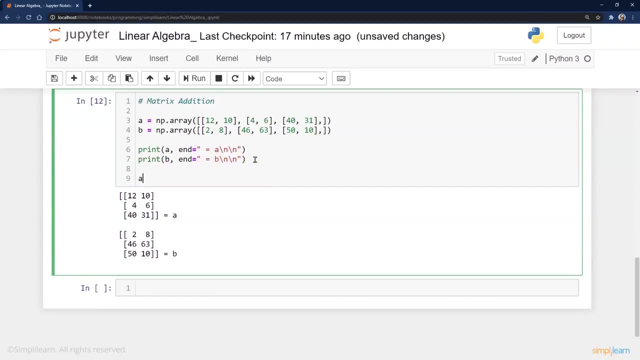 Here's your matrix. That's all this is. Comma n means it just tags it on the end. That's all that is doing on there, And then we can simply add in what is a plus b, And you should already guess, because this is the same as what we did before. 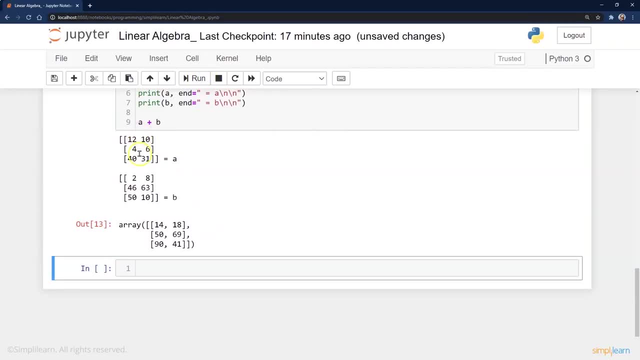 There's no difference When we do a simple vector addition. we have: 12 plus 2 is 14,, 10 plus 8 is 18, and so on. And just like we did the matrix addition, we can also do a minus b. 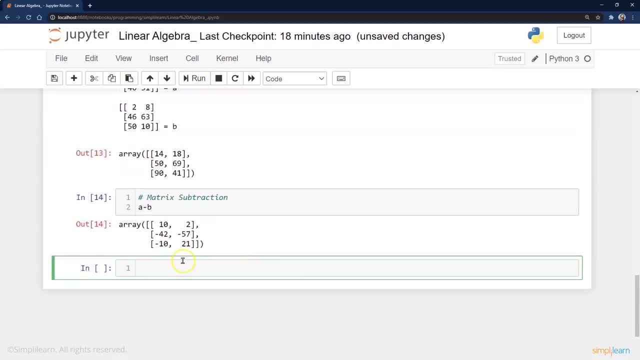 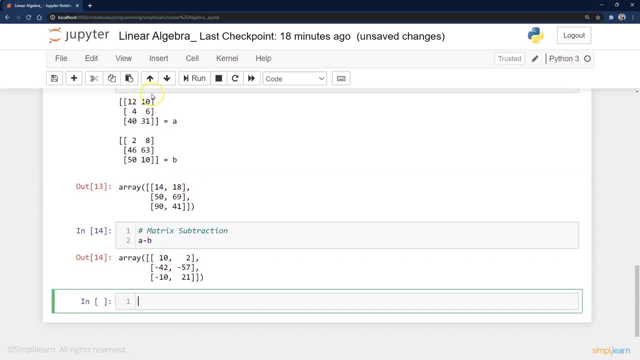 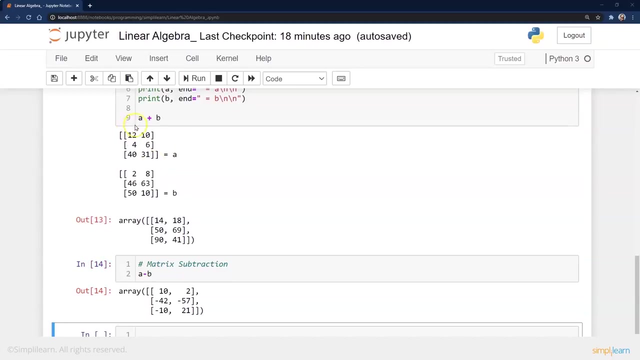 and do our matrix subtraction And we look at this. we have what? 12 minus 2 is 10, 10 minus 8, where are we? Oh, there we go. Eight minus ah, Confusing what I'm looking at. 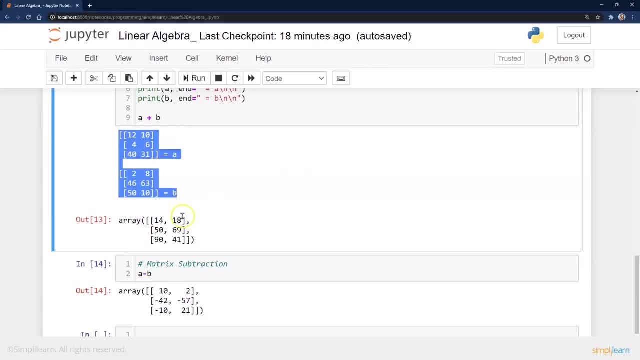 I should have reprinted out the original numbers, But we can see here: 12 minus 2 is of course 10,, 10 minus 8 is 2,, 4 minus 46 is minus 42, and so forth. So same as a subtraction as before. 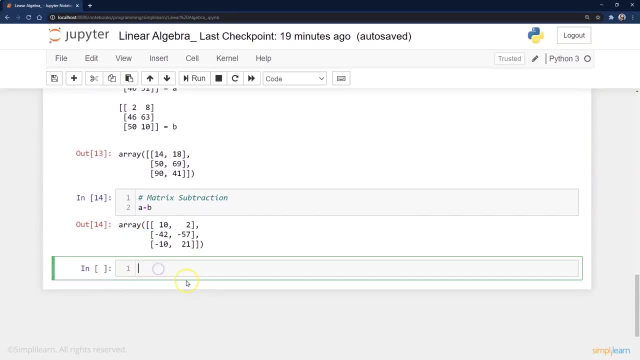 We just call it matrix subtraction. It's identical. Now, if you remember, up here we had a scalar addition. We're adding just one number to a matrix. You can also do scalar multiplication, And so simply if you have a single value, a. 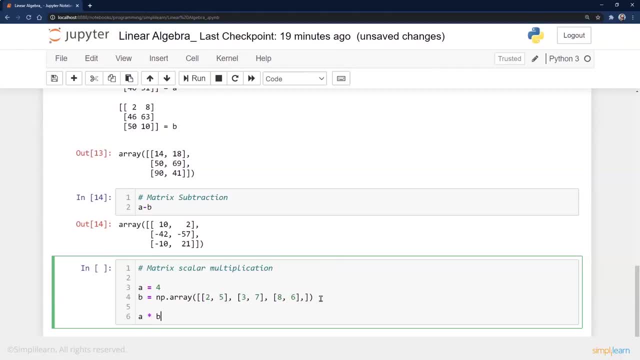 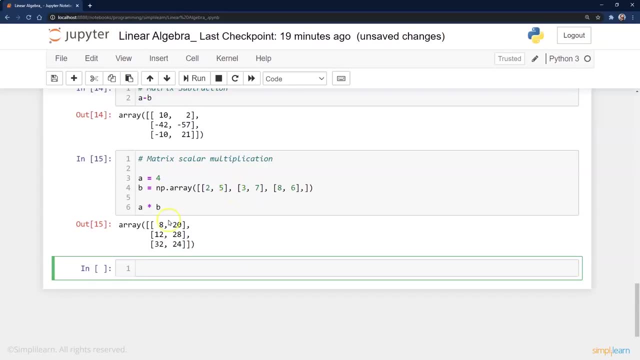 and you have b, which is your array. we can also do a times b When we run. that you can see here we have: 2 times 4 is 8,, 5 times 4 is 20, and so forth. You're just multiplying the 4. 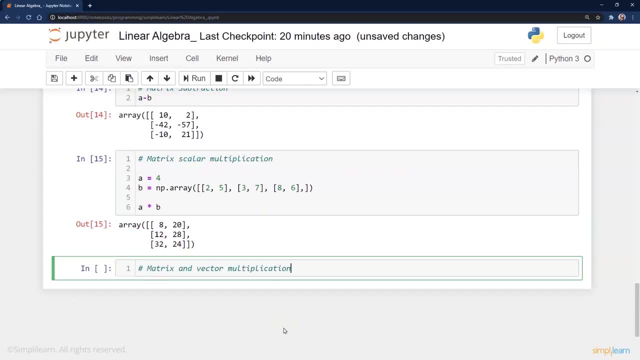 across each one of these values- And this is an interesting one- that comes up A little bit of a brain teaser, which is matrix and vector multiplication, And so when we're looking at this, we are just doing regular arrays. It doesn't necessarily have to be a numpy array. 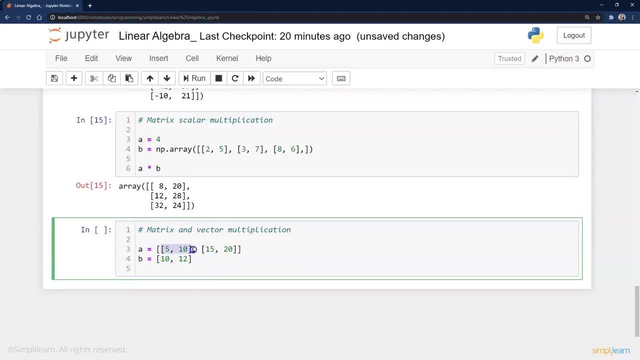 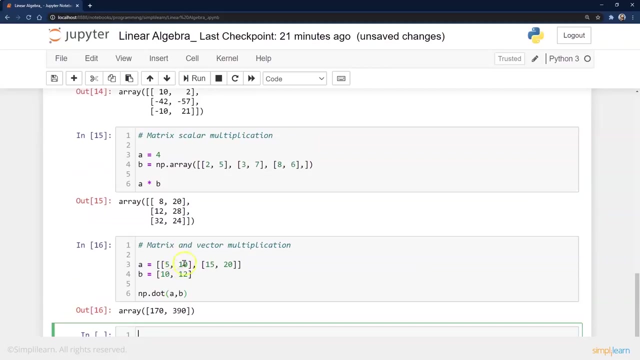 We have a, which has our array of arrays, and b, which is a single array, And so we can from here do the dot ab, And this is going to return two values. The first value is that you could say it's like we're doing this array. 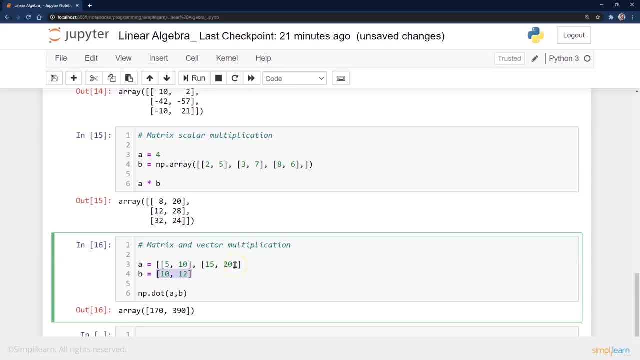 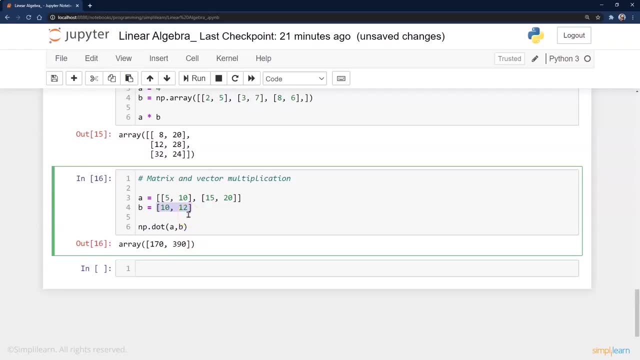 b array, first with a and then with a second one, And so it splits it up. So you have a matrix of vector multiplication and you can mix and match. When you get into really complicated backend stuff, this becomes more common because you're now 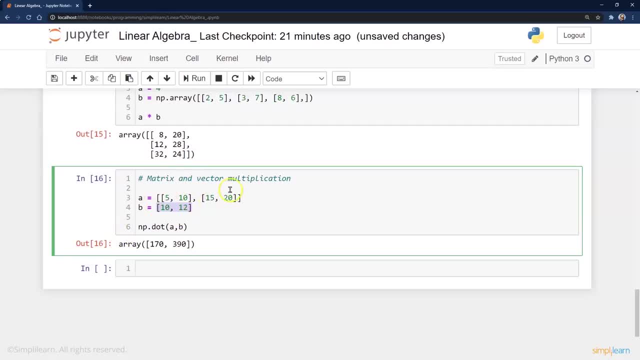 you've got layers upon layers of data, And so you'll end up with a matrix and a set of vector matrices that you want to multiply. Now keep in mind that if you're doing data science, a lot of times you're not looking at this. 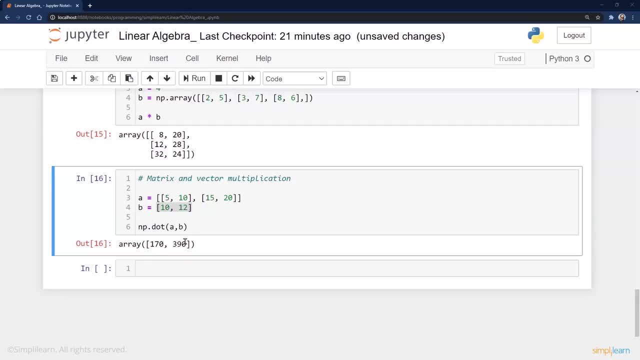 This is what's going on behind the scenes. So if you're in the scikit looking at sklearn where you're doing linear regression models, this is some of the math that's hidden behind the scenes that's going on. Other times you might find yourself having to do part of this. 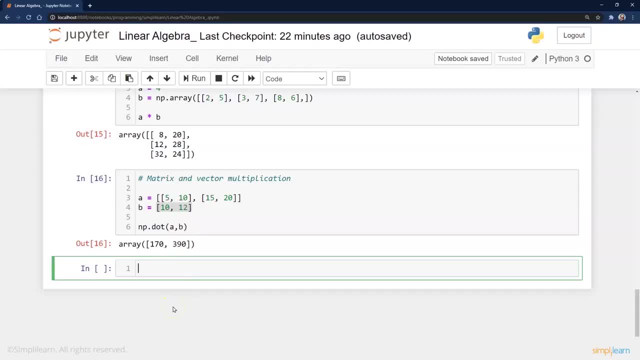 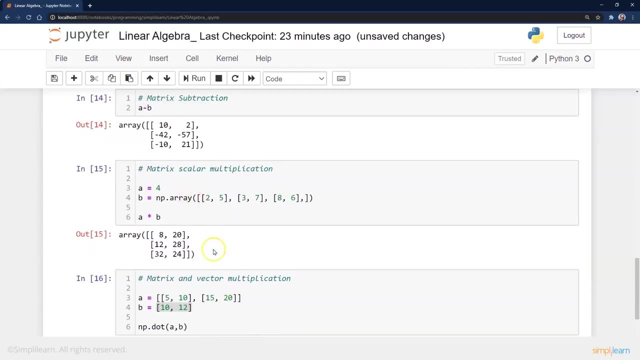 and manipulate the data around so it fits right. and then you go back in and you run it through the scikit And if we can do a pair of numbers, a pair where we did a matrix and vector multiplication, we can also do matrix to matrix multiplication. 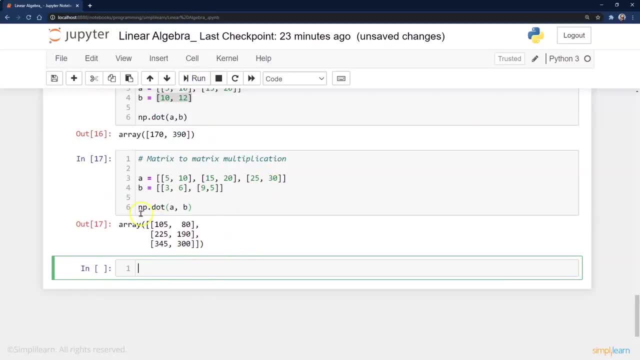 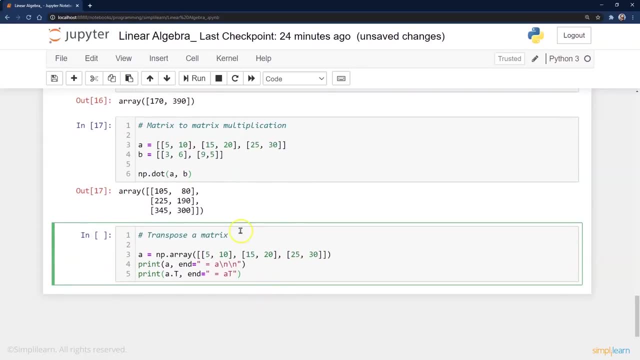 And if we run this, where we have the two matrices, you can see we have a very complicated array that of course comes out on there for our dot And, just to reiterate it, we have our transpose matrix, which is your dot T. And so if we create a matrix A and we do transpose it, 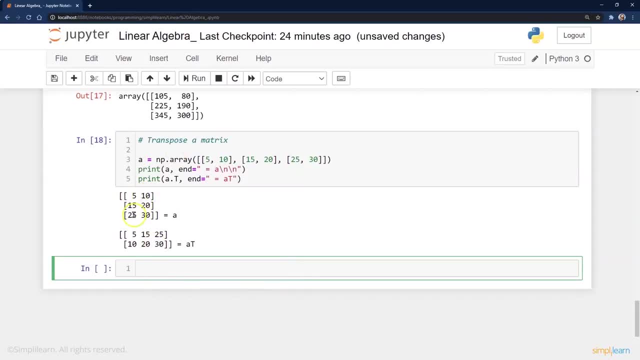 you can see how it flips it from 5, 10,, 15,, 20,, 25, 30 to 5, 15,, 20, 30.. 10, 20, 30. Rows and columns. 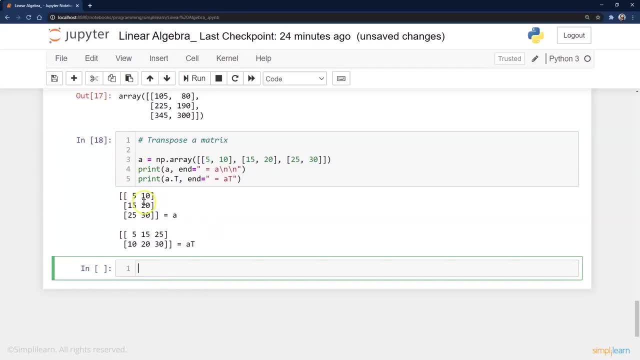 And certainly with the math this comes up a lot. It also comes up a lot with x- y plotting. When you put it into pi plot, you have one format where they're looking at pairs of numbers and then they want all of x's and all of y's. 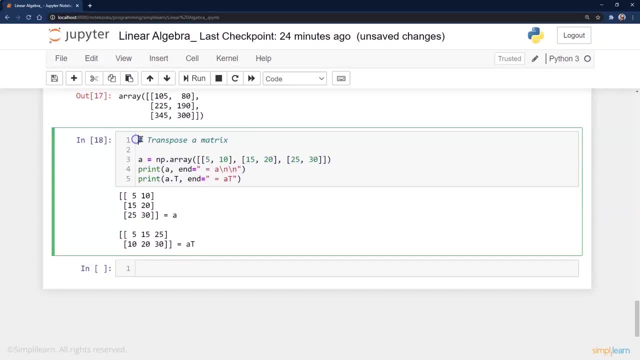 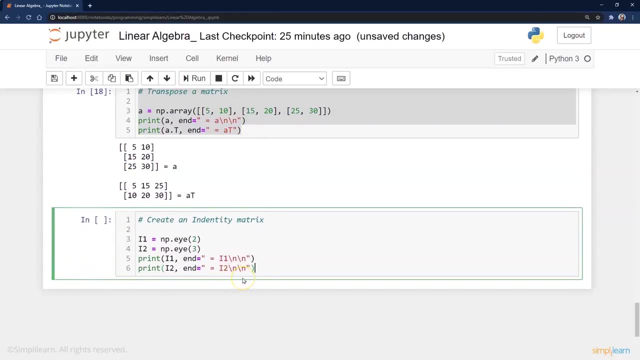 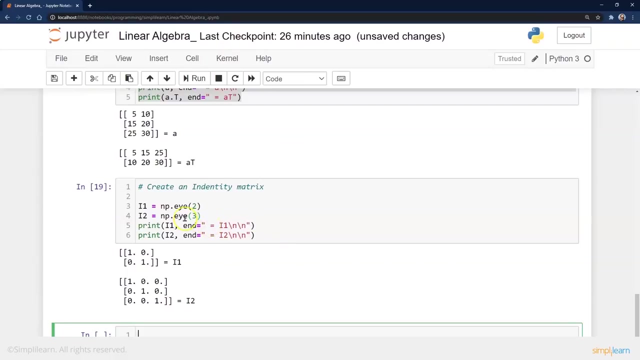 So you know, the transpose is an important tool, both for your math and for plotting and all kinds of things. Another tool that we didn't discuss is your identity matrix, And this one is more definition. The identity matrix we have here, one where we just did 2.. 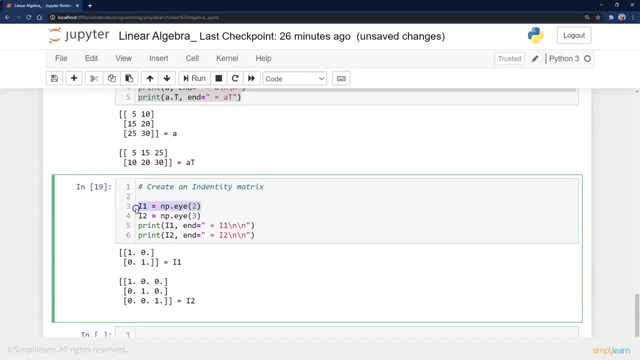 So it comes down as 1, 0, 0, 1.. 1, 0, 0, 0, 1, 0.. It creates a diagonal of 1.. And what that is is when you're doing your identities. 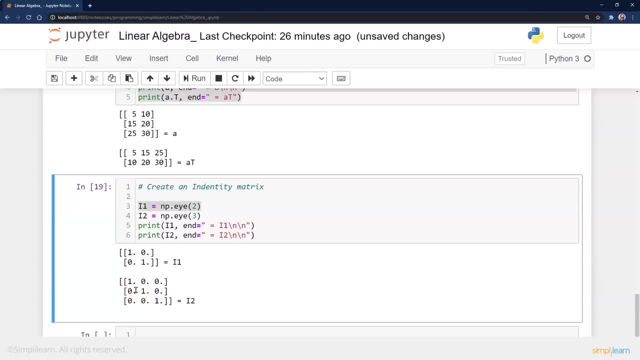 you could be comparing all your different features to the different features and how they correlate. And, of course, when you have your identity matrix, you're going to be comparing all your different features and how they correlate. And, of course, when you have feature 1. 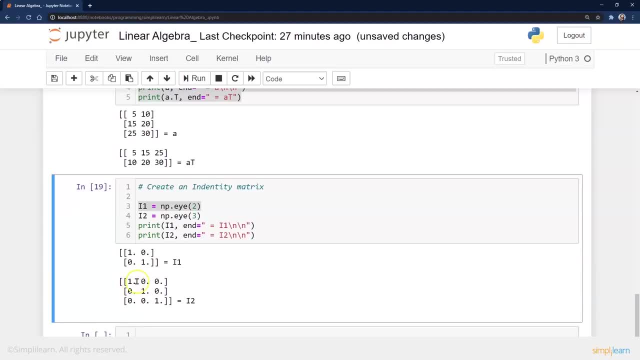 compared to feature 1 to itself, it is always 1, where usually it's between 0 and 1, depending on how well it correlates. So when we're talking about identity matrix, that's what we're talking about right here- is that you create this preset matrix. 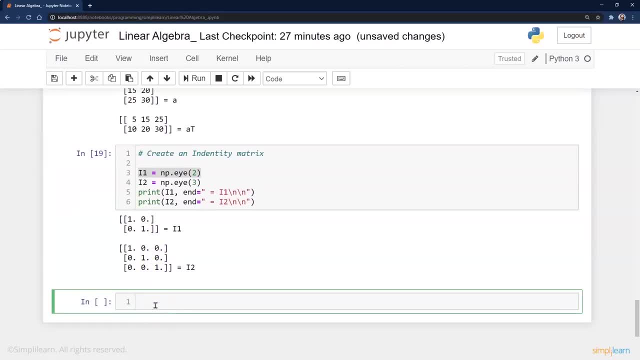 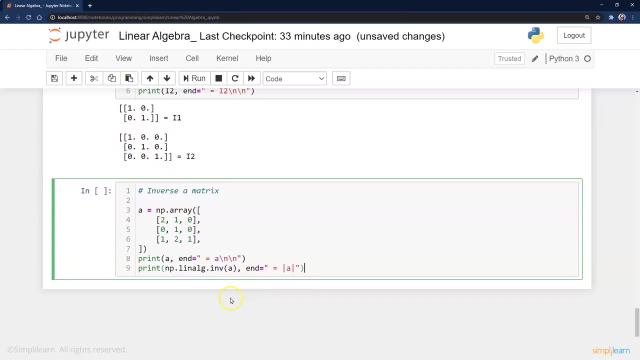 and then you might adjust these numbers depending on what you're working with and what the domain is. And then- another thing we can do to kind of wrap this up- we'll hit you with the most complicated piece of the puzzle. here is an inverse, A matrix. 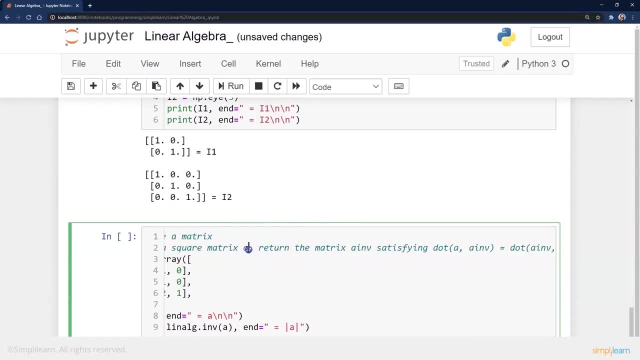 And let's just go ahead and put the- Oh it's a lengthy description. Let's go ahead and put the description. This is straight out of the website for NumPy. So, given a square matrix A, here's our square matrix A. 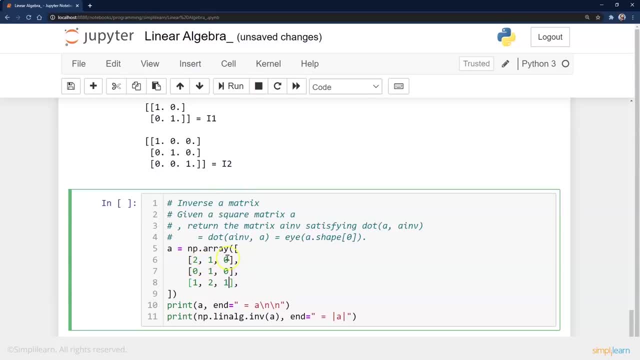 which is 2, 1, 0, 0, 1, 0, 1, 2, 1.. Keep in mind: 3 by 3 is square, It's got to be equal And return the matrix A inverse. 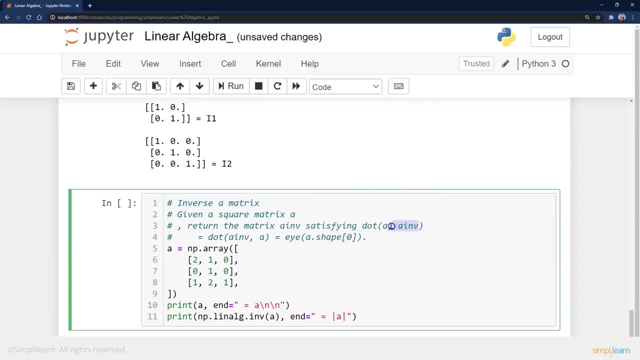 satisfying dot A inverse. So here's our matrix multiplication. And then of course it equals the dot A inverse of A with an identity shape of A dot shape 0. This is just reshaping the identity. That's a little complicated there, So we're going to have our 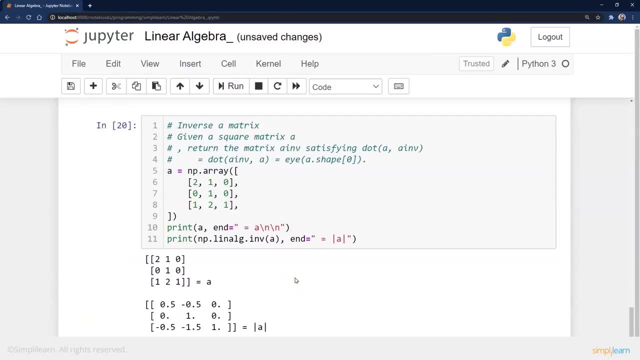 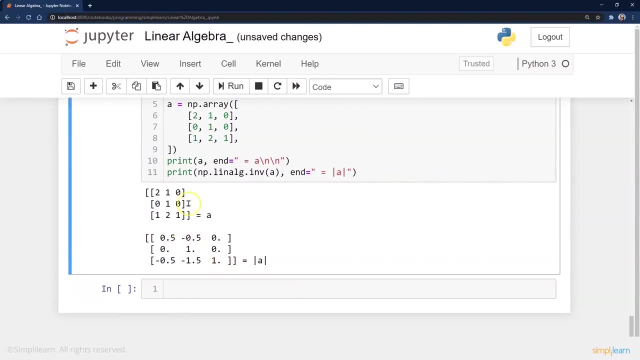 Here's our array. We'll go ahead and run this And you can see what we end up with is we end up with an array 0.5 minus 0.5 and so forth, with our 2,, 1, 1 going down. 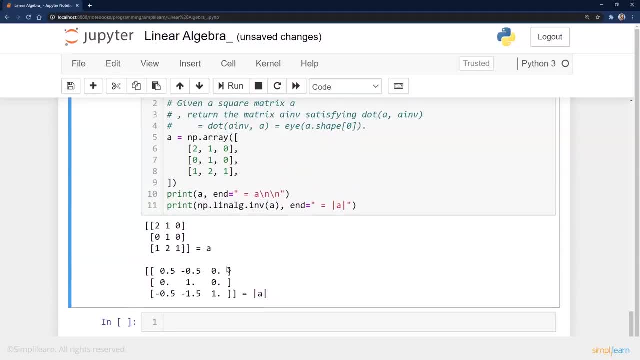 2, 1, 0, 0, 1, 0, 1, 2, 1.. Getting into a little deep on the math understanding when you need this is what's really important when you're doing data science. 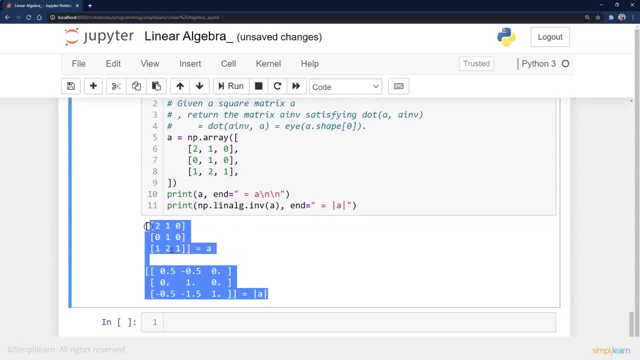 versus handwriting this out and looking up the math and handwriting all the pieces out. You do need to know about the linear algorithm and the inverse of A, So if it comes up you can easily pull it up or at least remember where to look it up. 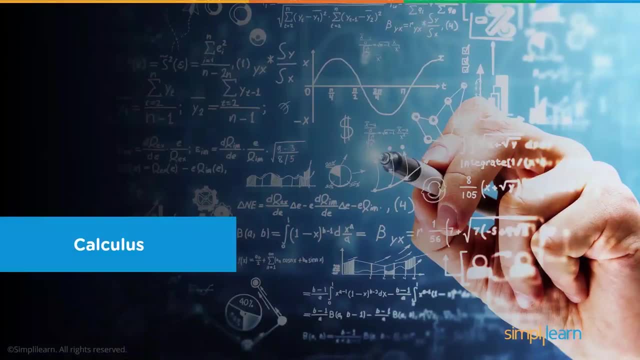 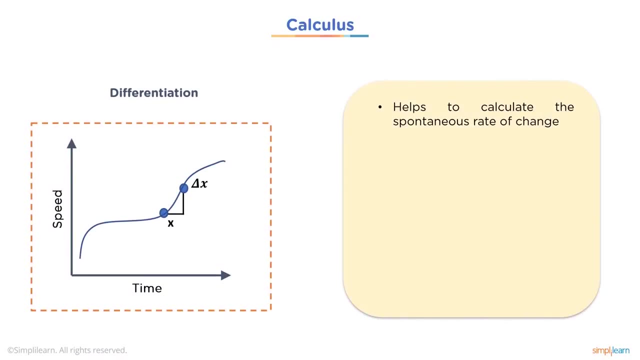 We took a look at the algebra side of it. Let's go ahead and take a look at the calculus side of what's going on here with the machine learning. So calculus, Oh my goodness. And differential equations. You got to throw that in there. 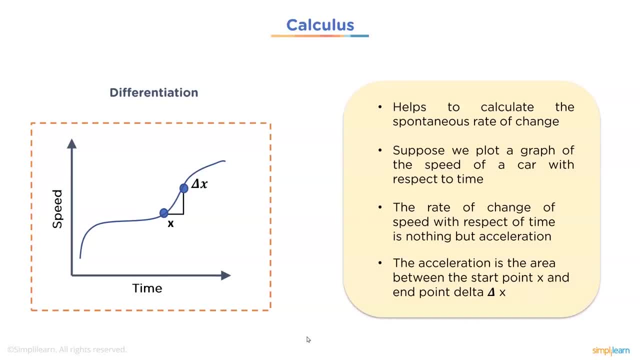 because that's all part of the bag of tricks, especially when you're doing large neural networks. but it also comes up in many other areas. The good news is most of it's already done for you at the end. So when it comes up, 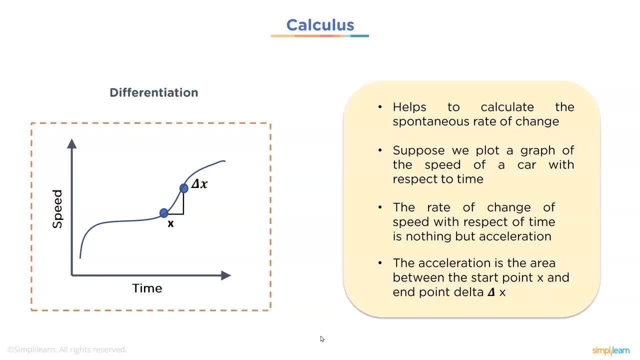 you really do need to understand from the data science, not data analytics. Data analytics means you're digging deep into actually solving these math equations, And a neural network is just a giant differential equation. So when we talk about calculus, we're going to go ahead and understand it. 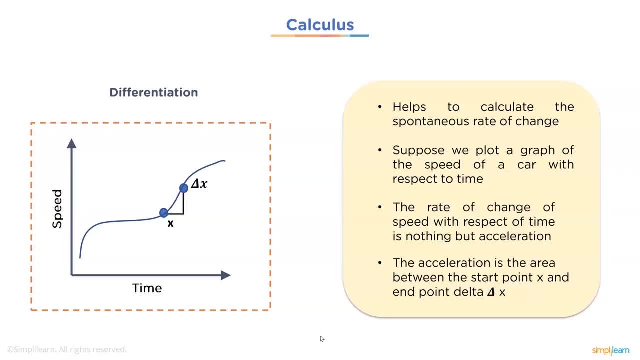 by talking about cars versus time and speed. So it helps to calculate the spontaneous rate of change. So suppose we plot a graph of the speed of a car with respect to time. So, as you can see here, going down the highway probably merged into the highway from an on-ramp. 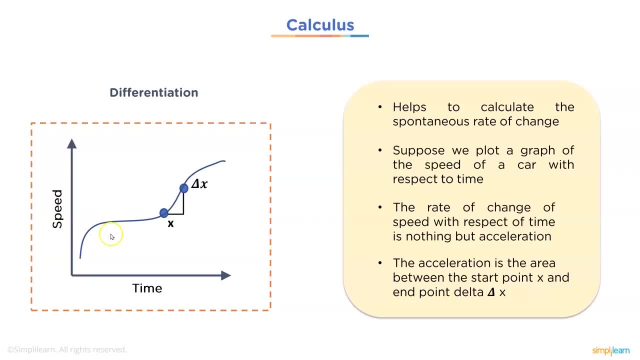 so I had to accelerate. so my speed went way up. Stuck in traffic, merged into the traffic, traffic opens up and I accelerate again up to the speed limit and maybe it peters off up there. So you can look at this as the speed versus time. 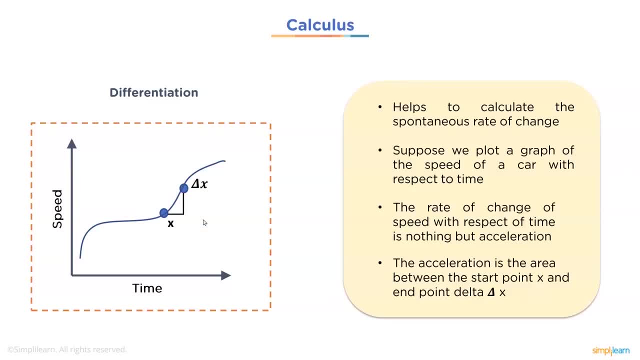 I'm getting faster and faster because I'm continually accelerating And if I hit the brakes it would go the other way. So the rate of change of speed with respect of time is nothing but acceleration. How fast are we accelerating? The acceleration is the area between the star point of x. 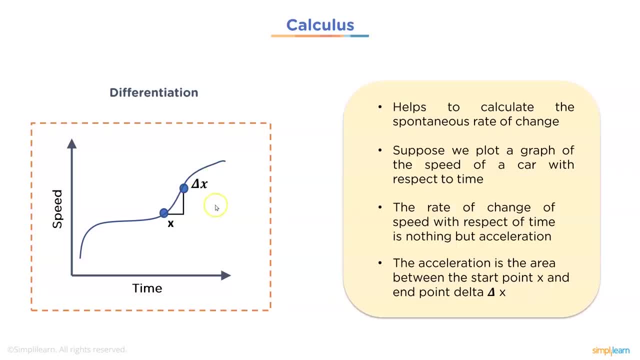 and the end point of delta x. So we can calculate a simple. if you had x and delta x, we could put a line there and that slope of the line is our acceleration. Now that's pretty easy when you're doing linear algebra. 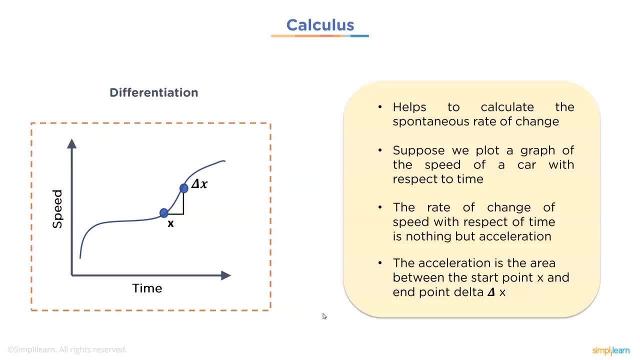 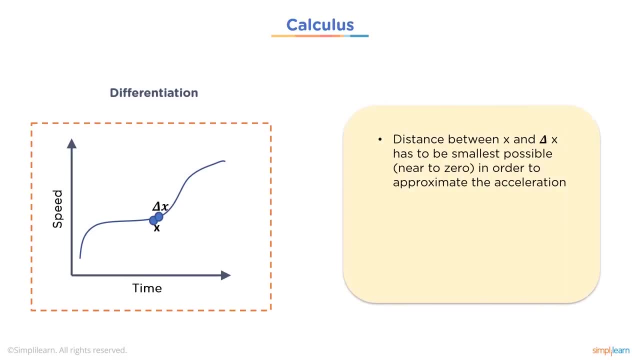 but I don't want to know it just for that line and those two points. I want to know it across the whole of what I'm working with. That's where we get into calculus. So when we talk about the distance between x and delta x, 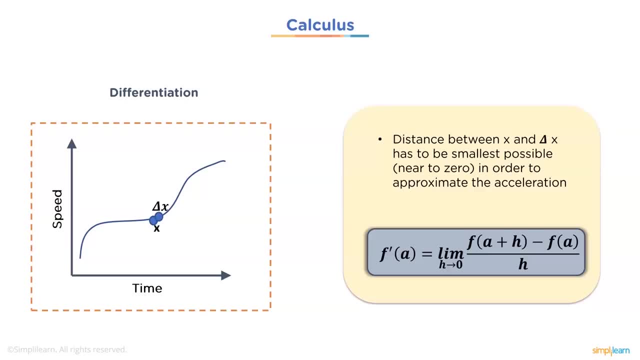 it has to be the smallest possible near to zero in order to approximate the acceleration. So the idea is that instead of- I mean, if you ever took a basic calculus class- they would draw bars down here and you would divide this area up. 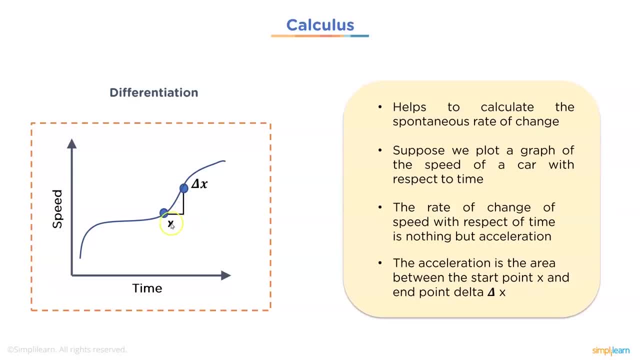 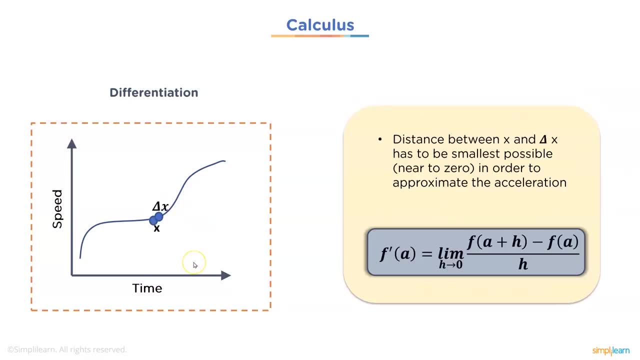 Let's go back up the screen. You divide this area of this time period up into maybe 10 sections and you'd use that and you could calculate the acceleration between each one of those 10 sections, kind of thing. And then we just keep making that space smaller and smaller. 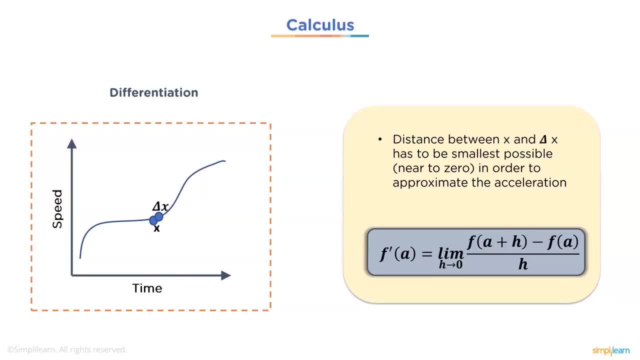 until delta x is almost infinitesimally small. And so we get a function of a equals a limit, as h goes to zero, of a function of a plus h minus, a function of a over h. And that is, you're computing the slope of the line. 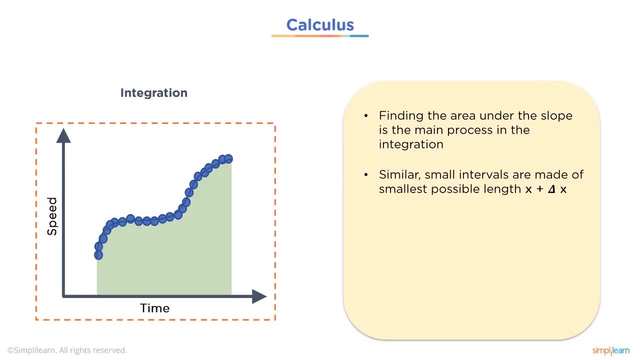 We're just computing that slope under smaller and smaller and smaller samples, And that's what calculus is. Calculus is the integral. You can see down here we have our nice integral sign. It looks like a giant S And that's what that means. 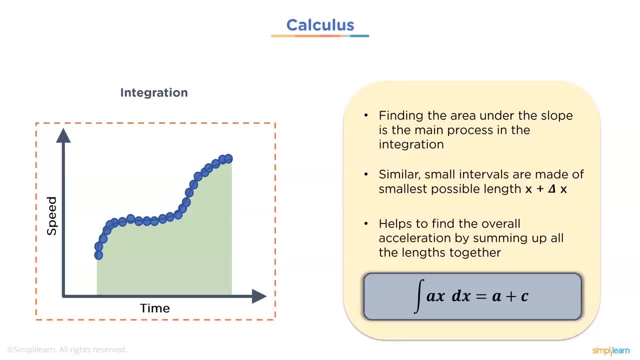 is that we've taken this down to as small as we can for that sampling. So we're talking about calculus, we're finding the area under the slope is the main process in the integration. Similar small intervals are made of the smallest possible length of x plus delta x. 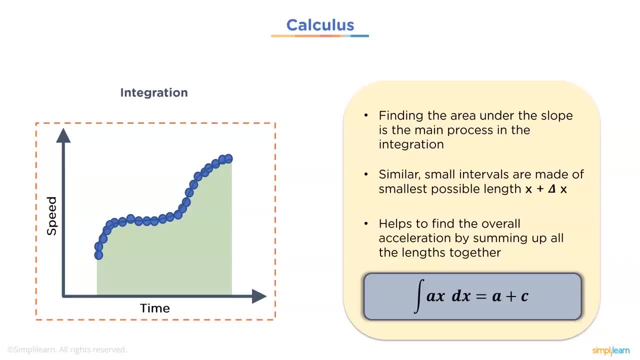 where delta x approaches almost an infinitesimally small space. And then it helps to find the overall acceleration by summing up all the lengths together. So we're summing up all the accelerations from the beginning to the end, And so here's our integral. 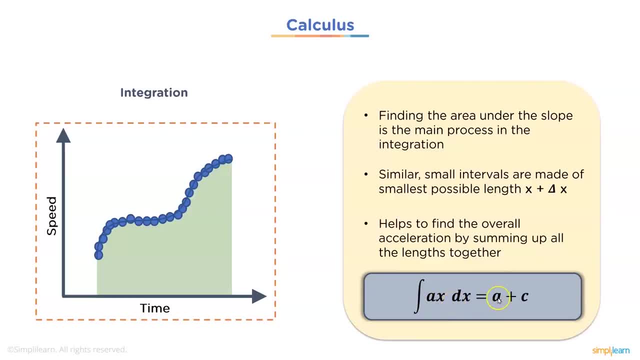 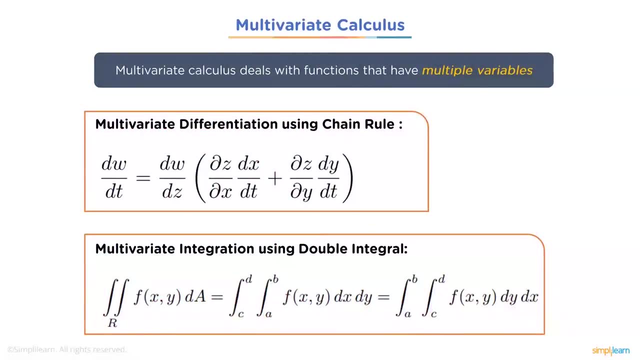 We sum of a of x times d of x equals a plus c, And that is our basic calculus here. So when we talk about multivariate calculus, multivariate calculus deals with functions that have multiple variables, And you can see, here we start getting into. 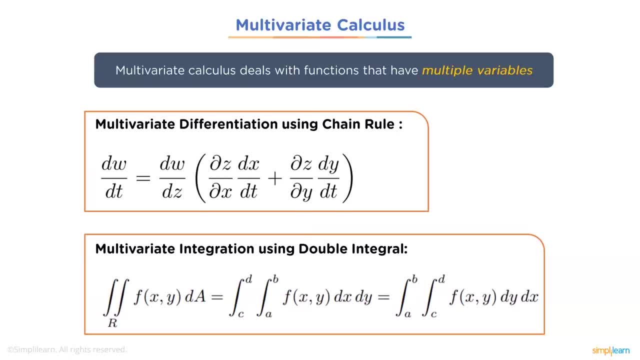 some very complicated equations: Change in w over change of time equals change of w over change of z, The differential of z to dx, differential of x to dt. It gets pretty complicated And it really translates into the multivariate integration using double integrals. 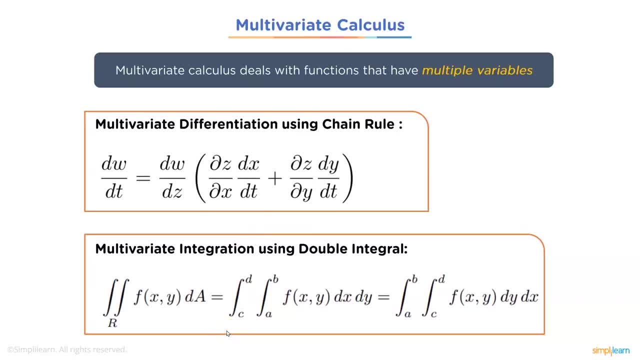 And so you have: the sum of the sum of f, of x, of y, of d, of a equals the sum from c to d, and a to b, of f, of x, of y, dx, dy equals the sum of a to b, sum of c to d, of f, x, of y, dy, dx. 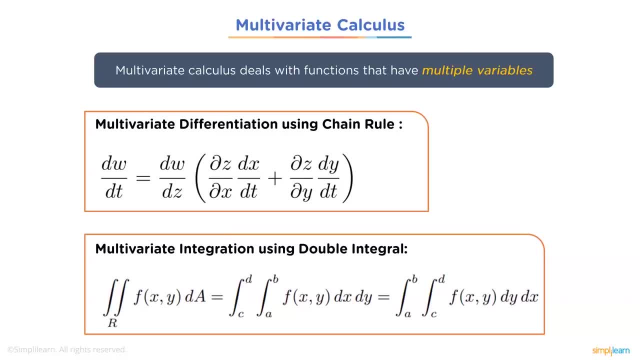 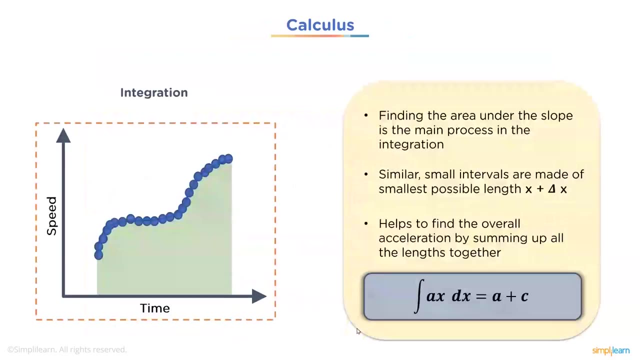 Understanding the very specifics of everything going on in here and actually doing the math is use the calculus one, calculus two and differential equations. So you're talking about three full length courses to dig into and solve these math equations. What we want to take from here: 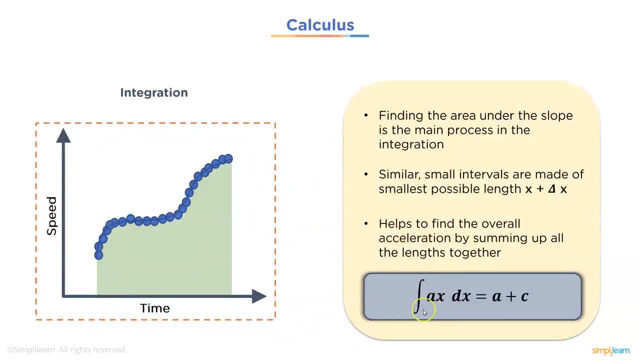 is when we're talking about calculus, we're talking about summing of all these different slopes, And so we're still solving a linear expression, We're still solving y equals mx plus b, But we're doing this for infinitesimally small x's. 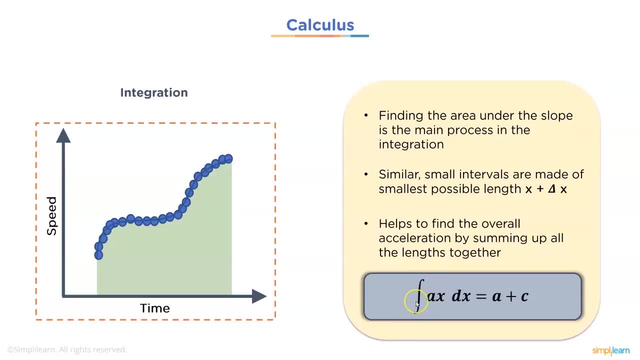 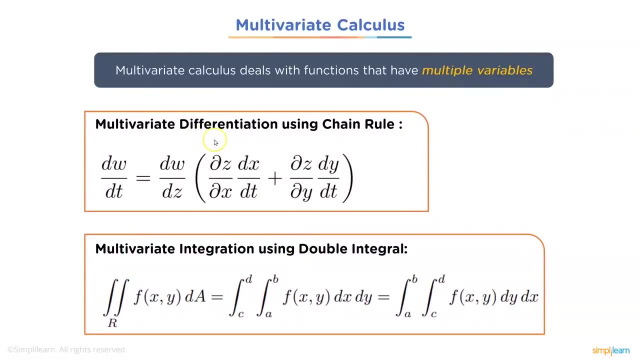 and we want to sum them up. That's what this integral sign means: The sum of a, of x, d of x equals a plus c. And when you see these very complicated multivariate differentiation using the chain rule, when we come in here and we have the change, 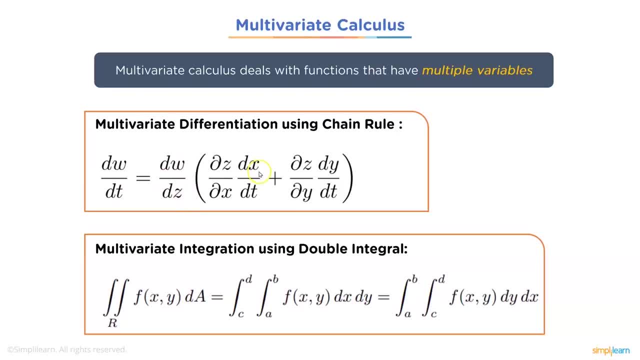 of w to the change of t equals the change of w, dz and so forth. That's what's going on here. That's what these means. We're basically looking for the area under the curve, which really comes to. how is the change changing? 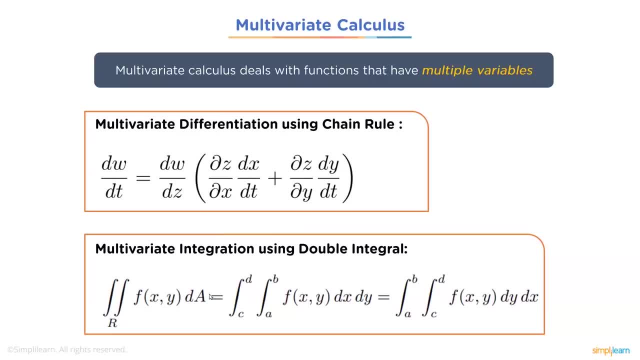 Speed's going up. How is that changing? And then you end up with a multiple layer. So if I have three layers of neural networks, how is the third layer changing, based on the second layer changing, which is based on the first layer changing? 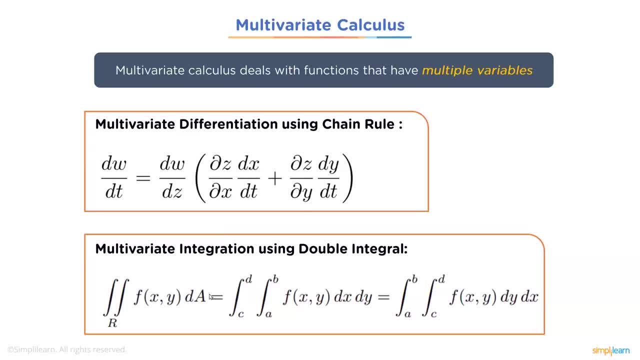 And you get the picture here that now we have a very complicated multivariate integration with integrals. The good news is we can solve this mathematically, and that's what we do when you do neural networks and reverse propagation. So the nice thing is that you don't have to. 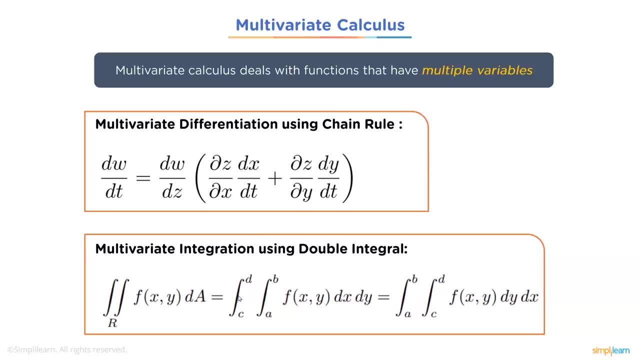 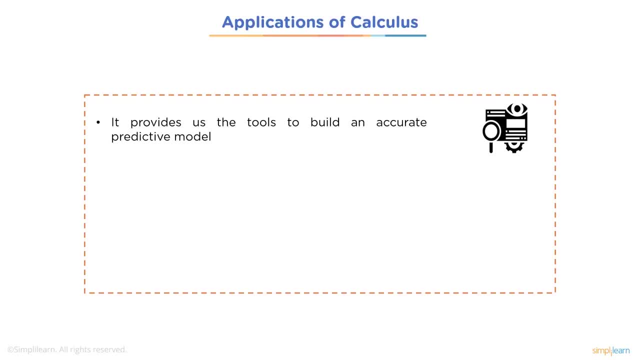 solve this on paper, unless you're data analysis and you're working on the back end of integrating these formulas and building the script to actually build them. So we talk about applications of calculus. It provides us the tools to build an accurate predictive model, So it's really behind the scenes. 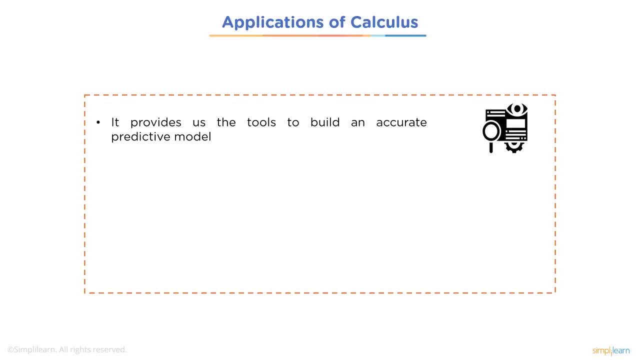 We want to guess at what the change of the change of the change is. That's a little goofy, I know, I just threw that out there. It's kind of a meta term, But if you can guess how things are going to change. 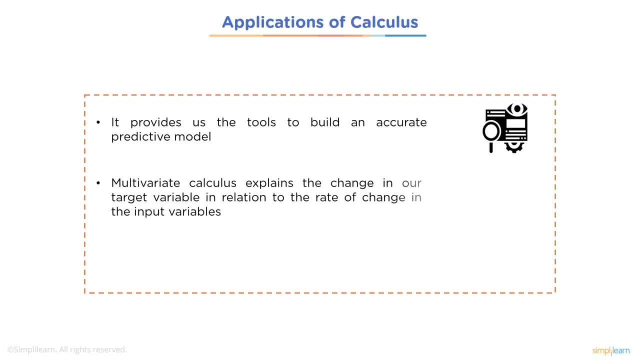 then you can guess what the new numbers are. Multivariate calculus explains the change in our target variable in relation to the rate of change in the input variables. So there's our multiple variables going in there. If one variable is changing, how does it affect? 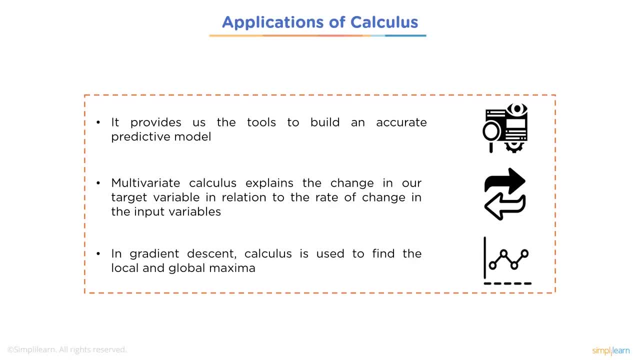 the other variable, And then in gradient descent, calculus is used to find the local and global maxima. And this is really big. We're actually going to have a whole section here on gradient descent, because it is really. I mean, I talked about neural networks and how. 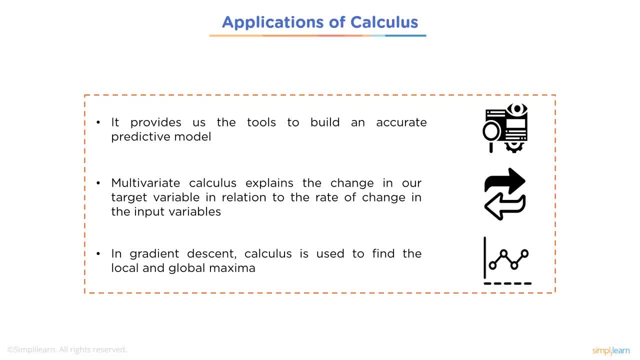 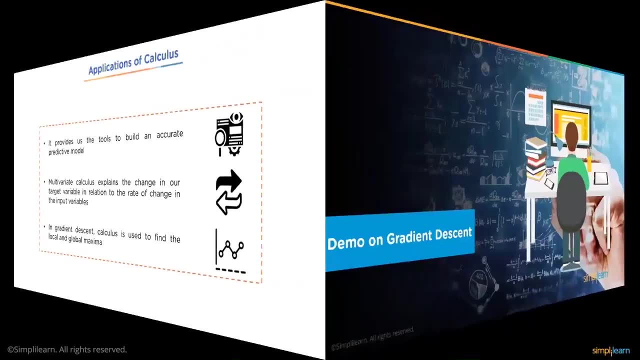 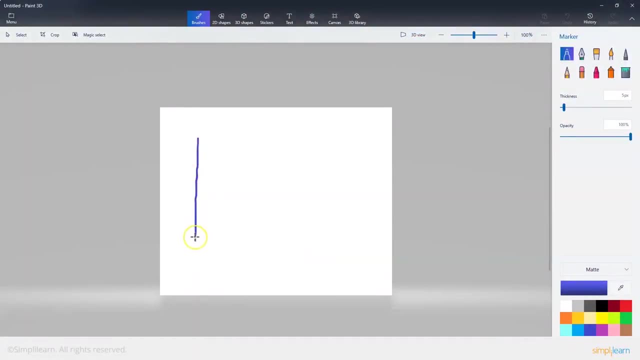 you can see how the different layers go in there, But gradient descent is one of the most key things for trying to guess the best answer to something. So let's take a look at the code behind gradient descent And, before we open up the code, let's just do real quick. 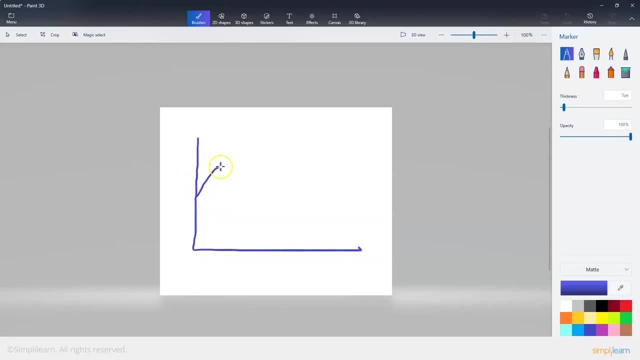 Gradient descent. Let's say we have a curve like this And most common Is that this is going to represent your error. Oops, Error, There we go, Error. Ah, hard to read there And I want to make the error as low as possible. 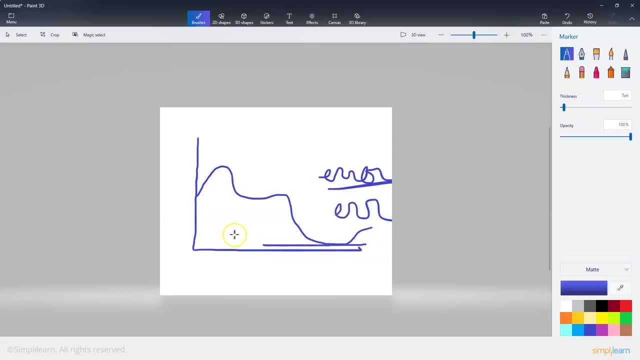 And so what I'm looking at it is: I want to find this line here which is the minimum value. So we're looking for the minimum, And it does that by sampling there And then, based on this, it guesses it might be someplace here. 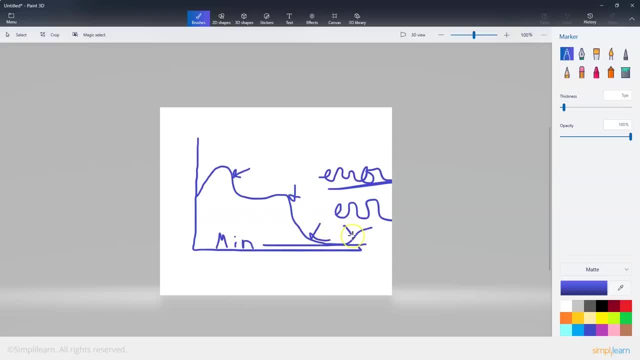 And it goes- hey, this is still going down. It goes here And then goes back over here And then goes a little bit closer And it's just playing a high-low until it gets to that spot, that bottom spot, And so we want to minimize the error. 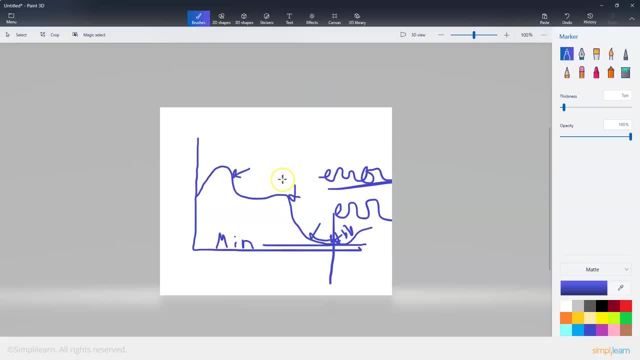 And on the flip note, you could also want to be maximizing something. You want to get the best output of it. That's simply minus the value. So if you're looking for where the peak is, this is the same as a negative for where the valley is. 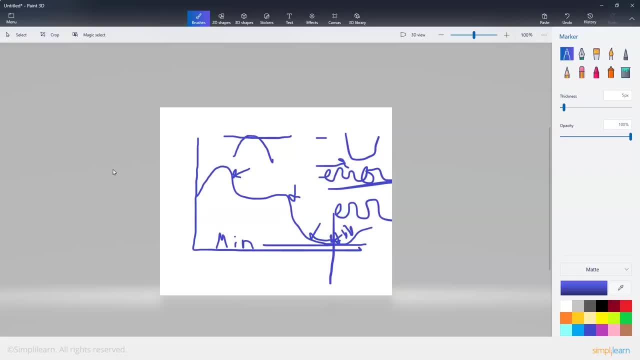 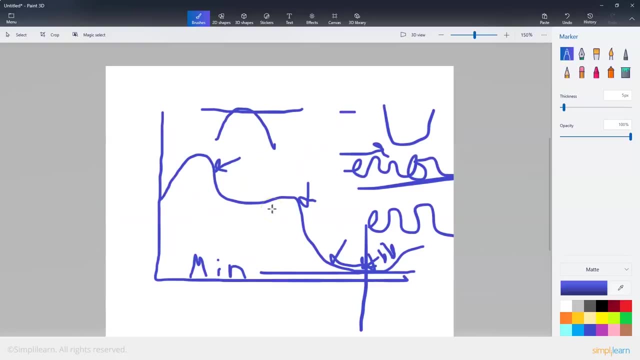 I'm looking for that valley. That's all that is, And this is a way of finding it. So the cool thing is: all the heavy lifting is done. I actually ended up putting together one of these a while back, when I didn't know about Sidekick. 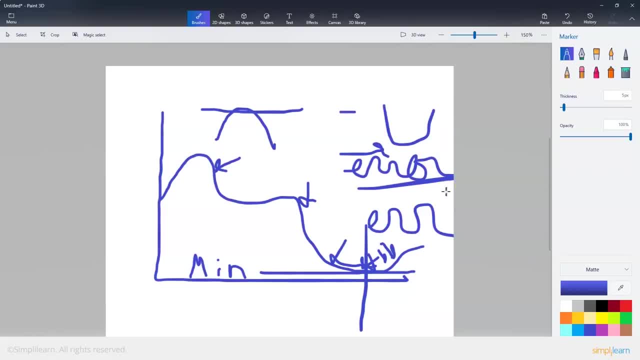 And I was just starting. Boy, it's a long while back And it's playing high-low. How do you play high-low, not get stuck in the valleys? figure out these curves and things like that. Well, you do that. 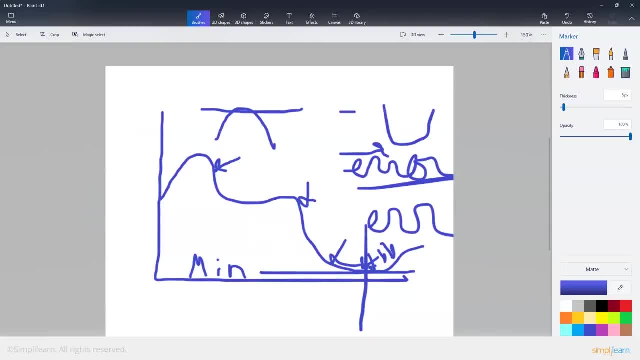 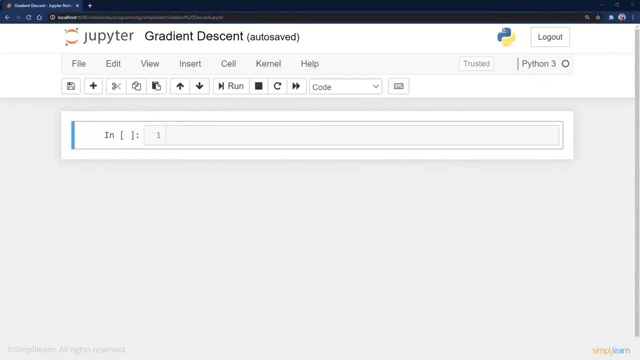 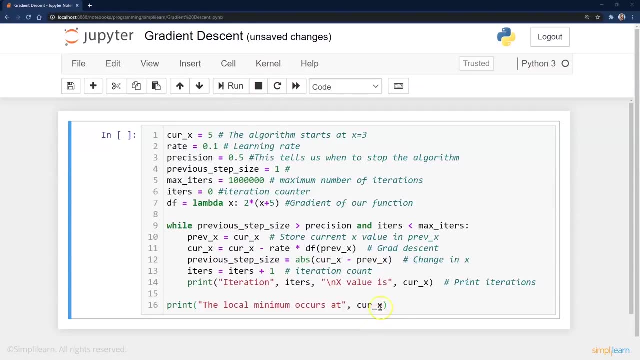 And the back end is all the calculus and differential equations to calculate this out. The good news is you don't have to do those, So instead we're going to put together the code And let's go ahead and see what we can do with that. 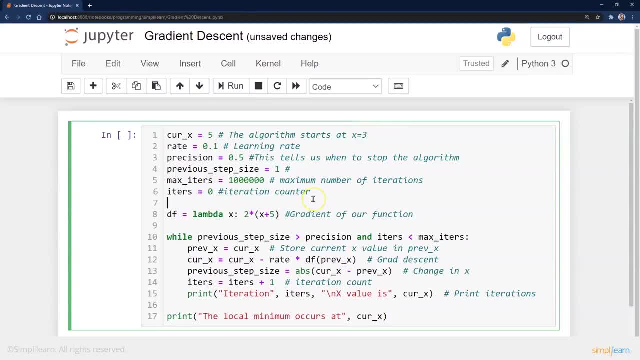 So guys in the back put together a nice little piece of code here, which is kind of fun. Some things we're going to note. This is really important stuff because when you start doing your data science and digging into your machine learning models, 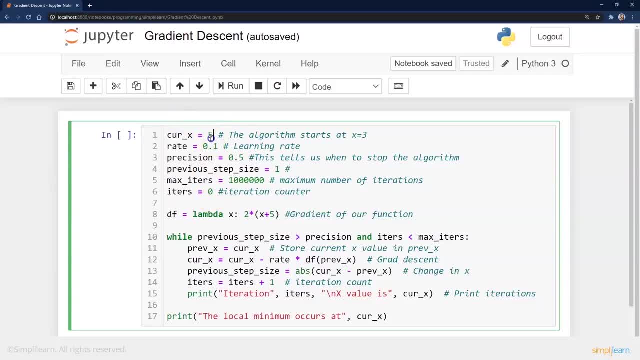 you're going to find these things are stumbling blocks. The first one is current x. Where do we start at? Keep in mind, your model that you're working with is very generic, So whatever you use to minimize it. the first question is: 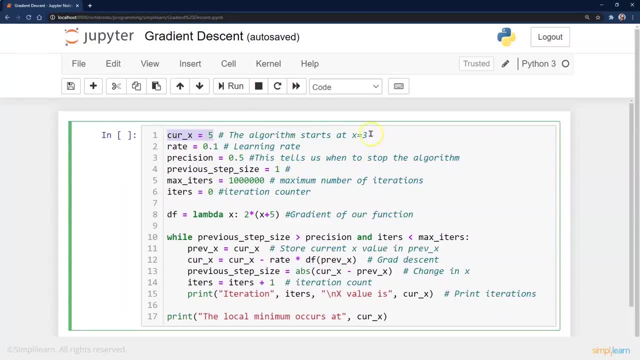 where do we start? And we started at this because the algorithm starts at x equals 3.. So we arbitrarily picked 5.. Learning rate is how many bars to skip going one way or the other. In fact, I'm going to separate that a little bit. 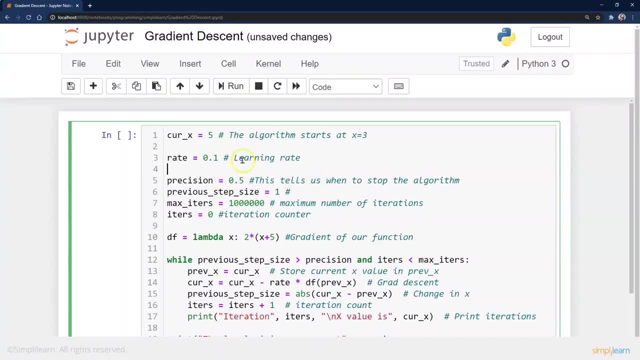 because these two are really important If we're dealing with something like this, where we're talking about: well, here's the function. we're going to use our gradient of our function: 2 times x plus 5.. Keep it simple. 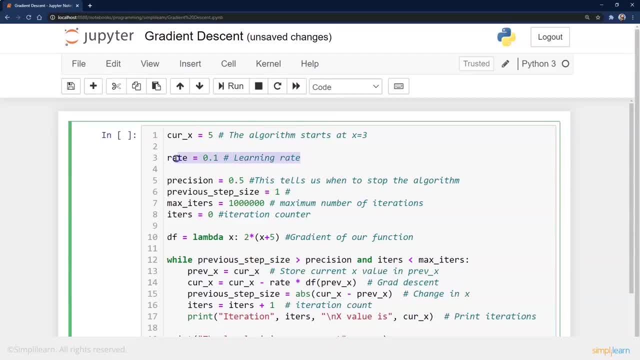 So that's the function we're going to work with. So if I'm dealing with increments of 1,000,, 0.1 is going to be a very long time, And if I'm dealing with increments of 1,000,. 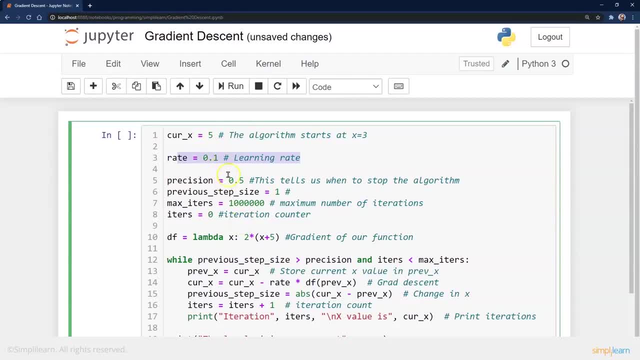 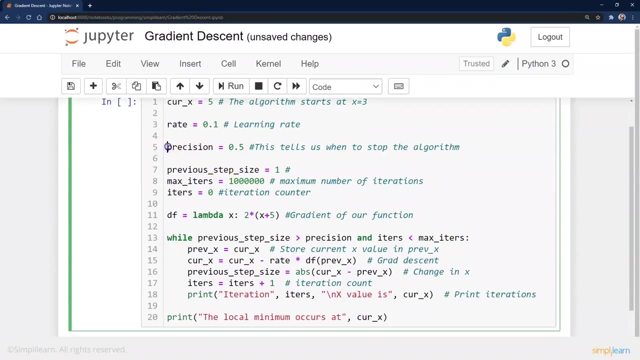 0.1 is going to skip over my answer, So I won't get a very good answer. And then we look at precision. This tells us when to stop the algorithm. So again, very specific to what you're working on. If you're working with money and you don't convert it into a float value, 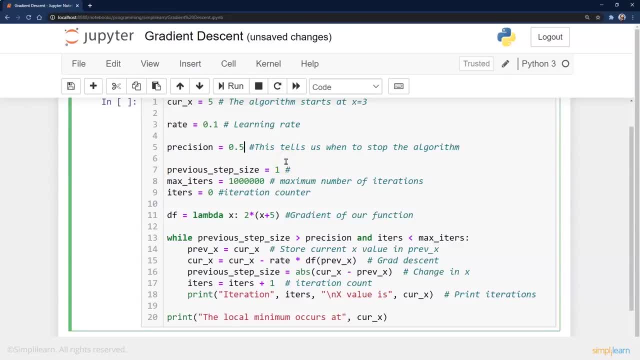 you might be dealing with 0.01, which is a penny. That might be your precision you're working with. And then, of course, the previous step: size max iterations. We want something to cut out at a certain point. Usually that's built into a lot of minimization functions. 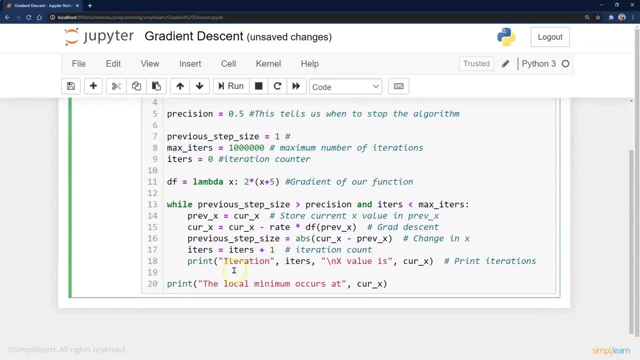 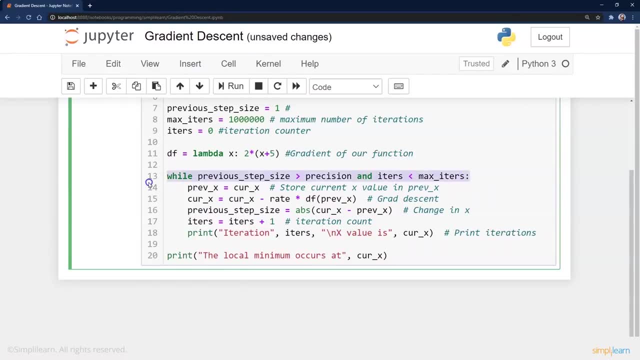 And then here's our actual formula we're going to be working with. And then we come in and we go. while previous step size is greater than precision and itters is less than max, itters say that 10 times fast. We're just saying: 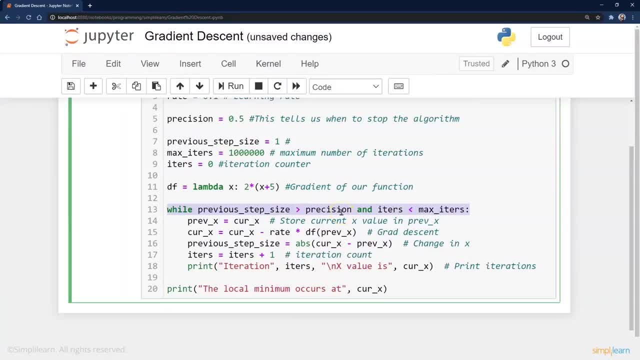 if we're still greater than our precision level, we still got to keep digging deeper, And then we also don't want to go past 1,000 or whatever. this is a million or 10,000 running. That's actually pretty high. 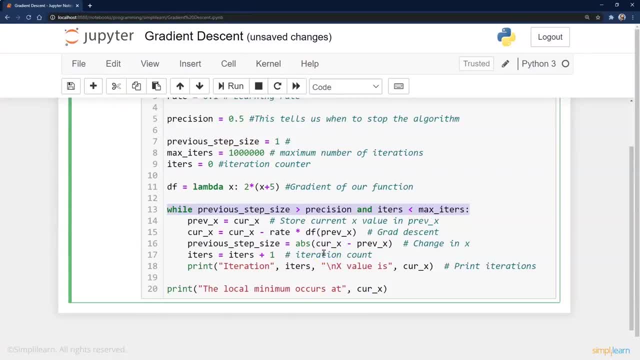 We almost never do max iterations more than like 100 or 200.. Rare occasions you might go up to 400 or 500, depending on the problem you're working with. So we have our previous equals, our current. That way we can track time-wise. 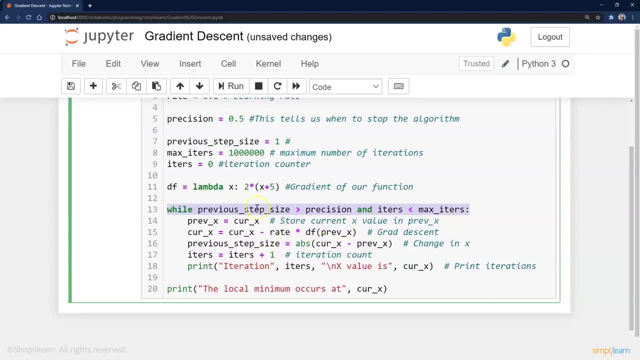 The current now equals the current rate times the formula of our previous x. So now we've generated our new version. Previous step size equals the absolute current previous. So we're looking for the change in x. Itters equals iterations plus 1.. 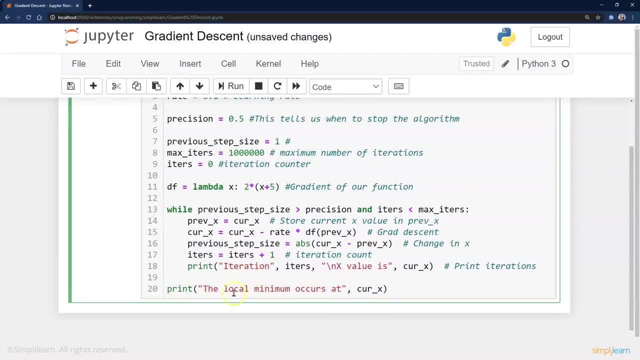 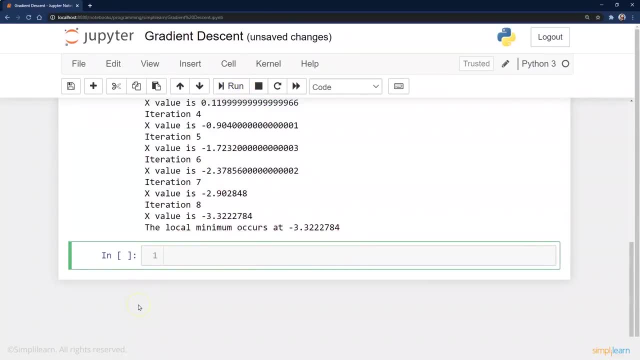 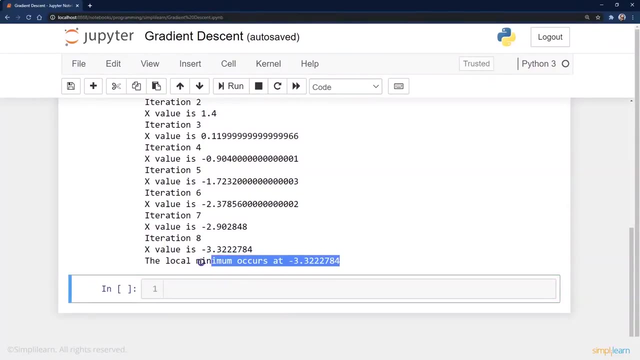 That's so we know to stop if we get too far. And then we're just going to print: the local minimum occurs at x on here, And if we go ahead and run this, you can see right here it gets down to this point and it says: hey, local minimum is minus 3.3222. 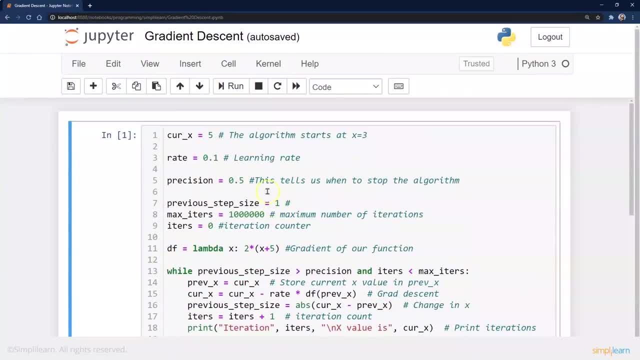 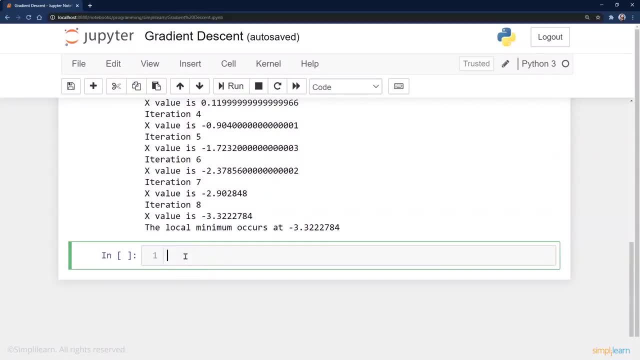 for this particular series we created. This is created off of our formula here: lambda x 2 times x plus 5.. Now when I'm running this stuff, you'll see this come up a lot with the sklearn kit And one of the nice reasons of breaking this down the way we did. 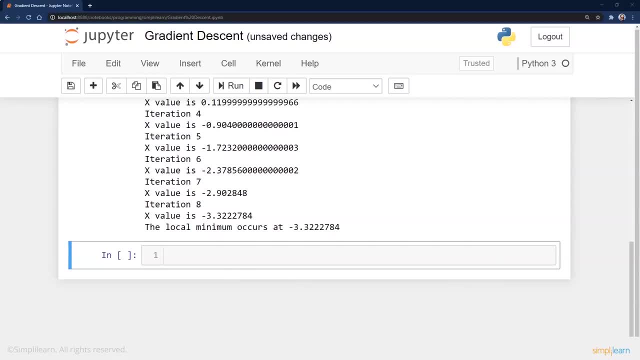 is. I could go over those top pieces. Those top pieces are everything. You start looking at these minimization toolkits in built-in code And so from we'll just do. it's actually docsscipyorg And we're looking at the scikit. 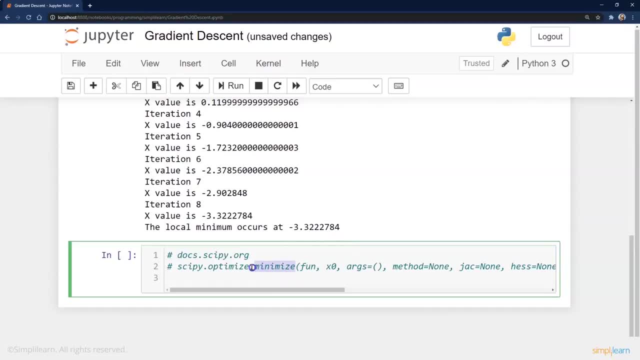 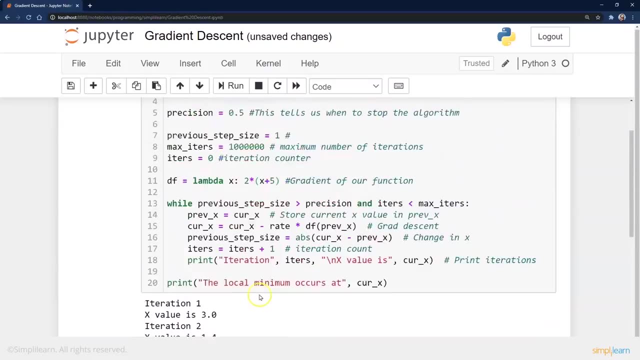 There we go: Optimize, minimize. You can only minimize one value. You have the function that's going in. The function can be very complicated, So we used a very simple function up here. It could be. there's all kinds of things that could be on there. 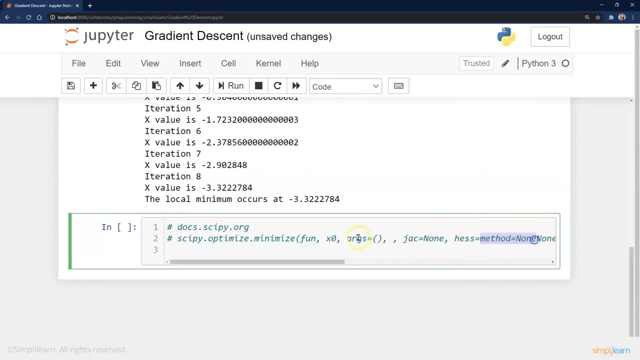 And there's a number of methods to solve this as far as how they shrink down And your x naught. there's your start value, So your function, your start value. there's all kinds of things that come in here that you can look at. 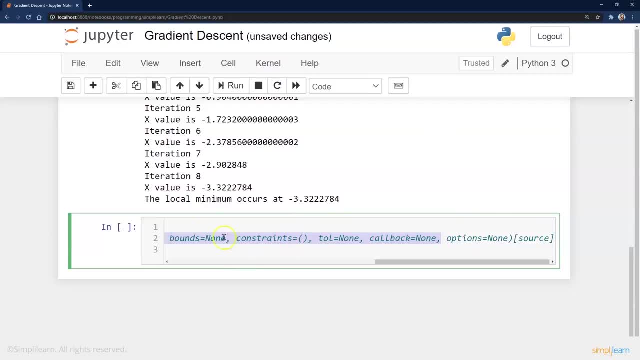 which we're not going to. Optimization automatically creates constraints, bounds. Some of this it does automatically, But really the big thing I want to point out here is you need to have a starting point. You want to start with something that you already know. 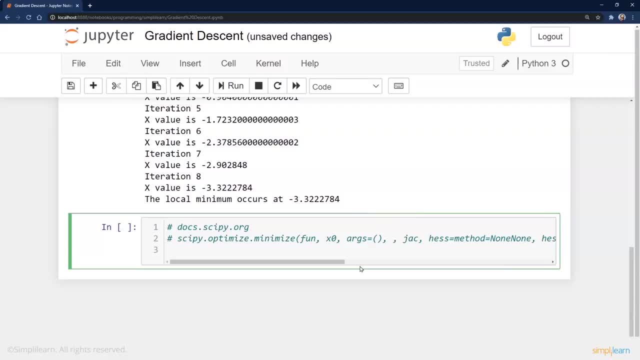 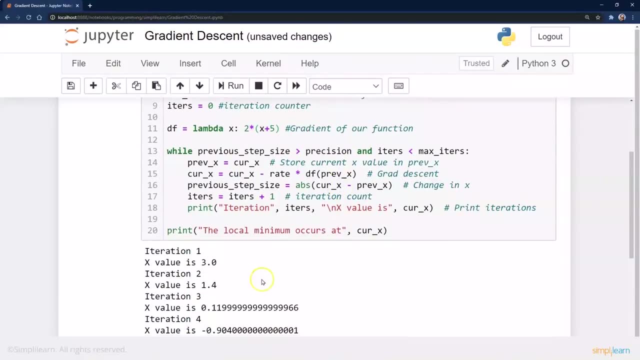 is mostly the answer. If you don't, then it's going to have a heck of a time trying to calculate it out. Or you can write your own little script that does this and does a high-low guessing and tries to find the max value. 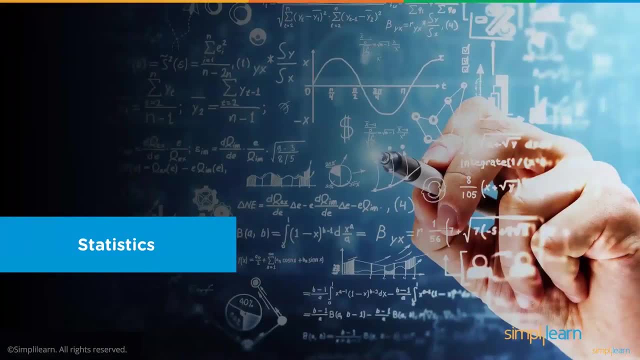 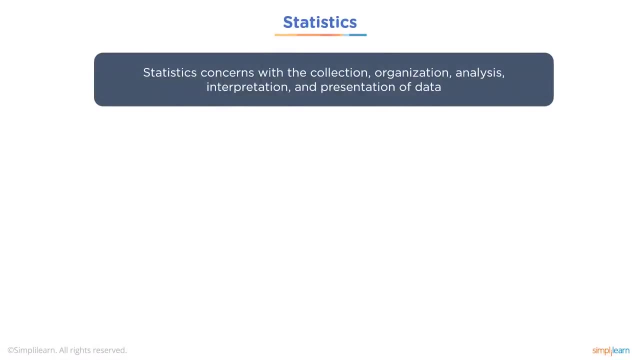 That brings us to statistics. What this is kind of all about is figuring things out, A lot of vocabulary and statistics. So statistics- well, I guess it's all relative. It's definitely not an Edel class. So a bunch of stuff going on in statistics. 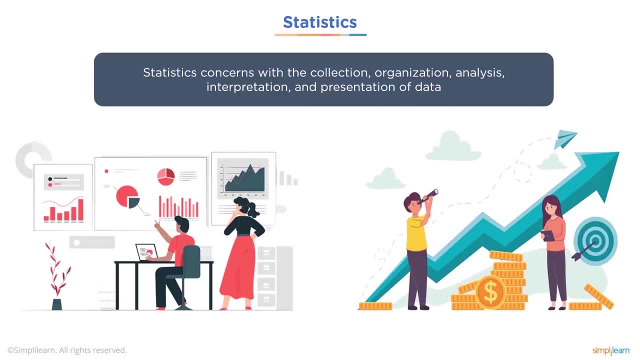 Statistics concerns with the collection, organization, analysis, interpretation and presentation of data. That is a mouthful, So we have from end to end. where does it come from? Is it valid? What does it mean? How do we organize it? 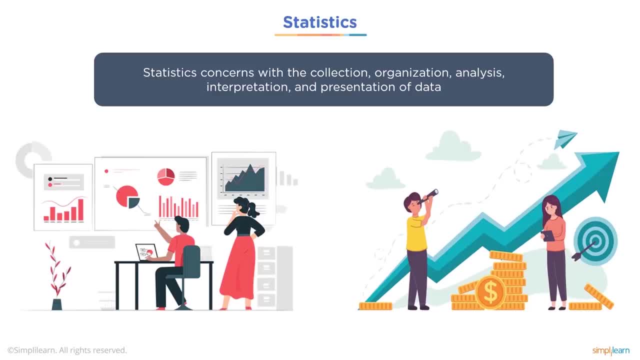 How do we analyze it? Then you've got to take those analyses and interpret it into something that people can use, kind of reduce it, Make it understandable, And nowadays you have to be able to present it. If you can't present it, then no one else is going to understand. 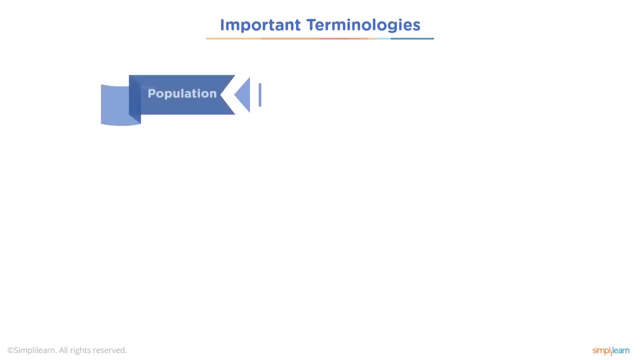 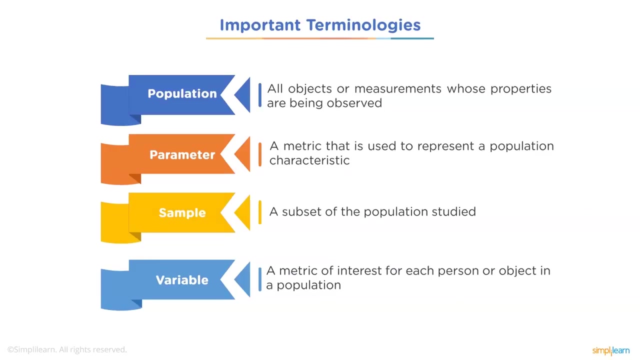 what the heck you did. So when we look at the terminologies, there is a lot of terminologies depending on what domain you're working in. So clearly, if you're working in a domain that deals with viruses and T cells- and where does it come from? 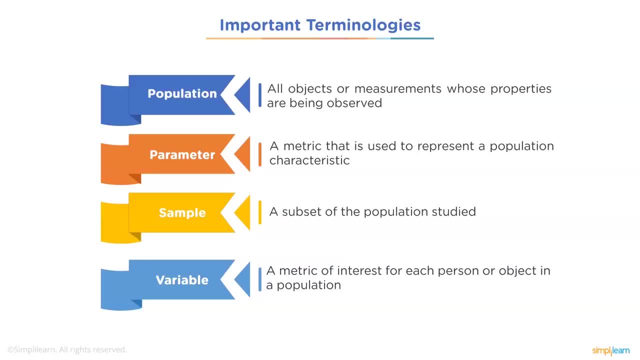 and you're studying the different people, then you're going to have a population- If you are working with mechanical gear, a little bit different. If you're looking for the wobbling statistics to know when to replace a rotor on a machine or something like that. 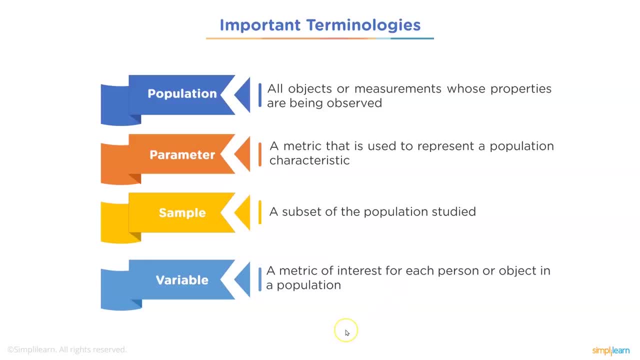 That can be a big deal. We have these huge fans that turn in our sewage processing systems, And so those fans- they start to wobble and hum and do different things. If the sensors pick up at one point, you replace them instead of waiting for it to break. 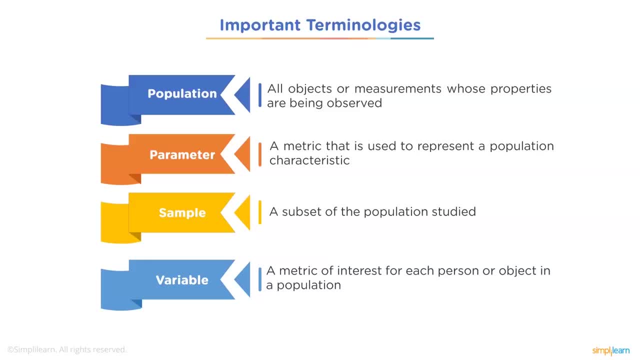 in which case it costs a lot of money. Instead of replacing a bushing, you're replacing the whole fan unit, An interesting project that came up for our city a while back. So population- All objects- are measurements whose properties are being observed. 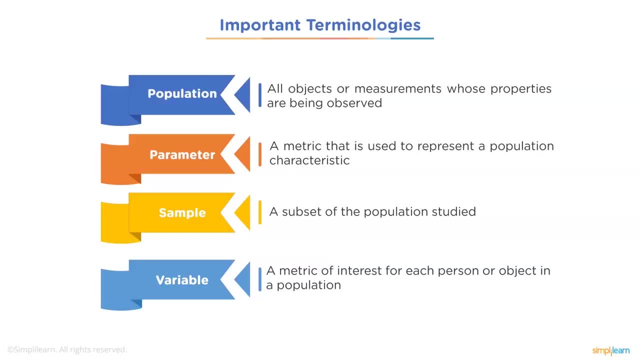 So that's your population, All the objects. It's easy to see it with people because we have our population in large, But in the case of the sewer fans, we're talking about the fan units. That's the population of fans that we're working with. 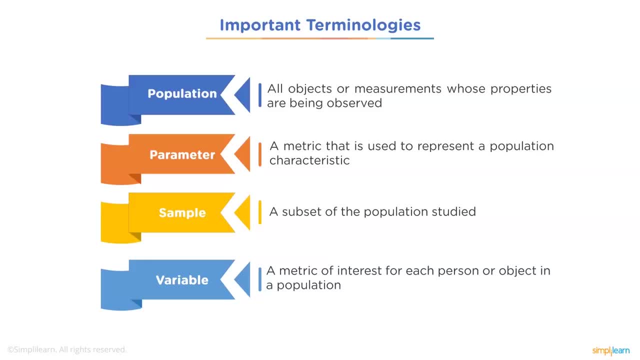 You have a parameter, a metric that is used to represent a population or characteristic. You have your sample, a subset of the population studied. You don't want to do them all, because then you don't have a if you come up with a conclusion for everyone. 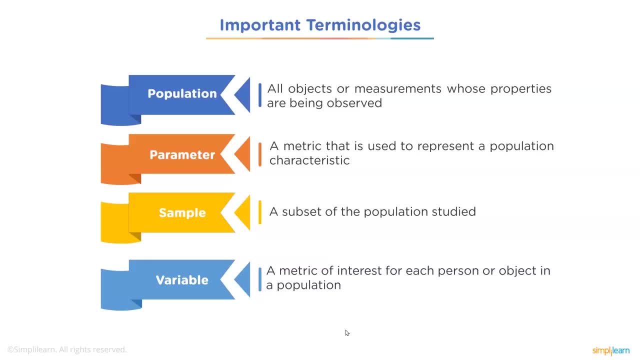 you don't have a way of testing it, So you take a sample. Sometimes you don't have a choice. You can only take a sample of what's going on. You can't study the whole population And a variable, a metric of interest for each person. 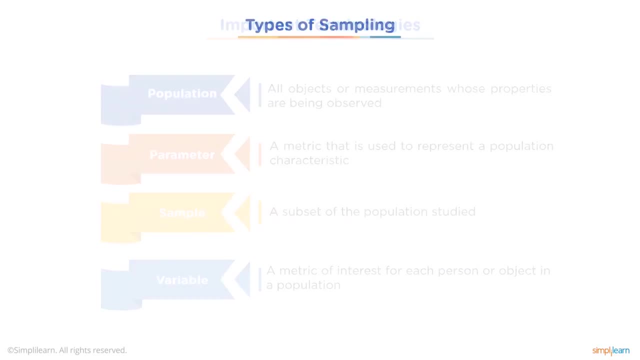 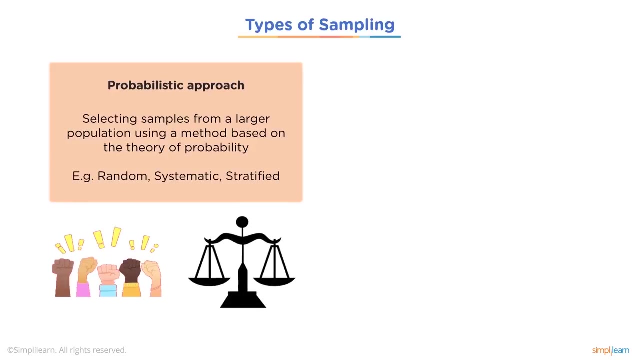 or object in a population. Types of sampling: We have probabilistic approach, selecting samples from a larger population using a method based on the theory of probability, And we'll go into a little bit more deeper on these. We have random, systematic stratified. 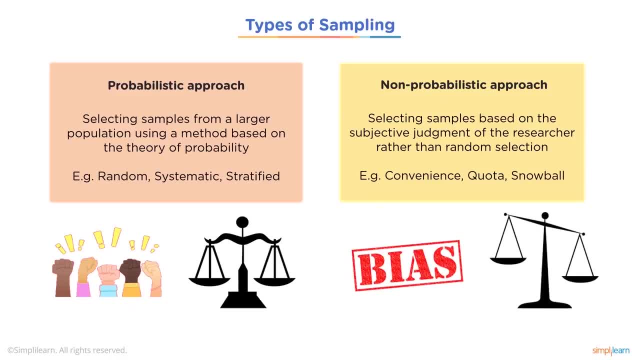 And then you have non-probabilistic approach, selecting samples based on the subjective judgment of the researcher rather than random selection. It has to do with convenience- whether you're going to reach a quota or a snowball- And they're very biased. 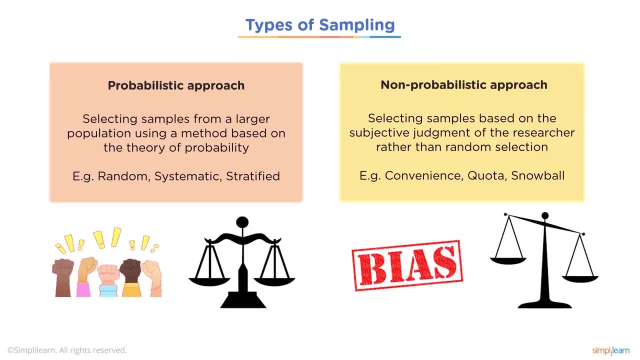 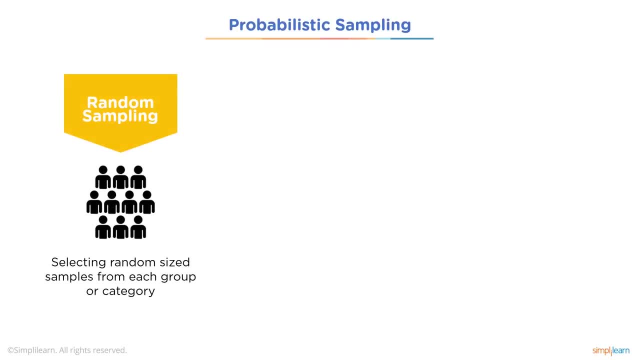 That's one of the reasons you'll see this big stamp on it that says biased. So you've got to be very careful on that. So, probabilistic sampling: When we talk about a random sampling, we select random size samples from each group or category. 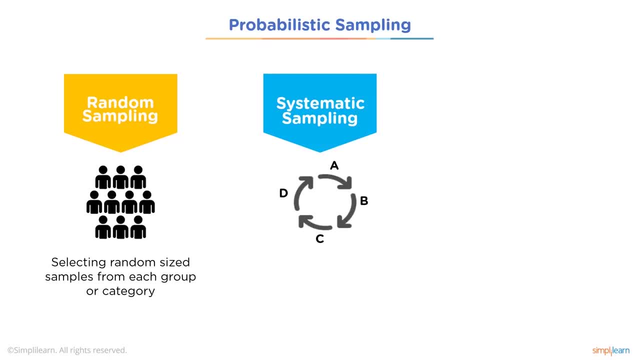 So it's as random as you can get. When we talk about systematic sampling, we're selecting random size samples from each group or category with a fixed periodic interval, So we kind of split it up. This would be like a time setup or different categories. 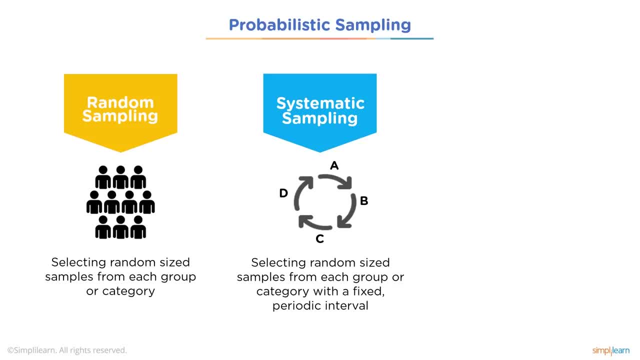 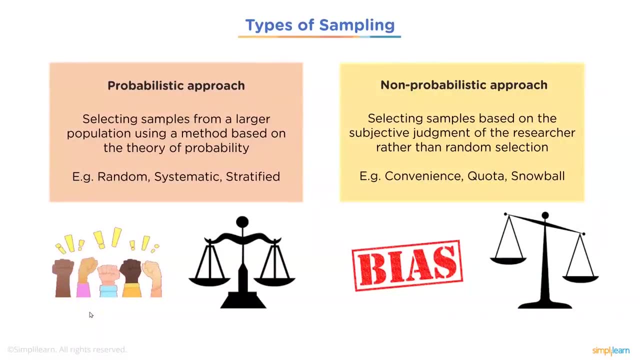 And you might ask your question: well, what is a category or a group? If you look at, I'm going to go back a window. Let's say we're studying economics of an area We know pretty much that based on their culture. 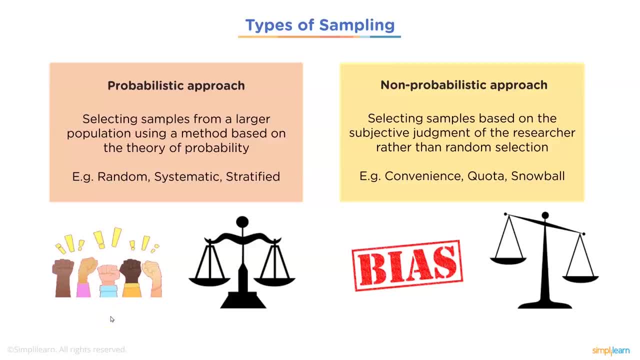 and where they came from, they might need to be separated, And so- And when I say separated, I don't mean separated from their place, where they live, I mean, as far as the analysis, we want to look at the different groups. 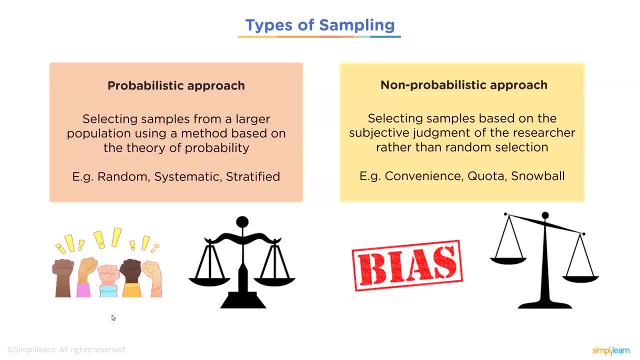 and make sure they're all represented. So if we had like an 80% of a group, that is say, Hispanic or Indian, and also in that same area we have 20% who are, let's call our expatriates. 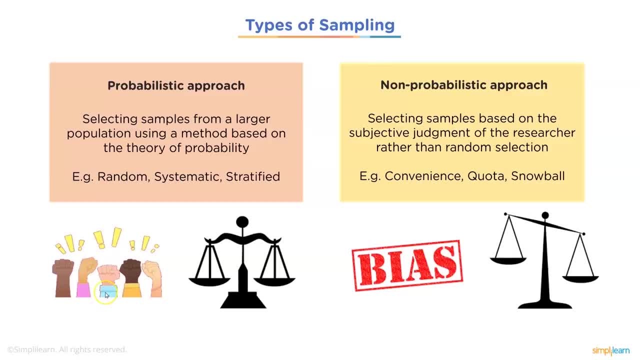 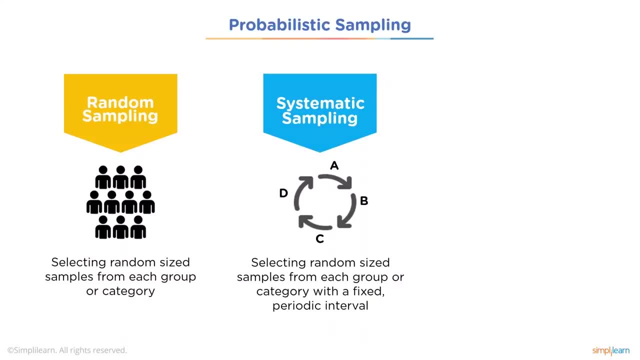 They left America and they're nice. your Caucasian group, We might want to sample a group that is representative of both. So we're talking about stratified sampling and we're talking about groups. Those are the groups we're talking about, And that brings us to stratified sampling. 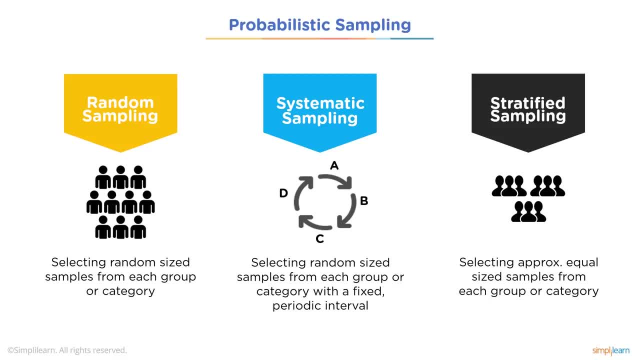 selecting approximately equal size samples from each group or category. This way we can actually separate the categories and give us an insight into the different cultures and how that might affect them in that area. So you can see, these are very, very different. kind of depends on what you're working with. 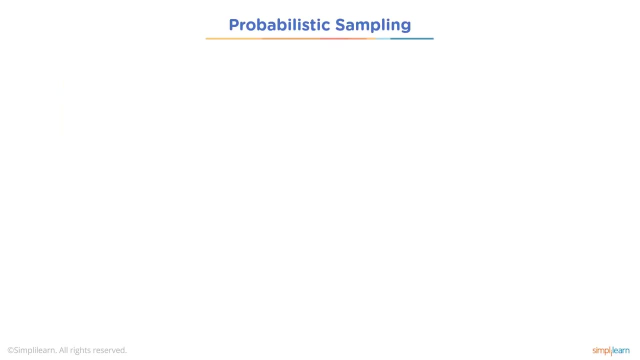 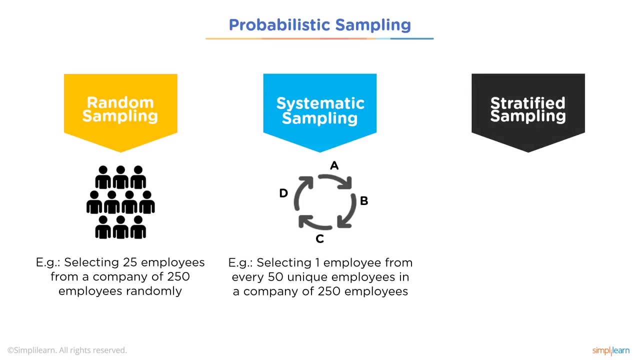 As far as your data and what you're studying, And so we can see here, just to go a little bit more, we'd have selecting 25 employees from a company of 250 employees randomly. Don't care anything about them, what groups they're in. 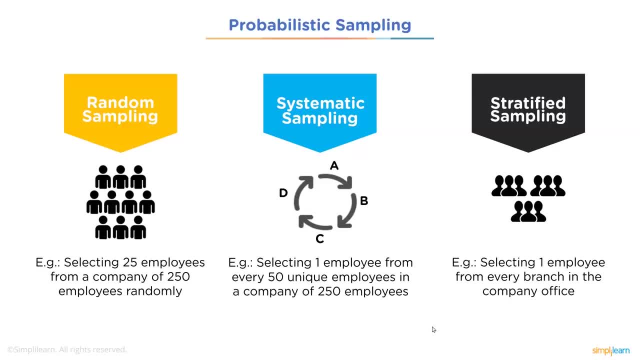 which office they're in nothing, And we might be selecting one employee from every 50 unique employees in a company of 250 employees. And then we have selecting one employee from every branch in the company office, So we have all the different branches. 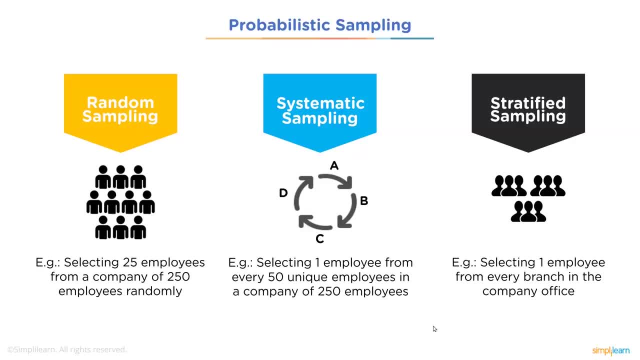 There's our group or our categories by the branch, And the category could depend on what you're studying, So it has a lot of variation on there. You see, this kind of grouping and categorizing is also used to generate a lot of misinformation. 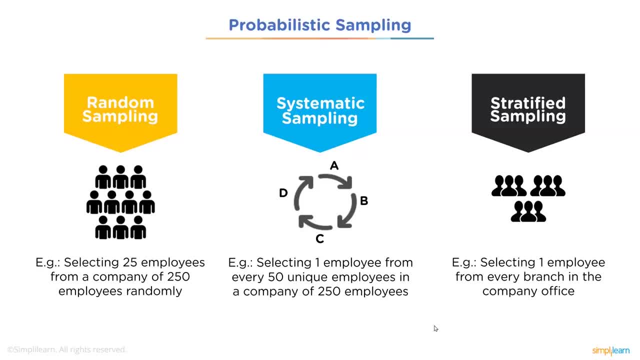 So if you only study one group and you say this is what it is, then everybody assumes that's what it is for everybody, And so you got to be very careful of that, and it's very unethical thing to kind of do So. types of statistics. 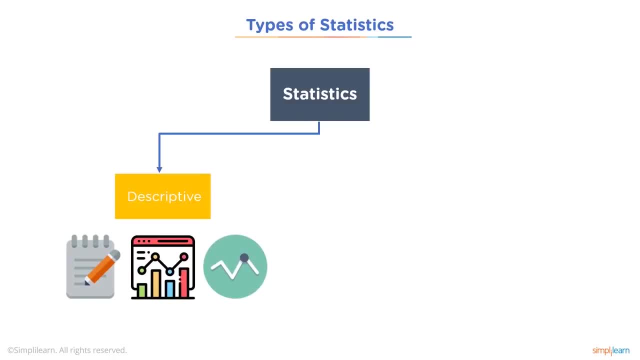 When we talk about statistics, we're going to talk about descriptive and inferential statistics. There are so many different terms and statistics to break it up, So we're talking about a particular setup. So we're talking about descriptive and inferential statistics. 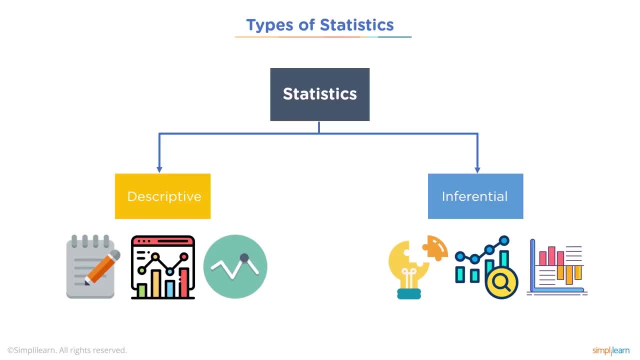 The base of the word describe is pretty solid. You're describing the data. What does it look like With inferential statistics? we're going to take that from the small population to a large population. So if you're working with a drug company, 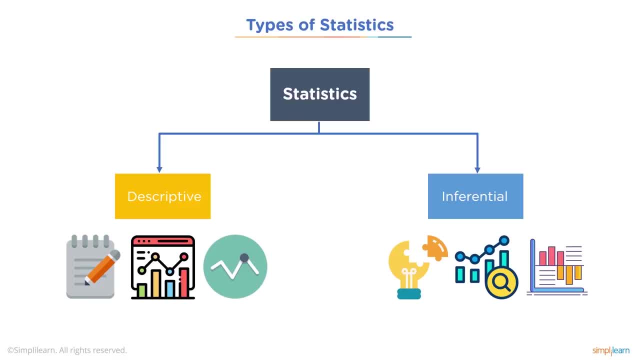 you might look at the data and say these people were helped by this drug. They did 80% better as far as their health, or 80% better survival rate, than the people who did not have the drug. So we can infer that that drug will work. 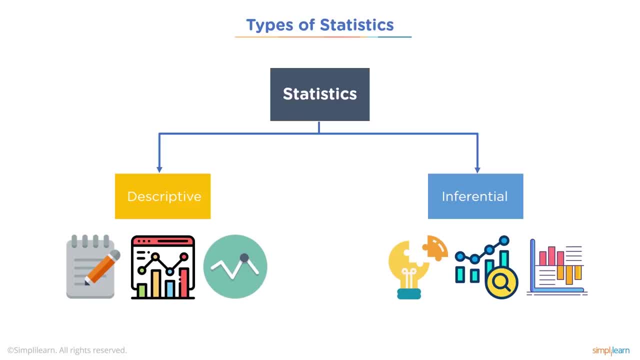 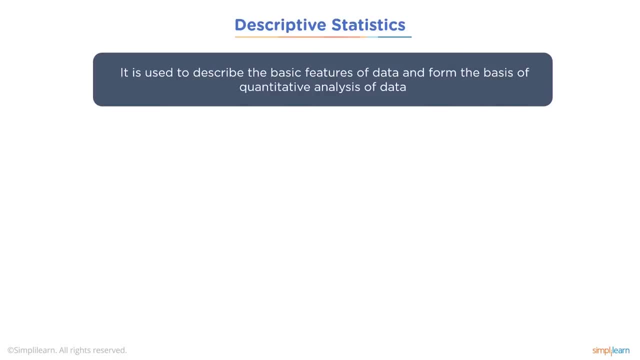 in the greater populace and will help people. So that's where you get your inferential. So we are predicting how it's going to affect the greater population. So descriptive statistics. It is used to describe the basic features of data and form the basis of quantitative analysis of data. 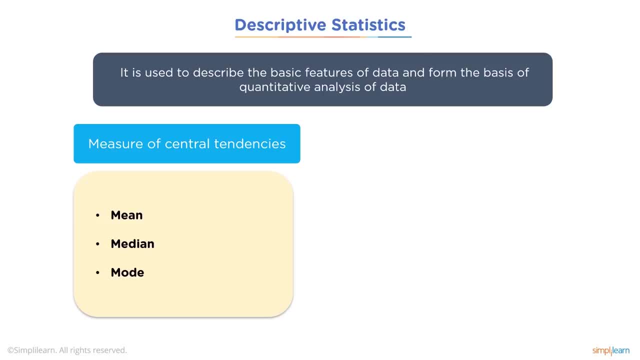 So we have a measure of central tendencies, We have your mean, median and mode, And then we have a measure of spread, like your range, your interquartile range, your variance and your standard deviation, And we're going to look at all these. 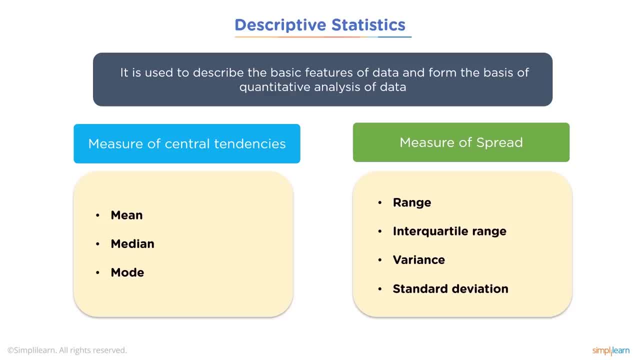 a little deeper here in a second, But one of them you can think of is how the data differences. what's the max- min range? all that stuff is your spread, And anything that's just a single number is usually your central tendencies. 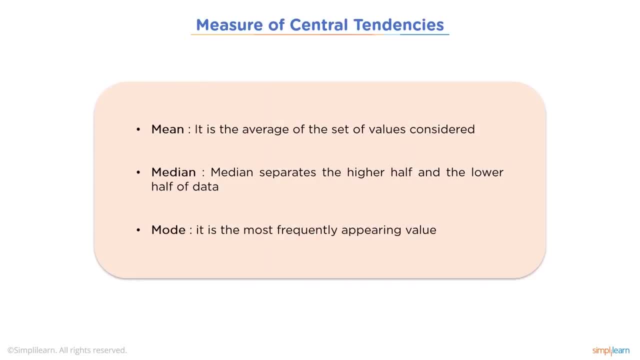 measure of central tendencies. So we talk about the mean. It is the average of the set of values considered. What is the average outcome of whatever's going on? And then your median separates the higher half and the lower half of data. So where's the center point? 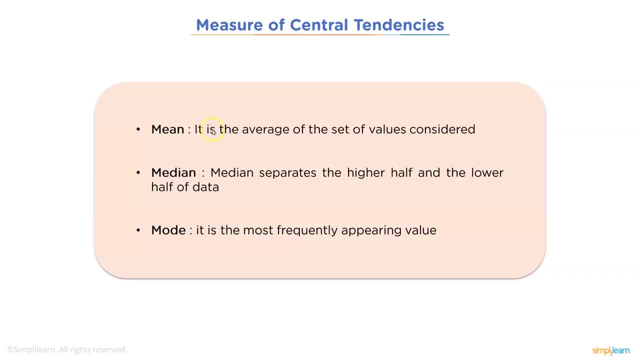 of all your different data points. So your mean might have a couple really big numbers that skew it so that the average is much higher than if you took those outliers out, where the median would, by separating the high from the low, might give you a much lower number. 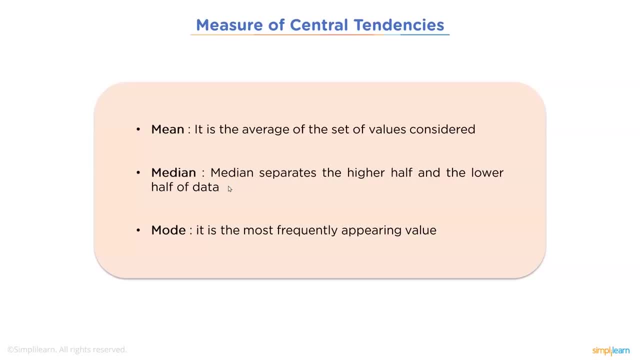 You might look at it and say, oh, that's odd. Why is the average so much higher than the median? Well, it's because you have some outliers, Or why is it so much lower? And then the mode is the most frequent appearing value. 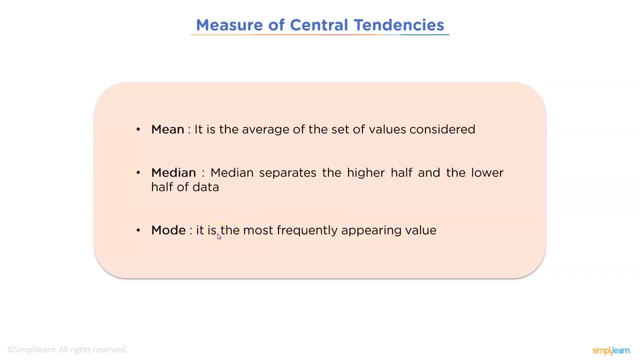 This is really interesting. if you're studying economics and how people are doing, You might find that the most common income, like in the US, was 1.24 thousand a year, where the average was closer to 80 thousand, And it's like, wow, what a difference. 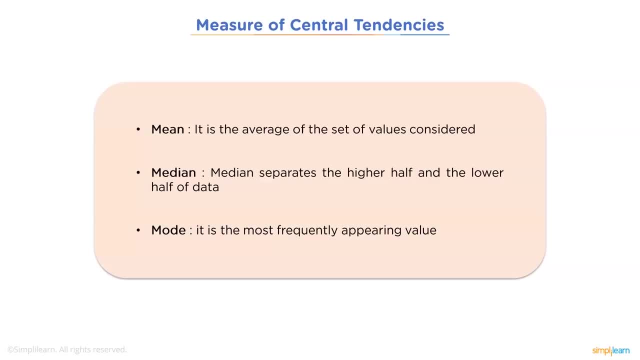 Well, there's some people who have a lot of money And so that skews that way up. So the average person is not making that kind of money. And then you look at the median income and you're like: well, the median income. 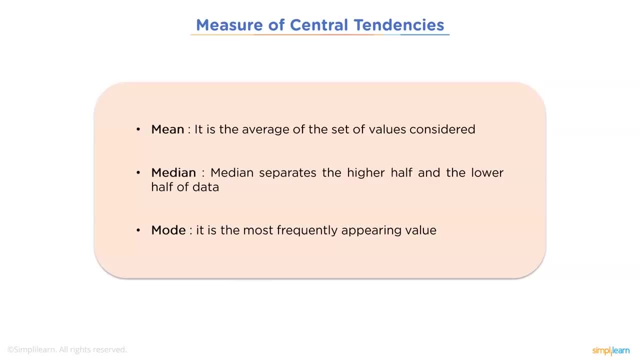 is a little bit closer to the average, So it does create a very interesting way of looking at the data. Again, these are all central tendencies, single numbers you can look at for the whole spread of the data And when we look at the measure of central tendencies. 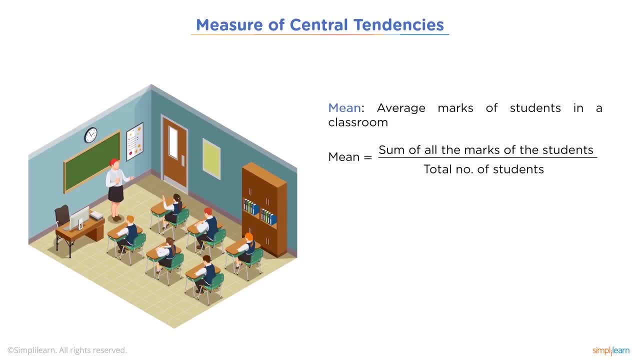 the mean is the average marks of a student in a classroom. So here we have the mean sum of the marks of the students, total number of students And, as we talked about the median, if we have 0 through 10, and we take half the numbers, 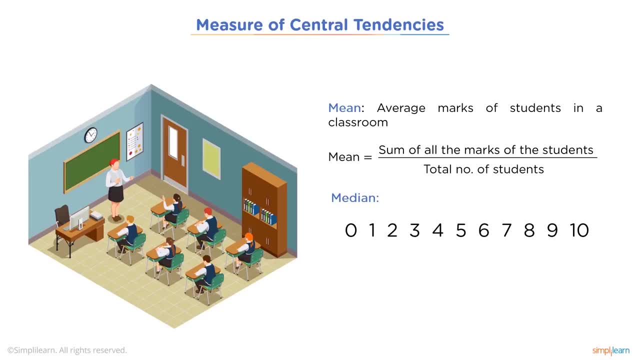 and put them on one side of the line. half the numbers on the other side of the line. we end up with 5 in the middle. And then the mode: What mark was scored by most of the students in a test? In a simple case where most people scored like an 82%, 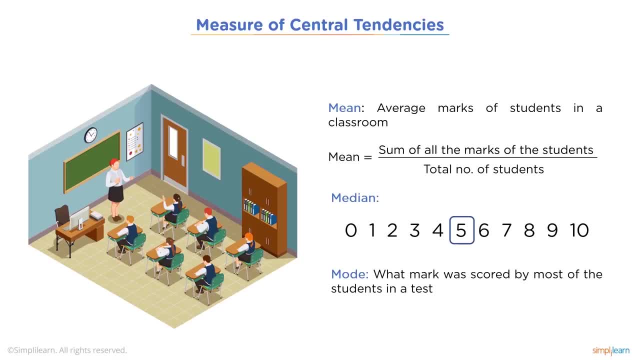 and got certain problems wrong. easy to figure out. Not so easy when you have different areas where, like you have, like the- oh, let's go back to economy- A little bit more difficult to calculate if you have a large group that makes 30,000. 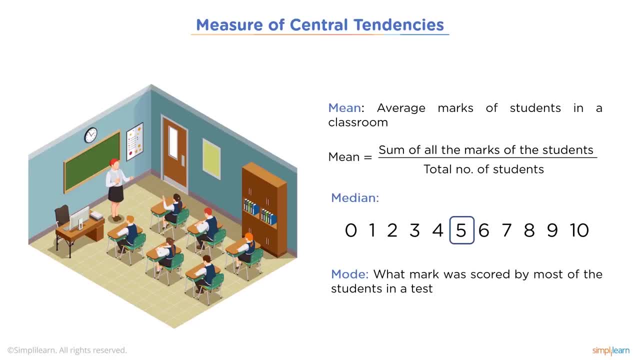 and a slightly bigger group that makes 26,000.. So what do you put down for the mode? Certainly, there's a number of ways to calculate that, and there's actually different variations depending on what you're doing. So now we're looking at a measure of spread. 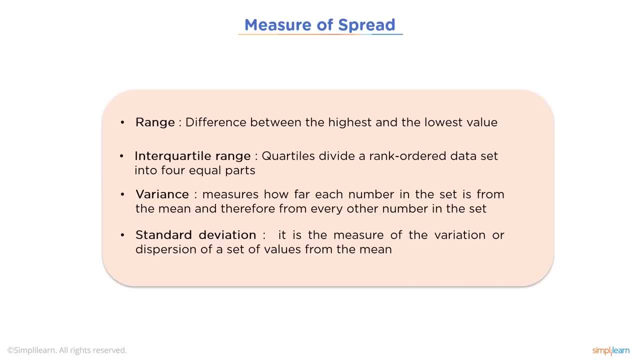 Range. What's the difference between the highest and the lowest value? First thing you want to look at. We had everybody in the test score between 60 and 100%. Somebody got 100% Or maybe 60 to 90%. It was so hard that a lot of people could not get 100%. 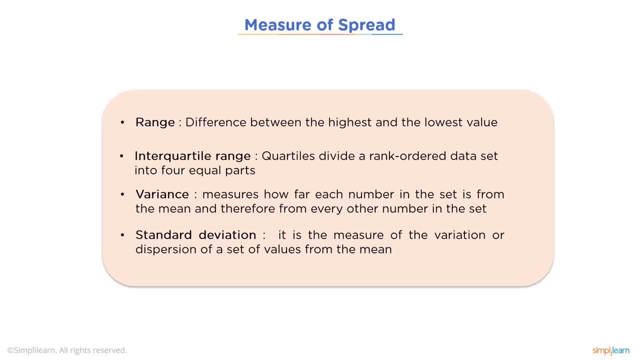 Then you have your interquartile range. Quartiles divide a rank order data set into four equal parts. Very common thing to do as part of all the basic packages, whether you're working in data frames with pandas, whether you're working in Scala. 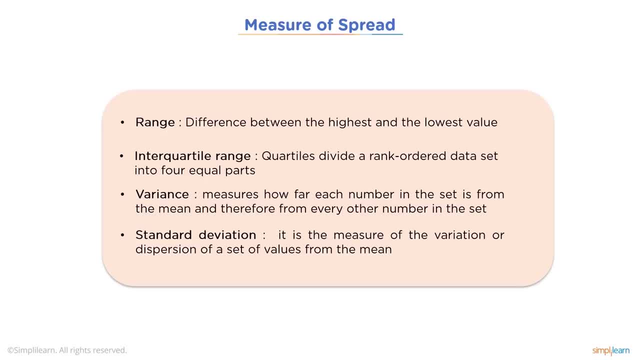 whether you're working in R, You'll see this come up where they have range, your min, your max, and then it'll have your interquartile range. How does it look like in each quarter of data Variance measures how far each number in the set? 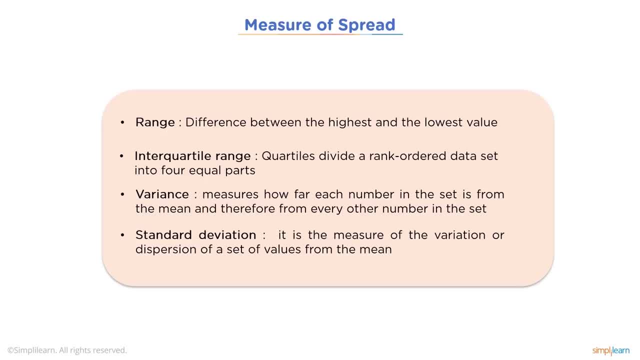 is from the mean and therefore from every other number in the set. So you have, like a how much turbulence is going on in this data? And then the standard deviation. It is the measure of the variance or the dispersion of a set of values from the mean. 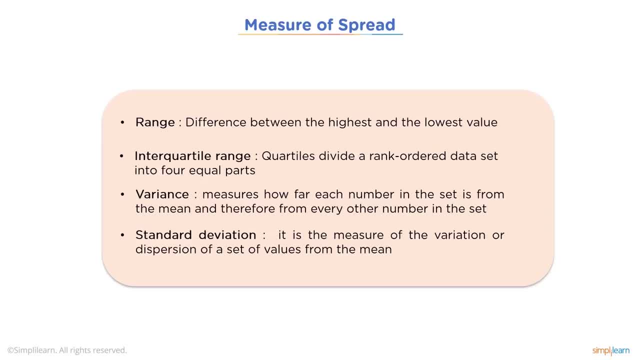 And you'll usually see if I'm doing a graph. I might have the value graphed and then, based on the error, I might graph the standard deviation and the error on the graph as a background so you can see how far off it is. 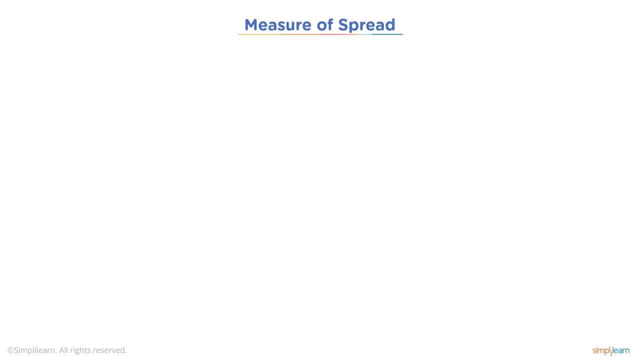 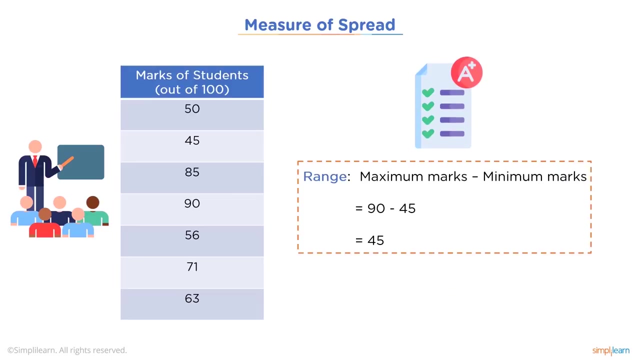 So standard deviation is used a lot. So measurement of spread Marks of a student out of 100.. We have here from 50 to 63, or 50 to 90.. So the range: maximum marks, minimum marks, we have 90 to 45,. 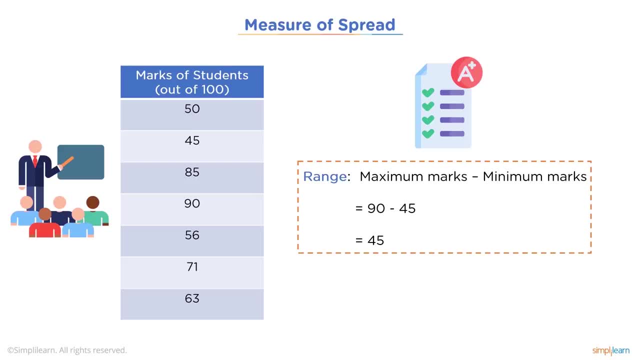 and the spread of that is 45.. 90 minus 45. And then we have the interquartile range. using the same marks over there, You can see here where the median is. And then there's the first quarter, the second quarter, 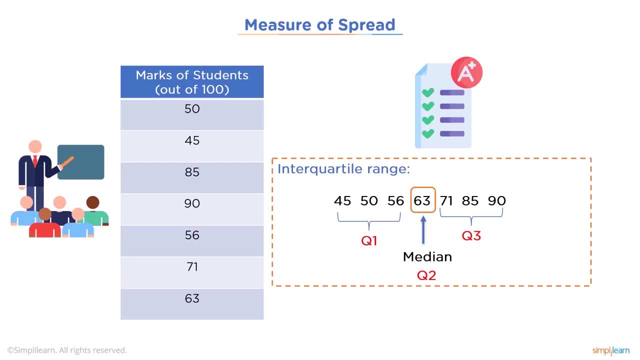 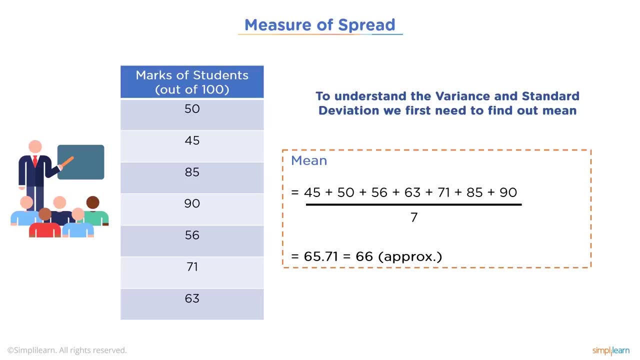 and the third quarter, based on splitting it apart by those values. And to understand the variance and standard deviation we first need to find out the mean. So here's our, you know, calculating the average there, We end up at approximately 66 for the average. 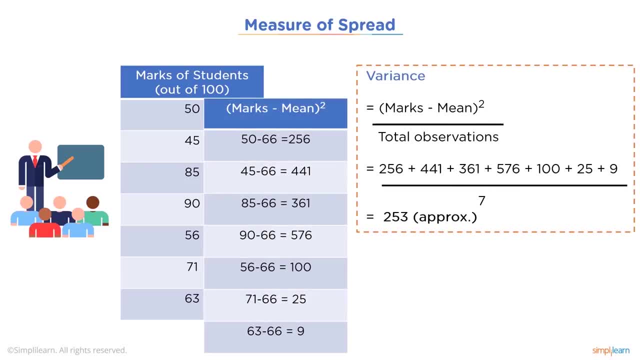 And then we look at that and the variance, once we know the means we can do, equals the marks minus the mean squared. Why is it squared? Because one you want to make sure you don't have. like, if you're putting all this stuff together. 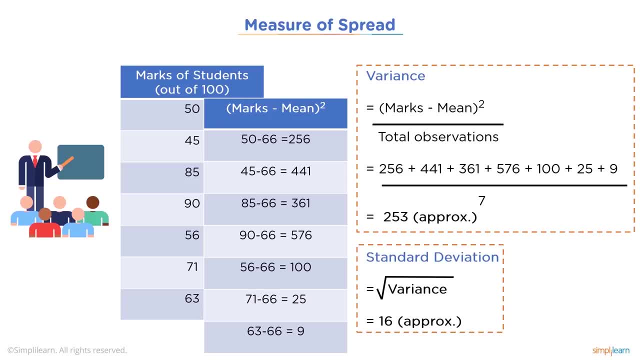 you end up with an error as far as one's negative, one's positive, one's a little higher, one's a little lower. So you always see the squared value and over the total observations, And so the standard deviation equals the square root of the variance. 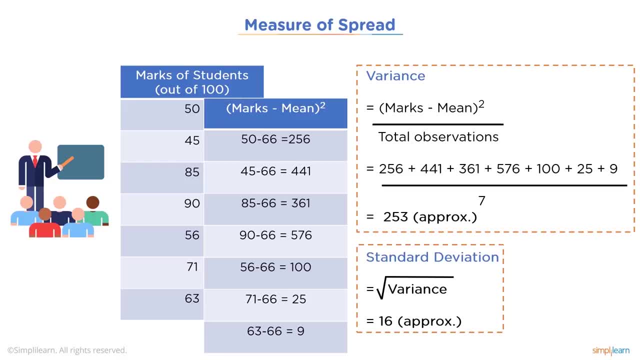 which is approximately 16.. And if you were looking at a predictable model, you would be looking at the deviation based on the error. How much error does it have? And that's again really important to know if your prediction is predicting something. 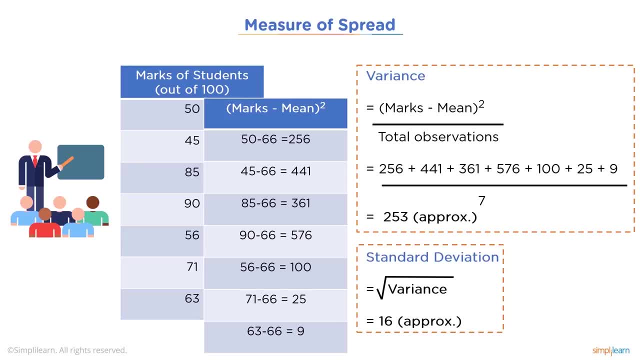 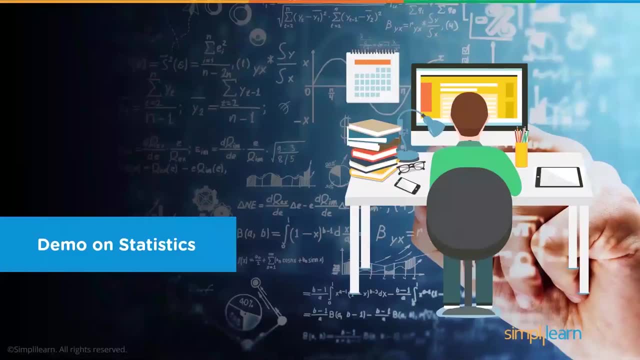 what's the chance of it being way off or just a little bit off? Now that we've looked at the tools, as far as some of the basics for doing your statistics and what we're talking about, let's go ahead and pull up a little demo. 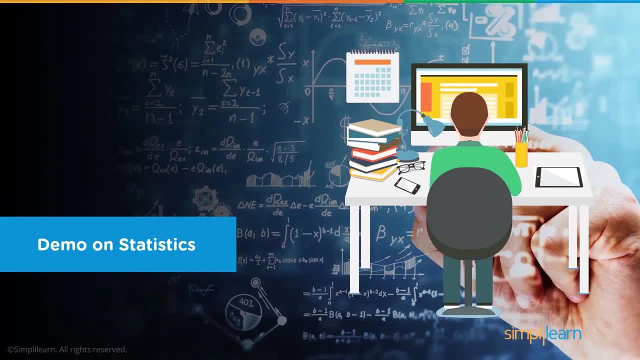 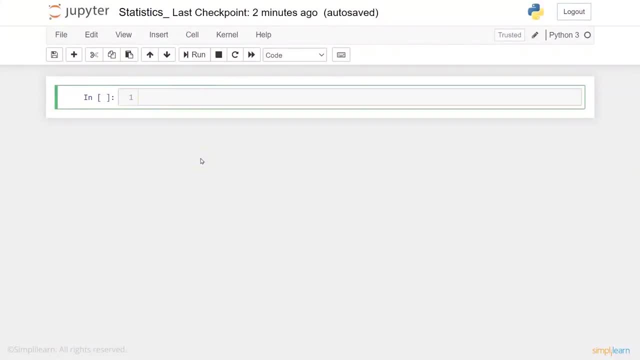 and show you what that looks like in Python code. So you can get some little hands on here. For that, let's go back into our Jupyter notebook in Python Now. almost all of this you can do in NumPy. Last time we worked in NumPy. 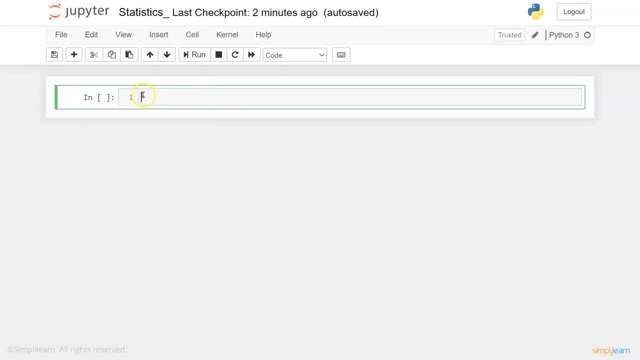 This time we're going to go ahead and use Pandas And if you remember from Pandas on YouTube, we had some pandas on here. This is basically a data frame: rows, columns- Let's just go ahead and do a print: dfhead. 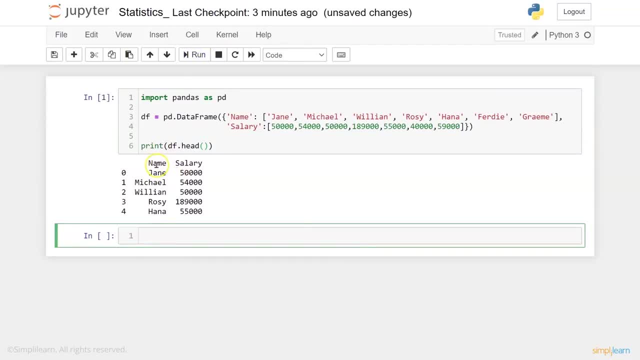 and run that And you can see. we have the name Jane, Michael, William, Rosie, Hannah and their salaries on here. And, of course, instead of having to do all those hand calculations and add everything together and divide by the total, 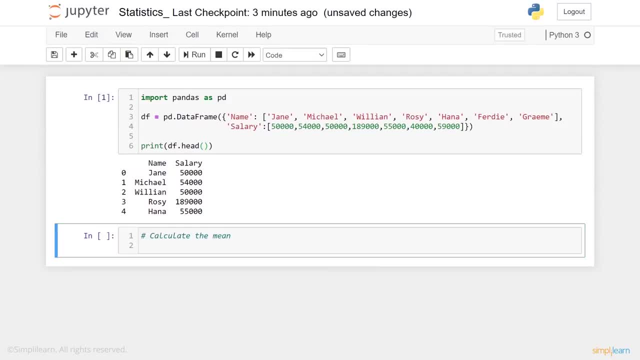 we can do something very simple on this, like use the command mean in Pandas. And so if I go ahead and do this, print df, pick our column salary, because we want to find the means of that collary. We want to find the means. 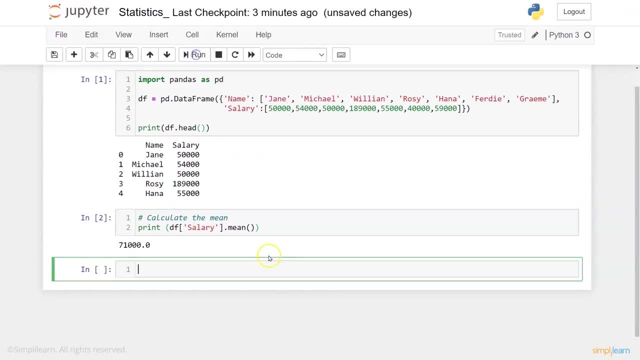 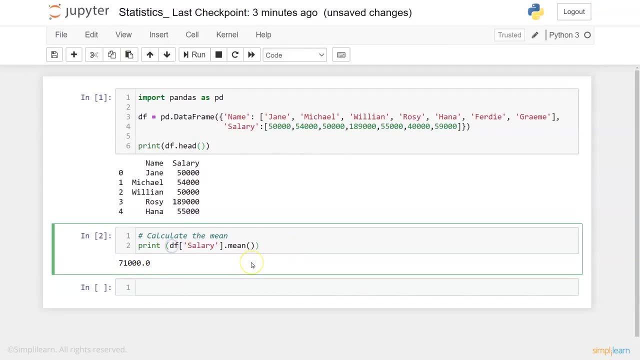 of that column And we go ahead and print this out And you can see that the average income on here is $71,000.. And let's just go ahead and do this. We'll go ahead and put in means, And if we're going to do that, 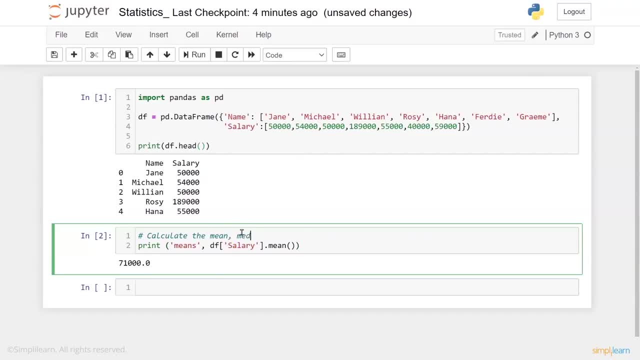 we also might want to find the median, And the median is very similar, except it actually is just median. We're used to means and average. It's kind of interesting that those are used as two different words. There can be in some computations. 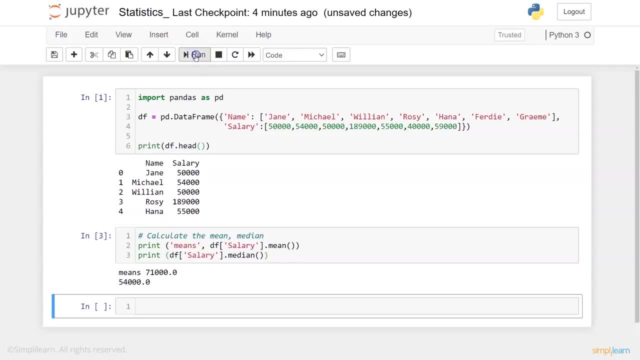 slight differences, but for the most part the means is the average. And then the median. oops, let's put a median here: df salary. that way it displays a little better. We can see the median is $54,000. 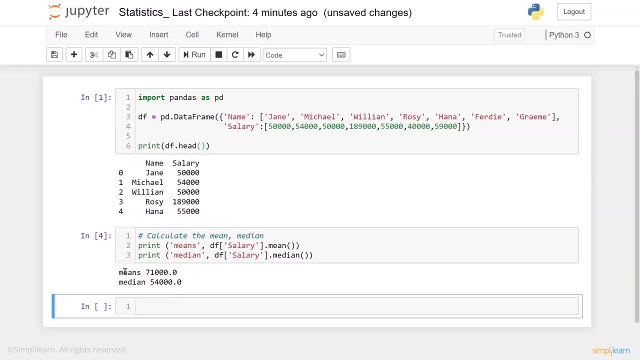 So the halfway mark is significantly below the average. Why? Because we have somebody in here who makes $189,000.. Darn you, Rosie, for throwing off our numbers, But that's something you'd want to notice. This is the difference between these. 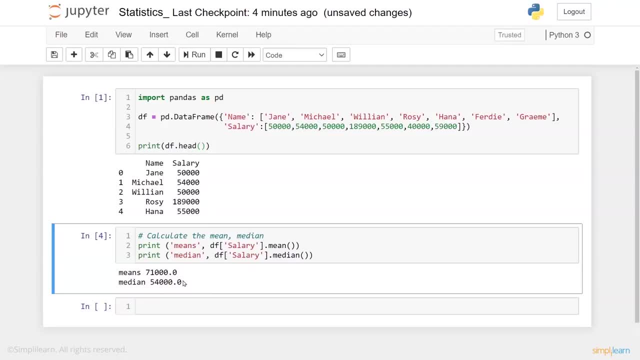 is huge, and so is what is the meaning behind that when you're studying a populace and looking at the different data coming in. And of course, we also want to find out, hey, what's the most common income that people make In this little, tiny sample? 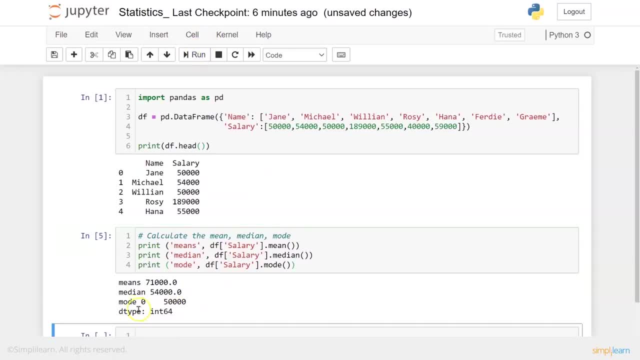 and so we'll go ahead and do the mode. And you can see here with the mode it's at $50,000.. So this is very telling that most people are making $50,000.. The middle point is at $54,000,. 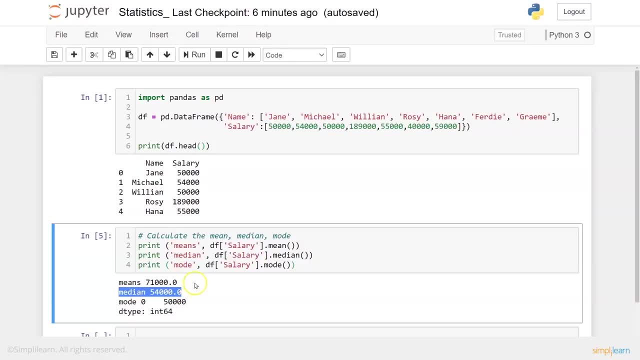 so half the people are making more than that. What that tells me is that if the most common income is below the median, then there's a lot of- you know- high salaries going up, but there's some really low salaries in there. 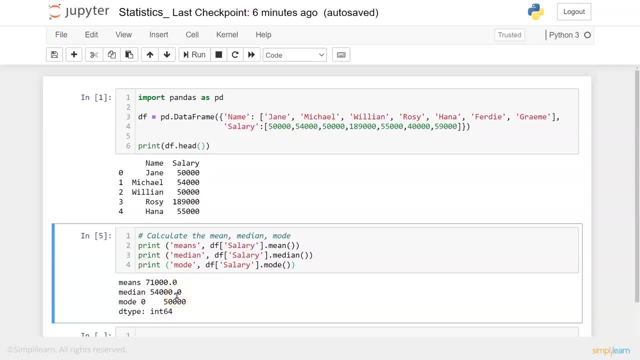 And so this trend, which is very common in statistic- you know, when you're analyzing the economy and different people's income- is pretty common And the bigger difference between these is also very important when we're studying statistics And when you hear someone just say: 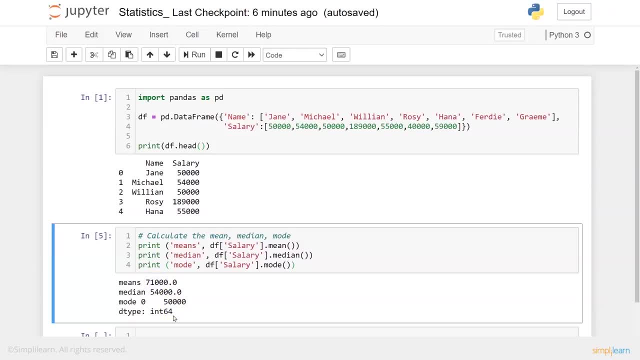 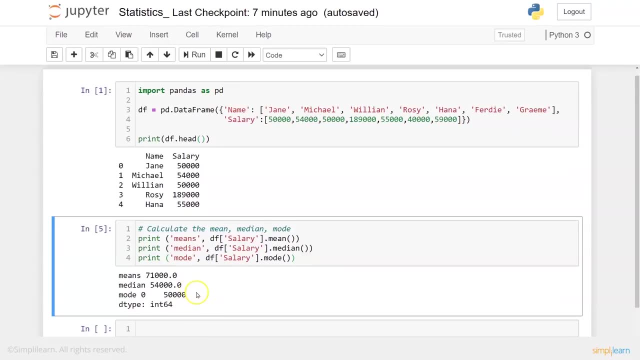 hey, the average income was. you might start asking questions at that point. Why aren't you talking about the median income? Why aren't you talking about the mode, the most common income? What are you hoping, you're hiding And if you're doing, 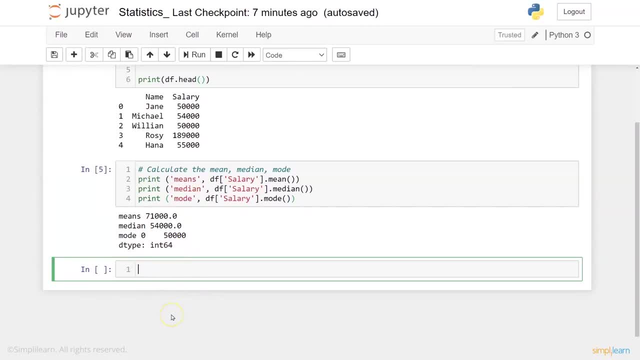 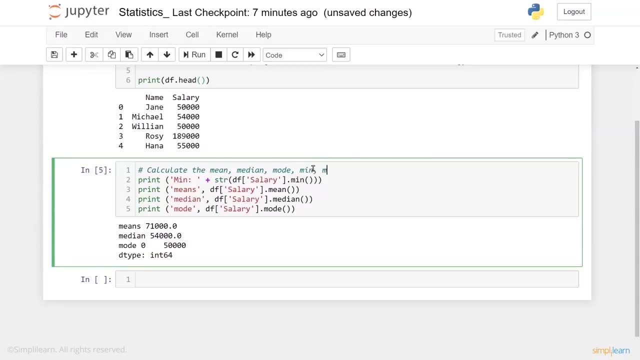 these analysis. you should be looking at these saying hey, why are these discrepancies, Why are these so different? And of course, with any analysis, it's important to find out the minimum and the maximum. So we'll go ahead. It's just simply dot min. 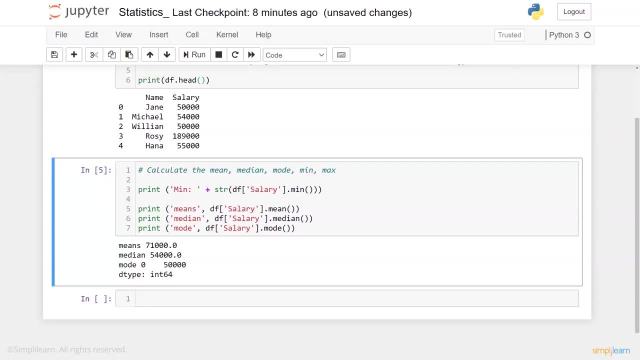 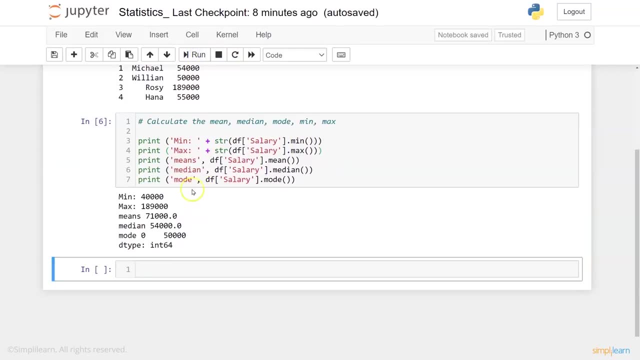 It'll pull up your minimum and then dot max pulls up the maximum. Pretty straightforward on as far as translating it and knowing what your- you know- lowest value and what your highest value is here, which you'll use to generate like a spread later on. 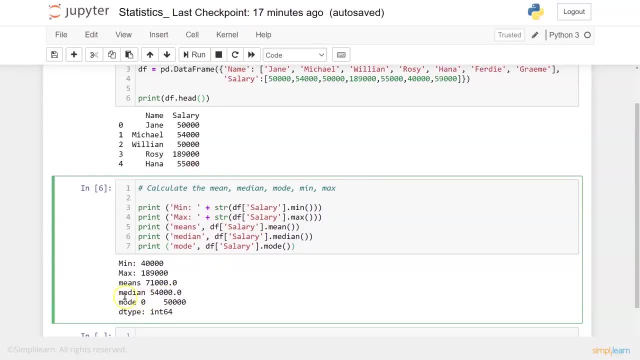 And real quick. on mode, note that it puts mode zero. Like I said, there's a couple different ways you can compute the mode. Although you know the standard one's pretty good, We can, of course do the range. 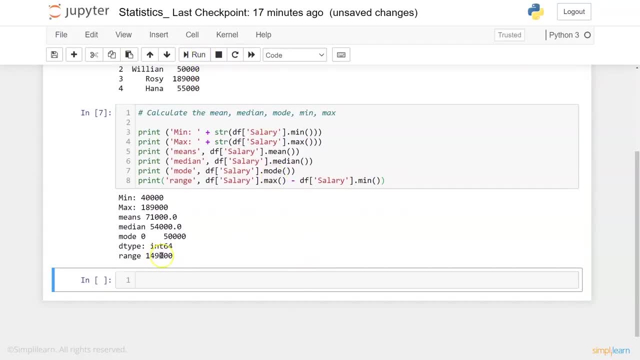 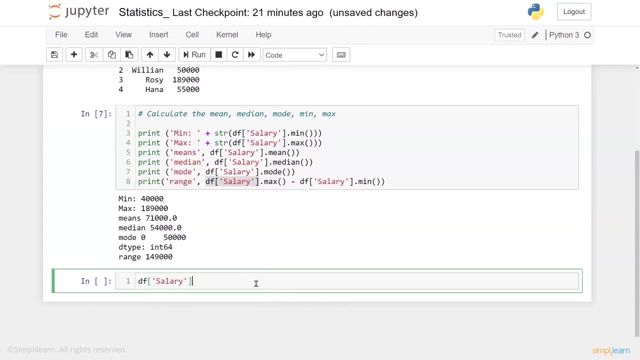 which is your max minus your min. So now we have a range of 149,000 between the upper end and the lower end, And you might want to be looking up the individual values on all of these, But it turns out there is a describe feature. 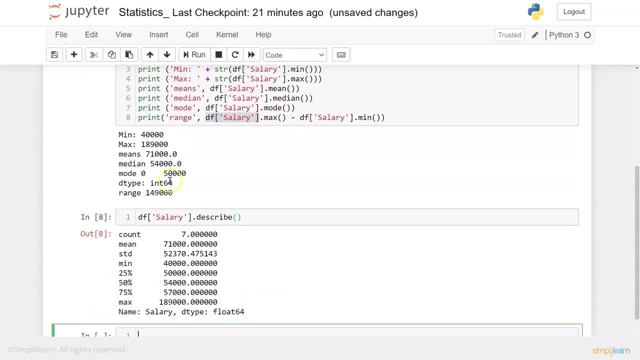 in Pandas, And so in Pandas we can actually do DFSALARYDESCRIBE, And if we do this, you can see we have that there's seven setups. Here's our mean, our standard deviation, which we didn't compute yet. 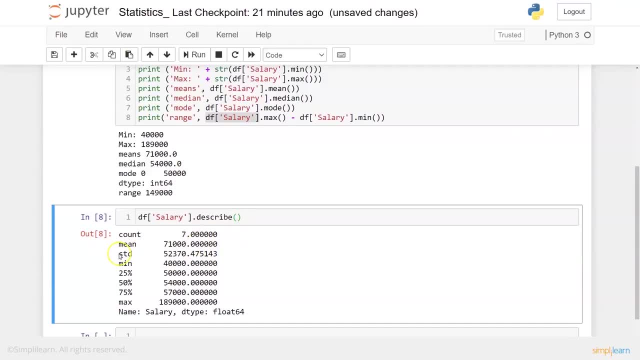 which would just be a dot STD. And you got to be a little careful, because when it computes it it looks for axes and things like that. We have our minimum value and here's our quartile, Our maximum value, and then, of course, 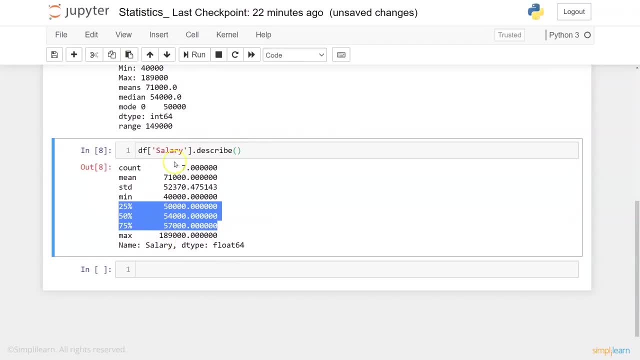 the name salary. So these are the basic statistics. You can pull them up and just describe. This is a dictionary, So I could actually do something like in here. I could actually go count and run And now it just prints the count. 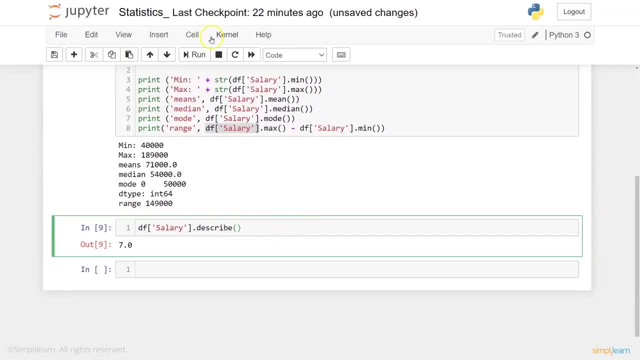 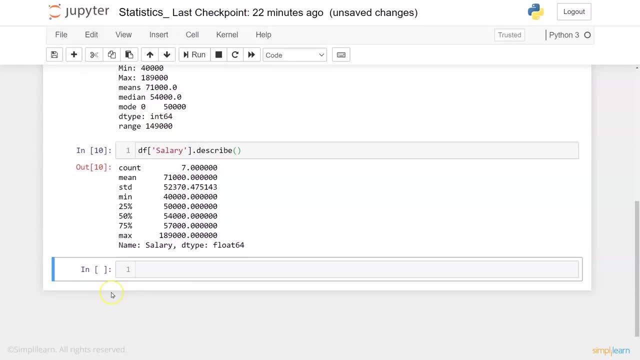 So, because this is a dictionary, you can pull any one of these values out of here. It's kind of a quick and dirty way to pull all the different information and then split it up and depending on what you need. Now, if I just walked in, 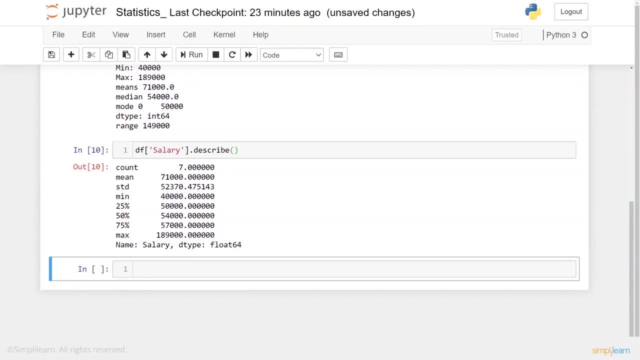 and gave you this information in a meeting at some point, you would just kind of fall asleep. That's what I would do anyway. So we want to go ahead and see about graphing it here And we'll go ahead and put it into a histogram. 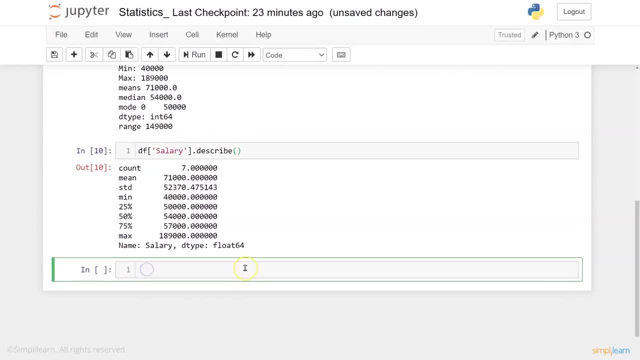 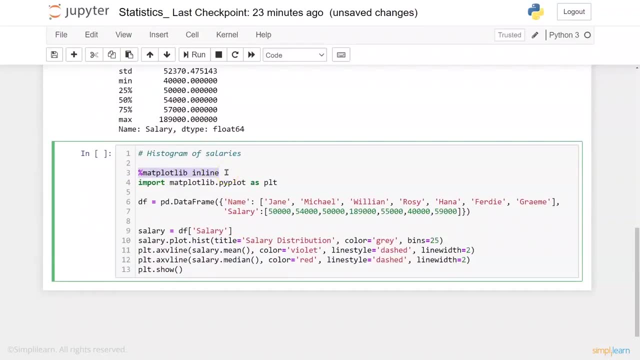 and plot that graph on it of the salaries And let's just go ahead and put that in here. So we do our map plot inline. Remember that's a Jupyter's notebook thing. A lot of the new version of the map plot library. 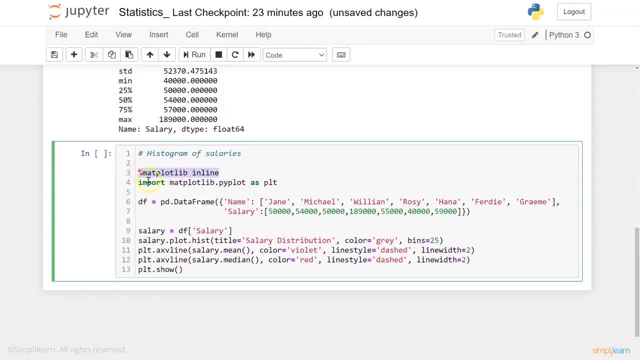 does it automatically, But just in case I always put it in there. Import map plot library. Pyplot is PLT. That's my plotting, And then we have our data frame. I guess I really don't need to re-spell the data frame. 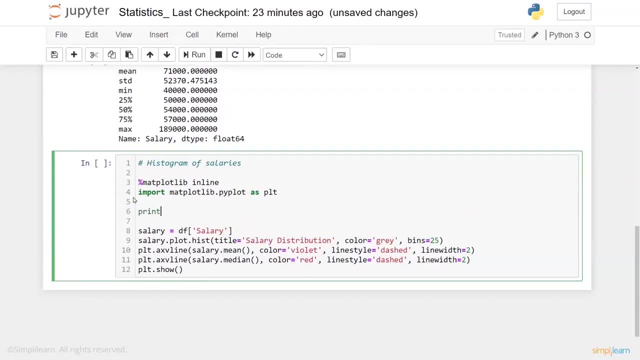 Maybe we could just remind ourselves what's in it. So we'll go ahead and just print df. That way we still have it, And then we have our salary df. salary salaryplot history. title: salary distribution. color: gray plot ax. 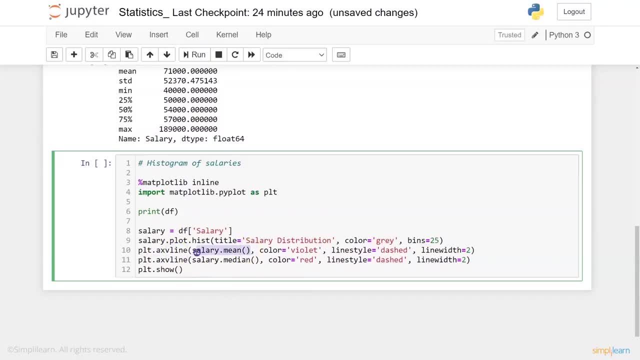 vline salary, the mean value. So we're going to take the mean value. Color violet line style dash- This is just all making it pretty. What color dash line line width of two, that kind of thing, And the median. 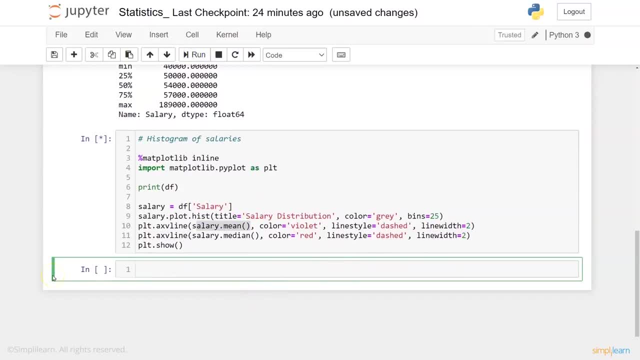 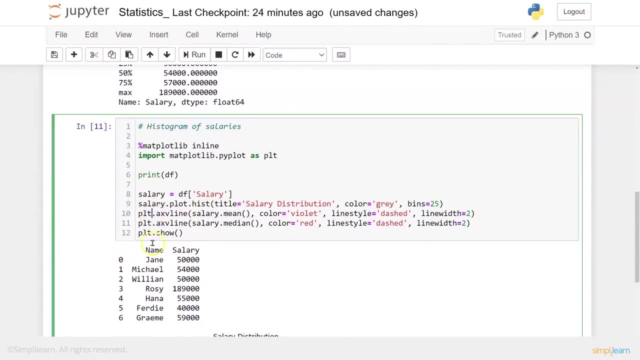 And let's go ahead and run this, just so you can see what we're talking about. And so up here we are taking on our plot. So here's the data, Here's our data frame. Print it out so you can see it, with the salaries. 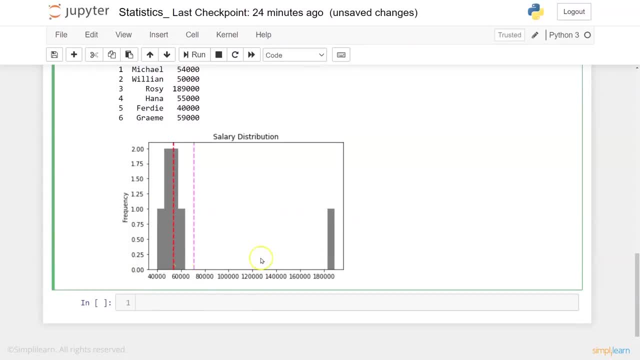 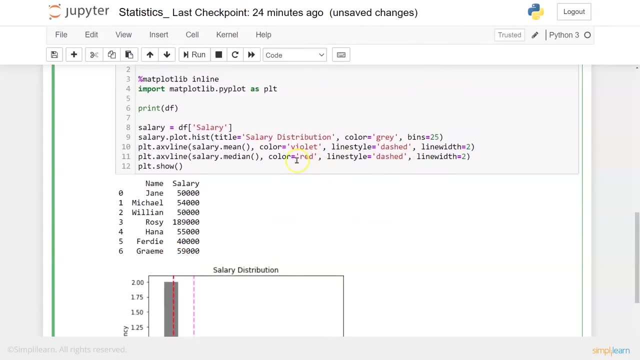 And we'll look at the salary distribution. And just look at this: the way the salary is distributed. You have our. in this case we did. let's see. we had red for the median, We have violet for our average or mean. 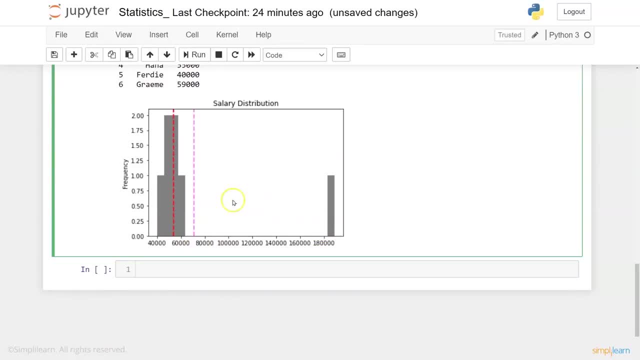 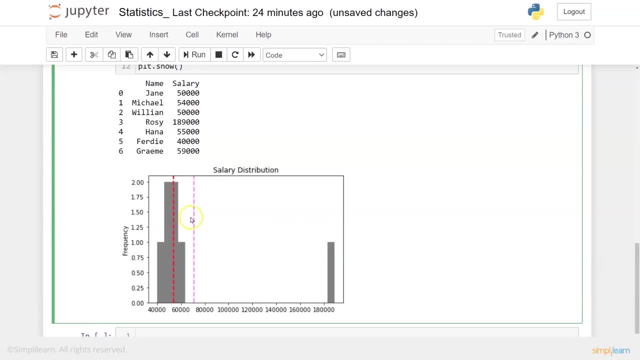 And you can just see how it really. here's our outlier, Here's our person who makes a lot of money. Here's the average And here's the median, And so, as you look at this, you can say, wow, based on the average. 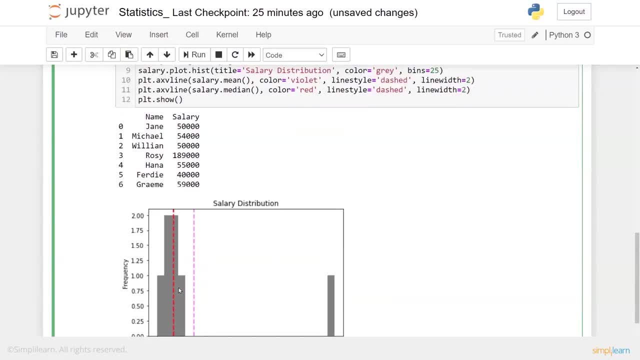 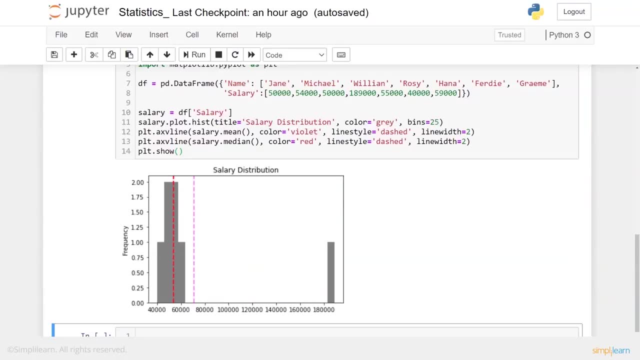 it really doesn't tell you much about what people are really taking home. All it does is tell you how much money is in this, what the average salary is. So some of the things you want to take away in addition to this is that it's very easy. 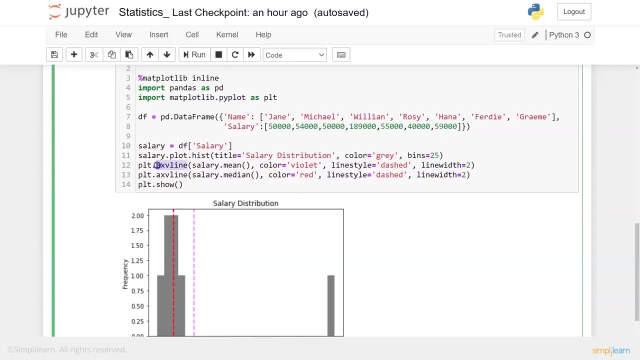 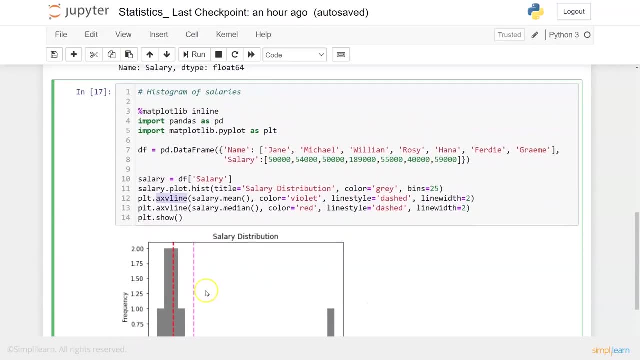 to plot an AXV line. These are these up and down lines for your markers And as you display the data, I mean you can add all kinds of things to this and get really complicated. Keeping it simple is pretty straightforward. I look at this and I can see. 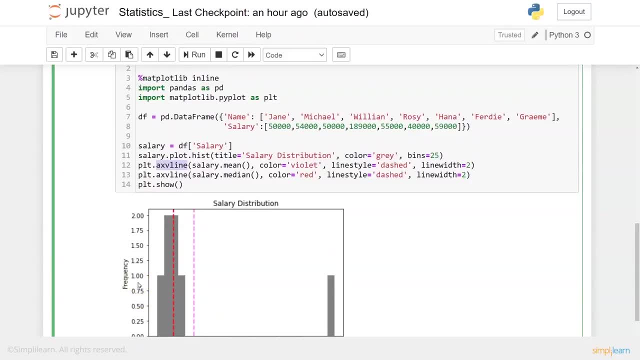 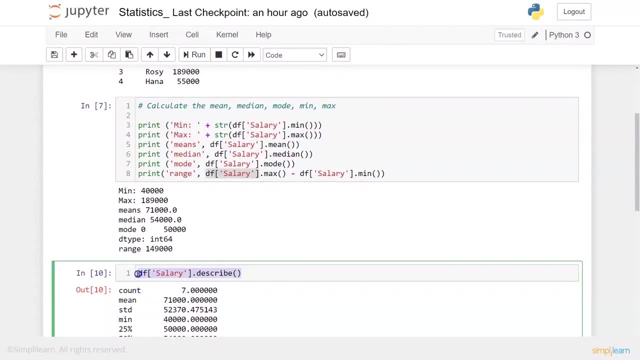 we have a major outlier out here. We can definitely do a histogram and stuff like that, But you know a picture's worth a thousand words. What you really want to make sure you take away is that we can do a basic describe. 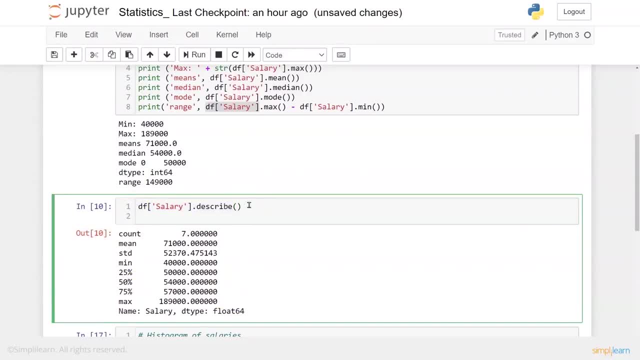 which pulls all this information out, and we can print any of the individual information from the describe, because this is a dictionary And so if we want to go ahead and look up the mean value, we can also do describe mean. So if you're doing a lot, 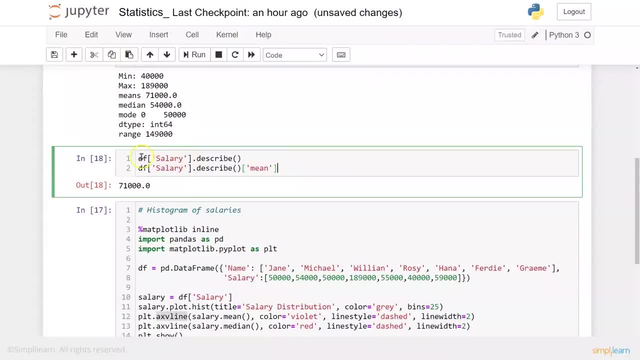 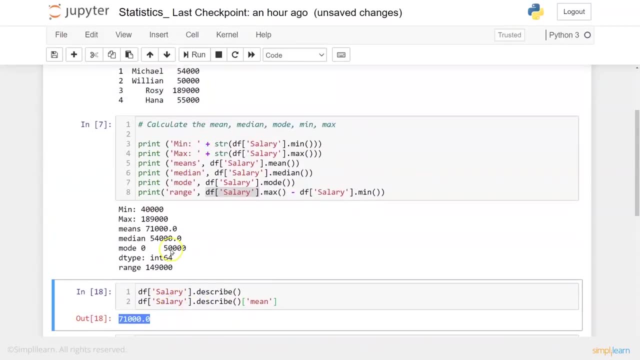 of statistics being able to. it doesn't have the print on there, so it's only going to print the last one, which happens to be the mean. You can very easily reference any one of these, And then you can also if you're doing something. 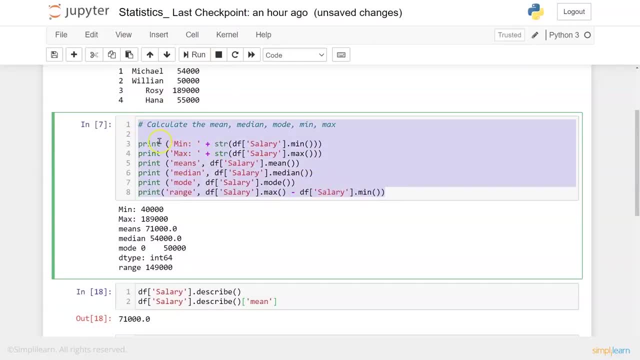 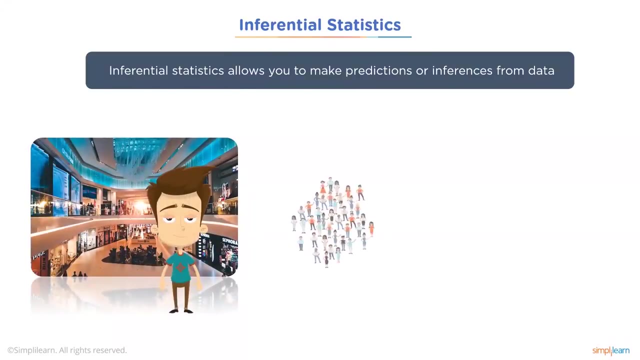 a little bit more complicated and you don't need just the basics. you can come through and pull any one of the individual references from the pandas on here. So now we've had a chance to describe our data. Let's get into inferential statistics. 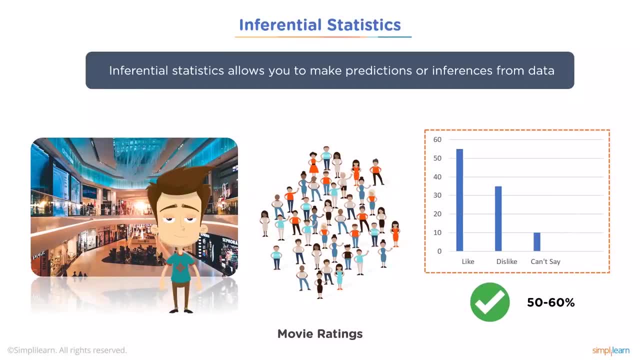 Inferential statistics allows you to make predictions or inferences from data And you can see, here we have a nice little picture, movie ratings. and if we took this group of people and said, hey, how many people like the movie, dislike it, can't say. 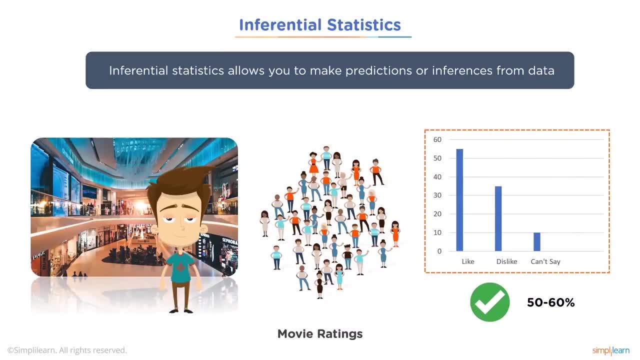 and then you ask just a random person who comes out of the movie who hasn't been in this study you can infer 55% chance of saying liked, 35% chance of saying disliked, or 10 or 11% chance of can't say. 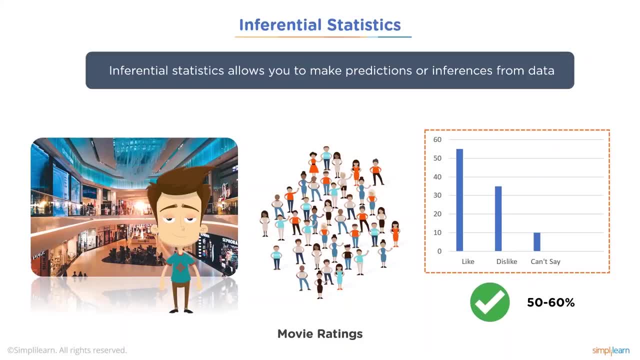 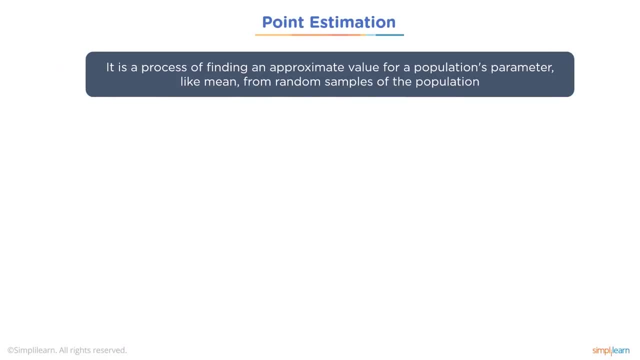 So that's real basics of what we're talking about- is you're going to infer that the next person is going to follow these statistics. So let's look at point estimation. It is a process of finding an approximate value for a population's parameter. 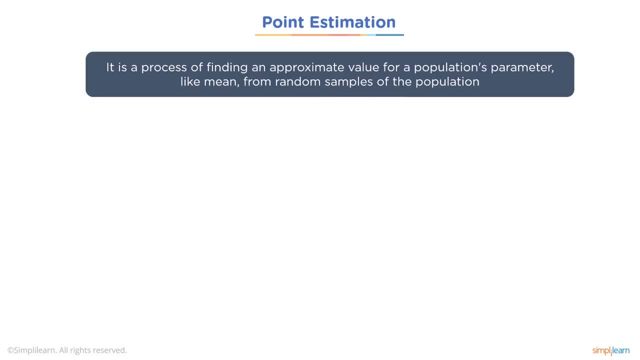 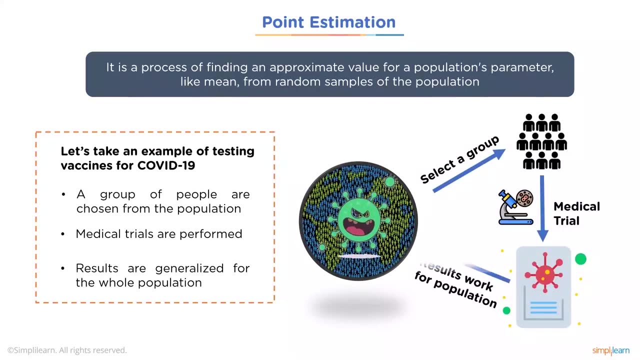 like mean or average from random samples of the population. Let's take an example of testing vaccines for COVID-19.. Vaccines and flu bugs, all of that. it's a pretty big thing of how do you test these out and make sure they're going. 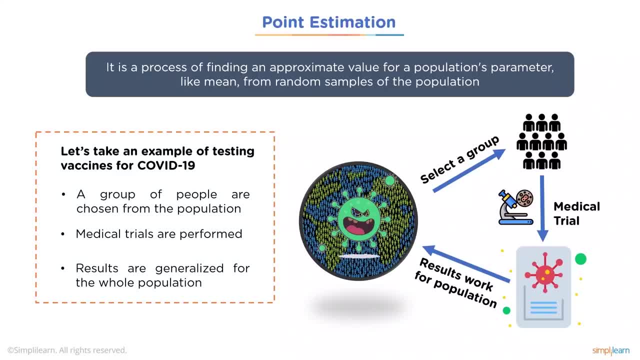 to work on the populace. A group of people are chosen from the population, Medical trials are performed, Results are generalized for the whole population. So here's our small group up here, where we've selected them, We run medical trials on them and then the results. 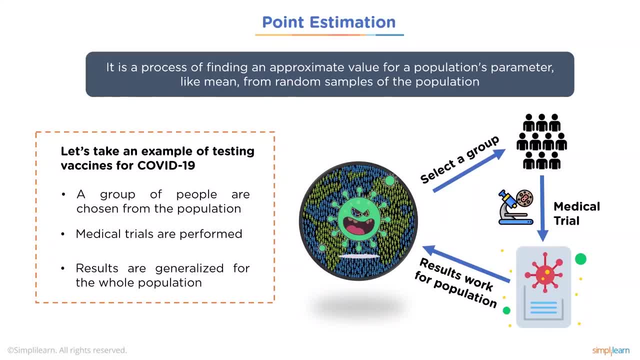 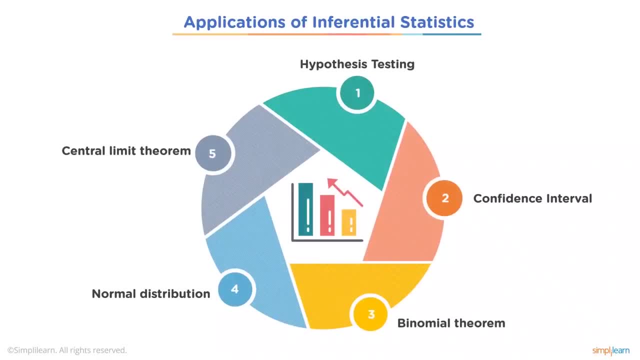 work for the population. Nice diagram with the arrows going back and forth and the very scary COVID virus in the middle of one. And let's take a look at the applications of inferential statistics. Very central is what they call hypotheses testing and the confidence interval. 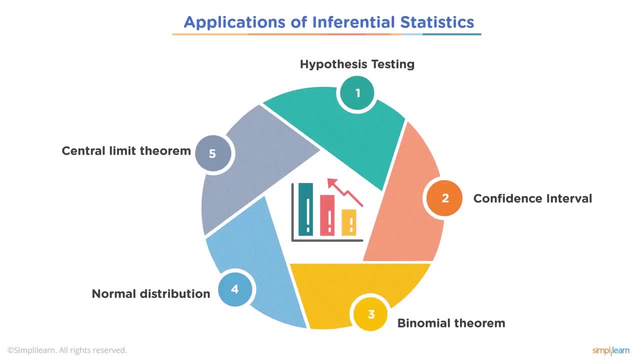 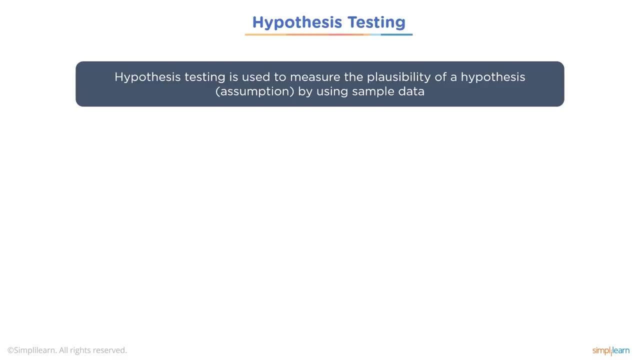 which go with that. And then, as we get into probability, we get into our binomial theorem, our normal distribution and central limit theorem. Hypothesis testing: Hypothesis testing is used to measure the plausible possibility of a hypothesis Assumption by using sample data. 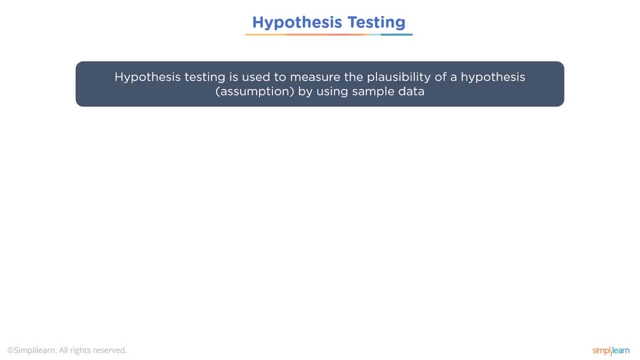 Now, when we talk about theorems, theory, hypothesis, keep in mind that if you are in a philosophy class, theory is the same as hypothesis, where theorem is a scientific statement. that is something that has been proven, although it is always up for debate. 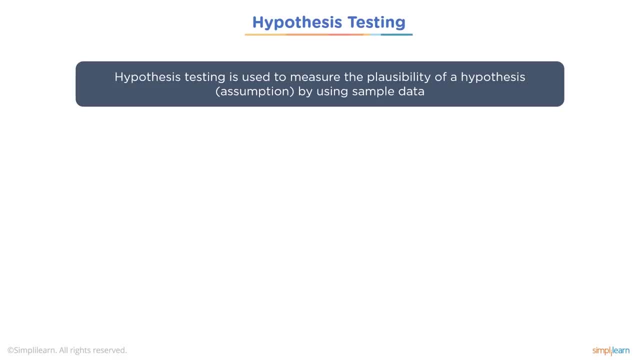 because in science we always want to make sure things are up to debate. So hypothesis is the same as a philosophical class calling a theory where theory in science is not the same. Theory in science says this has been well proven: Gravity is a theory. 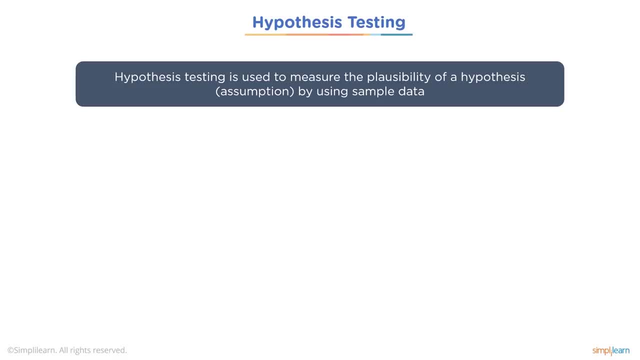 So if you want to debate the theory of gravity, try jumping up and down. If you want to have a theory about why the economy is collapsing in your area, that is a philosophical debate Very important. I've heard people mix those up and it is a pet peeve of mine. 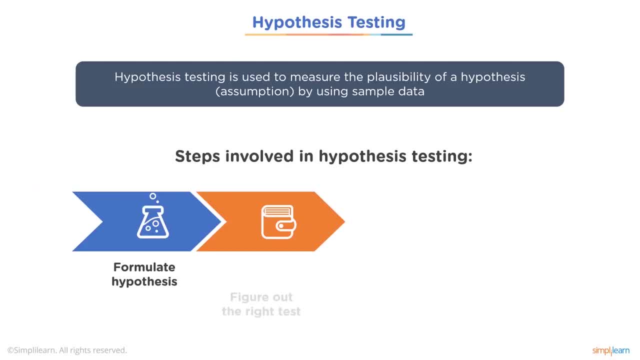 When we talk about hypothesis testing. the steps involved in hypothesis testing is: first we formulate a hypothesis, We figure out the right test to test our hypothesis, We execute the test and we make a decision. And so when you're talking about hypothesis, you're usually trying to disprove it. 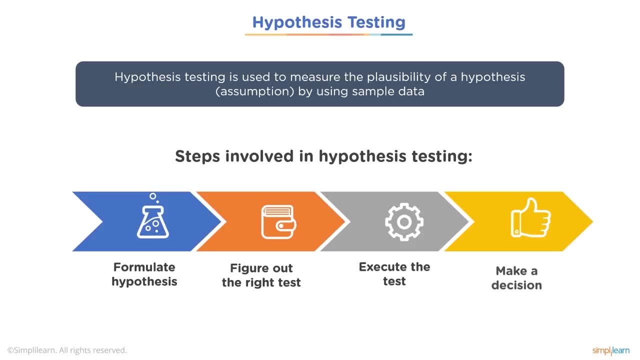 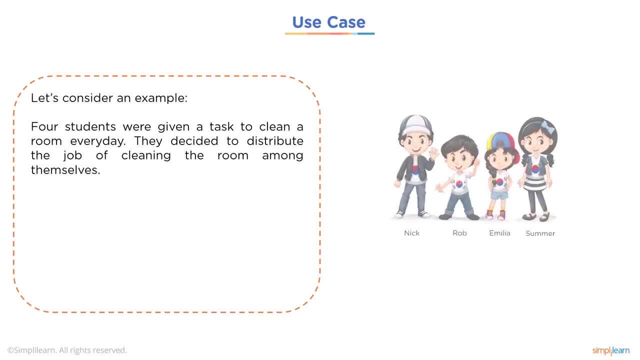 If you can't disprove it and it works for all the facts, then you might call that a theorem at some point. So in a use case, let's consider an example. We have four students who are given a task to clean a room every day. 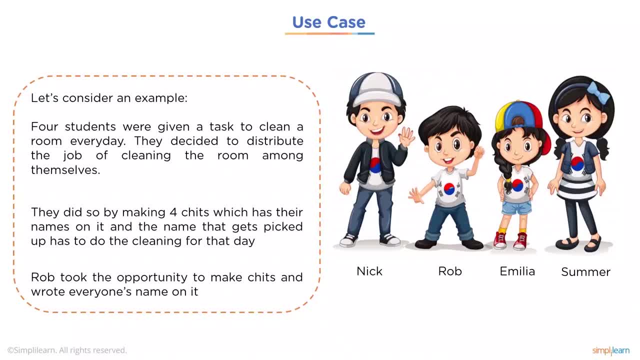 Sounds like working with my kids. They decided to distribute the job of cleaning the room among themselves. They did so by making four chits, which has their names on it, and the name that gets picked up has to do the cleaning. for that day, Rob took the opportunity. 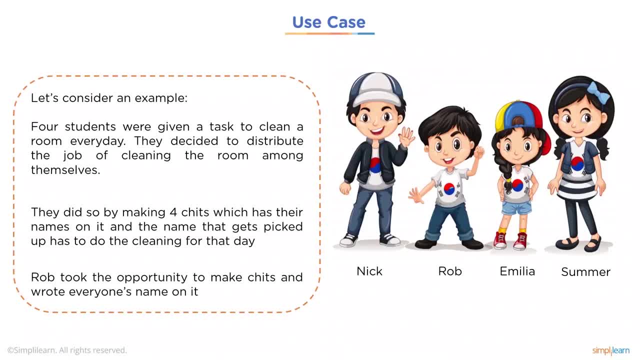 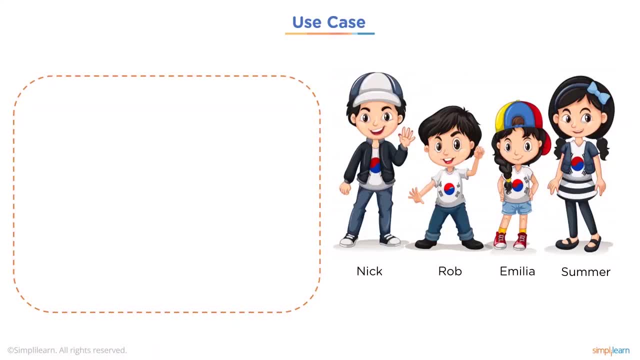 to make chits and wrote everyone's name on it. So here's our four people: Nick, Rob, Imlia and Summer. Now Rick, Imlia and Summer are asking us to decide whether Rob has done some mischief in preparing the chits. 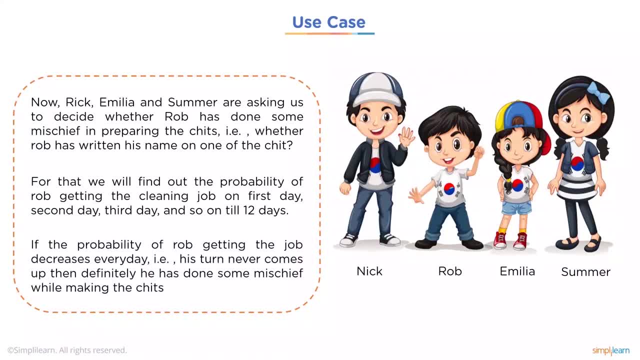 ie whether Rob has written his name on one of the chit. For that we will find out the probability of Rob getting the cleaning job on first day, second day, third day and so on till 12 days. The probability of Rob getting the job. 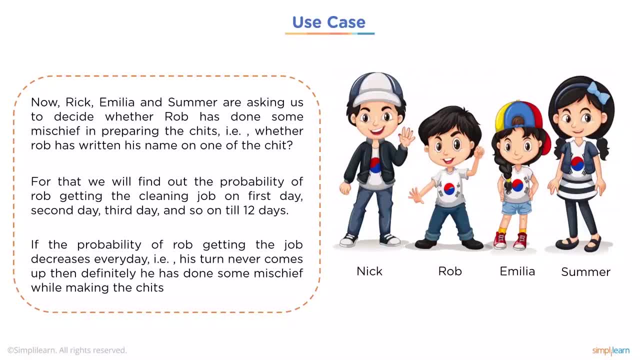 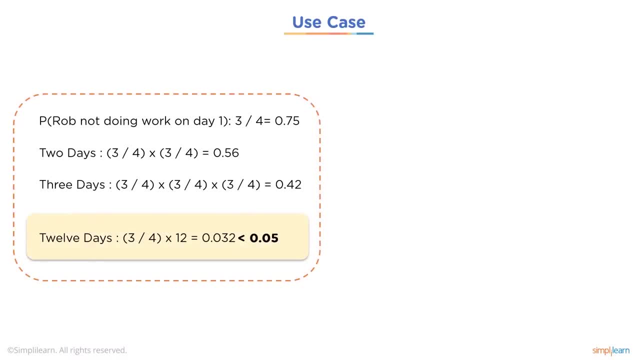 decreases every day, ie his turn never comes up, then definitely he has done some mischief while making the chits. So the probability of Rob not doing work on day one is three out of four. There's a .75 chance that he did it. 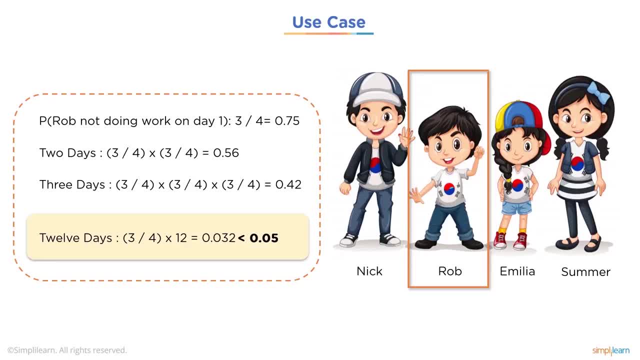 He didn't do work. Two days, 3 fourths times 3 fourths equals .56.. Three days, you have 3 fourths, 3 fourths, 3 fourths, which equals .42.. When you get to day 12,, 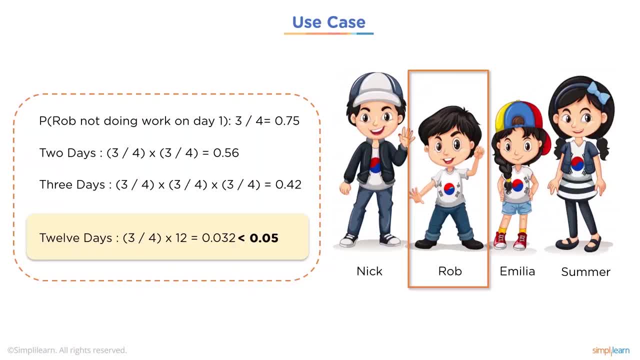 it's .032,, which is less than .05.. Remember this .05.. That comes up a lot when we're talking about certain values, when we're looking at statistics. Rob is cheating, as he wasn't chosen for 12 consecutive days. 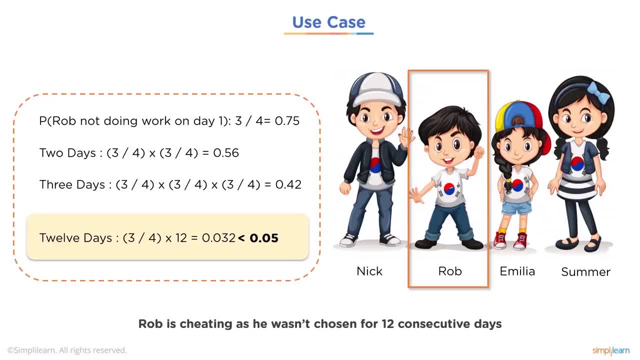 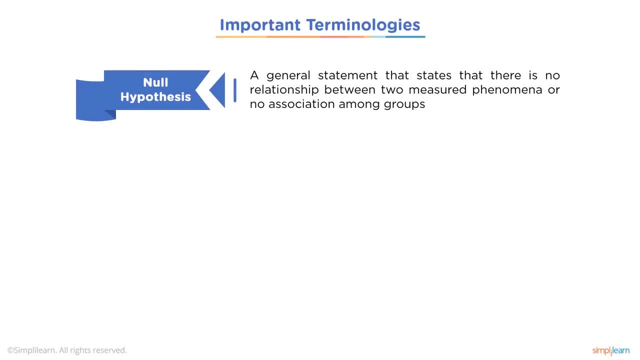 That's a very high probability when on day 12 he still hasn't gotten the job cleaning the room. So we come up to our important, important terminologies. We have null hypothesis, a general statement that states that there is no relationship between two measured phenomenon. 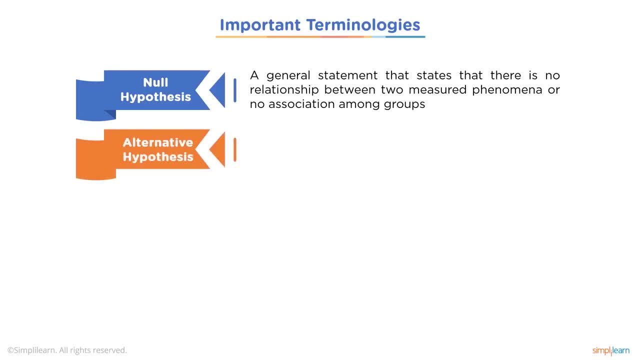 or no association among the groups. Alternative hypothesis: Contrary to the null hypothesis, it states: whenever something is happening, a new theory is preferred instead of an old one, And so the two hypotheses go hand in hand. So your null, and this is always interesting. 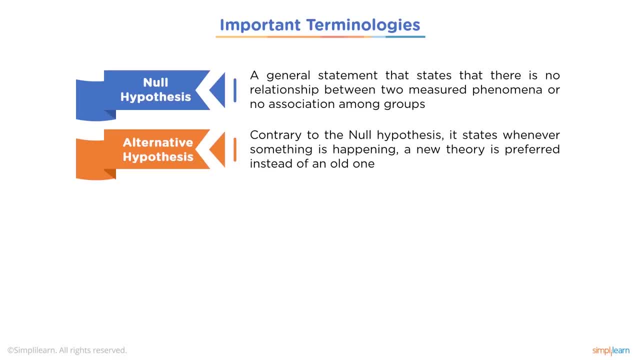 when talking about data science and the math behind it, it's about proving that the things have no correlation. Null hypothesis says these two have zero relation to each other, Where the alternative hypothesis says: hey, we found a relation. this is what it is. 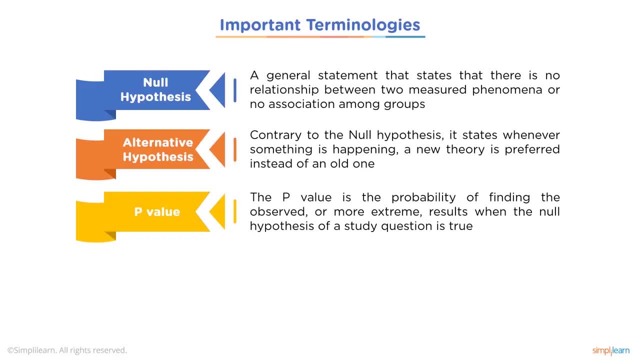 We have p-value. The p-value is the probability of finding the observed or more extreme results when the null hypothesis of a study question is true, And the t-value: it is simply the calculated difference represented in units of standard error. The greater the magnitude of t. 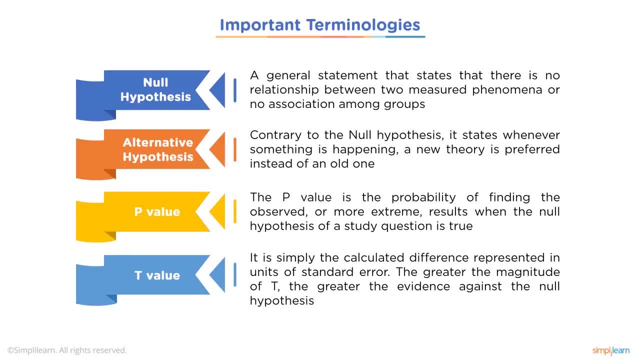 the greater the evidence against the null hypothesis And you can look at the t-value as being specific to the test you're doing, where the p-value is derived from your t-value and you're looking for what they call the 5% or the .05,. 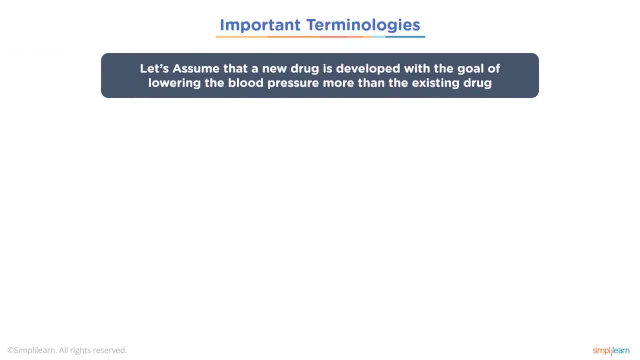 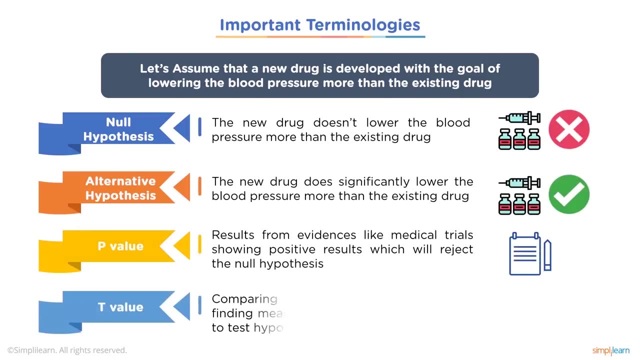 showing that it has a high correlation. So, digging in deeper, let's assume that a new drug is developed with the goal of lowering the blood pressure more than the existing drug, And this is a good one, because the null value here isn't that you don't have any drug. 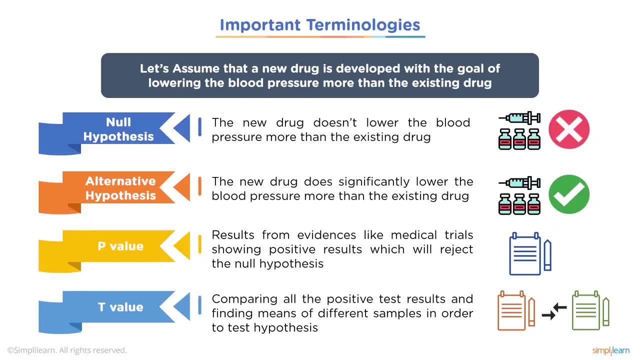 the null value here is that it's better than the existing drug. The new drug doesn't lower the blood pressure more than the existing drug. Now if we get that, that says our null hypothesis is correct. there is no correlation and the new drug. 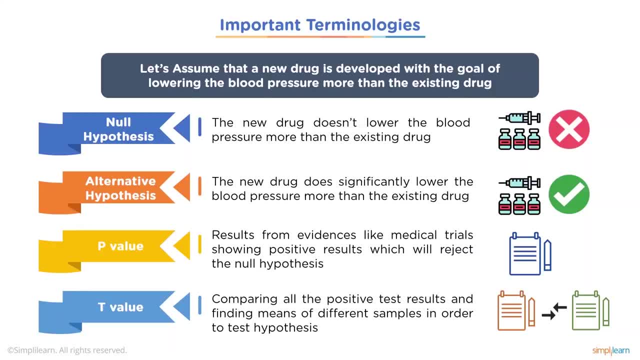 is not doing its job. The alternative hypothesis: the new drug does significantly lower the blood pressure more than the existing drug. Yay, we got a new drug out there and that's our alternative hypothesis, or the H1 or HA, And we look at the p-value. 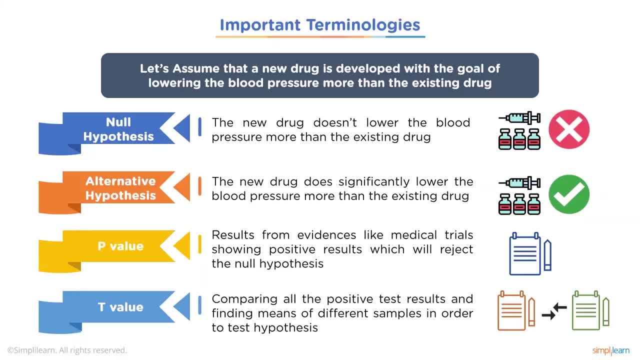 results from the evidence, like medical trials showing positive results which will reject the null hypothesis. And again they're looking for a .05 or 5% And the t-value, comparing all the positive test results and finding means of differentiation of different samples in order to test hypothesis. 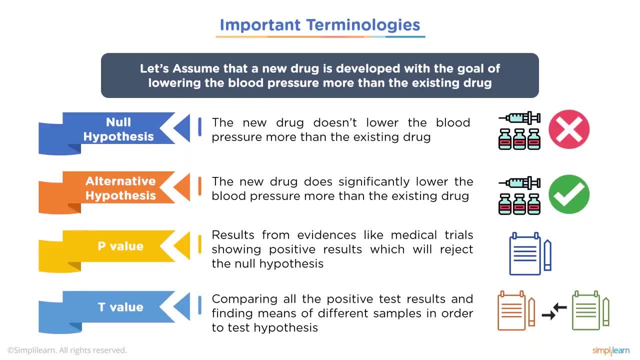 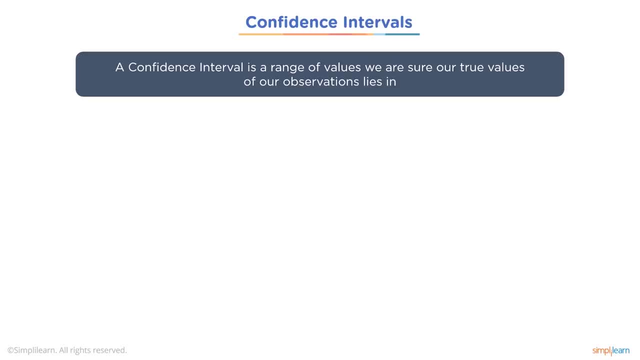 So this is specific to the test: How, what percentage of increase did they have? And this leads us to the confidence intervals. A confidence interval is a range of values we are sure are true. values of observations lie in, Let's say, you asked. 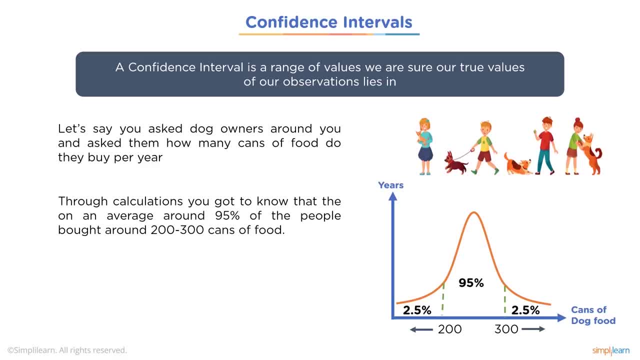 a dog owner around you and asked them: how many cans of food do you buy for your per year for your dog? Through calculations, you got to know that the, on an average, around 95% of the people bought around 200. 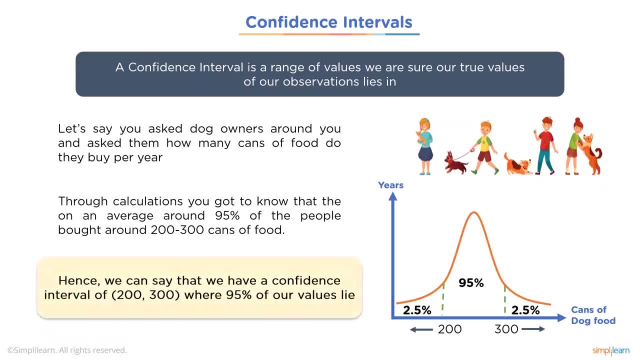 to 300 cans of food. Hence we can say that we have a confidence interval of 2,300, where 95% of our values lie in that data spread, And this, the graph, really helps a lot. So you can start seeing. 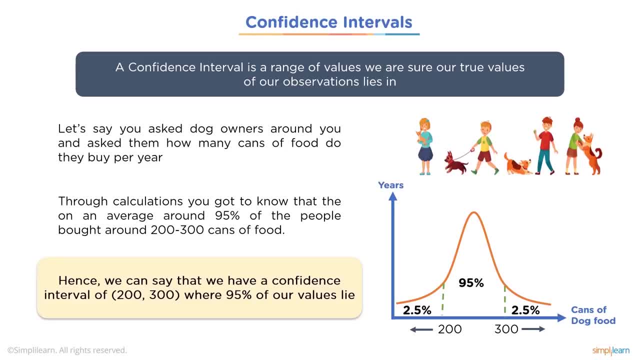 what you're looking at here. where you have the 95%, You have your peak. In this case it's a normal distribution, so you have the nice bell curve, equal on both sides. It's not asymmetrical And 95% of all the values lie. 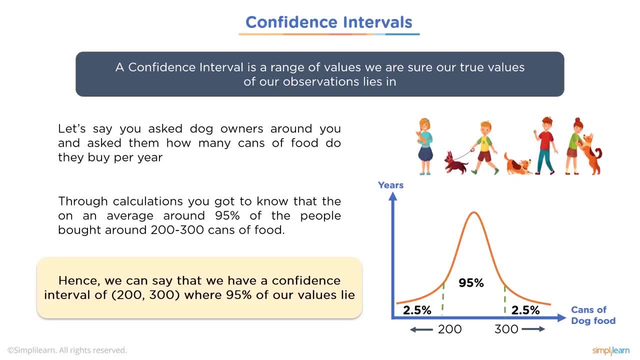 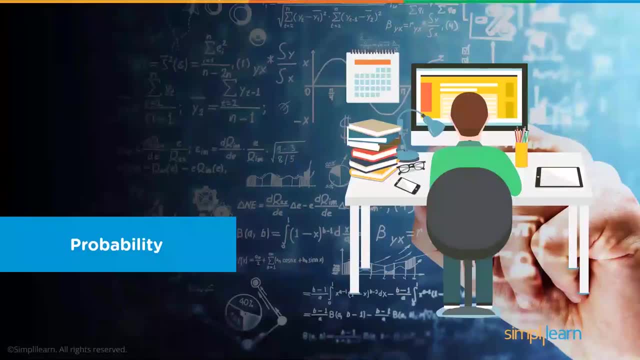 within a very small range. And then you have your outliers, the 2.5% going each way. So we touched upon hypothesis. We're going to move into probability. So you have your hypothesis. Once you've generated your hypothesis, we want to know the probability. 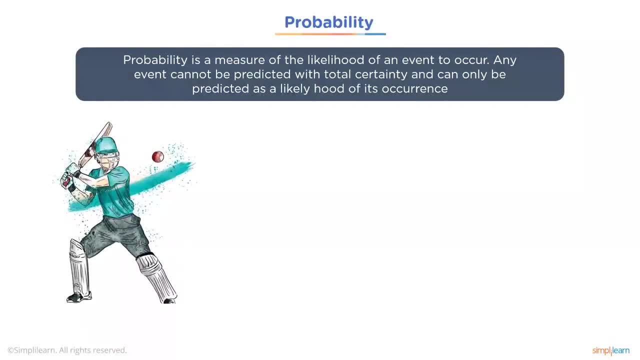 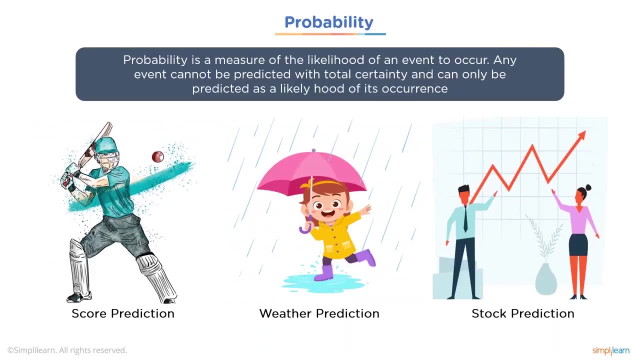 of something occurring. Probability is a measure of the likelihood of an event to occur. Any event can be predicted with total certainty and can only be predicted as a likelihood of its occurrence. So any event cannot be predicted with total certainty and can only be predicted. 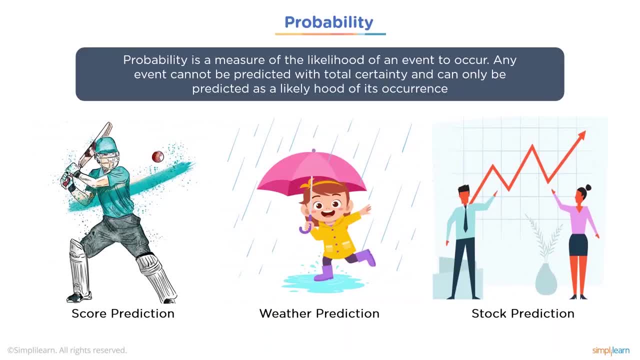 as a likelihood of its occurrence: Score prediction, how good you're going to do in whatever sport you're in, weather prediction, stock prediction. If you've studied physics and chaos theory, even the location of the chair you're sitting on has a probability. 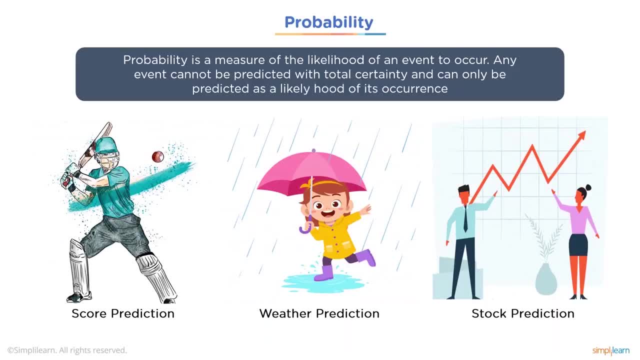 that it might move three feet over. Granted, that probability is one in like I think we calculated it as under one in trillions upon trillions. So the better the probability, the more likely it's going to happen. Some things have such a low probability. 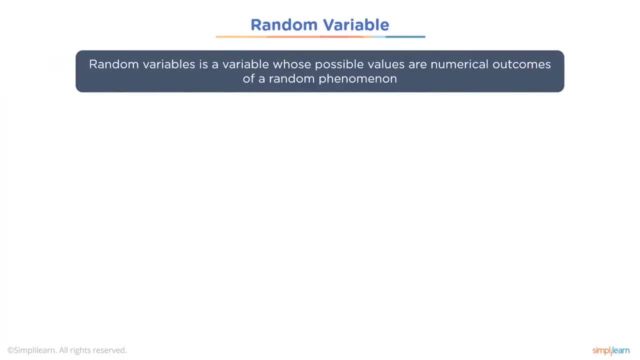 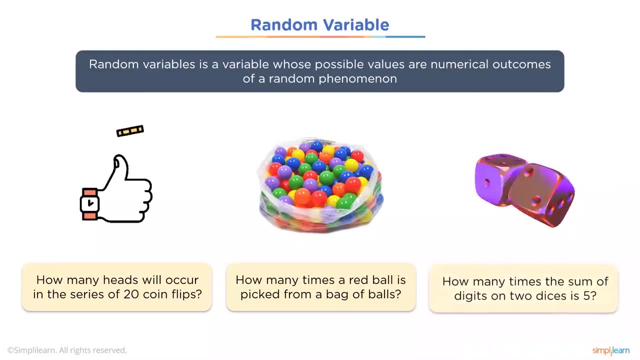 that we don't see them. So we talk about a random variable. A random variable is a variable whose possible values are numerical outcomes of a random phenomena. So we have the coin toss: How many heads will occur in the series of 20 coin flips? 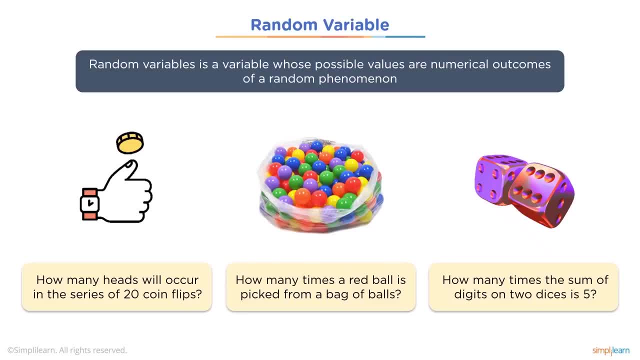 Probably. you know on average there are 10, but you really can't know, because it's very random, How many times a red ball is picked from a bag of balls If there's equal number of red balls and blue balls and green balls in there. 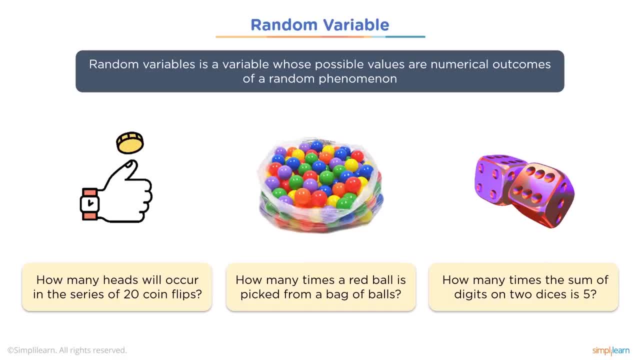 How many times is the sum of digits on two dice result, or five each. So you know how often are you going to roll two fives on your pair of dice. So in a use case, let's consider the example of rolling two dice. 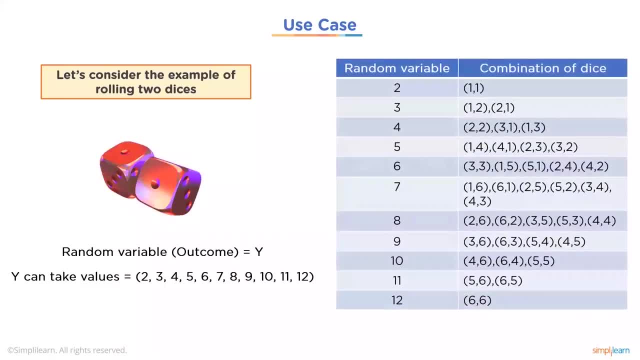 We have a random variable, outcome equals y. You can take values two, three, four, five, six, seven, eight, nine, 10,, 11,, 12.. So we have a random variable and a combination of dice And instead of looking 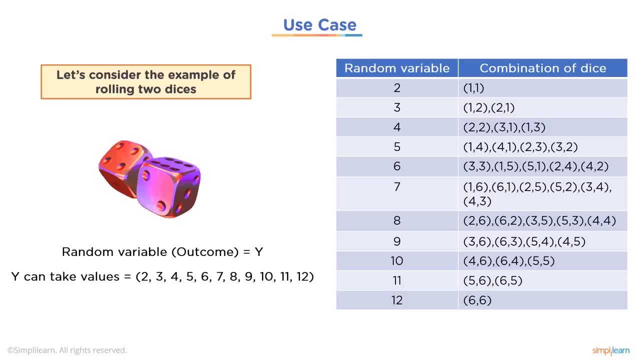 at how many times both dice will roll five. let's go ahead and look at total sum of five And you have, as far as your random variables. you can have a one. four equals five, four, one, two, three. 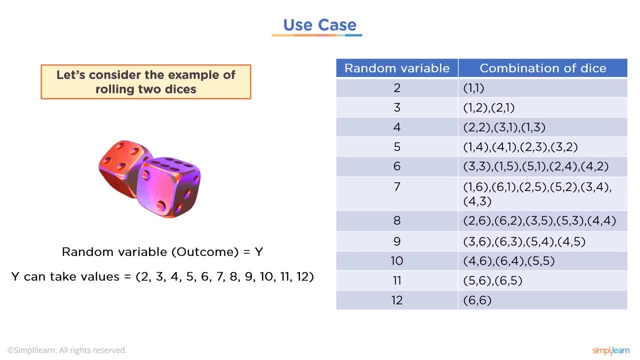 three, two, So four of those rolls can be. if you look at all the different options, you have four of those random rolls can be a five, And if we look at the total number, which happens to be 36 different options. 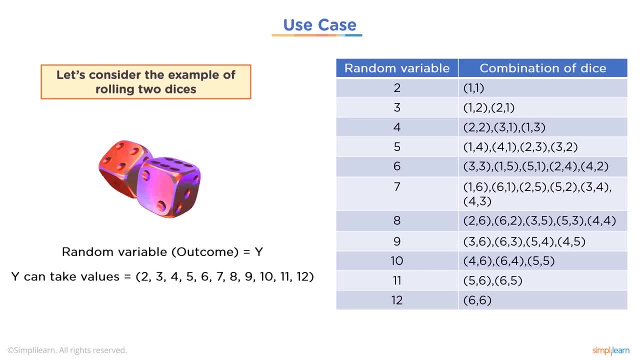 you can see that we have four out of 36 chance. every time you roll the dice, that you're going to roll a total of five, You're going to have an outcome of five, And we'll look a little deeper as to what that means. 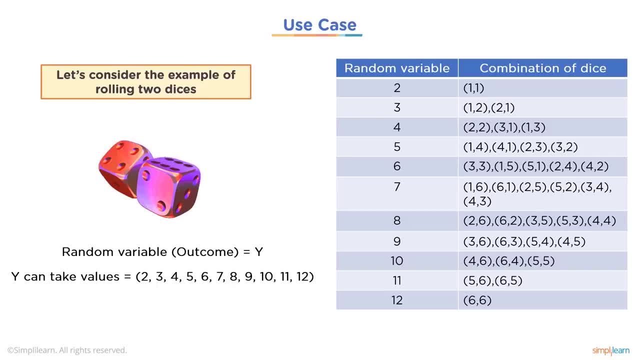 But you could think of that. at what point, if someone never rolls a five, or they always roll a five, can you say, hey, that person's probably cheating. We'll look a little closer at the math behind that, But let's just consider. 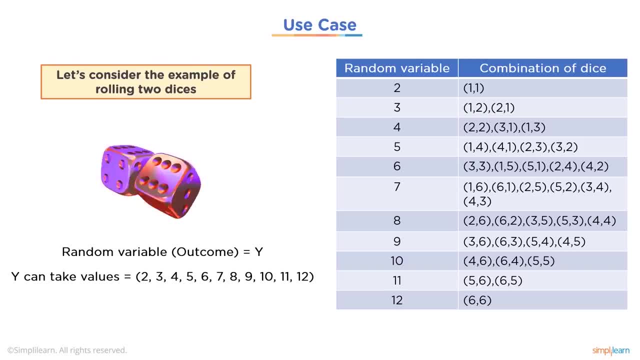 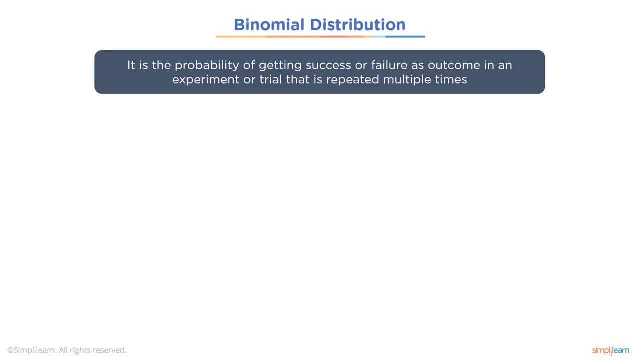 this is one of the cases is rolling two dice and gambling. There's also a binomial distribution. It is the probability of getting success or failure as an outcome in an experiment or trial. that is repeated multiple times And the key is is by meaning. 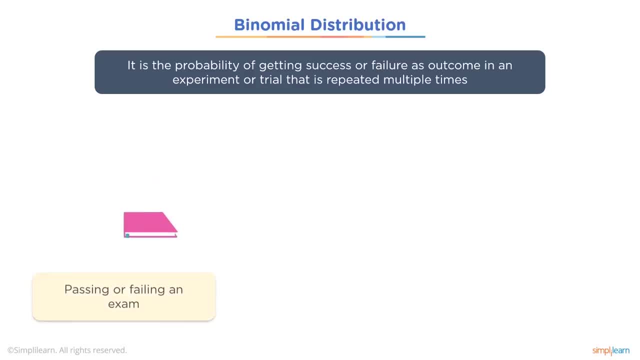 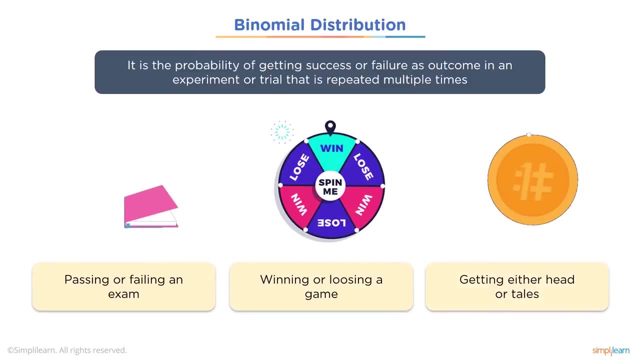 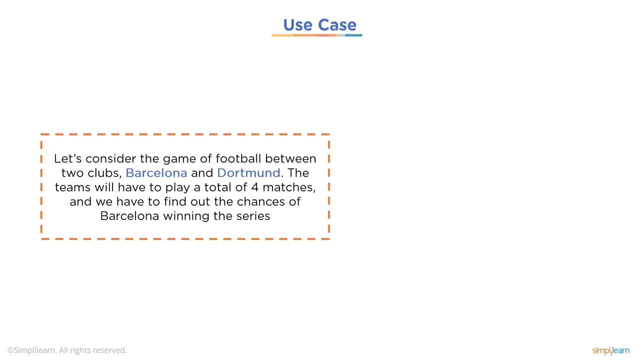 two binomial, So passing or failing an exam, winning or losing a game, getting either head or tails. So if you ever see binomial distribution, it's based on a true, false kind of setup: You win or lose. Let's consider a use case. 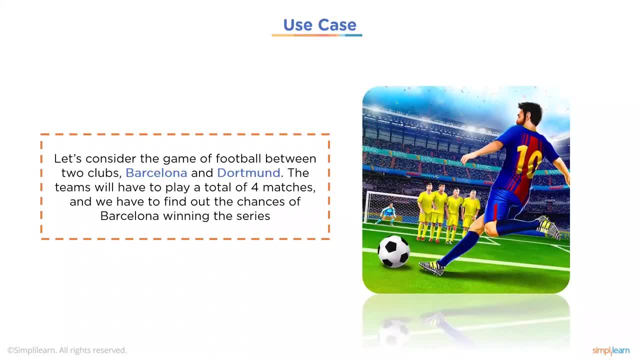 And let's consider the game of football between two clubs, Barcelona and Dortmund. The teams will have to play a total of four matches And we have to find out the chances of Barcelona winning the series. So we look at the total games and we're looking at 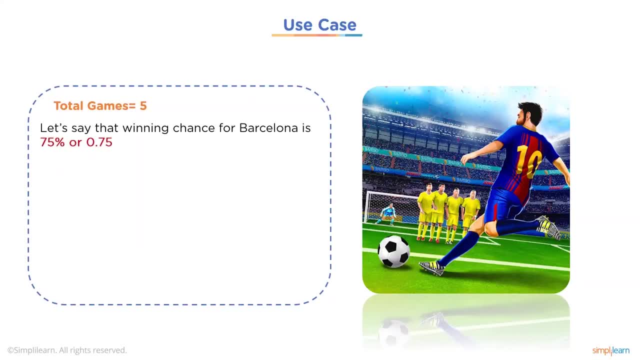 five different games or matches. Let's say that the winning chance for Barcelona is 75% or 0.75.. That means that each game they have a 75% chance that they're going to win that game And losing chances are 25% or 0.25.. 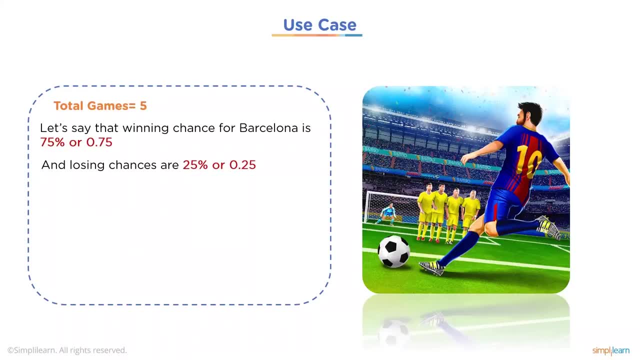 Clearly, 0.75 plus 0.25 equals one, So that accounts for 100% of the game. Probability for getting K wins in N matches is calculated And we're talking like so if you have five games and you want to know. 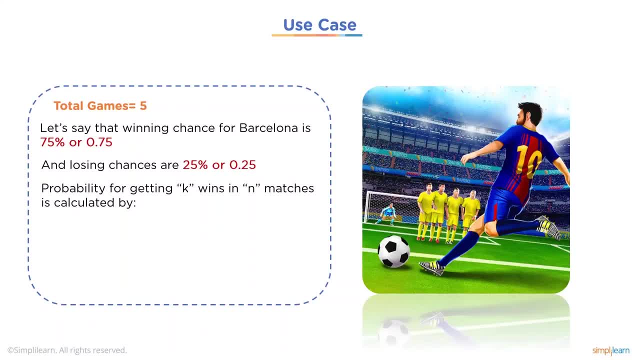 if I play how many wins in those five games should I get? What's the percentage on those? And the probability for getting K wins in N matches is calculated by: PX equals K equals NCK. P to the K, Q to the N minus K. 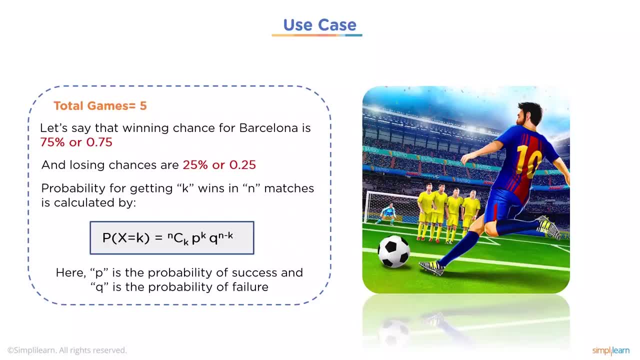 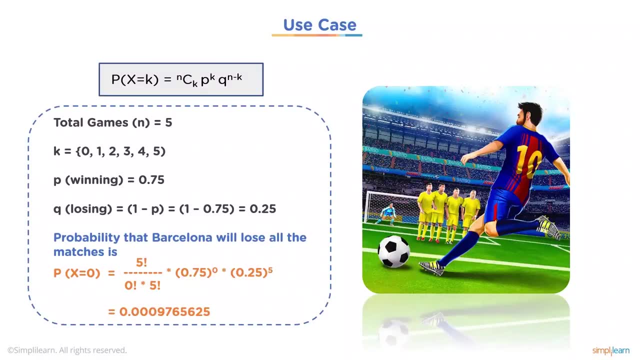 Here P is a probability of success and Q is a probability of failure, And so we can do total games. of N equals five, where K equals 0,, 1,, 2,, 3,, 4,, 5.. P, which is the chance of winning. 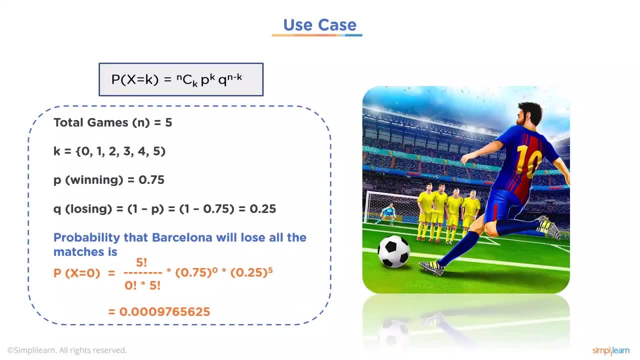 is 0.75.. Q- the chance of losing- equals one minus P, which equals one minus 0.075, which equals 0.25.. The probability that Barcelona will lose all of the matches can then just plug in the numbers. 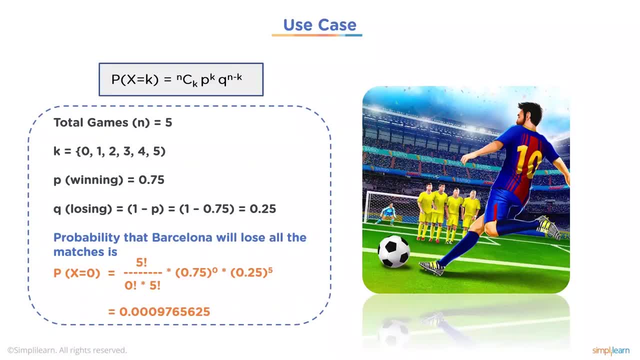 and we end up with a 0.000979.. 0.065625.. So a very small chance. they're going to lose all their matches And we can plug in the value for two matches: Probability that Barcelona will win at least two matches. 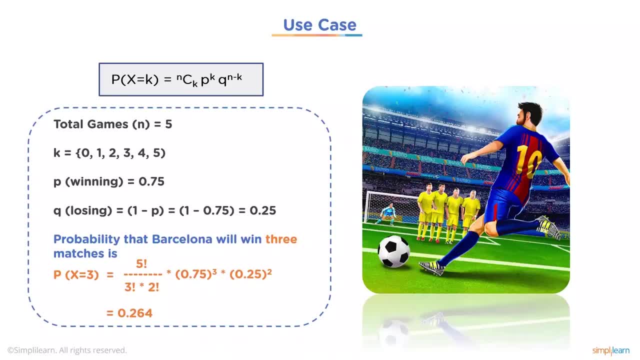 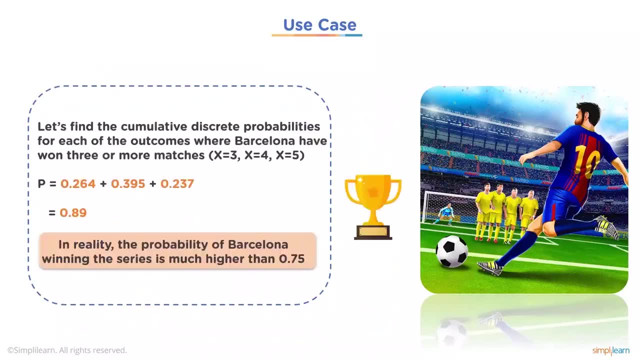 is 0.0878.. And of course, we can go on to the probability that Barcelona will win three matches- the 0.26, and, of course, four matches and so on, And it's always nice to take this information and let's find the cumulative. 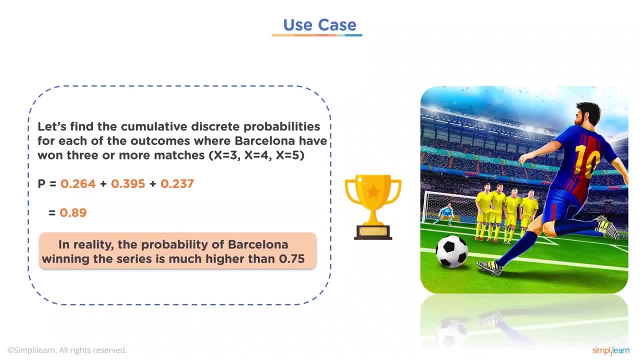 discrete probabilities for each of the outcomes Where Barcelona has won three or more matches: X equals three, X equals four, X equals five, And we end up with the P equals 0.264 plus 0.395 plus 0.237,. 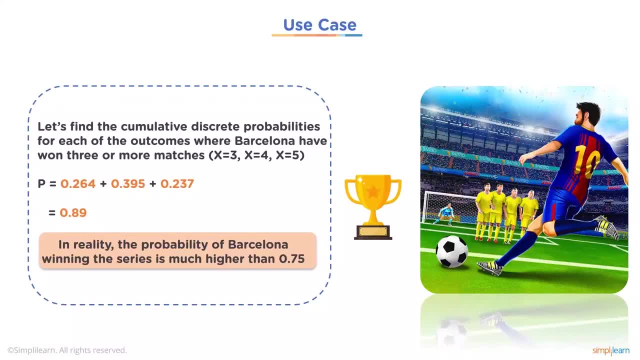 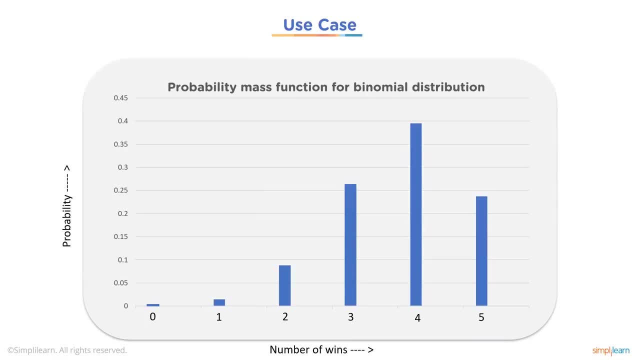 which equals 0.89.. In reality, the probability of Barcelona winning the series is much higher than 0.75.. And it's always nice to put out a nice graph so you can actually see the number of wins to the probability and how that pans out. 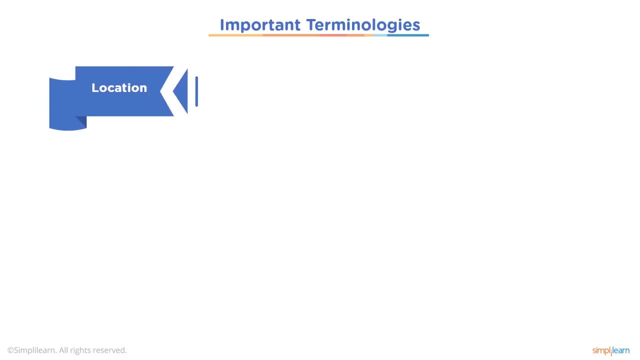 with our probability binomial case, Continuing in our important terminology location. The location of the center of the graph depends on the mean value, And this is some very important things. So much of the data we look at and when you start looking, 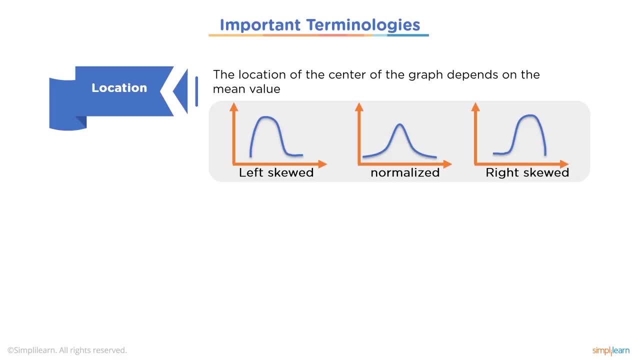 at probabilities almost always has a normalized look, like the graph in the middle. But you do have left skewed, where the data is skewed off to the left, and you have more stuff happening off to the left and you have right skewed data. 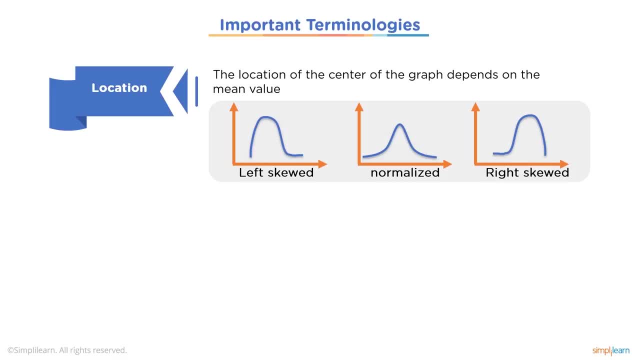 And so when this comes up and these probabilities come up where they're skewed, it's really important to take a closer look at that. Mostly, you end up with a normalized set of data, but you got to also be aware that sometimes it's a skewed data. 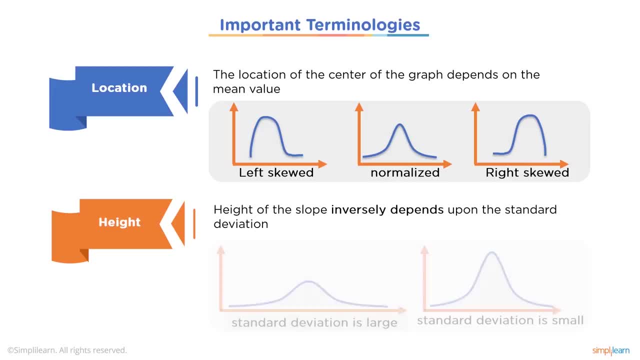 And then the height Height of the slope inversely depends upon the standard deviation. So you can see down here the standard deviation is really large, It kind of squishes it out. And if the standard deviation is small then most of your data 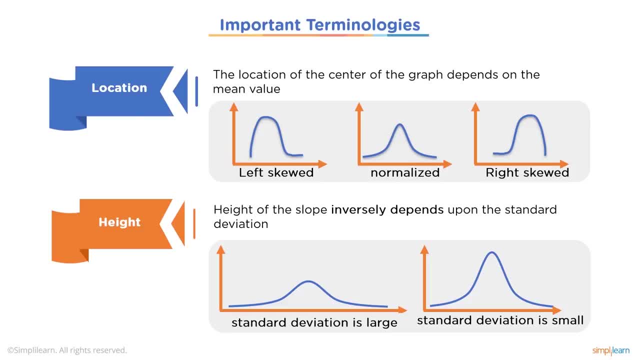 is going to hit right there in the middle. You're going to have a nice peak And so, being aware of this, that you might have a probability that fits certain data, but it has a lot of outliers, So if you have a really high, 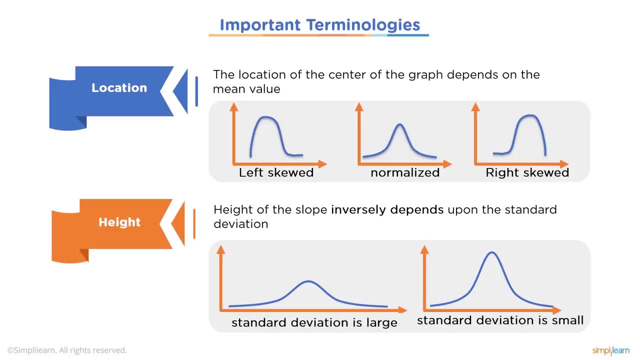 standard deviation. if you're doing stock market analysis, this means your predictions are probably not going to make you much money, Where, if you have a very small deviation, you might be right on target and set to become a millionaire. Which leads us to the Z-score. 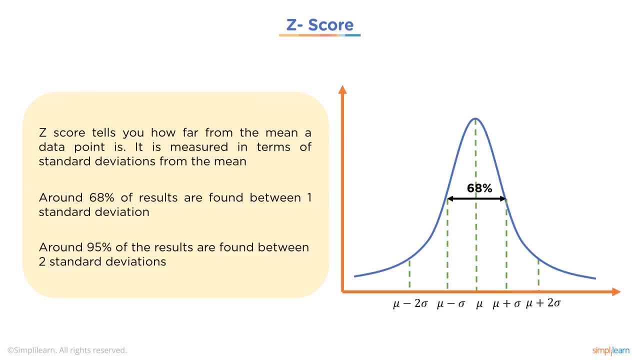 Z-score tells you how far from the mean a data point is. It is measured in terms of standard deviations from the mean. around the mean. around 68% of the results are found between one standard deviation. Around 95% of the results. 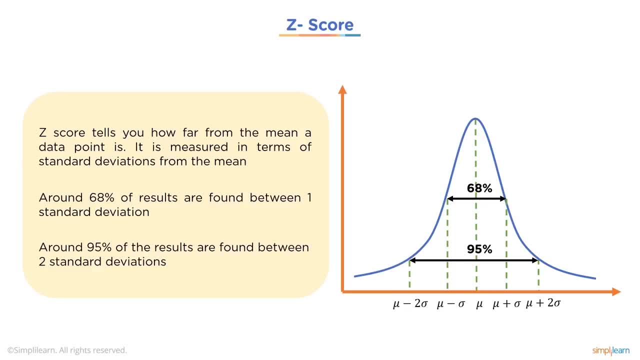 are found between two standard deviations And you read the symbols. Of course I love to throw some Greek letters in there. We have mu minus two. sigma Mu is just a quick way, it's a kind of funky U, It just means the mean. 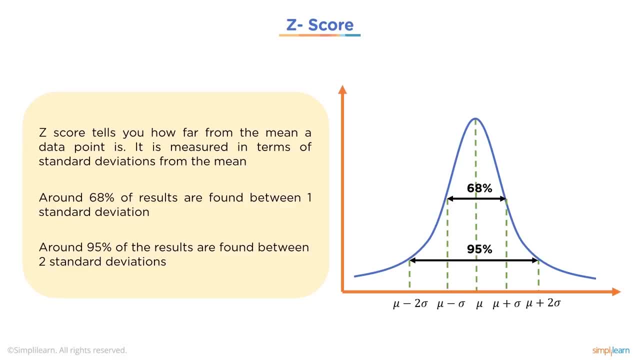 And then the sigma is the standard deviation, And that's the O, with the little arrow off to the right or the little waggly tail going up With a line on it. So mu minus two sigma is your 95% of the results. 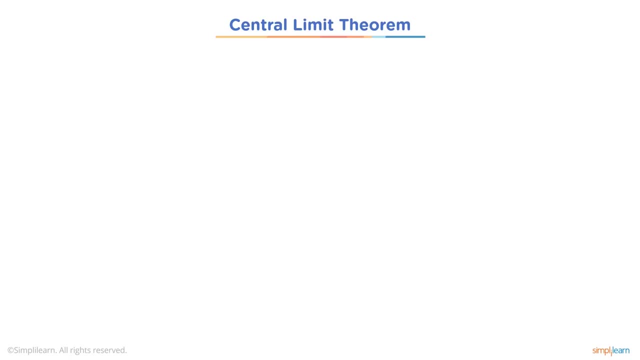 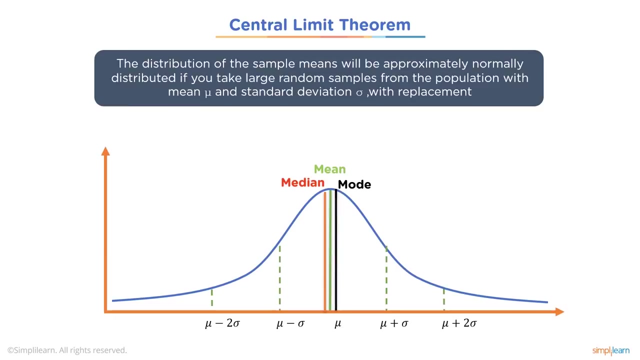 are found between two standard deviations: Central limit theorem. This goes back to the skew. If you remember, we were looking at the skew values on this previous slide. Have left skewed normalized and right skewed When we're talking about it being skewed or not skewed. 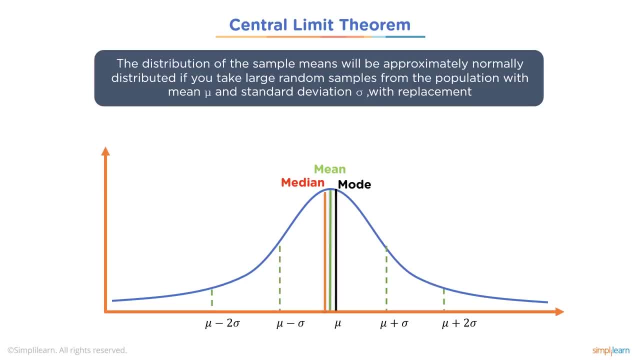 the distribution of the sample means will be approximately normally distributed, Evenly distributed, not skewed. If you take large random samples from the population with the mean mu and the standard deviation sigma with replacement, And you can see here: 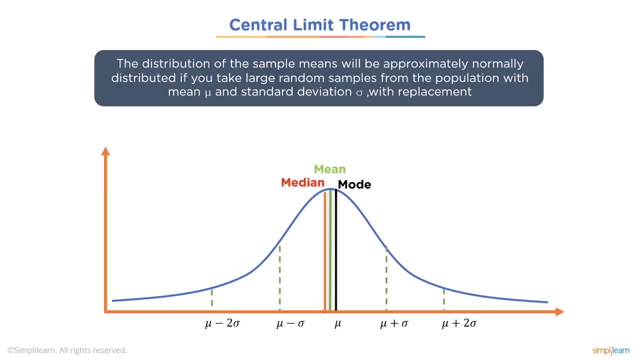 of course we have our mu minus two sigma and the spread down here, The mean, the median and the mode, And so when you're talking about very large populations, these numbers should come together and you shouldn't have a skewed value, If you do. 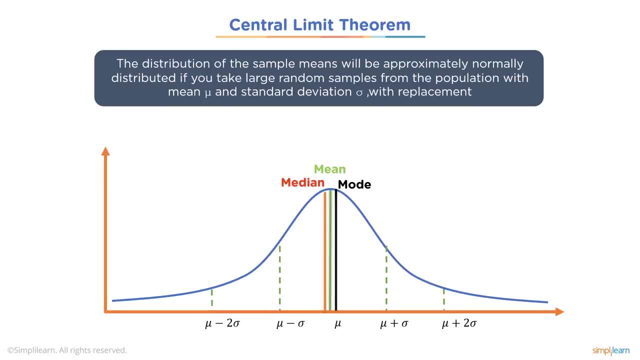 that's a flag that something's wrong. That's why this is so important: to be aware of what's going on with your data, where your samples are coming from and the math behind it. And if we're gonna do all this, we gotta jump into. 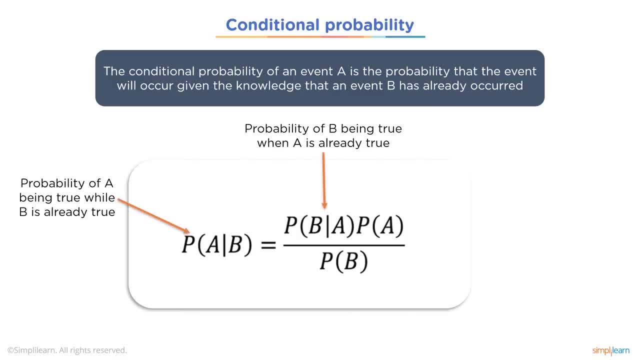 conditional probability. The conditional probability of an event A is the probability that the event will occur given the knowledge that an event B has already occurred, And you'll see this as Bayes' Theorem B-A-Y-E-S Bayes, And this is read: 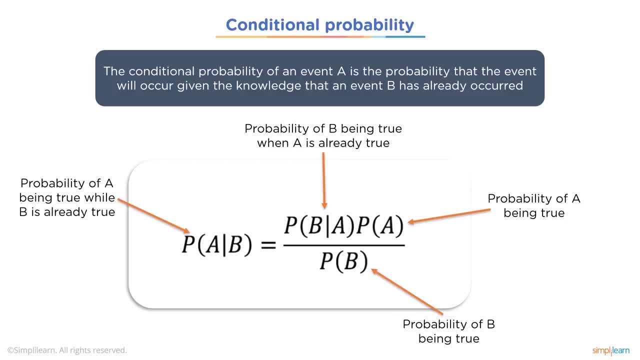 I mean, you have these funky looking little P brackets: A, B. This is the probability of A being true while B is already true, And you have the probability of B being true when A is already true. So P, B of A. 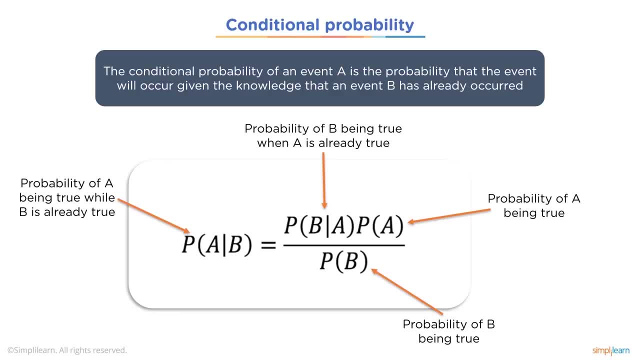 The probability of A being true divided by the probability of B being true. And we talk about Bayes' Theorem, which occurred back in the 1800s when he discovered this. This is such an important formula And it's really. 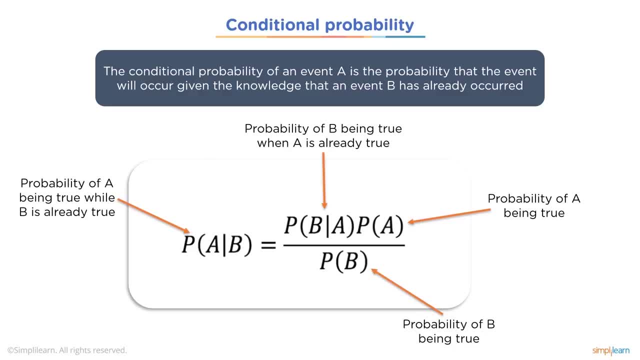 if you actually do the math, you could just kind of do X Y equals J, K, and then you divide them out and you're going to see the same math. But it works with probabilities, which makes it really nice, And so if you have a set, 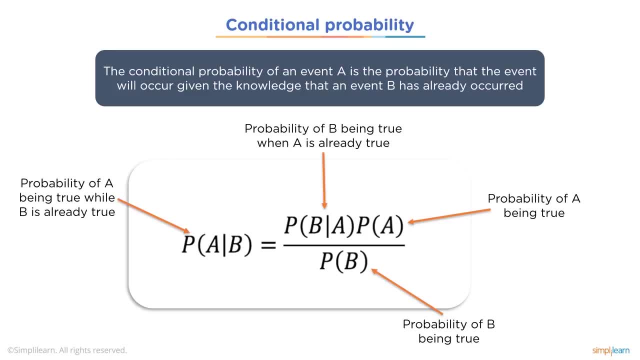 you might have eight or nine different studies going on in different areas. Different people have done the studies. They brought them together. If we look at today's COVID virus, the virus spread. certainly the studies done in China versus the studies the way they're done in the US. 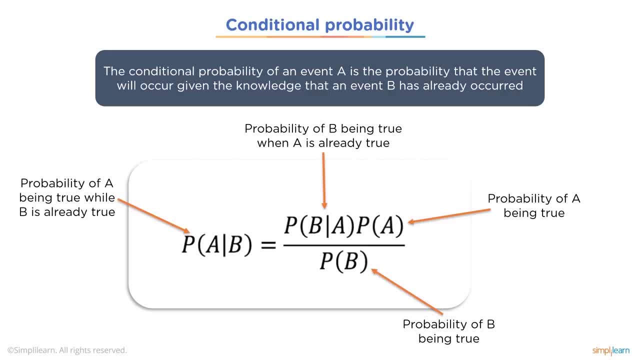 that data is different in each of those studies, But if you can find a place where it overlaps, where they're studying the same thing together, you can then compute the changes that you need to make in one study to make them equal. And this is also true. 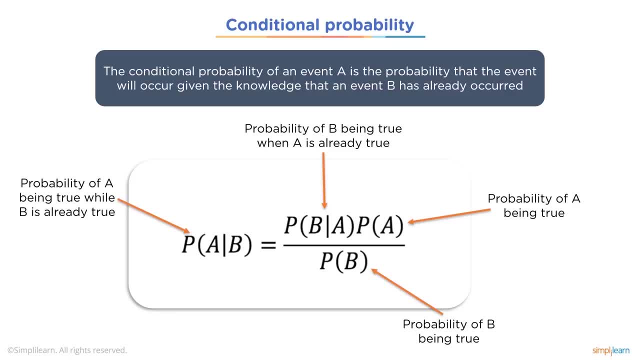 if you have a study of one group and you want to find out more about it. So this formula is very powerful And it really has to do with the data collection part of the math and data science And understanding where your data is coming from. 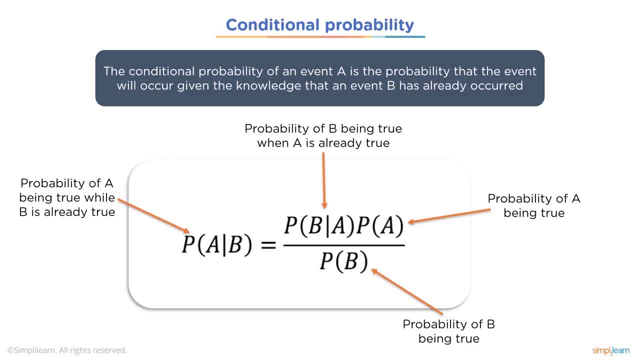 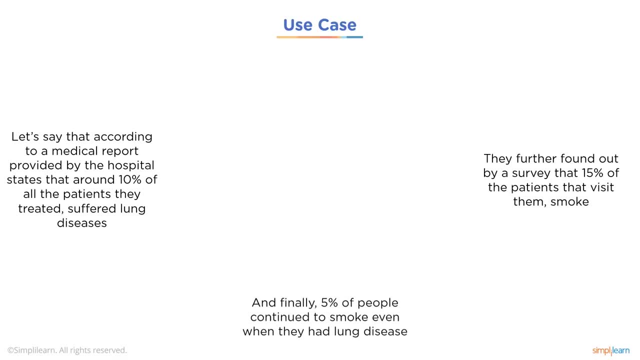 and how you're going to combine different studies in different groups And we'll go into a use case. Let's find out the chance of a person getting lung disease due to smoking, And this is kind of interesting the way they word this. Let's say that, according to medical report, 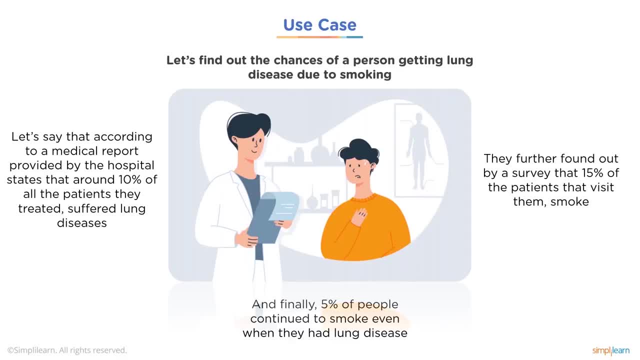 provided by the hospital states that around 10% of all patients they treated suffered lung disease, So we have kind of a generic medical report. They further found out by a survey that 15% of the patients that visit them smoke, So we have 10% that are lung disease. 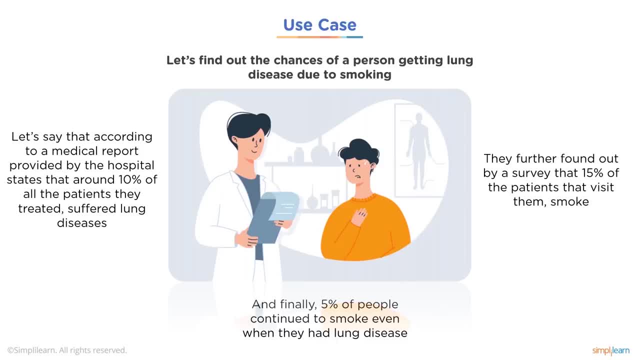 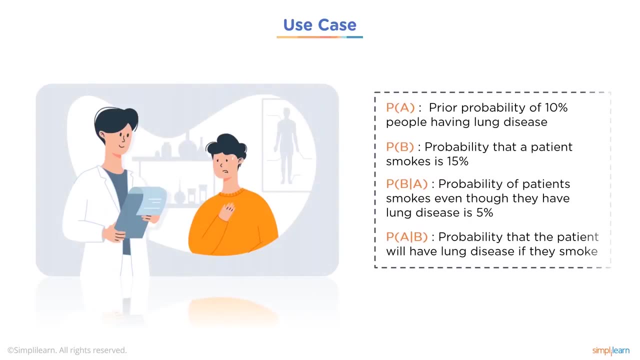 and 15% of the patients smoke. And finally, 5% of the people continued smoke even when they had lung disease. Not the brightest choice, but it is an addiction, so it can be really difficult to kick, And so we can look at the probability of A. 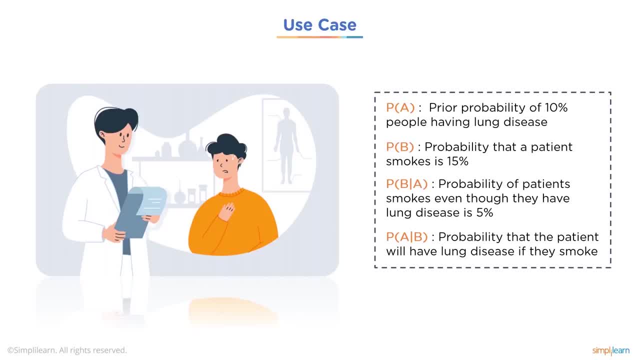 Prior probability of 10% people having lung disease And then probability B- probability that a patient smokes is 15% And the probability of B. if B then A, the probability of a patient smokes even though they have lung disease is 5%. 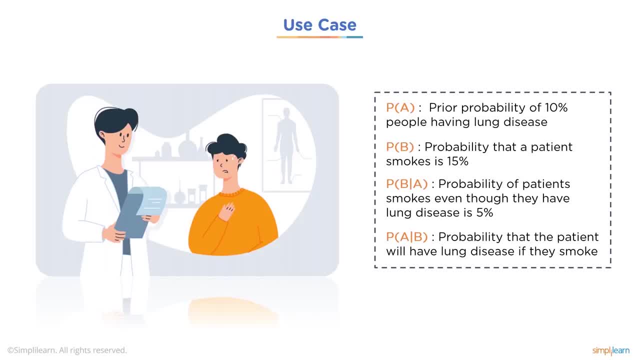 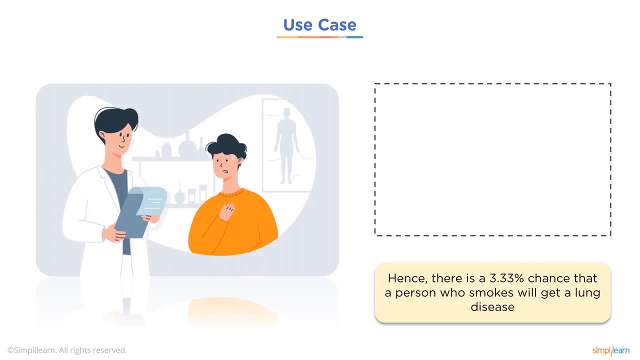 And probability of A is B, probability that the patient will have lung disease if they smoke. And then when you put the formulas together, you get a nice solution. here You get the probability of A of B, probability that the patient will have lung disease if they smoke. 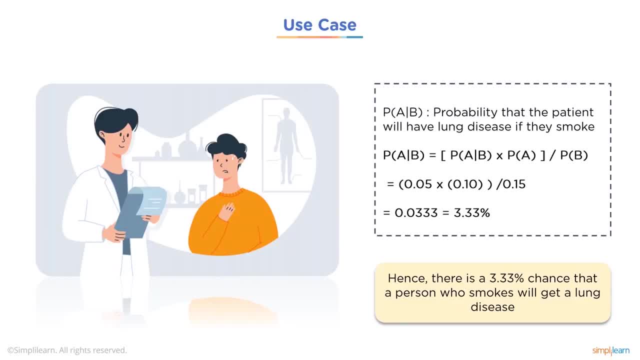 And you can just plug the numbers right in and we get a 3.33% chance. Hence, there is a 3.33% chance that a person who smokes will get a lung disease. So we're going to pull up a little Python code. 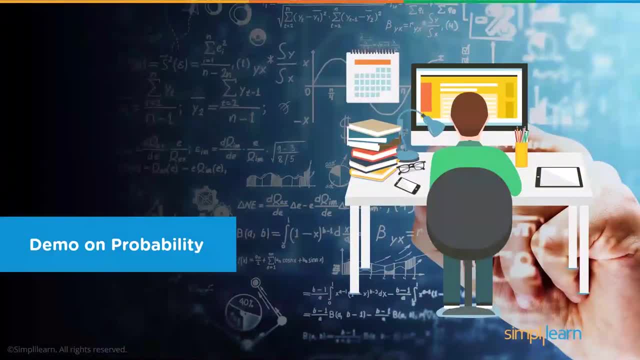 Always my favorite- roll up the sleeves. Keep in mind we're going to be doing this kind of like the back end way so that you can see what's going on, And then later on we're going to create. we'll get into another demo. 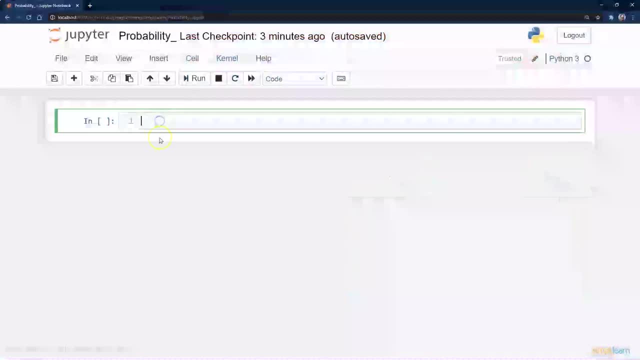 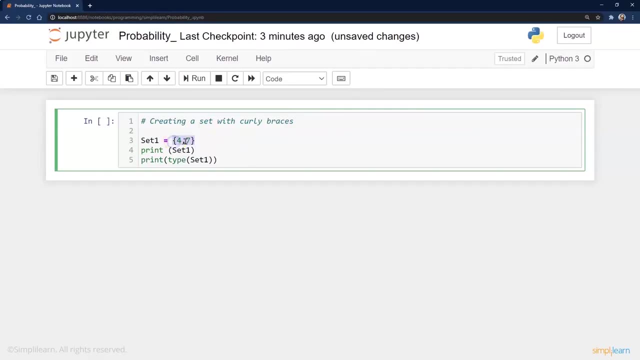 which shows you some of the tools that are already pre-built for this. Let's start by creating a set. So we're going to create a set with curly braces. This means that our set has only unique values. So you have a list. 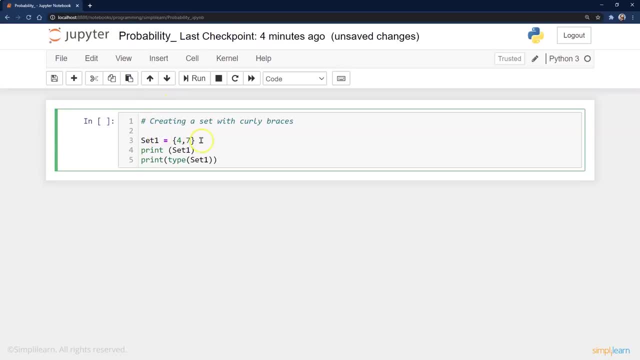 you have your tuples, which can never change, And then you have, in this case, the set, So four, seven. You can't create a four seven comma four. It'll delete the four out, So it's only unique values. 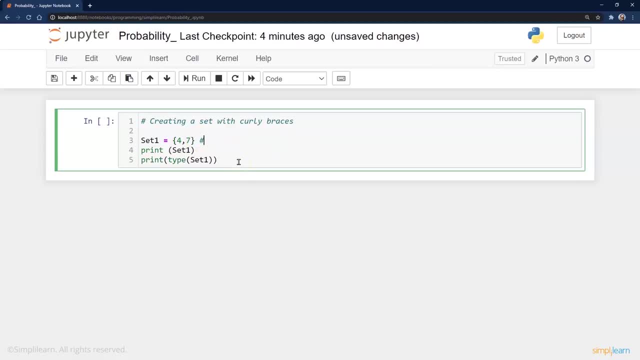 And if you use dictionaries, quick reminder: this should look familiar because it is a dictionary where you have a value and that value is assigned to, or that key is assigned to a value. So you can have a key value set up as a dictionary. 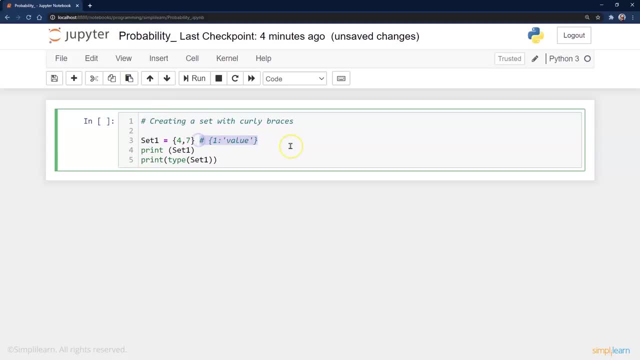 So it's like a dictionary without the value. It's just the keys and they all have to be unique And if we run this, we have a set of four, seven. We can also take a list, a regular set up, and I'm going to go ahead. 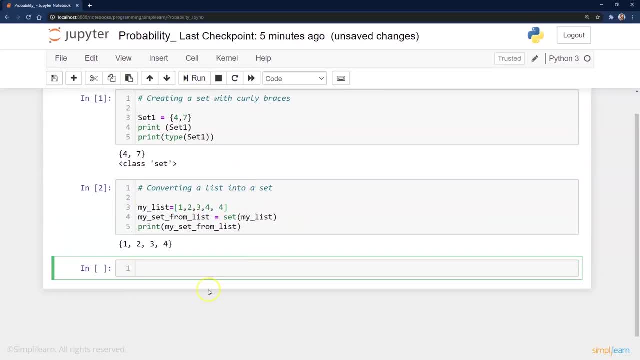 and just throw in another number in here- four- and run it, And you can see here if I take my list one, two, three, four, four, and I convert it to a set and here it is my set from list equals set my list. 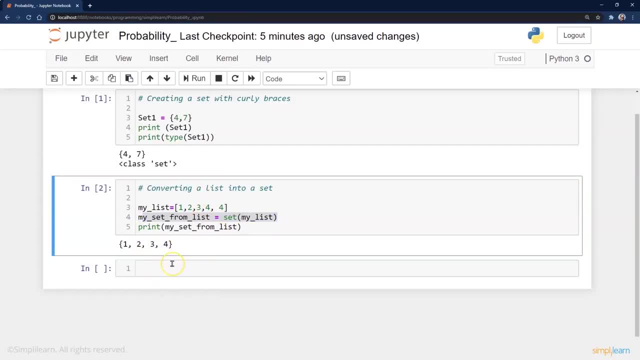 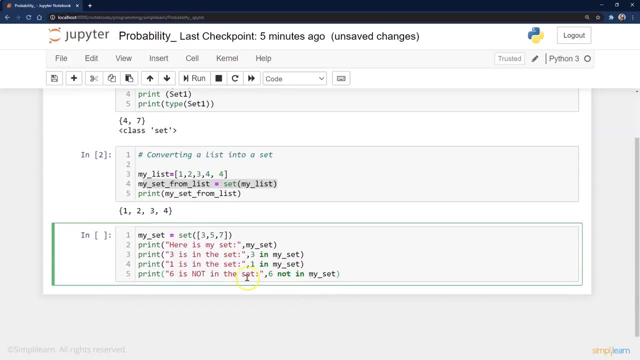 the result is one, two, three, four. So it just deletes that last four right out of there And with the sets you can also go in there and print. here is my set, my set, three is in the set and then, if you do, three in my set. 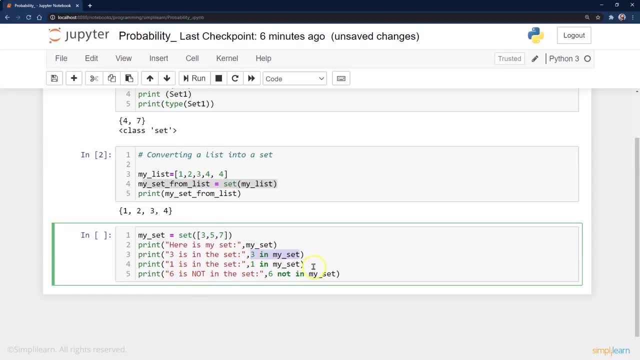 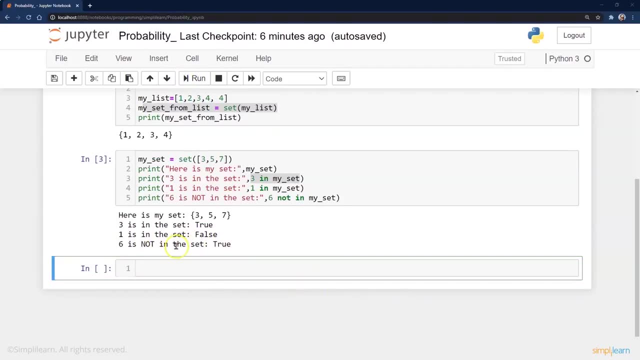 that's going to be a logic function. And one in my set, six is not in the set, and so forth. If we run this, we get: three is in the set- true. one is in the set false because three, five, seven. 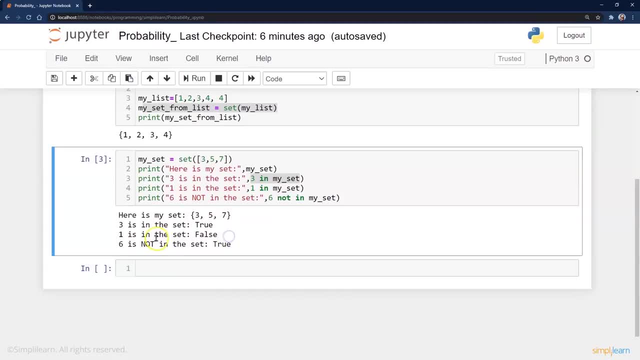 is another one. six is in the set. six is not in the set, so not in my set. You can also use this with a list. We could have just used three, five, seven and it would have the same response on there. 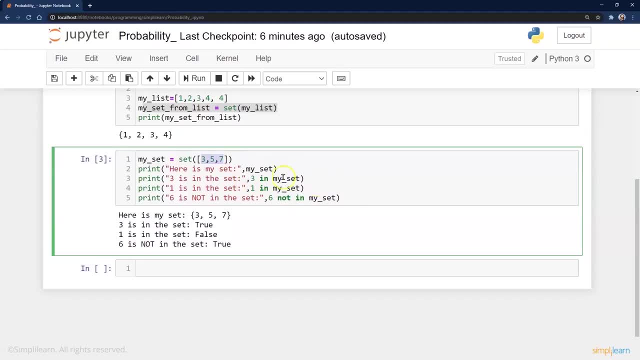 is three in. usually you do if three is in, but three in my set still works on just a regular list And we'll go ahead and do a little iteration. We're going to do kind of the dice: one: Remember one, two, three, four, five, six. 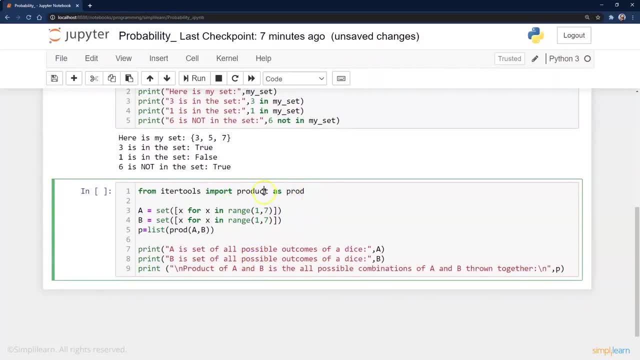 And so we're going to bring in the iteration tool and import product as product, And I'll show you what that means in just a second. So we have our two dice, We have dice A, and it's going to be a set of values. 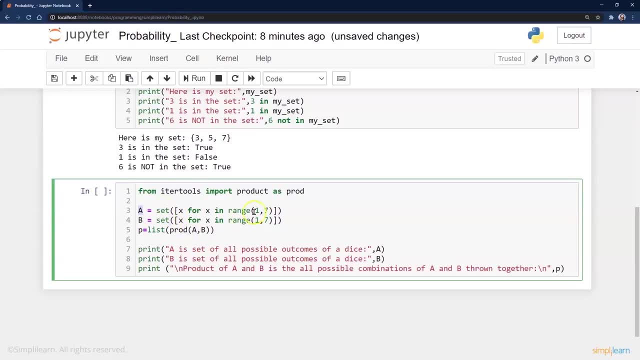 They can only have one value for each one. That's why they put it in a set And if you remember, from range it is up to seven. So this is going to be one, two, three, four, five, six. 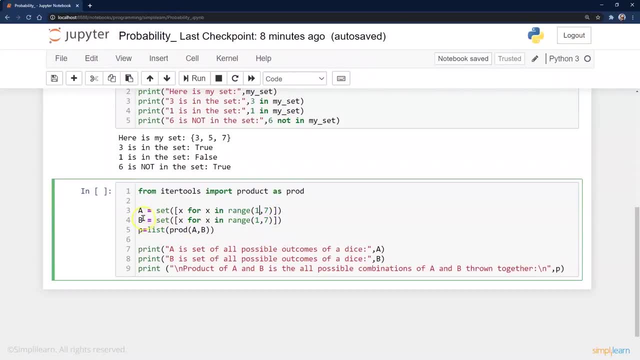 It will not include the seven, And the same thing for our dice B. And then what we're going to do is we're going to create a list which is the product of A and B, So it's A plus B, And if we go ahead and run this, 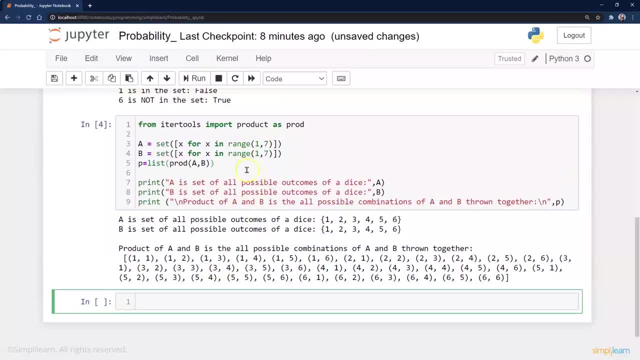 it'll print that out and you'll see. in this case, when they say product- because it's an iteration tool- we're talking about creating a tuple of the two. So we've now created a tuple of all possible outcomes of the dice, where dice A is one, two, three. 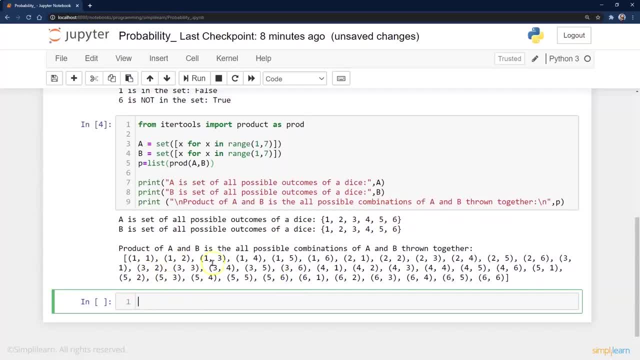 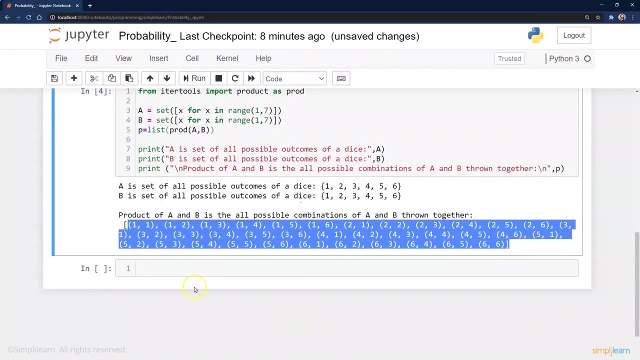 one to six and dice B is one to six And you can see one to one, one to two, one to three and so forth. And you can remember we had a slide on this earlier where we talked about the different, all the different outcomes of a dice. 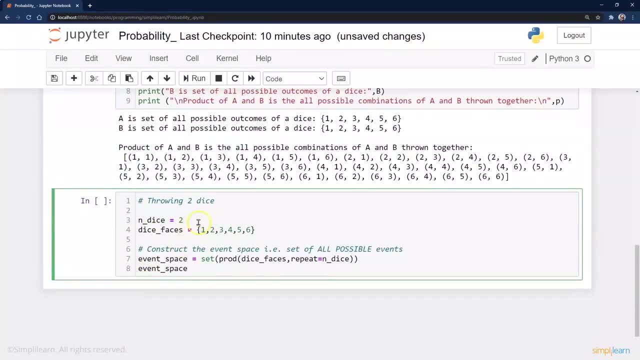 We can play around with this a little bit. We can do: end dice equals two, dice faces one, two, three, four, five, six- Another way of doing what we did before- and then we can create an event space where we have a set. 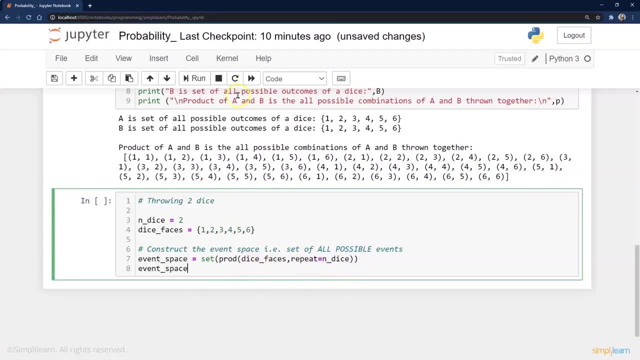 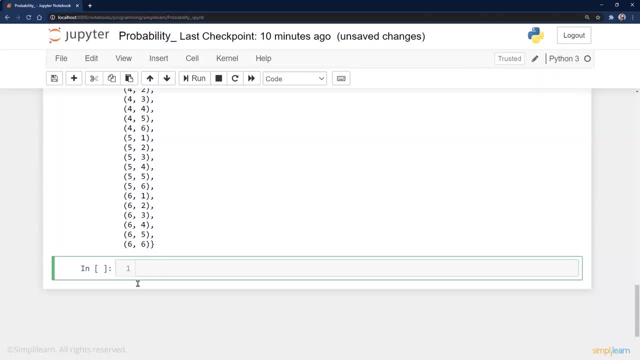 which is the product of the dice faces, repeat, equals, end dice, And we'll go ahead and just run this. You can see here it just again puts it through all the different possible variables we can have. And then if we wanted to take the same set on here, 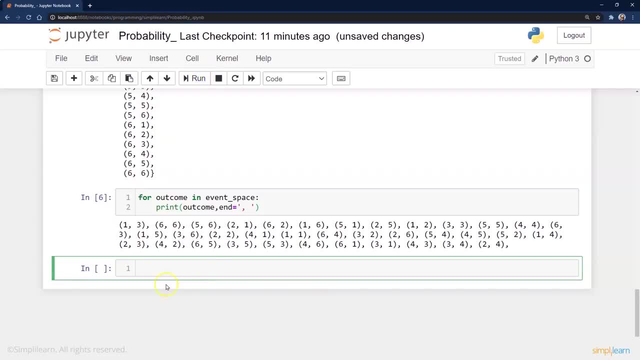 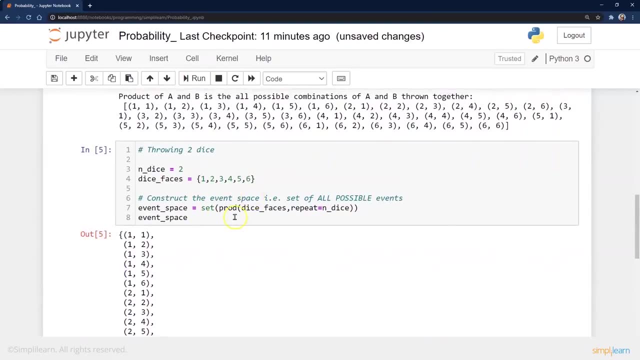 and print them all out like we had before. we can just go through for outcome and event space. outcome end equals. So the event space is creating a sequence And, as you can see here, when we print it out it stacks them versus going through. 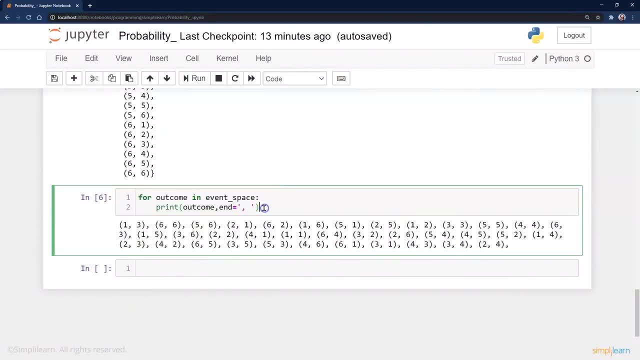 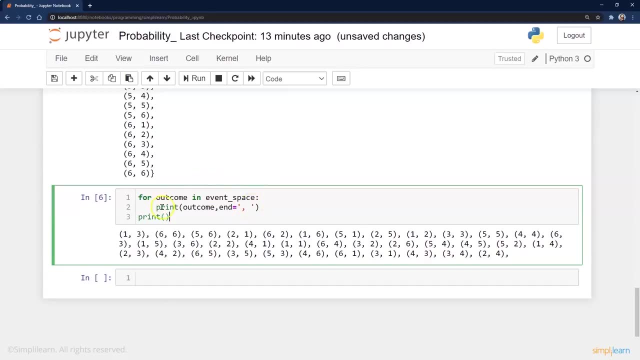 and putting them in a nice line And we'll go ahead and do something. Let's go print. Since we have the end printing with a comma, that just means it's just going to, it's not going to hit the return going down to the next line. 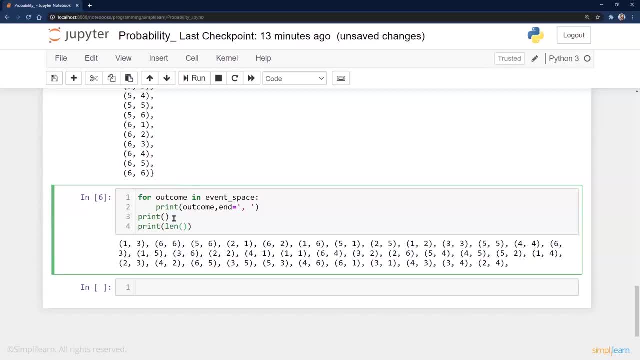 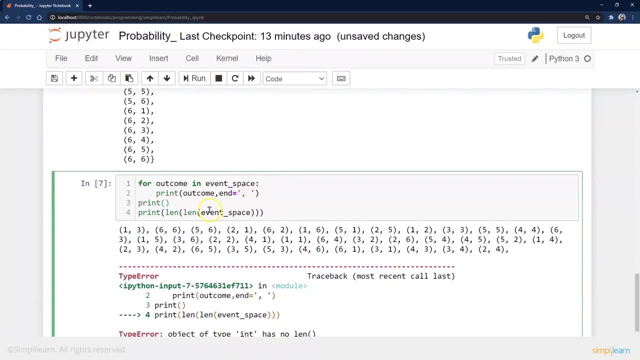 And we'll go ahead and do the length of our event space. That'll be an important variable we're going to want to know in a minute And, of course, if I get carried away with my typing of length, we'll print it twice. 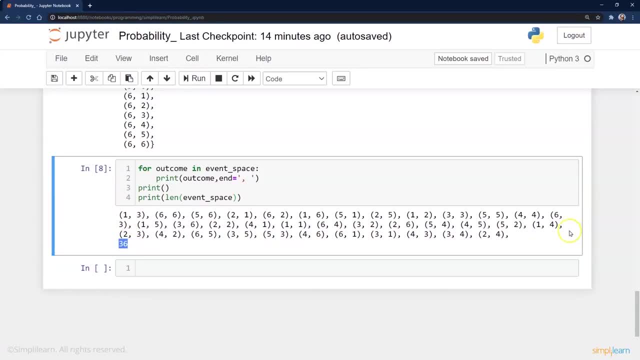 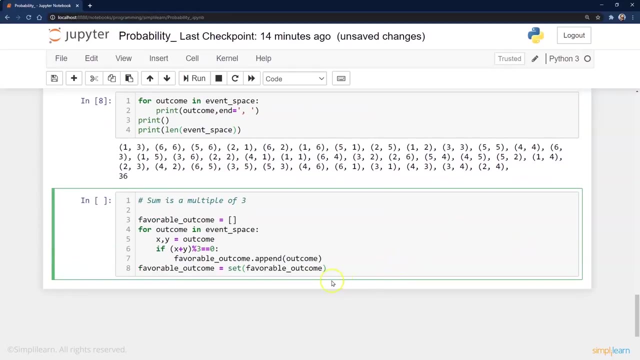 and it'll give me an error. So we have 36 different possible variations here And we might want to calculate something like: what about the multiple of three? What if we want to have the probability of the multiple of three in our setup? 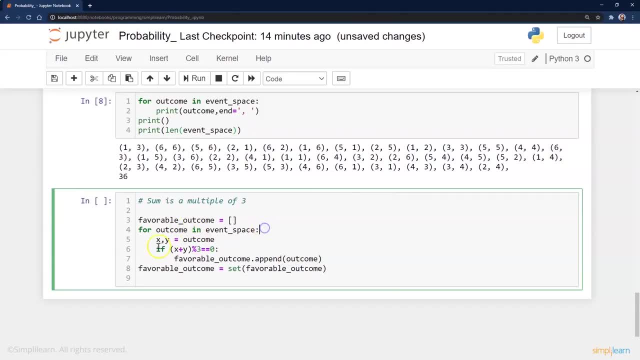 And so we can put together the code for the outcome. and event space of xy equals outcome if x plus y remainder three. So we're going to divide by three and look at the remainder and it equals zero, Then it's a favorable outcome. We're going to pop that outcome. 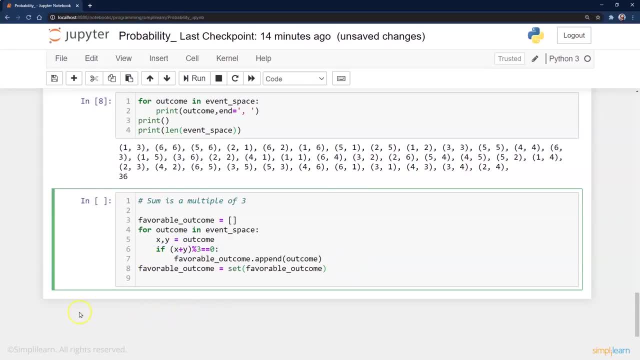 on the end there And we'll turn it into a set. So the favorable outcome equals a set. Not necessary because we know it's not going to be repeating itself, But just in case, we'll go ahead and do that. And if we want to print out, 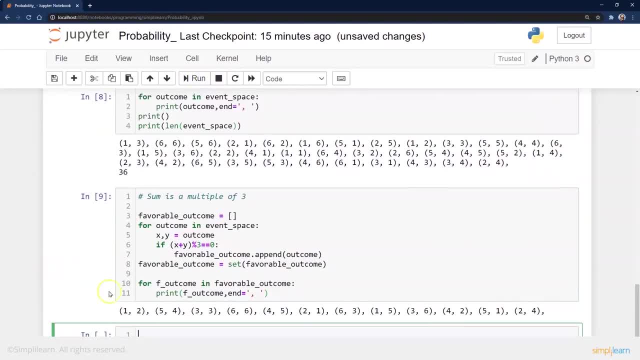 the outcome. we can go ahead and see what that looks like And you can see here. these are all multiples of three. One plus two is three, five plus four is nine, which divided by three is three and so forth. And just like we looked up, 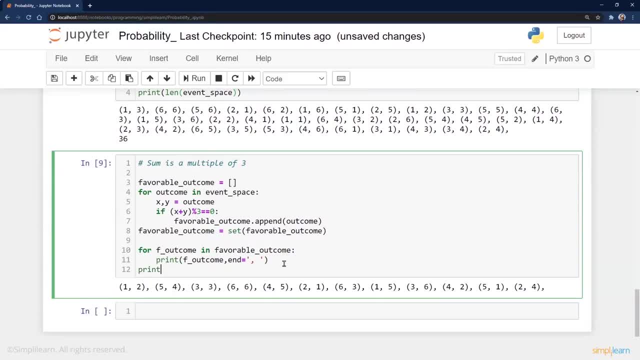 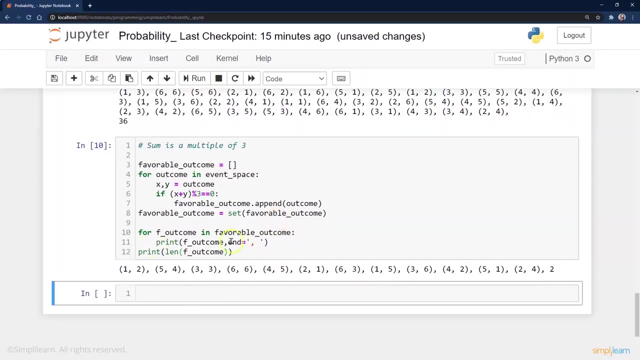 the length of the one before let's go ahead and print the length of our f outcome, So we can see what that looks like. There we go, And of course I did forget to add the print in the middle because we're looping through. 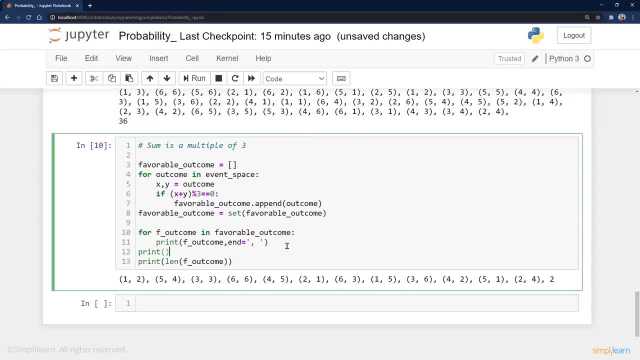 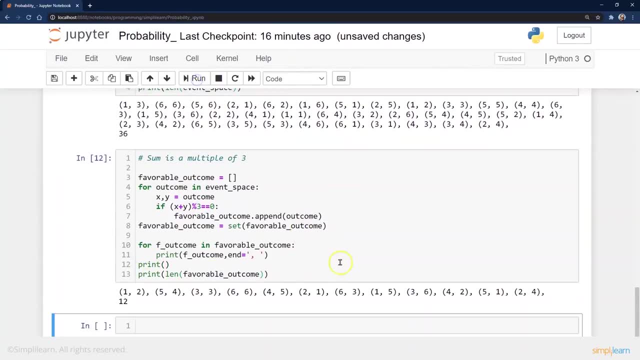 and putting an end on the setup on there. So we're going to put the print in there And if I run this, you can see we end up with 12.. So we have 36 total options. We have 12 that are multiple. 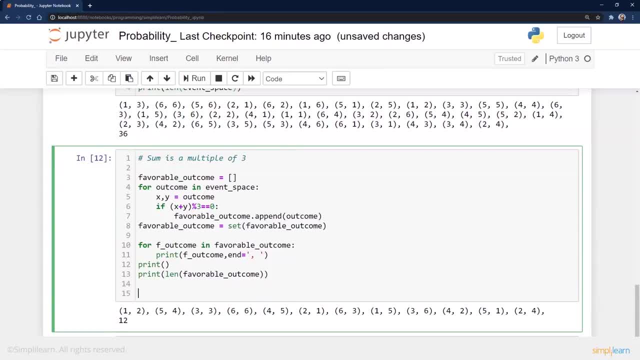 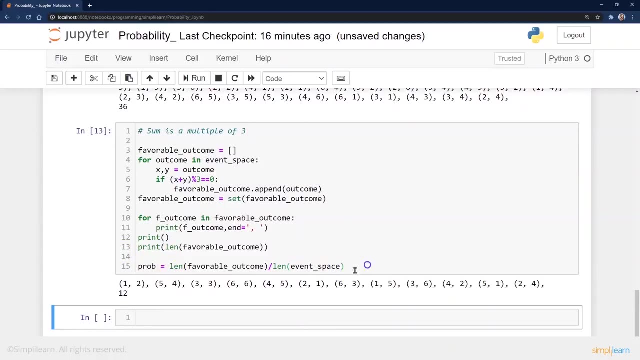 that add up to a multiple of three. And we can easily compute the probability of this by simply taking the length of our favorable outcome over the length of the event space. And if we print it out, let me put that in there: probability last line. 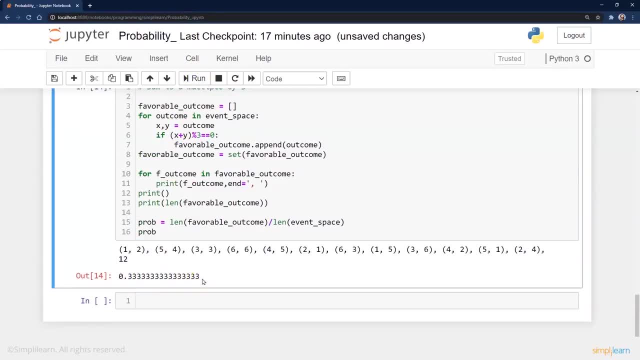 so we can just type it in. we end up with a .3333 chance, And that's roughly a third, And we might want to make this look nice, so let's go ahead and put in another line there The probability of getting. 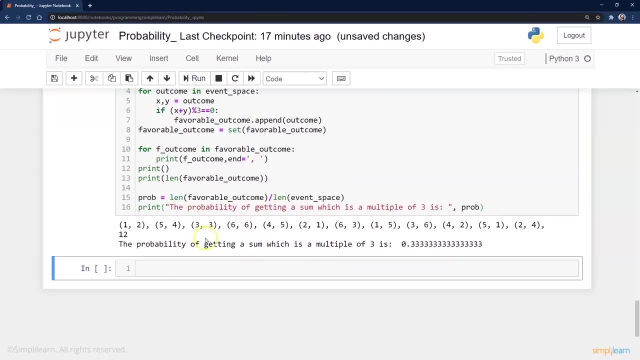 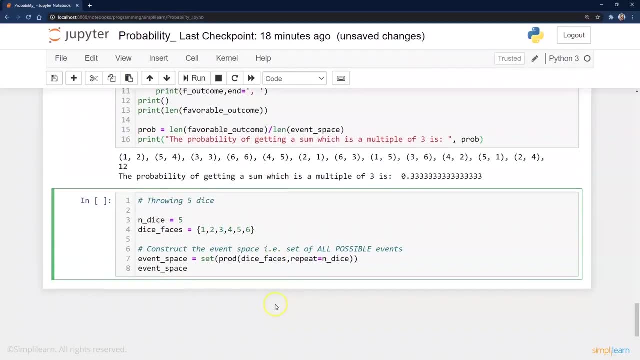 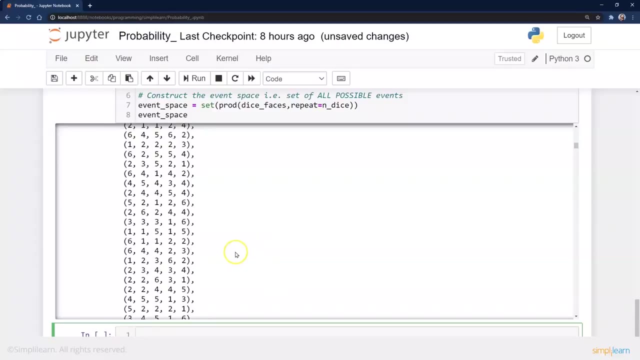 the sum, which is a multiple of three, is .3333.. We can compute the same thing for five dice And if we do this for five dice and go ahead and run it, you can see we just have a huge amount of choices. 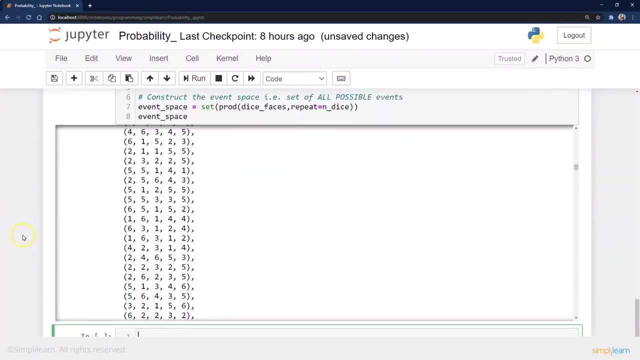 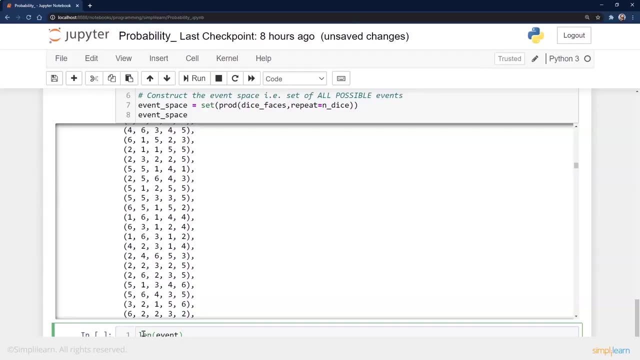 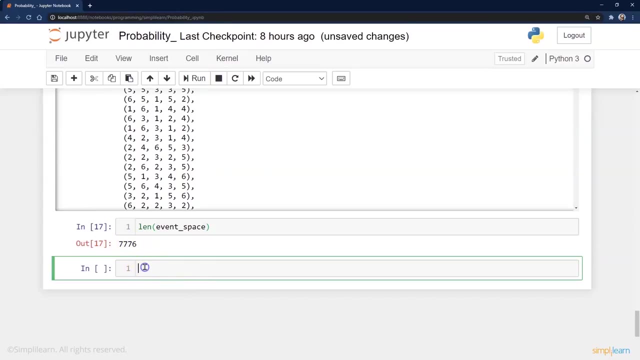 So it just goes on and on down here And we can look at the length of the event space And we have over 7,776 choices. That's a lot of choices, And if we want to ask the question like we did above, 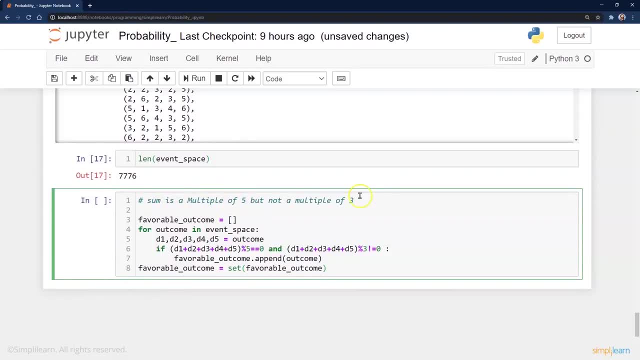 where the sum is a multiple of five but not a multiple of three. we can go through all of these different options and then you can see here: D1, D2,, D3,, D4, D5 equals the outcome, And if you add these all together, 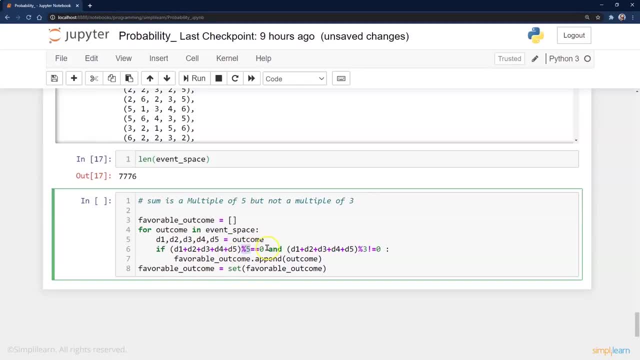 and the division by five does not have a remainder of zero, but the remainder is also of a division by three is not equal to zero. So the multiple of five is equal to zero, but the multiple of three is not. We can just append that on here. 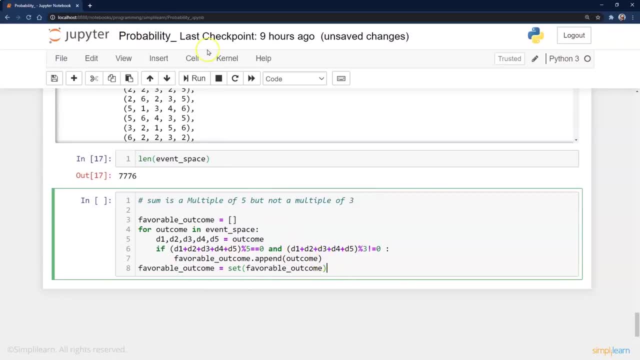 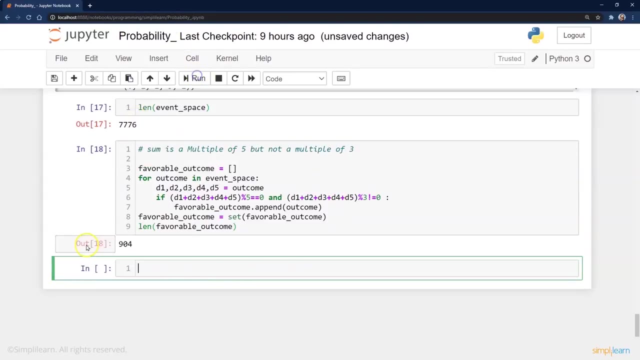 And then we can look at that favorable outcome And we'll go ahead and set that And we'll just take a look at this. What's our length of our favorable outcome? It's always good to see what we're working with, And so we have 904. 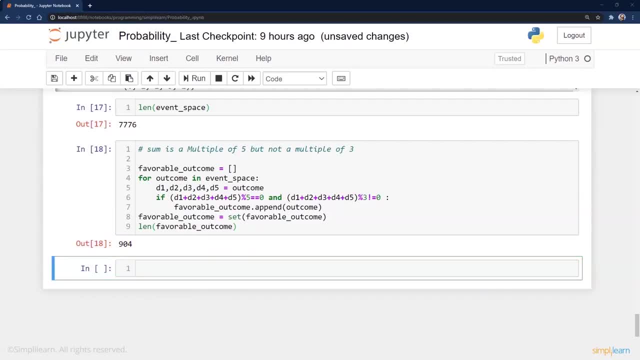 out of seven, So we have 904 out of 776.. And then, of course, we can just do a simple division to get the probability on here. What's the probability that we're going to roll a multiple of five when you add them together? 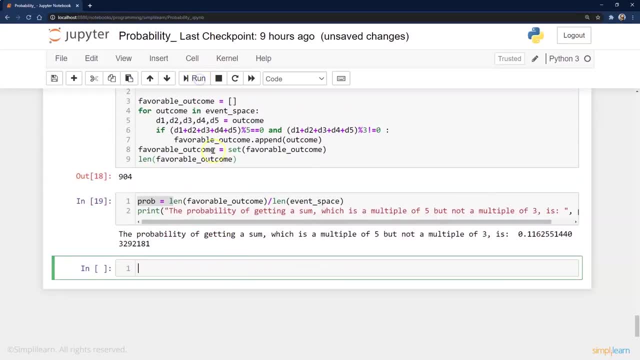 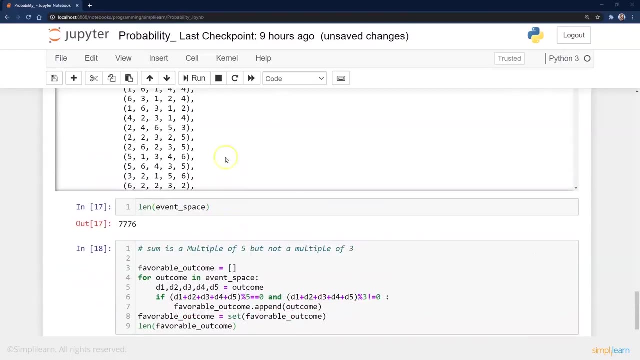 but not a multiple of three, And so we're just going to divide those two numbers And you can see here we get 0.116255 or 11.62%, And so you can really have a nice visual that this is not really complicated math. 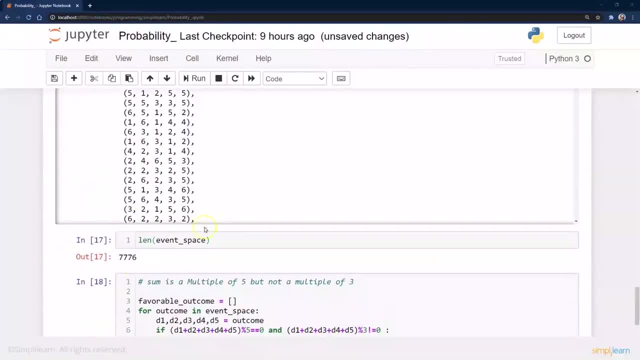 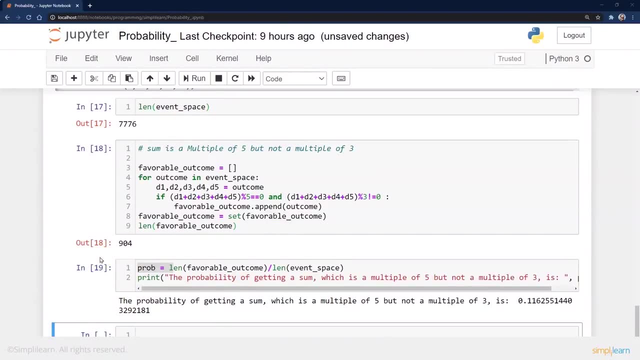 right here on probabilities. It's: just how many options do you have and how many of those are you possibly going to be able to come up with the solution you're looking for? And this leads us to a confusion matrix. A confusion matrix is a table. 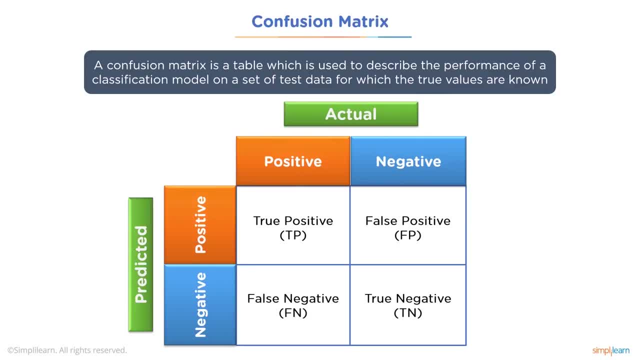 which is used to describe the performance of a classification model on a set of test data for which the true values are known. And so you'll see, on the left we have the predicted and the actual And we have a negative, false, negative. 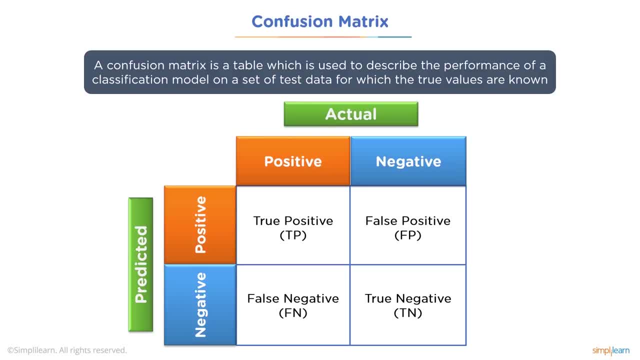 positive, true positive, and then we have false positive and true negative, And you can think of this as your predicted model. What does that mean? That means if you divided your data and you used two-thirds of it to create the model, you might then test it. 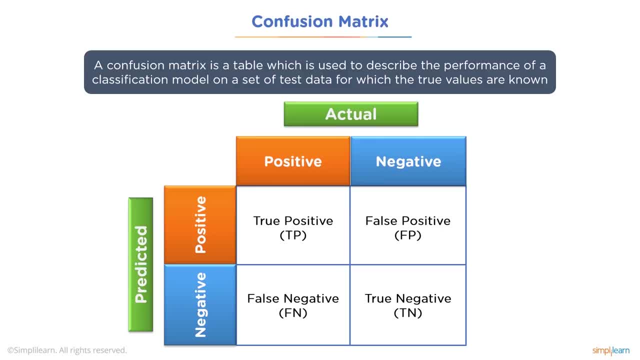 against an actual case for the last third, to see how well it comes out. How many times was it true positive versus true negative Versus false positive? You get a false positive response And you can imagine in medical situations this is a pretty big deal. 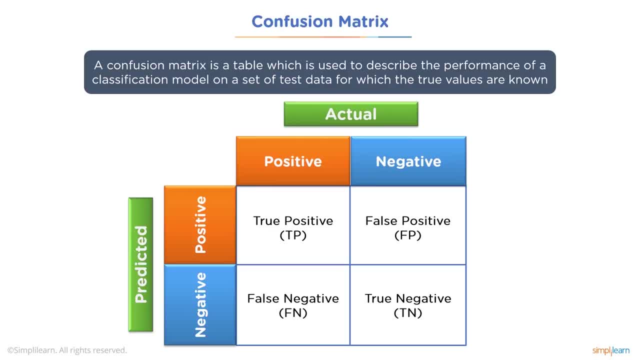 You don't want to give a false positive, So you might adjust your model accordingly so you don't have a false positive, Say with a COVID virus test. it'd be better to have a false negative and then go back and get retested than to have 30%. 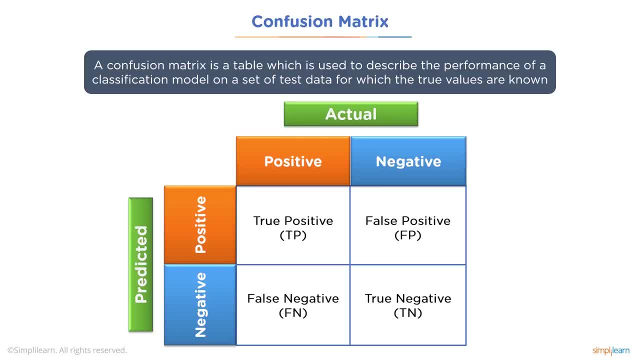 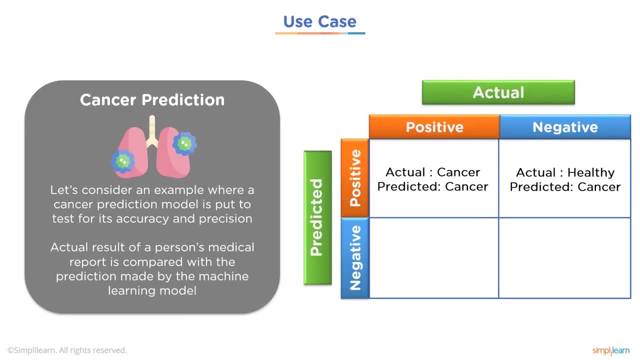 false positives, where then the test is pretty much invalid. So in a used case like cancer prediction, let's consider an example where a cancer prediction model is put to the test for its accuracy and precision. Actual result of a person's medical report is compared. 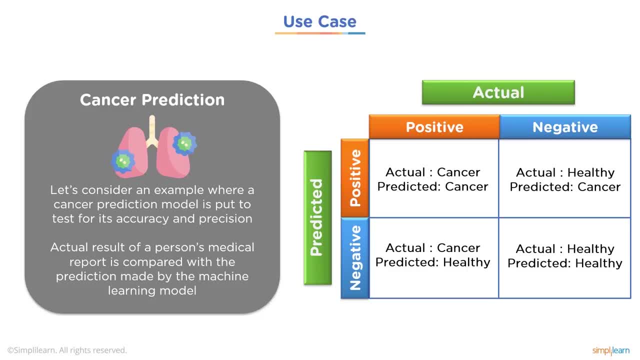 with the prediction made by the machine learning model, And so you can see here, here's our actual predicted. whether they have cancer or not, You know cancer, a big one. you don't want to have a false positive, I mean a false negative. 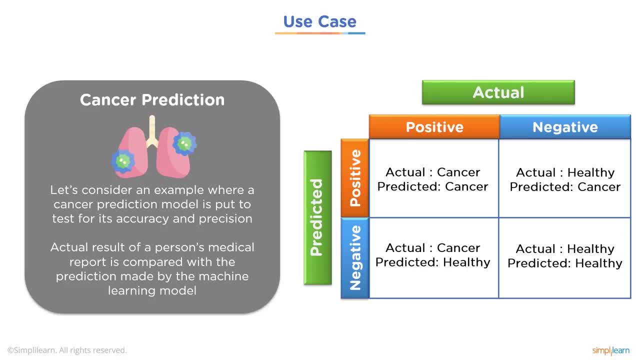 In other words, you don't want to have it tell you that you don't have cancer when you do So. that would be something you'd really be looking for in this particular domain. You don't want a false negative, And this is again. 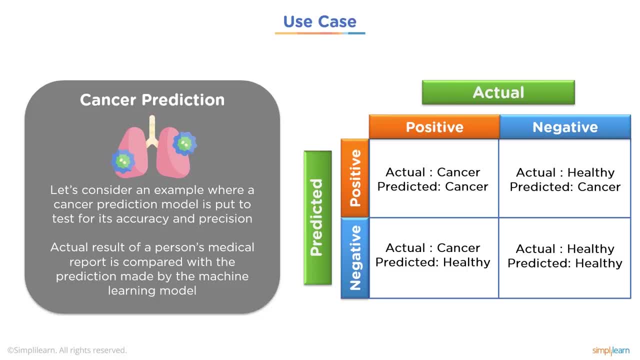 you know you've created a model. you have hundreds of people or thousands of pieces of data that come in. There's a real famous case study where they have the imagery and all the measurements they take And there's about 36 different measurements they take. 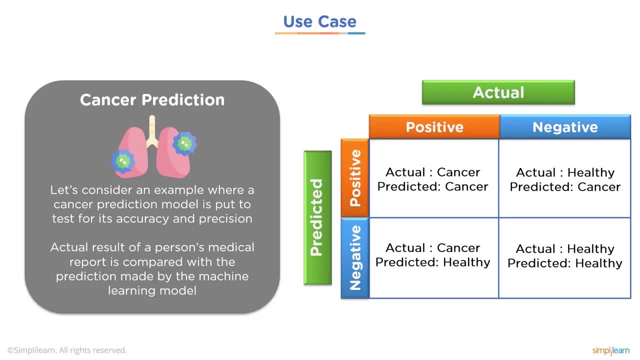 And then if you run a basic model, you want to know just how accurate it is. How many negative results do you have that are either telling people they have cancer that don't, or telling people that don't have cancer that don't have cancer that they do? 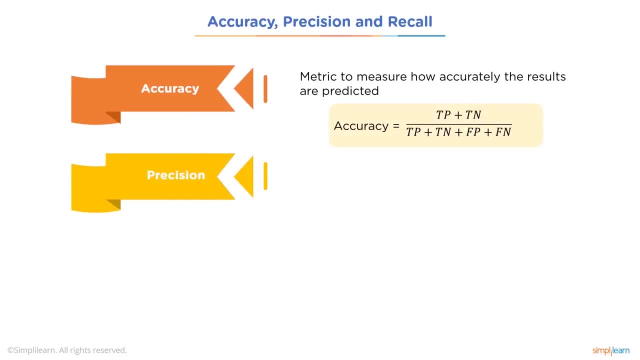 And then we can take these numbers and we can feed them in to our accuracy, our precision and our recall. So accuracy, precision and recall: Accuracy metric to measure how accurately the results are predicted. And this is your total true, where you've got. 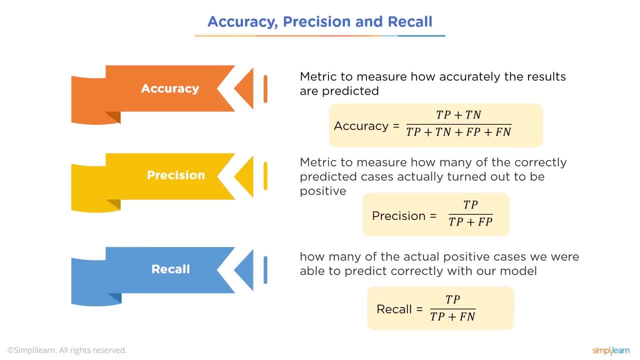 the right results. you add them together, the true positive, the true negative, over all the results. So what percentage of them were accurate versus what were wrong? When we talk about, precision is a metric that's used to measure how many of the correctly. 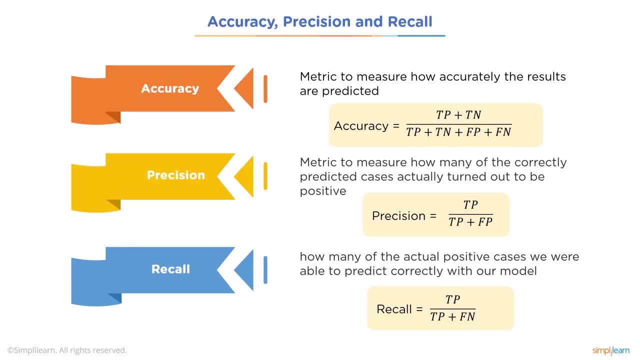 predicted cases are actually turned out to be positive. So we have a precision on true positive. Again, if you're talking about, like COVID testing with the viruses, you really want this to be a high number. You want this true that to be the center point. 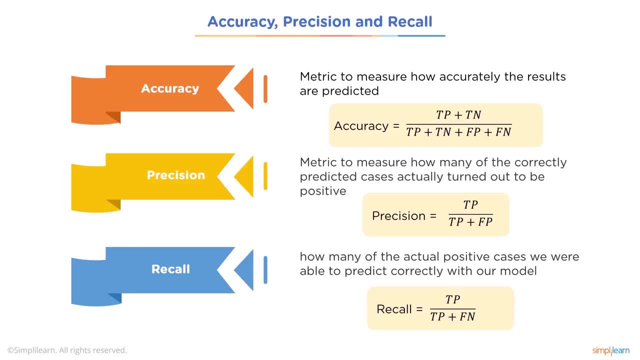 where you might have the opposite, if you're dealing with cancer, where you want no false negatives. So this is your metric on here. Precision is your test positive, true positive plus false positive, And then your recall how many of the actual positive cases. 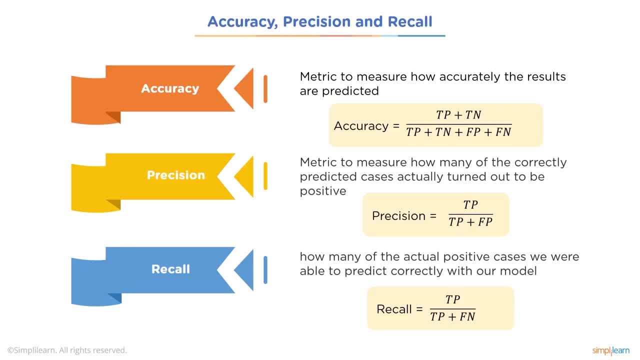 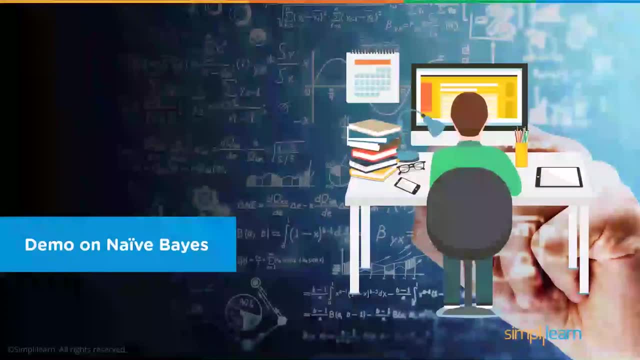 we were able to predict quickly with our model. So test positive is the test positive plus the false negative on there And we'll want to go ahead and do a demo on the Naive Bayes classifier Before I get too far into Naive Bayes classifier. 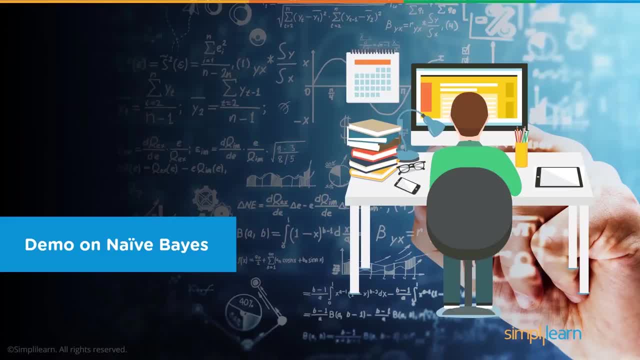 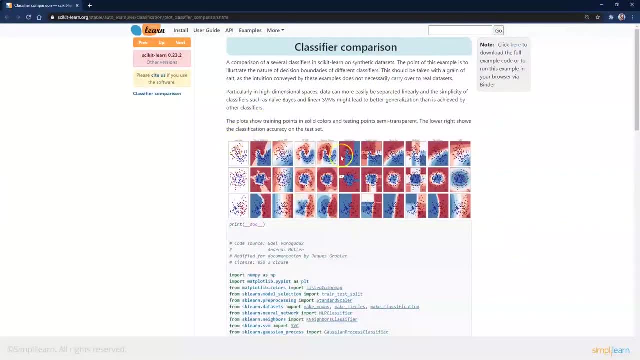 because we're going to pull it from the sklearn or the scikit. Let's go ahead. Kind of an interesting page here for classifiers. When you go into the sklearn kit there's a lot of ways to do classification And I'll just zoom up in here. 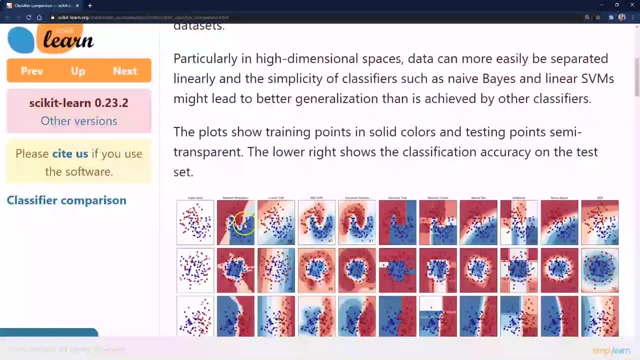 so you can see some of the titles. There's everything from the nearest neighbor, linear, but we're going to be focusing on the Naive Bayes over here And this is just a sample data set that they put together and you can see how. 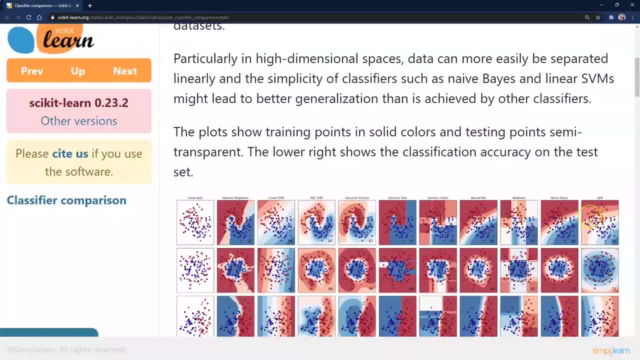 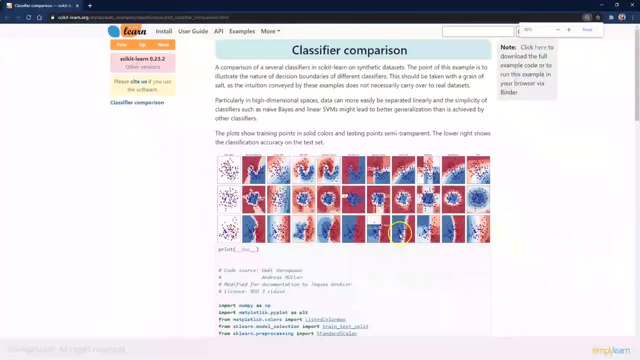 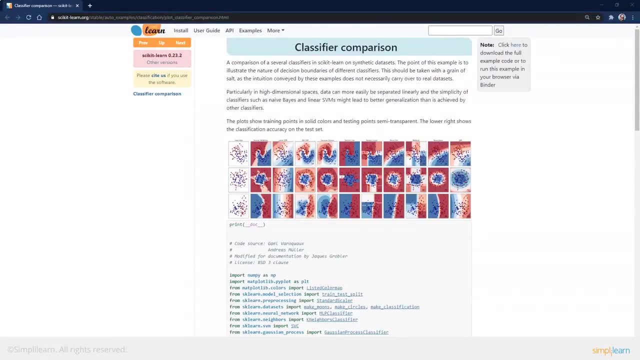 some of these have a very different output. The Naive Bayes, remember, is set up as probably the most simplified calculator or set of predictions out there, And so what we've been talking about with the true-false and stuff like that, where there's a belief, 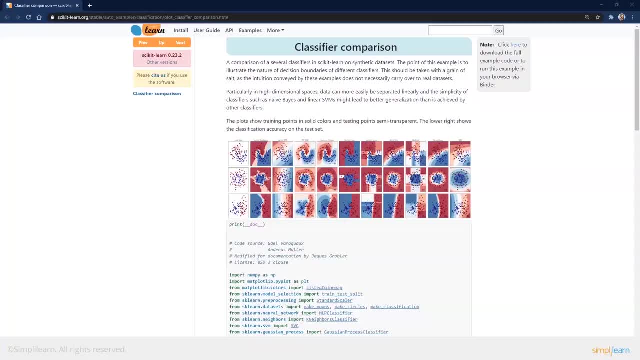 that there is an independent assumption between the features. where the features are very assumed to have some kind of connection, Then we can go ahead and use that for the prediction, And so that's what we're using as a Naive Bayes classifier versus many of the other classifiers. 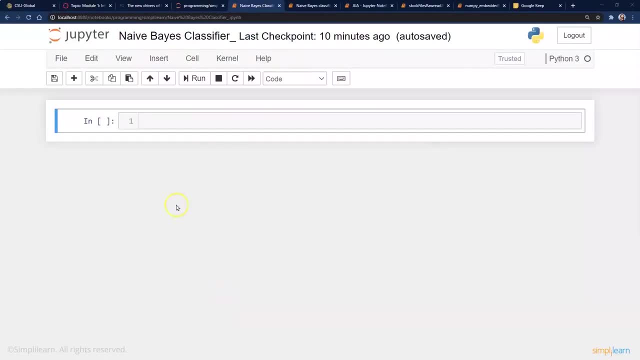 that are out there. For this we're going to use the social network ads. It's a little data set on here And let me go ahead and just open that up the file. Here we go. It has user ID, gender, age. 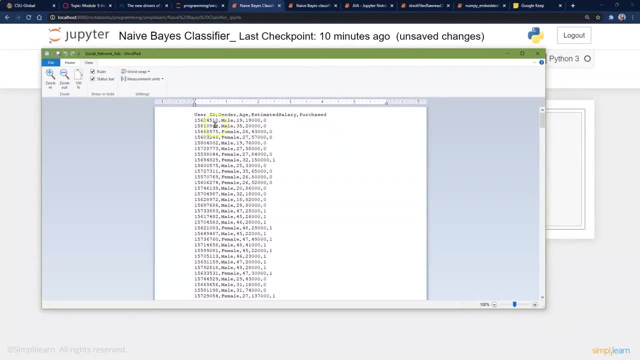 estimated salary: purchased. And so we can see the user ID: male 19,. estimated salary: 19,000, and purchase: just zero. So it's either going to make a purchase or not. So look at that last one, 01.. 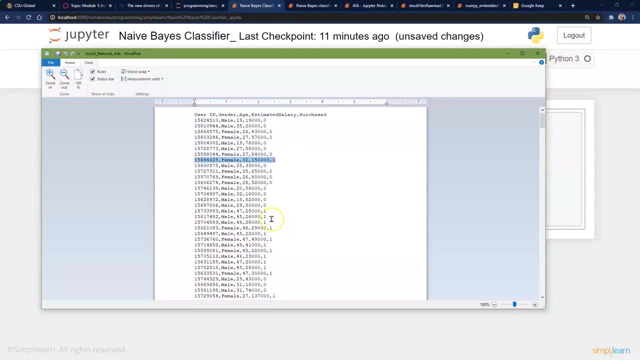 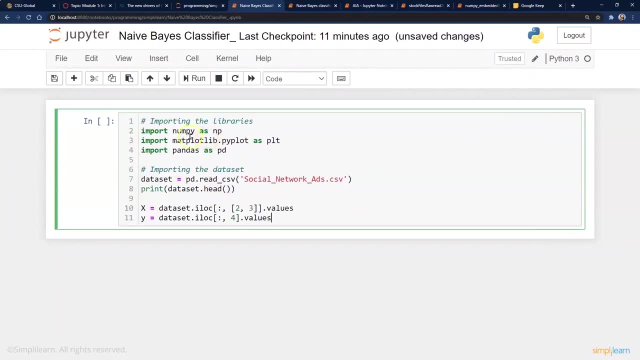 We should be thinking of binomials. We should be thinking of simple Naive Bayes classifier kind of setup. So if we close this out, we're going to go ahead and import our numpy as np We're going to like to have. 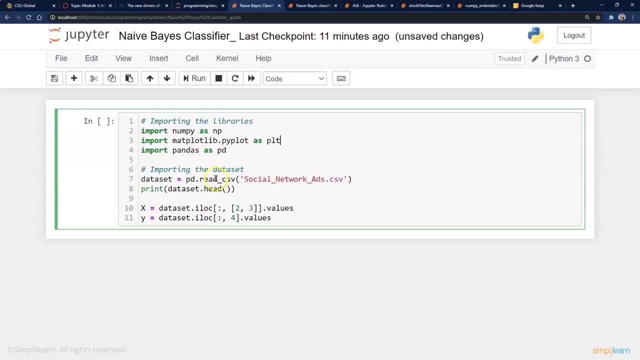 a good visual of our data. So we'll put in our Matplot library- Here's our pandas, our data frame, And then we're going to go ahead and import the data set. And the data set's going to be. we're going to read it from: 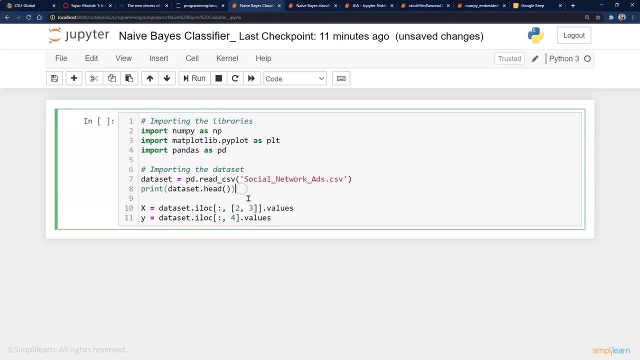 the socialnetworkadscsv, Then we're going to print the head, just so you can see it again, even though I showed you it in the file. And X equals the data set. I, location two, three values and Y is going to be the four. 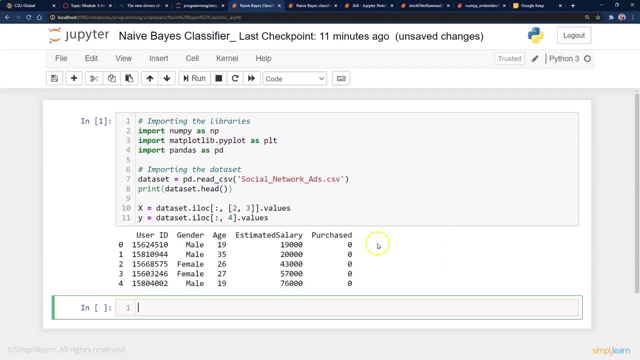 column four. Let me just run this so it's a little easier to go over that. You can see right here we're going to be looking at. 012 is age and estimated salary. so two, three And that's what I location just means that we're looking. 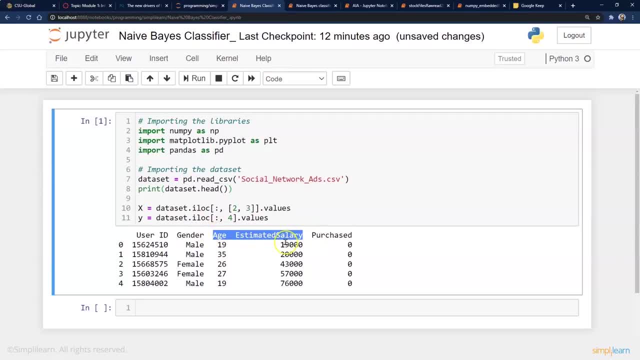 at the number versus a regular location. A regular location, you'd actually say age and estimated salary. And then column four is: did they make a purchase? They purchased something. So those are the three columns we're going to be looking at when we do this. 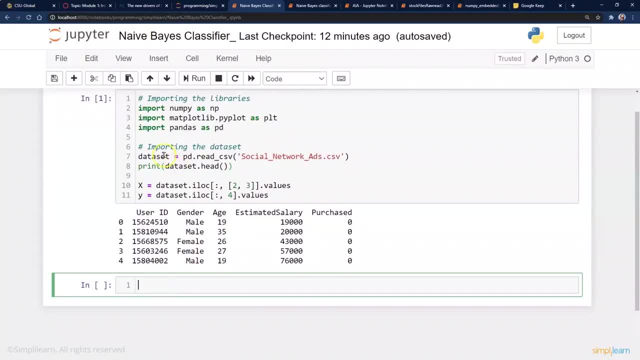 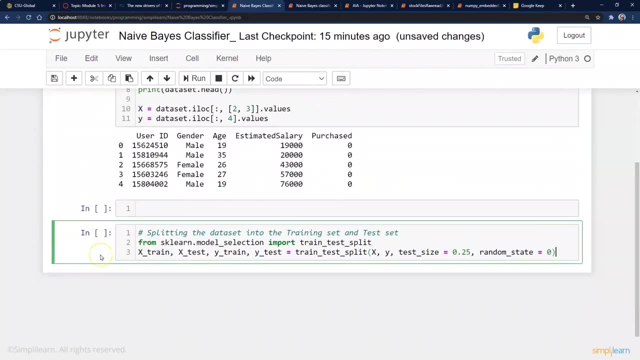 And we've gone ahead and imported these and imported the data. so now our data set is all set with this information in it And we're going to go ahead and split the data up. So we need our from the sklearn model selection. 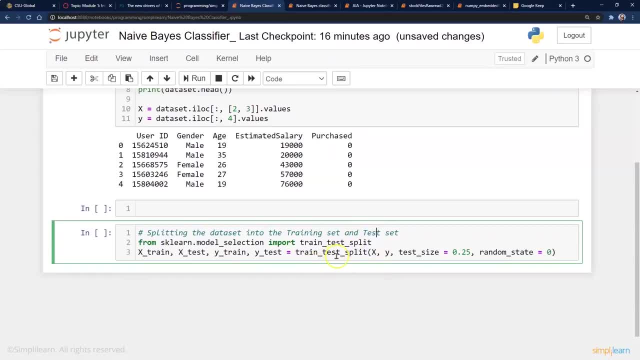 we can import train test split. This does a nice job. We can set the random state so it randomly picks the data And we're just going to take 25% of it's going to go into the test- our X test and our Y test. 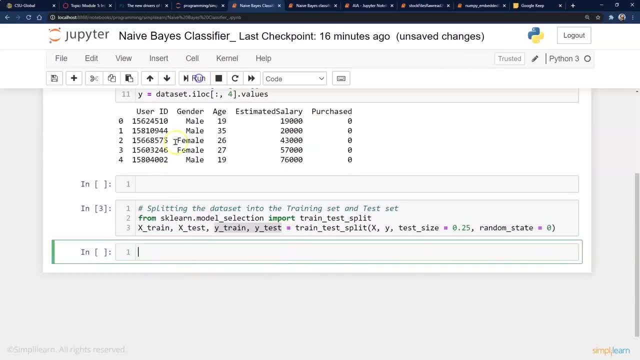 and the 75% will go to X train and Y train. That way, once we create our model, we can then have data to see just how accurate or how well it has performed with our prediction. The next step in pre-processing our data is to go ahead. 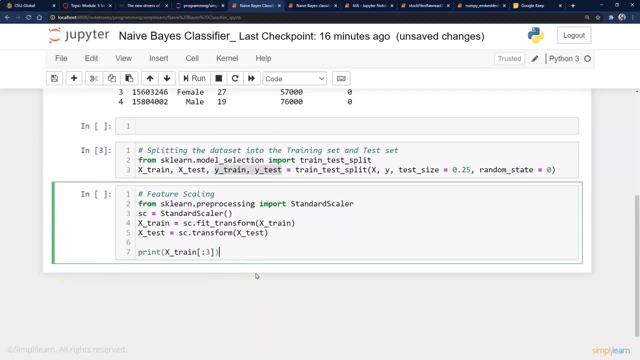 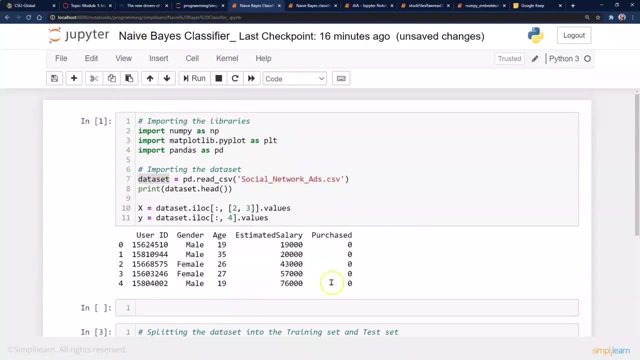 and do feature scaling. Now a lot of this is starting to look familiar. If you've done a number of the other modules and setup, you should start noticing that we bring in our data. we take a look at what we're working with. 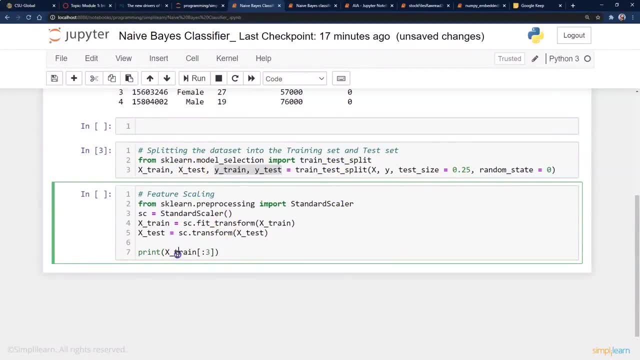 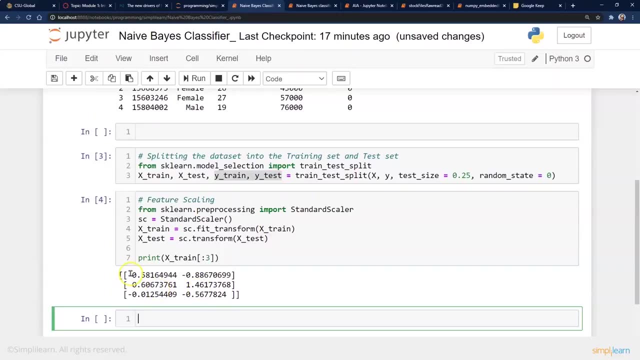 We go ahead and split it up into training and testing. In this case, we're going to go ahead and scale it. Scale it means we're putting it between a value of minus one and one or someplace in the middle ground there. 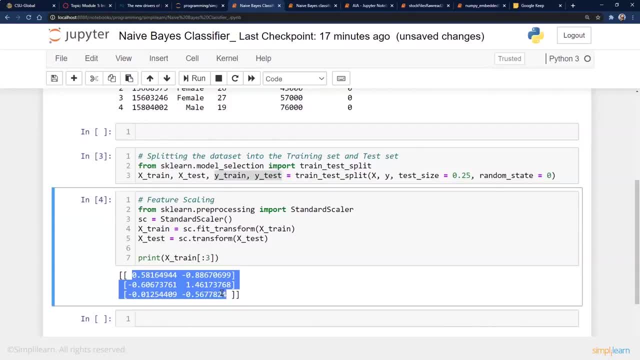 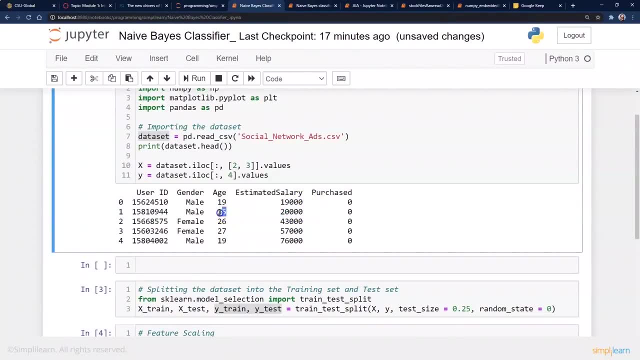 This way, if you have any huge, you don't have this huge setup. if we go back up to here, where salary is 20,000 versus age 35, well, there's a good chance with a lot of the back-end math. 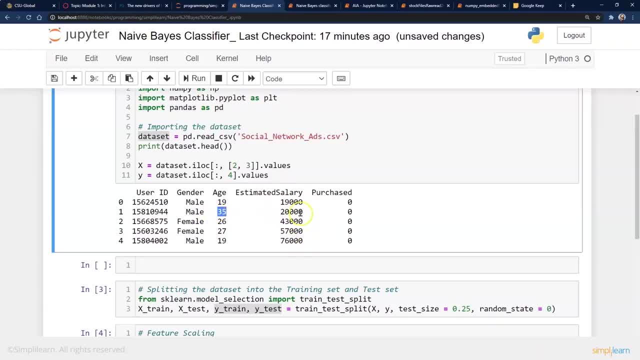 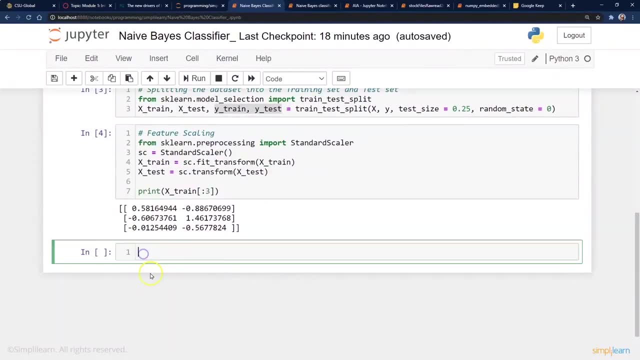 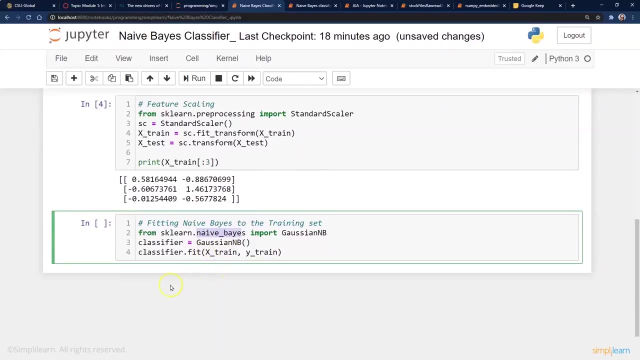 that 20,000 will skew the results, and the estimated salary will have a higher impact than the age, instead of balancing them out and letting the calculations weigh them properly. And finally, we get to actually create our naive Bayes model, And then we're going to go ahead. 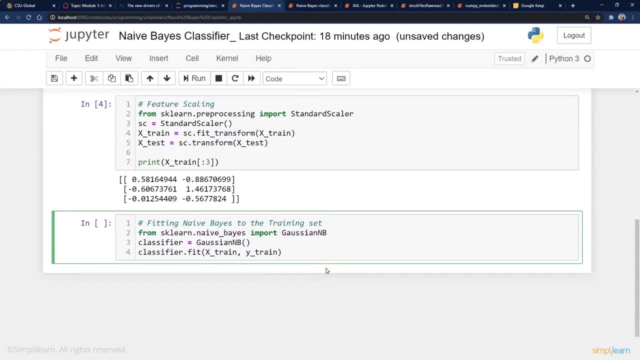 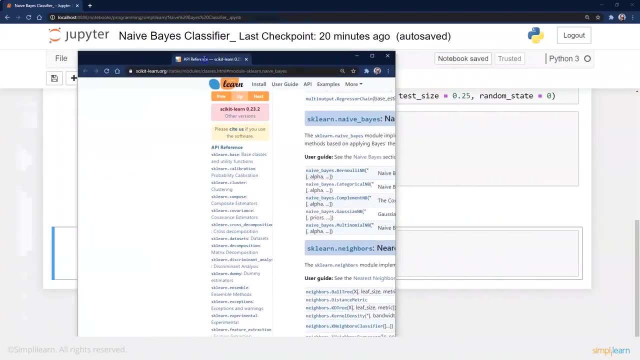 and import the Gaussian naive Bayes, And the Gaussian is the most basic one. That's what we're looking at now. It turns out, though, if you go to the sklearn kit, they have a number of different ones you can pull in there. 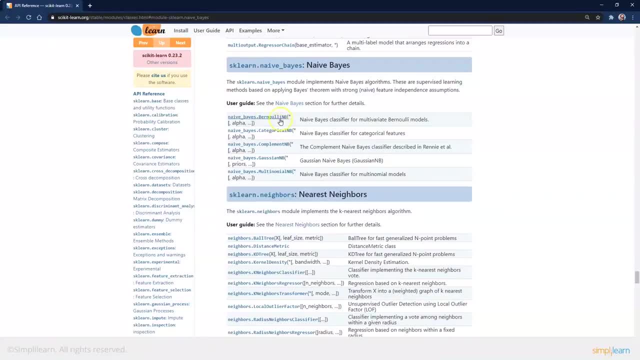 There's Bernoulli- I've never used that one Categorical Complement- and here's our Gaussian. So there's a number of different options you can look at. Gaussian, when you come to the naive Bayes is the most commonly used. 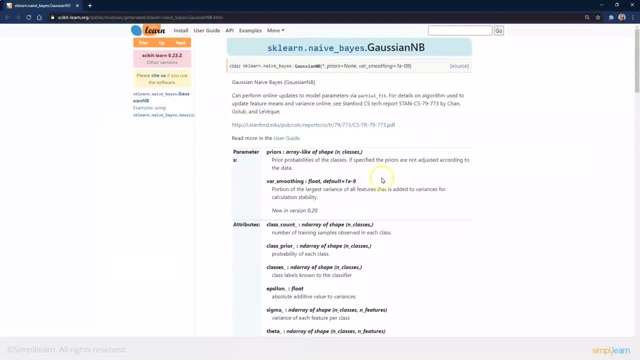 So we're talking about the naive Bayes. That's usually what people are talking about when they're pulling this in, And one of the nice things about the Gaussian- if you go to their website to sklearn the naive Bayes, Gaussian. 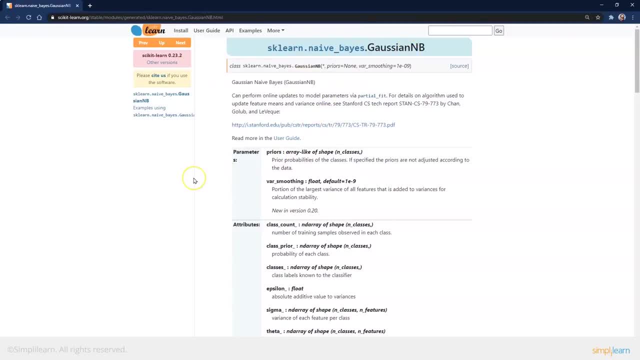 there's a lot of cool features. One of them is you can do partial fit on here. That means if you have a huge amount of data, you don't have to process it all at once. You can batch it into the Gaussian NB model. 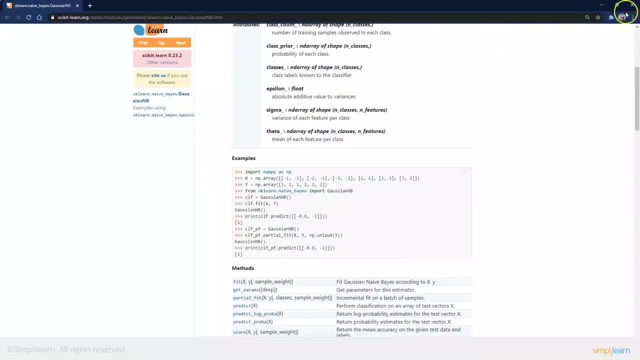 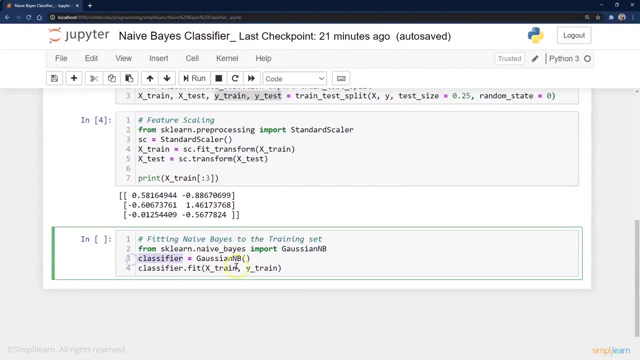 And there's many other different things you can do with it as far as fitting the data and how you manipulate it. We're just doing the basics, So we're going to go ahead and create our classifier. We're going to equal the Gaussian NB. 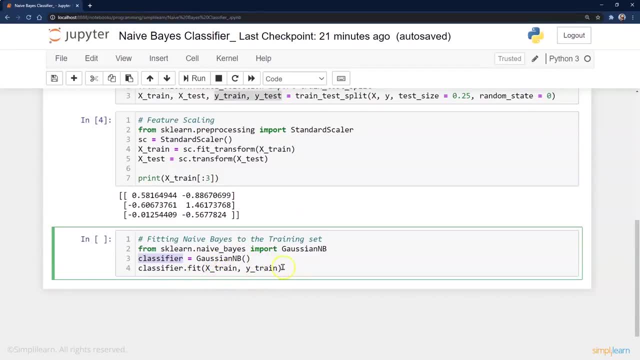 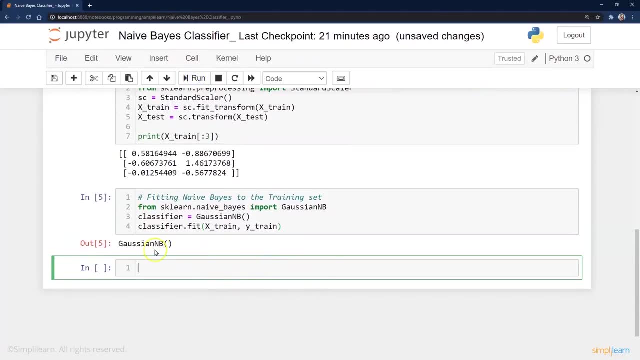 And then we're going to do a fit. We're going to fit our training data and our training solution. So X train, Y train, And we'll go ahead and run this. It's going to tell us that it ran the code, right there. 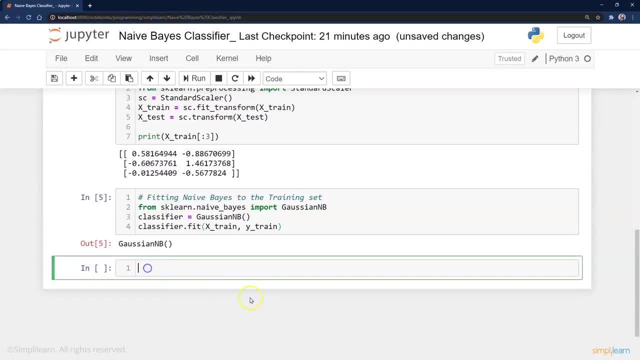 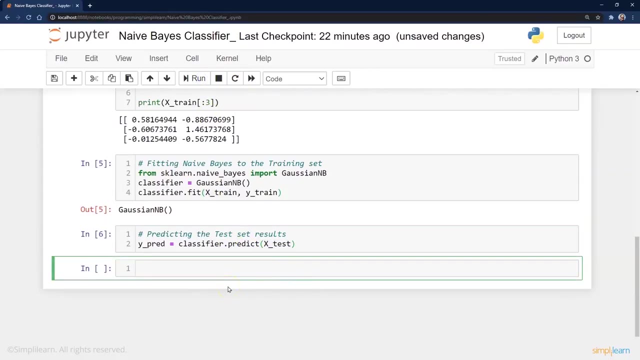 And now we have our trained classifier model. So the next step is we need to go ahead and run a prediction. We're going to do our Y predict equals the classifier dot predict X test. So here we fit the data And now we're going to go ahead and predict. 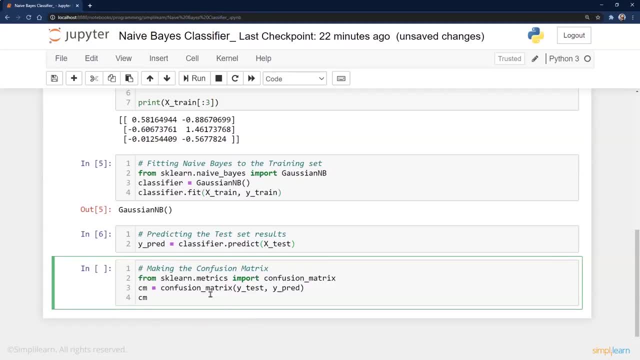 And now we get to our confusion matrix. So from the sklearn matrix you can import your confusion matrix, just as it saves you from doing all the simple math. that does it all for you. And then we'll go ahead and create our confusion matrix with the Y test and the Y predict. 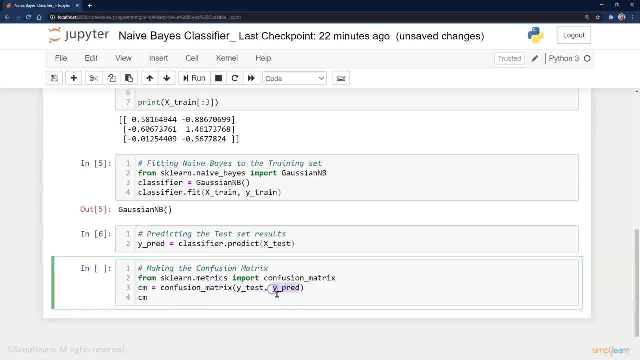 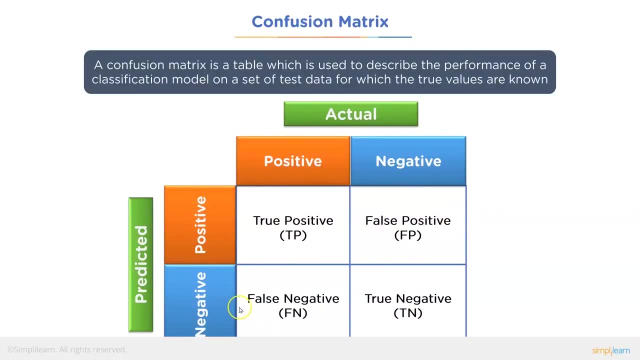 So we have our actual and we have our predicted value And you can see from here- this is the chart we looked at- Here's predicted. So true positive, false positive, false negative, true negative. And if we go ahead and run this, 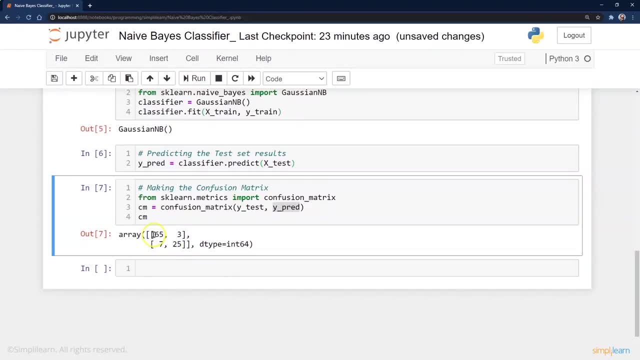 there we have it: 65,, 3,, 7,, 25.. And in this particular prediction we had 65 were predicted. the truth as far as a purchase: They're going to make a purchase And we guessed three wrong. 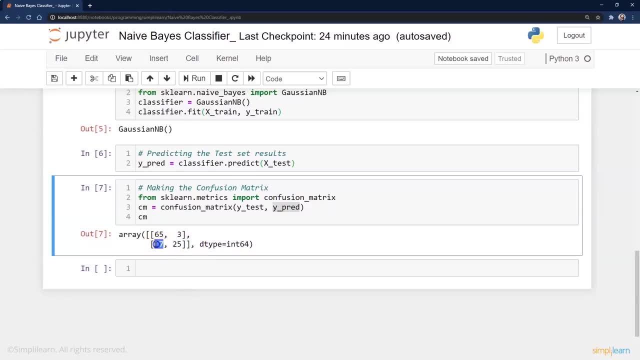 And then we had 25 we predicted would not purchase and seven of them did. So there's our confusion matrix. At this point, if you were with your shareholders or a board meeting, you would start to hear some snoozing if they were looking at the numbers. 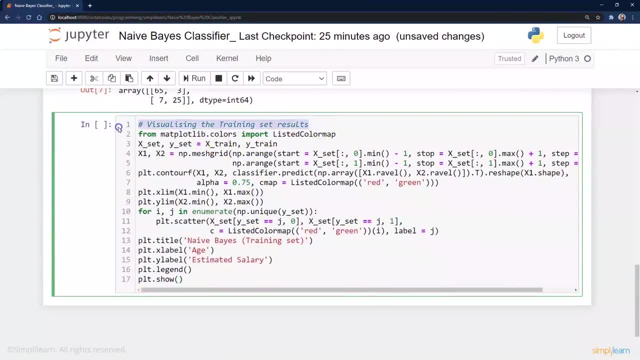 And you say, hey, here's my confusion- matrix. So let's go ahead and visualize the results And we're going to pull from the Matplot library colors, import listed color map. And this is actually my machine's going to throw an error. 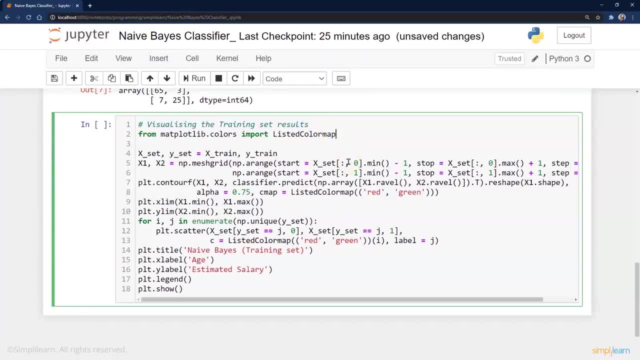 because this is being because of the way the setup is- I have a newer version on here than when they put together the demo- And we need our X set and our Y set, which is our X train and Y train, And then we'll create our X1, X2.. 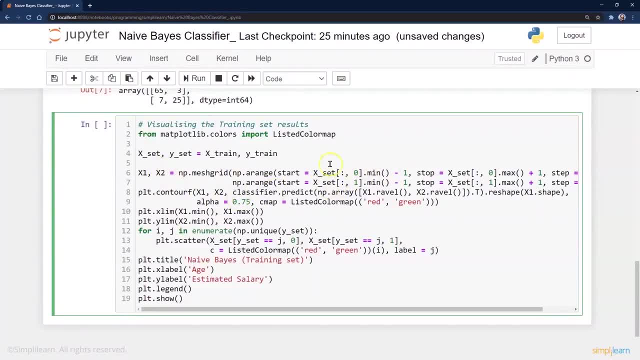 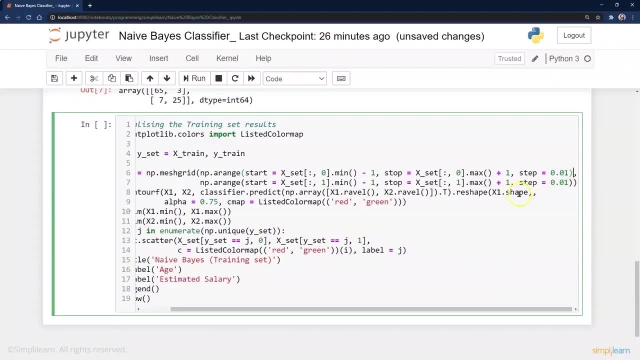 And we'll put that into a grid And we set our X set minimum stop and our X set max stop And if you come all the way over here, we're going to step 0.01.. This is going to give us a nice line. 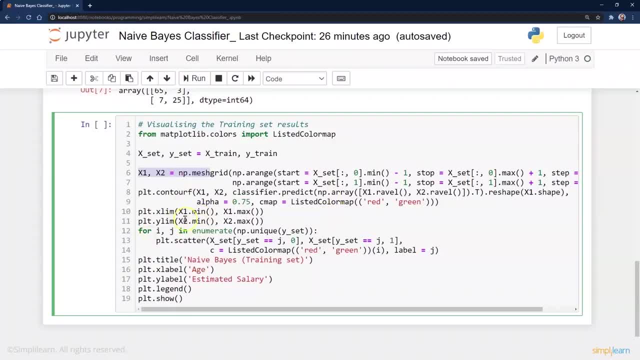 is what that's doing. And then we're going to plot the contour, plot the X limit, plot the Y limit and put the scatter plot in there. Now let's go ahead and run this. To be honest, when I'm doing these graphs, 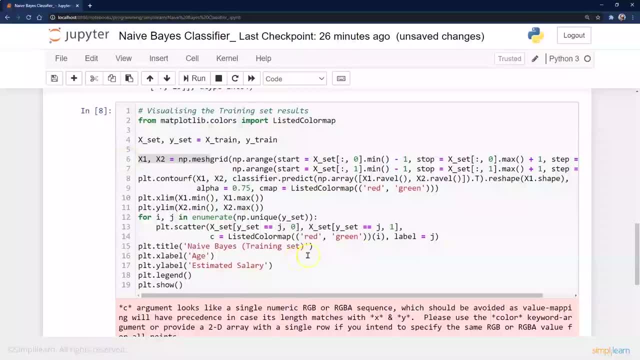 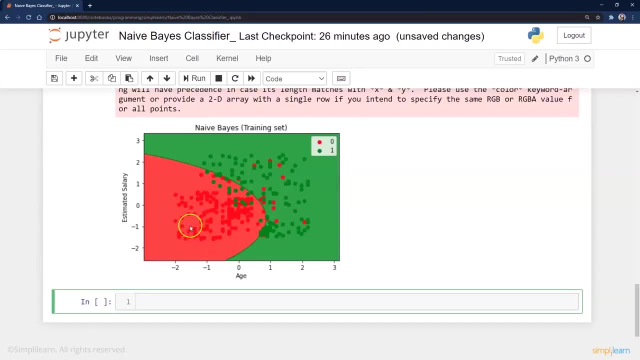 there's so many different ways to do that. There's so many different ways to put this code together To show you what we're doing. it's a lot easier to pull up the graph and then go back up and explain it. So the first thing we want to note here: 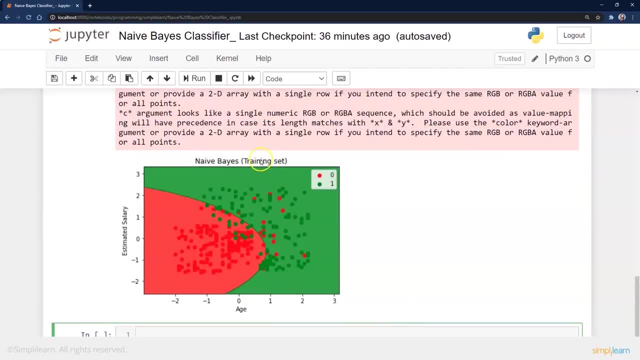 when we're looking at the data is: this is the training set. And so we have those who didn't make a purchase. We've drawn a nice area for that. It's defined by the Naive Bayes setup. And then we have those who did make a purchase. 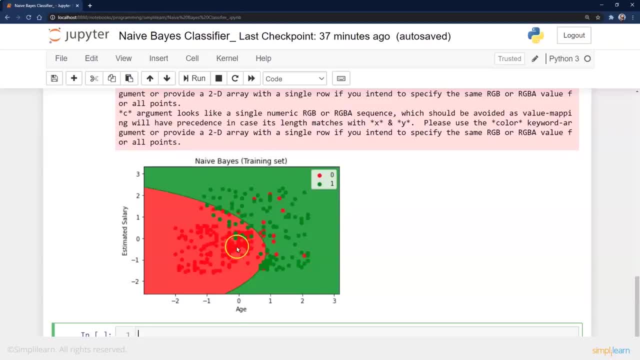 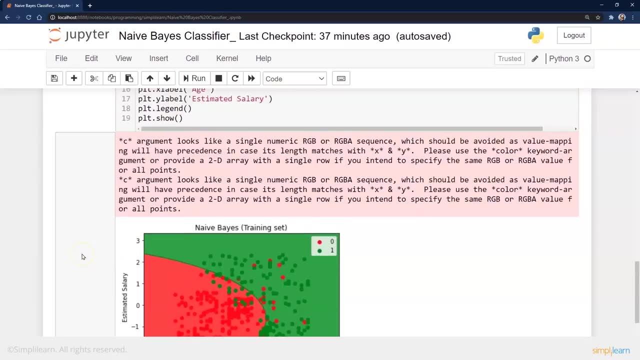 the green, And you can see that some of the green dots fall into the red area and some of the red dots fall into the green. So even our training set isn't going to be 100%. We couldn't do that, And so we're looking at our different data coming down. 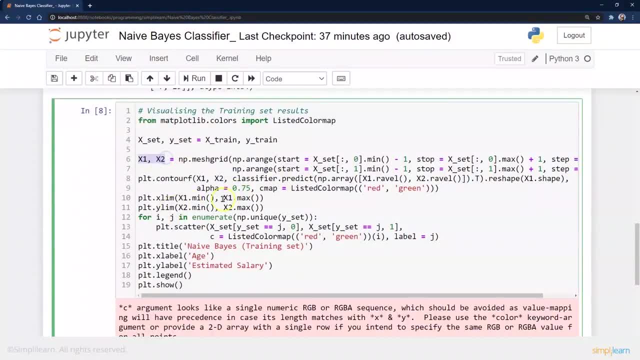 We can kind of arrange our X1, X2 so we have a nice plot going on And then we're going to create the contour. That's that nice line. That's that nice line that's drawn down the middle on here with the red green. 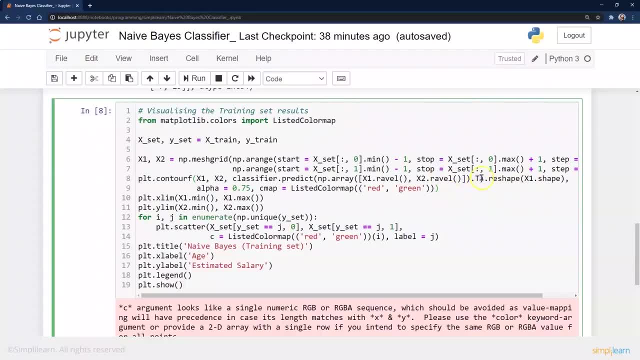 That's what this is doing right here with the reshape, And notice that we had to do the dot T. If you remember from NumPy, if you did the NumPy module, you end up with pairs X1, X2, X1, X2- next row, and so forth. 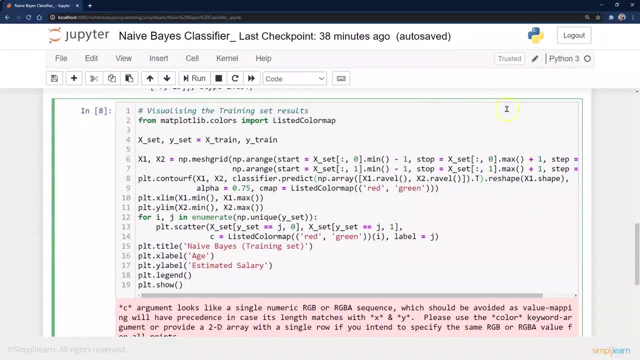 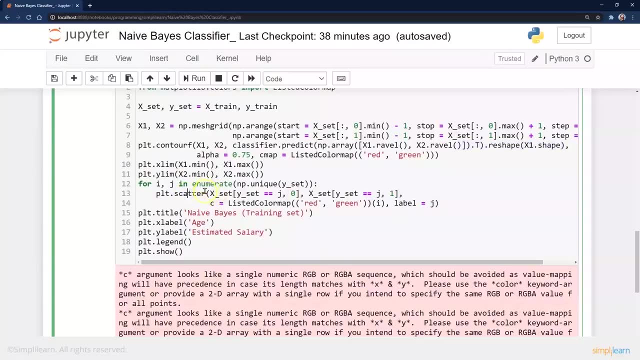 You have to flip it, so it's all one row. You have all your X1s and all your X2s. So this is what we're kind of looking for right here on this setup, And then the scatter plot is, of course, 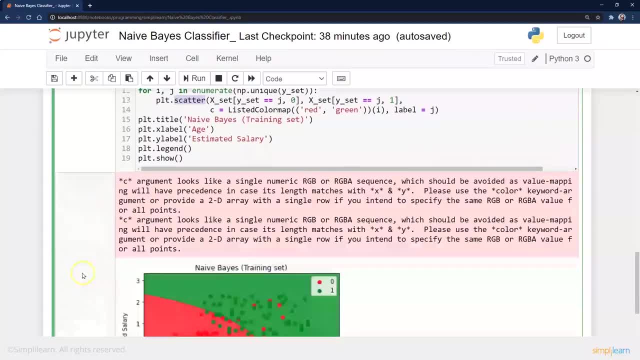 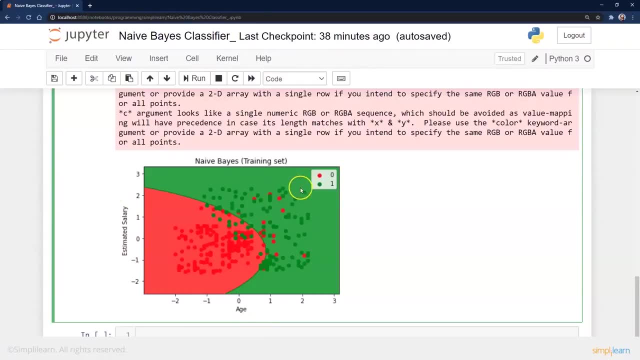 your scattered data across there. We're just going through all the points. That puts these nice little dots onto our setup on here And we have our estimated salary and our age, And then, of course, the dots are: did they make a purchase or not? 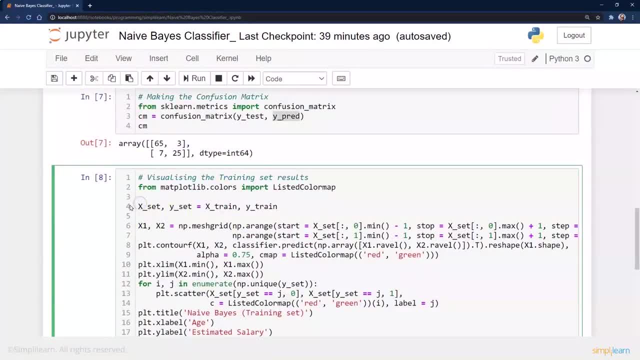 And just a quick note. this is kind of funny. You can see up here where it says Xset, Yset equals Xtrain, Ytrain, which seems kind of a little weird to do. This is because this is probably originally a definition. 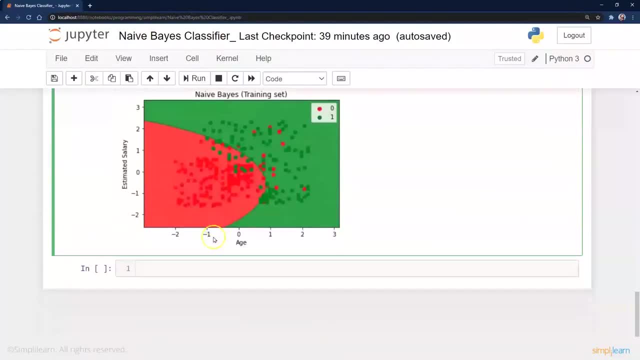 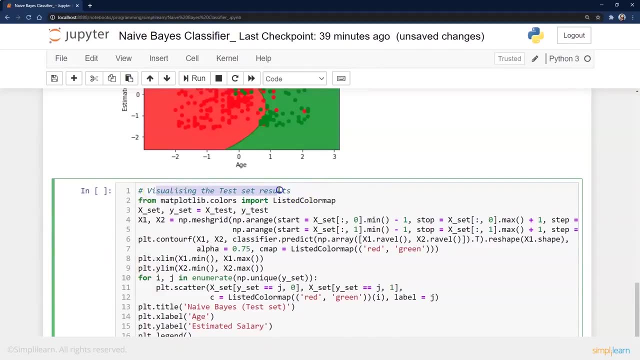 So it's its own module that could be called over and over again, which is really a good way to do it, because the next thing we're going to want to do is do the exact same thing, but we're going to visualize the test set results. 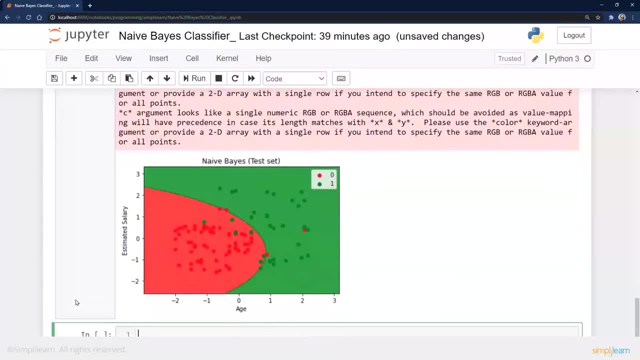 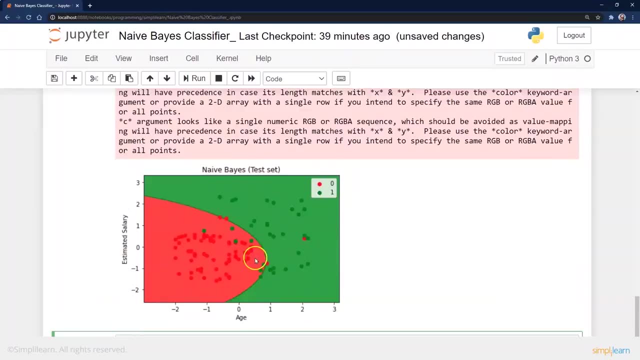 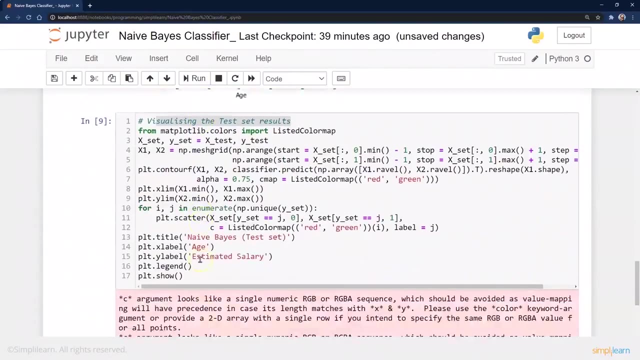 That way we can see what happened with our test group, our 25%, And you can see down here. we have the test set And if you look at the two graphs next to each other, this one obviously has 75%, So it's going to show a lot more. 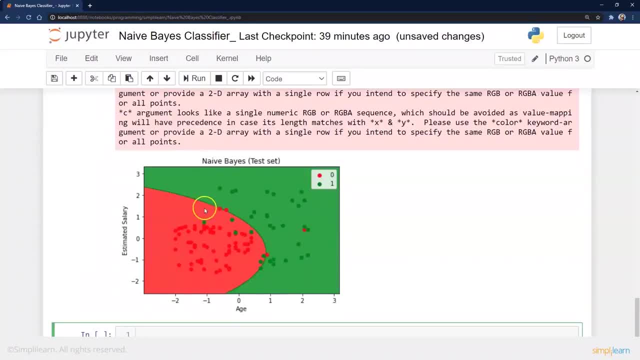 This is only 25% of the data. You can see that there's a number that are kind of on the edge as to whether they could guess by age and income they were going to make a purchase or not. But that said, it still is pretty clear. 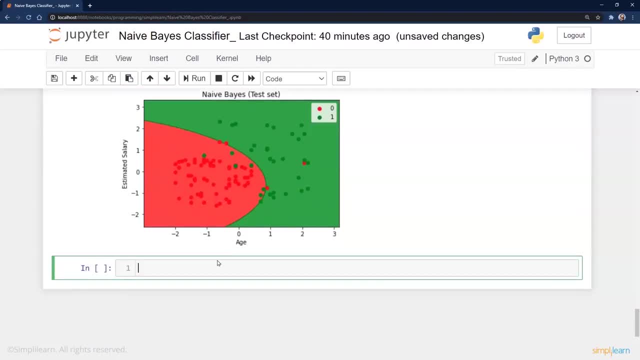 It's pretty good as far as how much the estimate is and how good it does. Now, graphs are really effective for showing people what's going on, But you also need to have the numbers, And so we're going to do from sklearn. 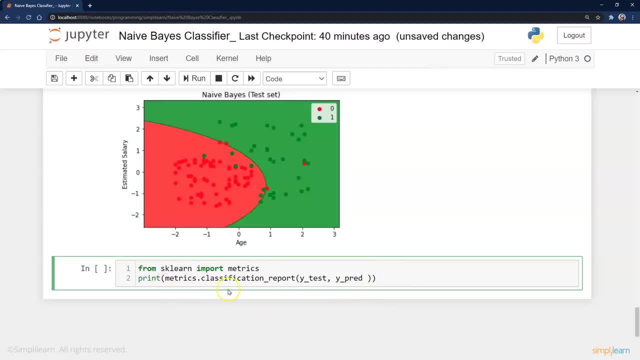 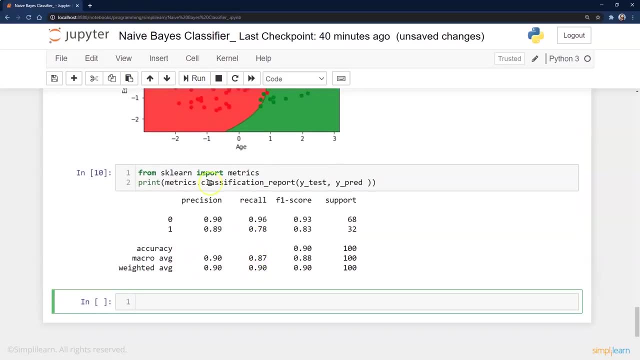 we're going to import metrics And then we're going to print our metrics classification report from the Y test and the Y predict And you can see here we have precision. The precision of zeros is 90.. There's our recall: 0.96. 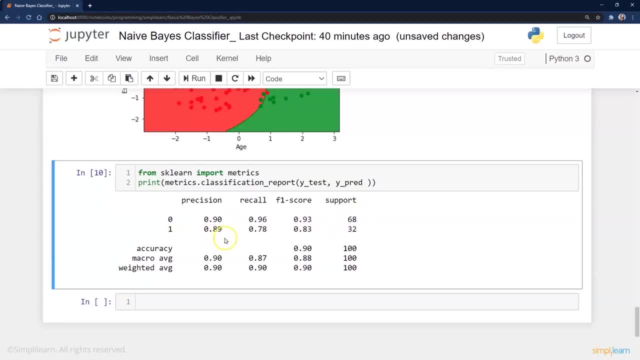 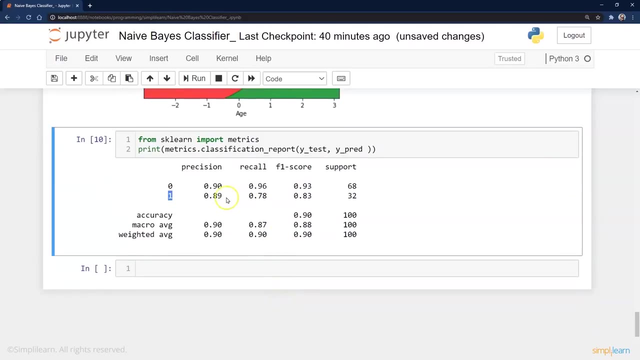 We have an F1 score and a support And we have our precision, the recall on getting it right, And then we can do our accuracy, the macro average and the weighted average. So you can see it pulls in pretty good as far as how accurate it is. 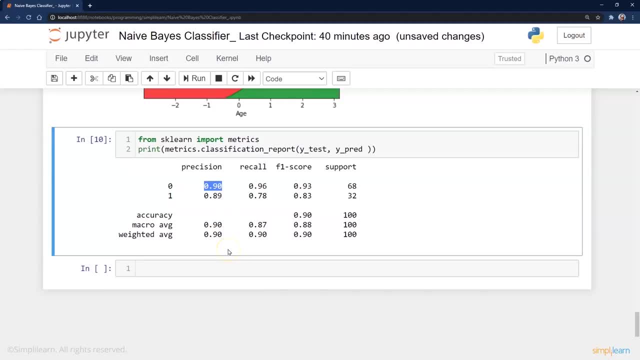 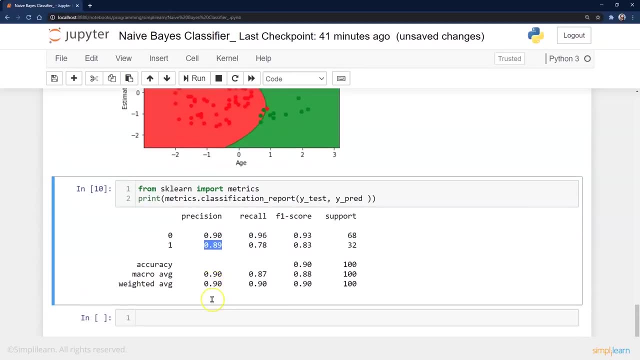 You could say it's going to be about 90% is going to guess correctly that they're not going to purchase And we had an 89% chance that they are going to purchase. And then the other numbers as you get down have a little bit different meaning.